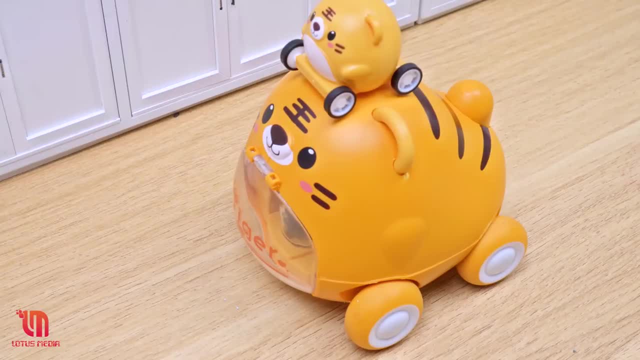 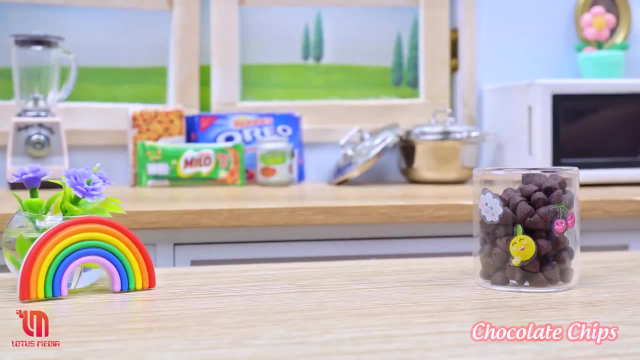 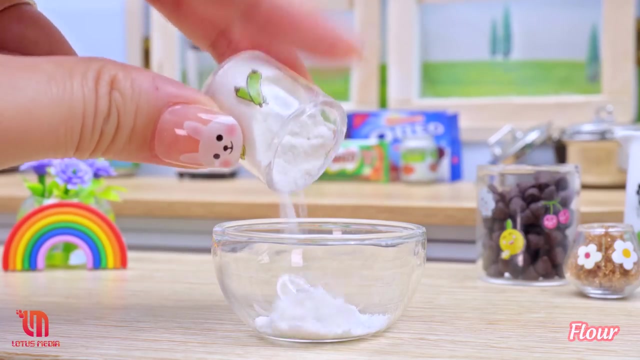 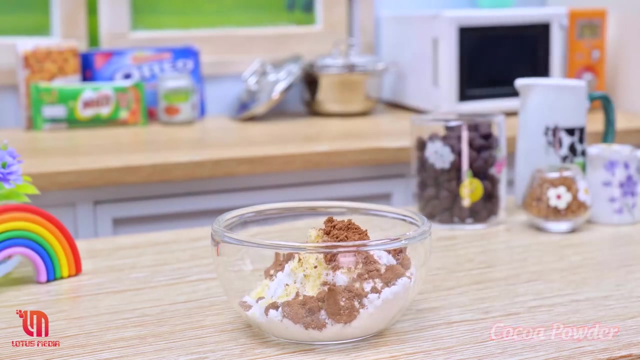 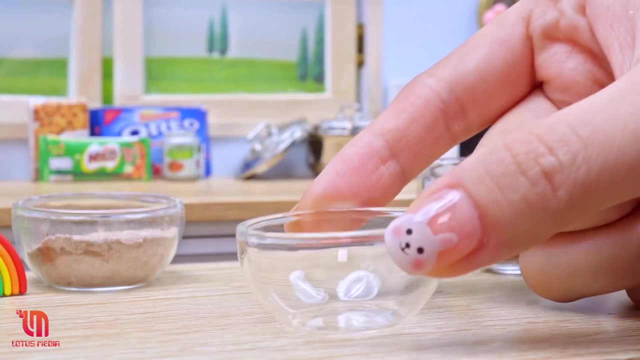 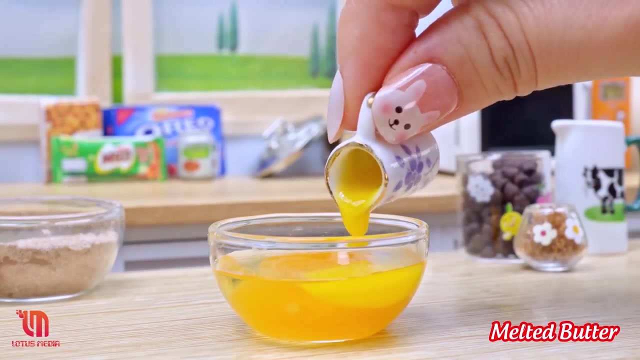 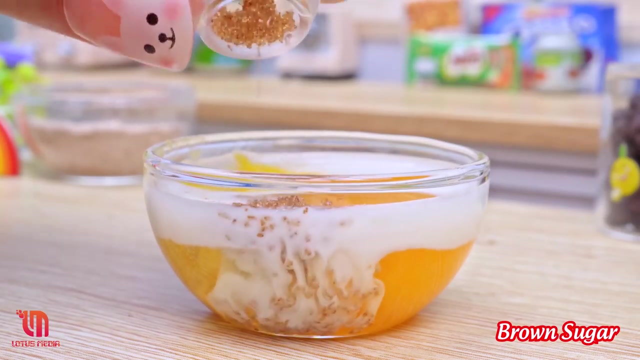 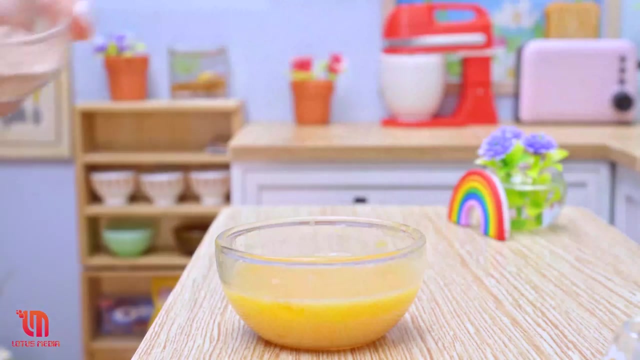 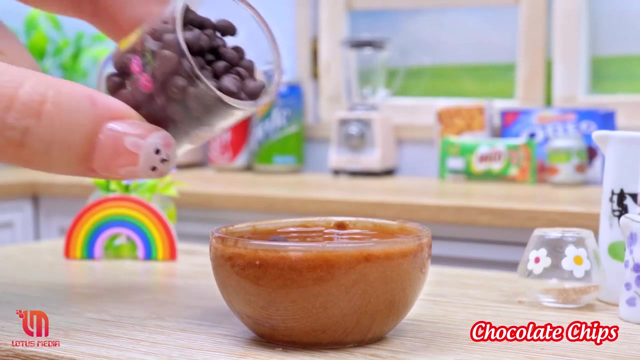 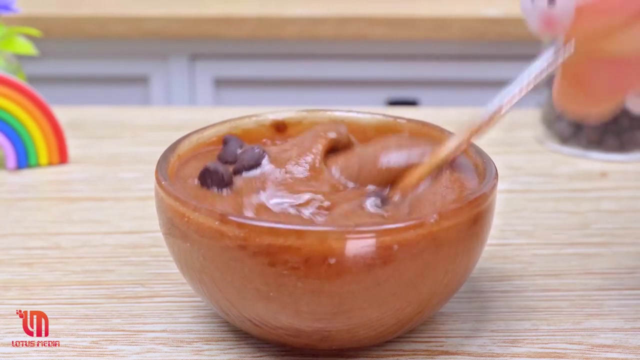 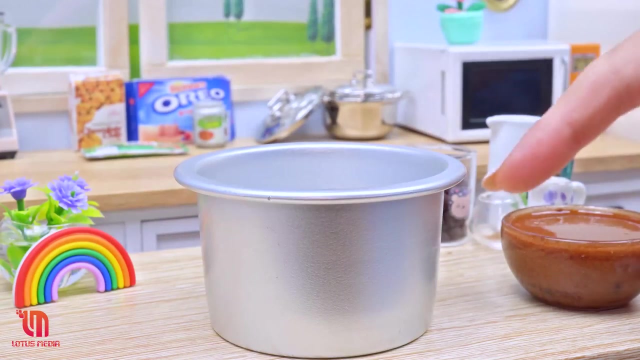 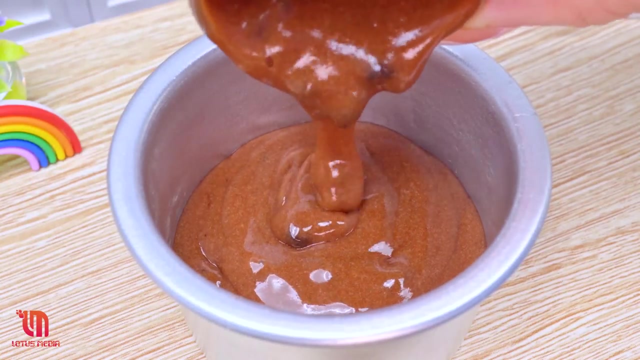 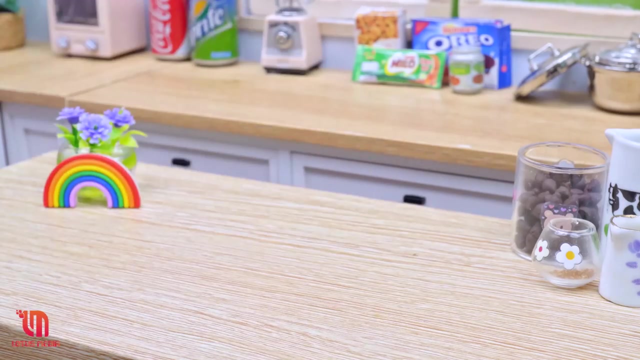 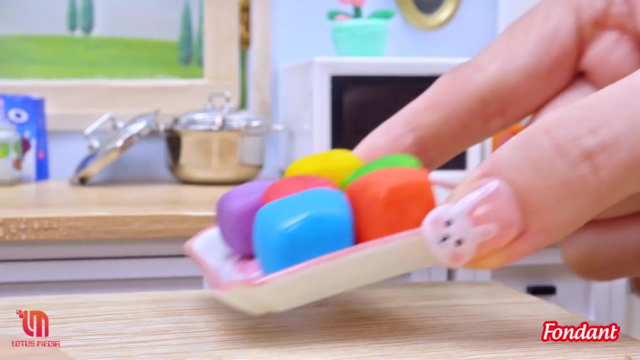 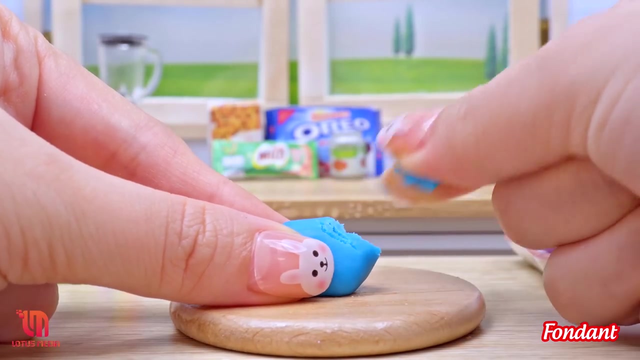 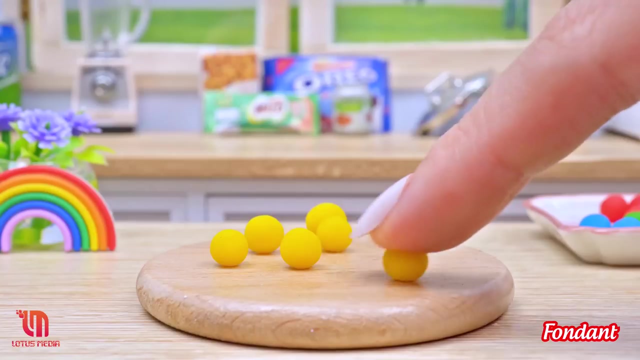 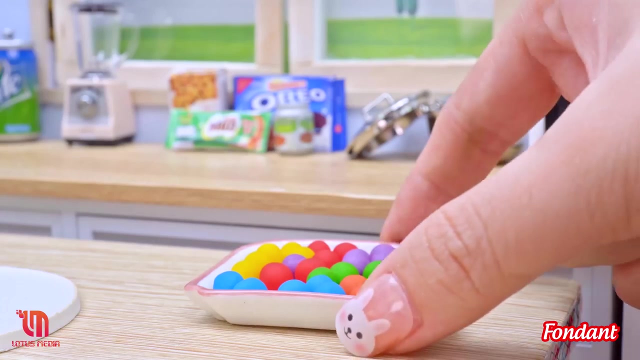 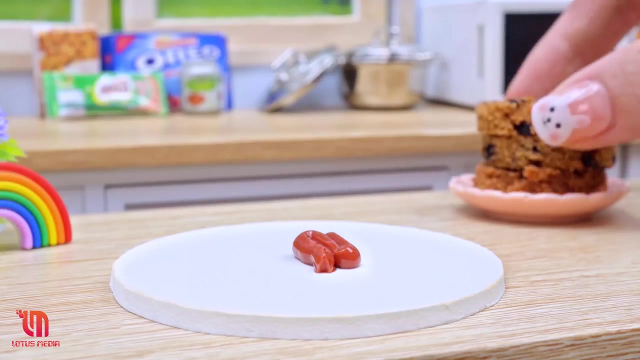 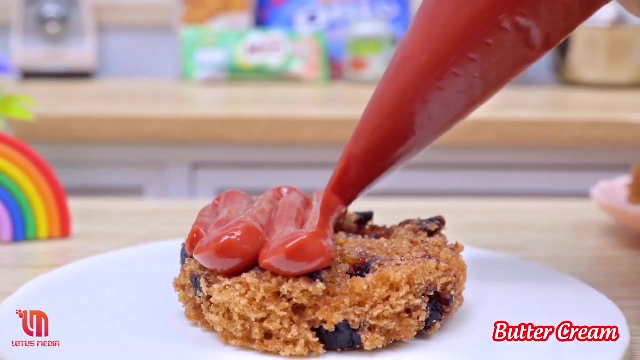 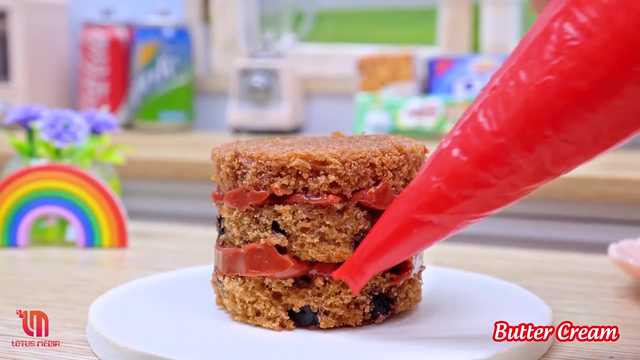 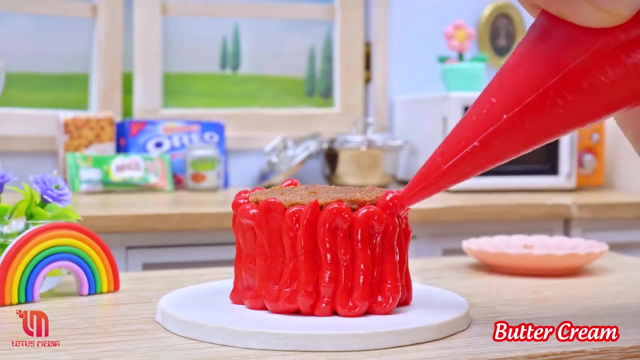 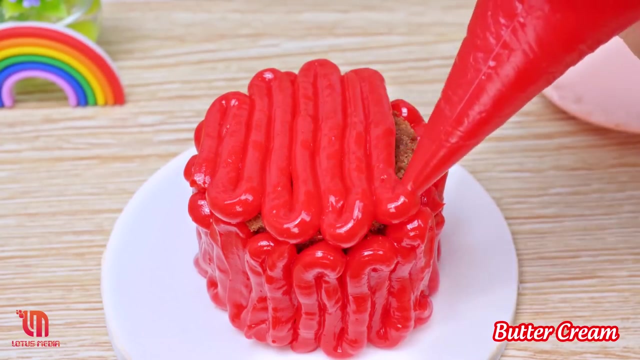 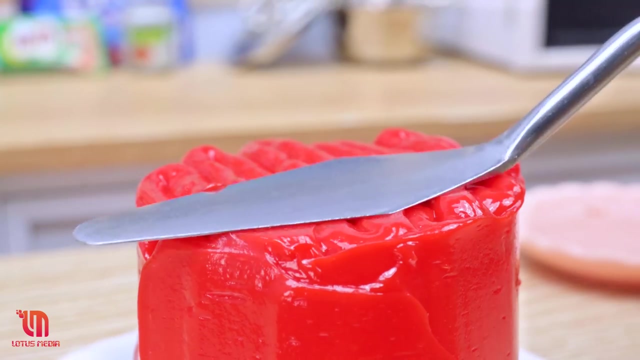 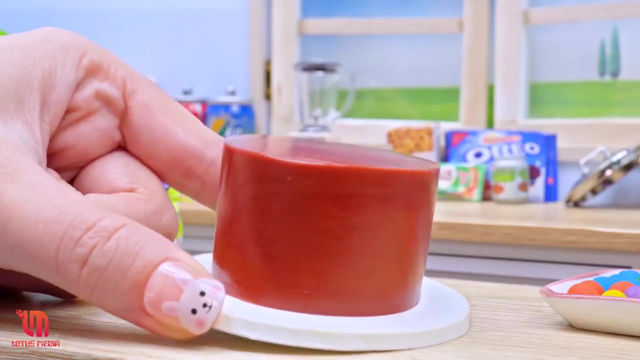 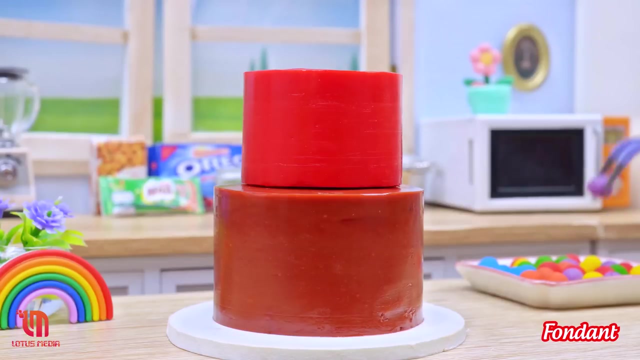 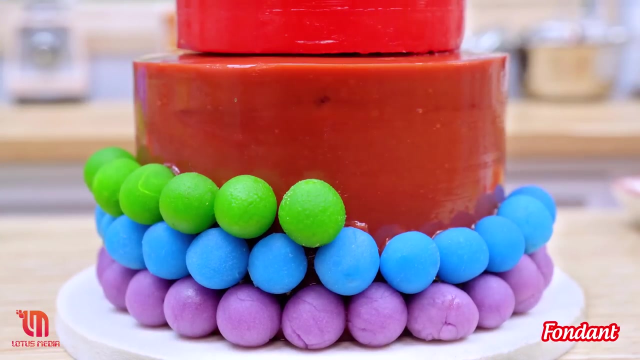 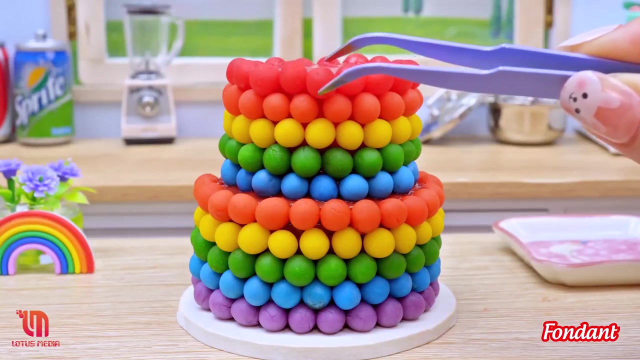 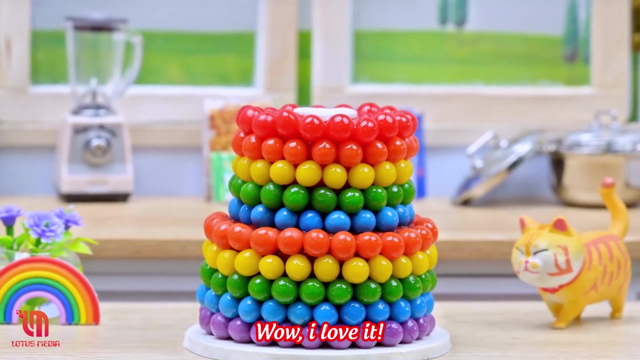 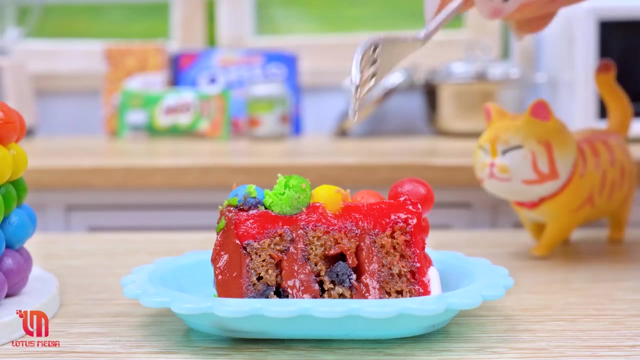 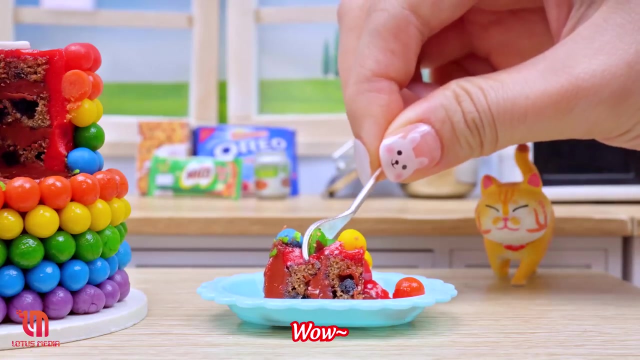 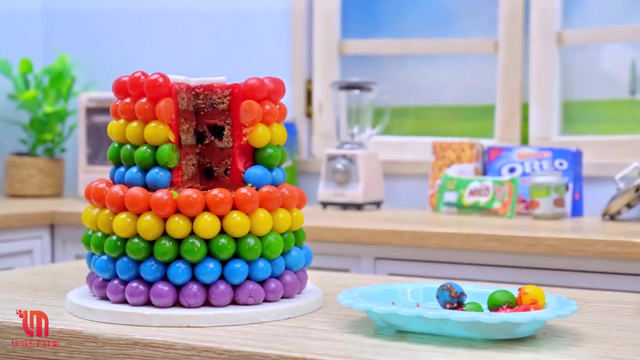 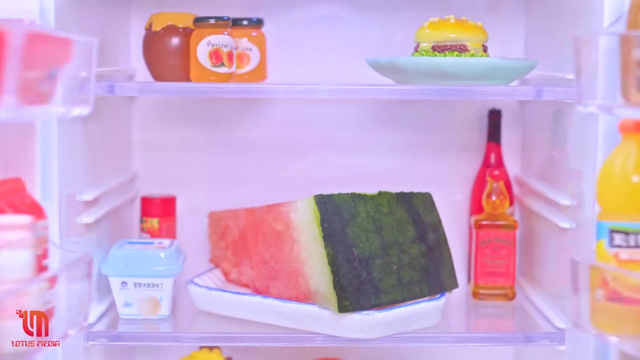 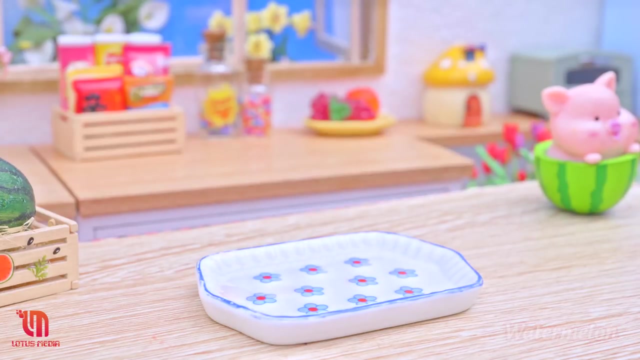 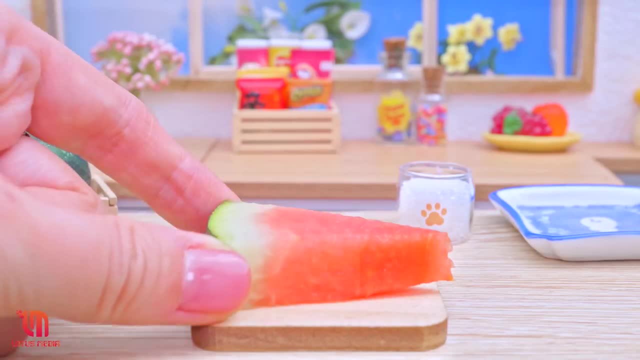 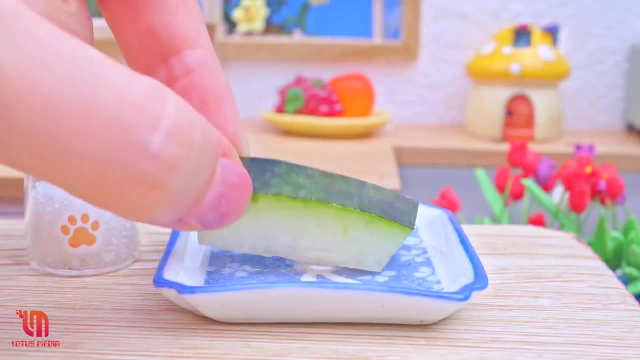 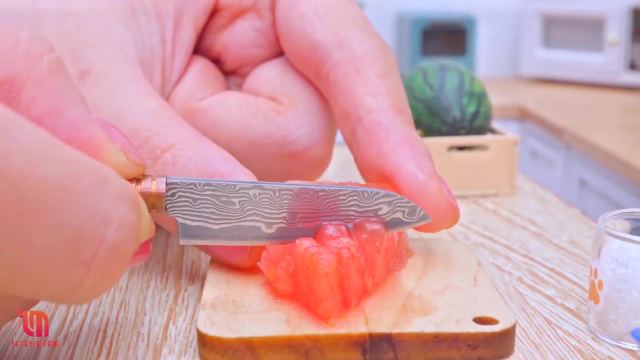 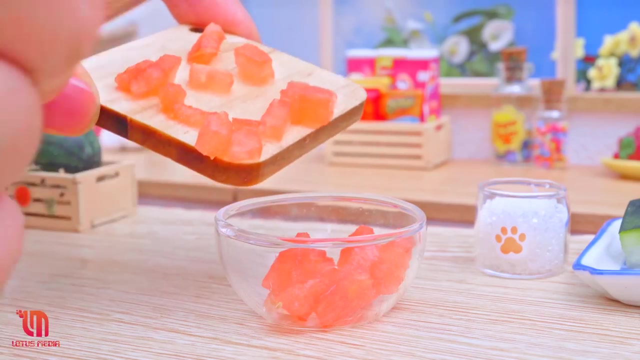 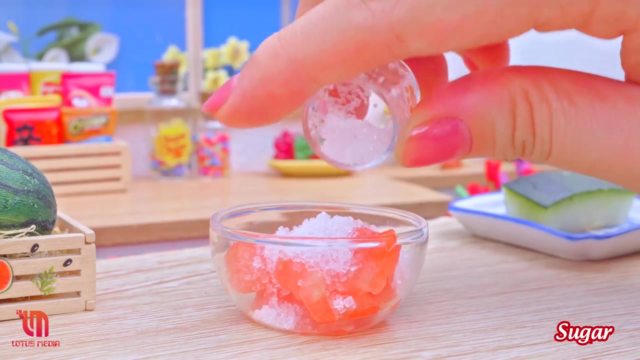 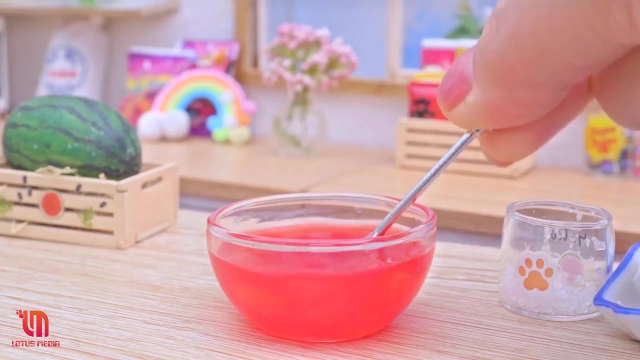 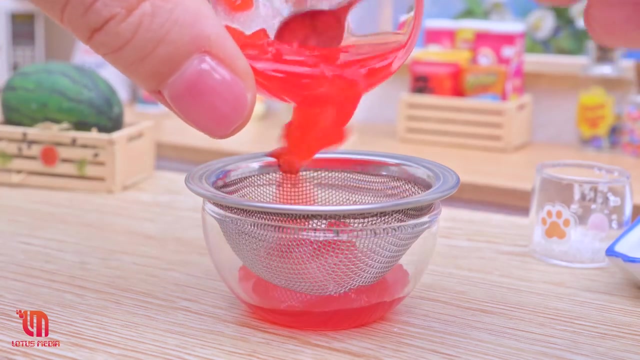 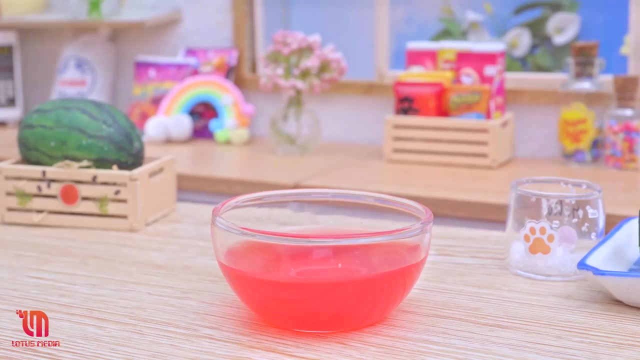 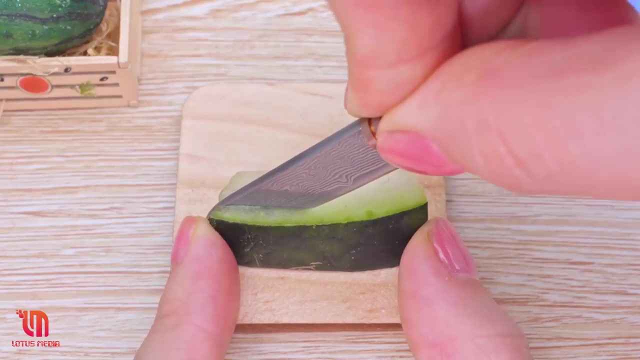 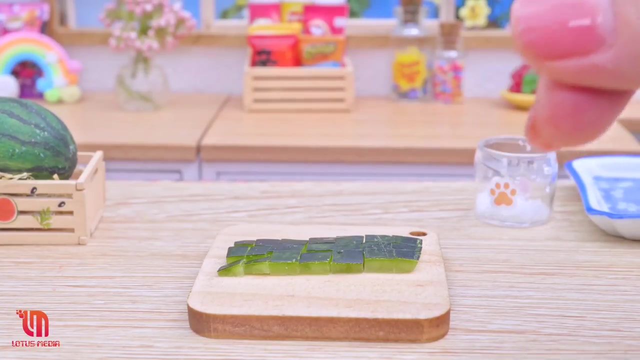 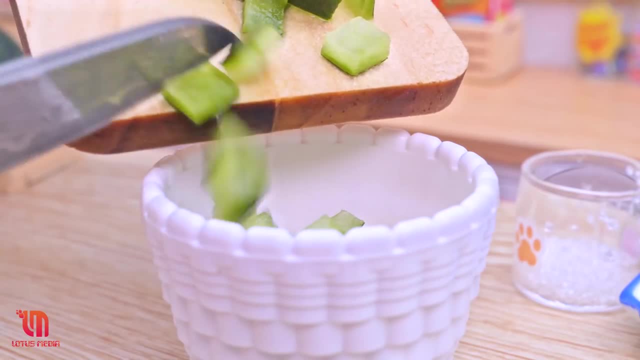 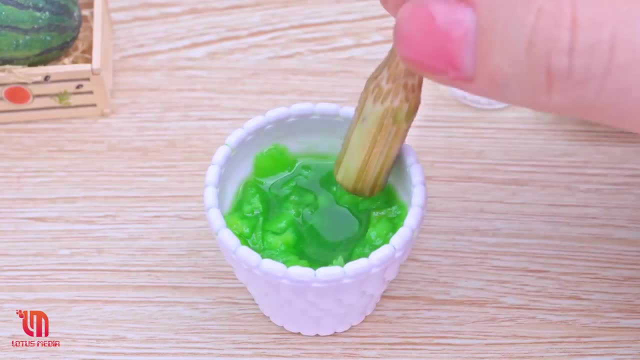 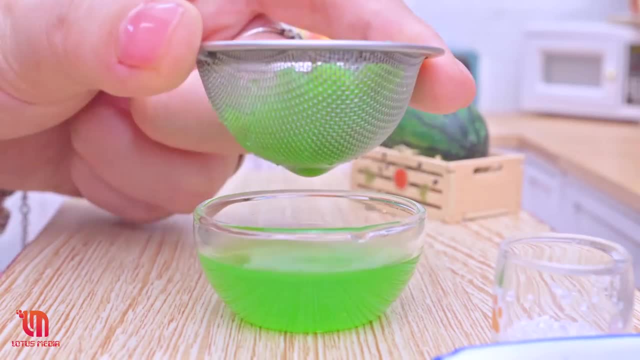 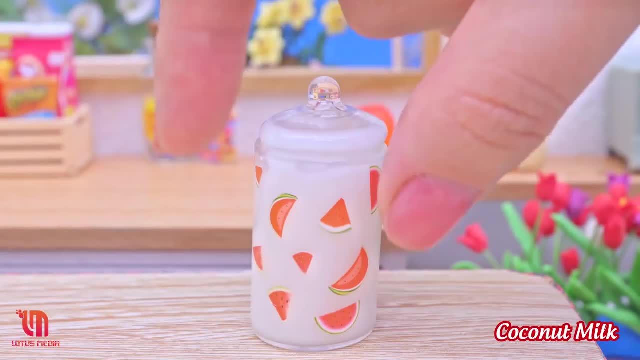 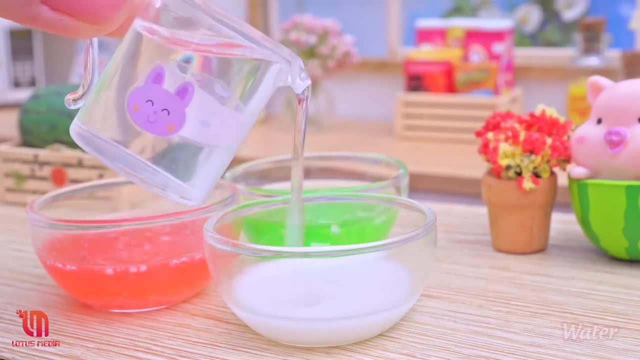 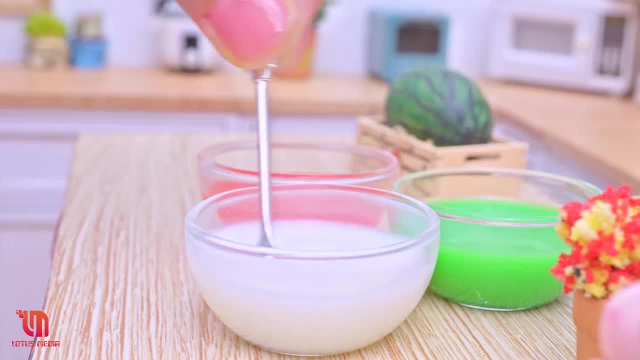 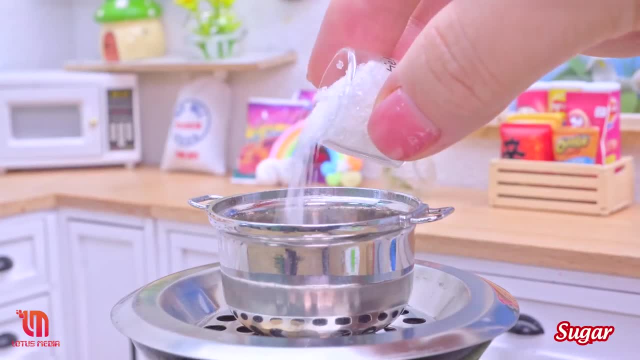 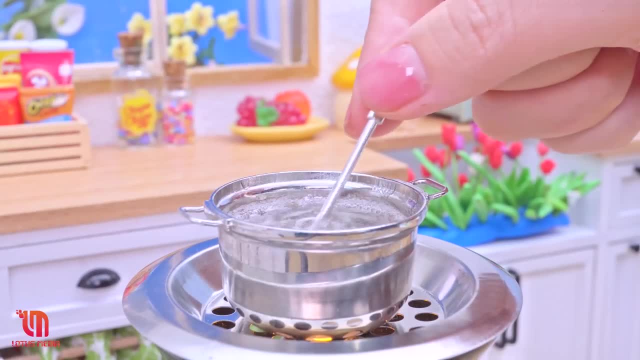 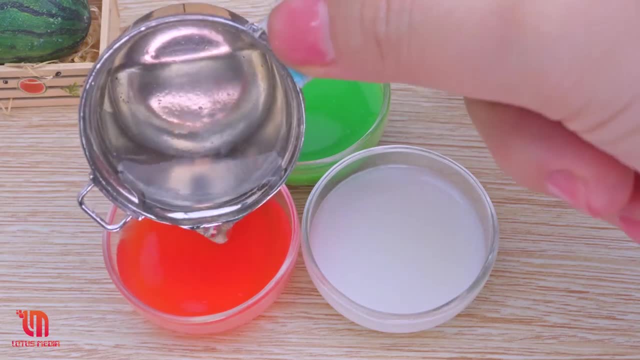 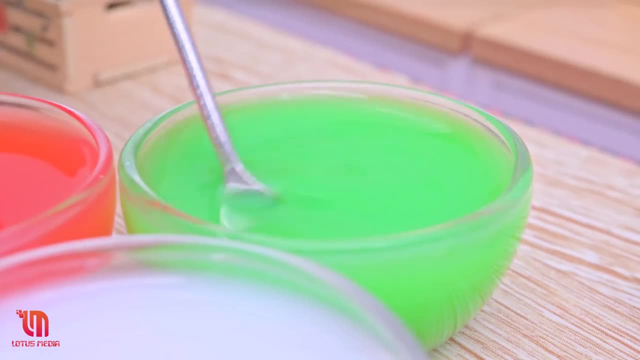 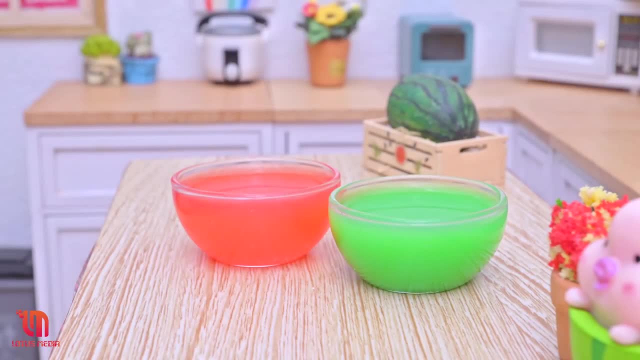 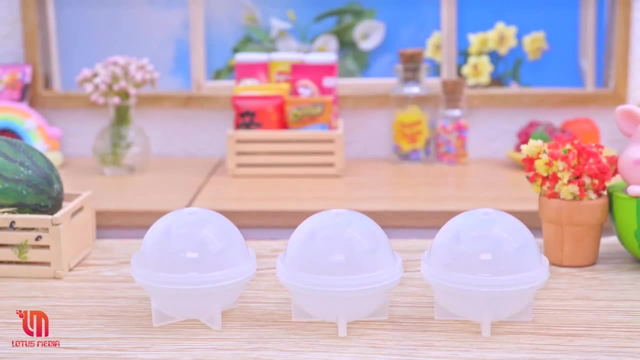 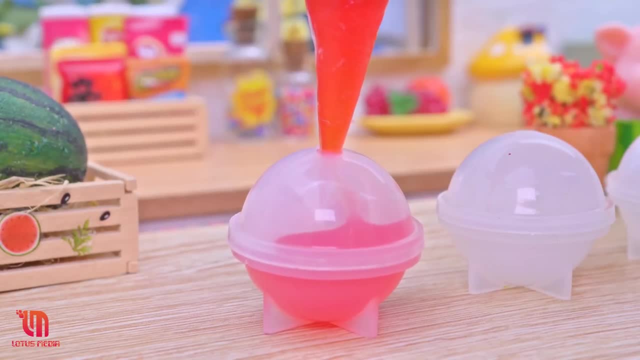 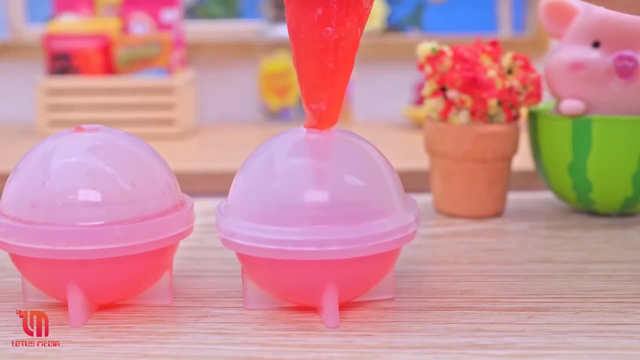 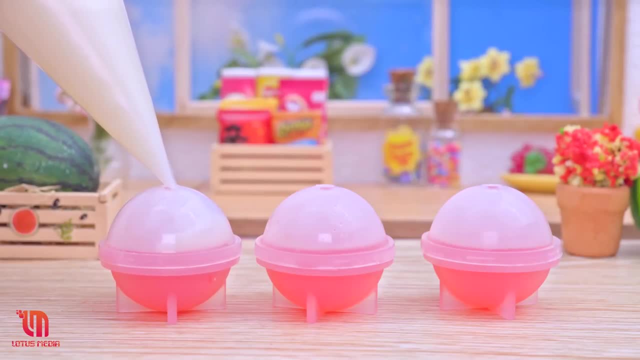 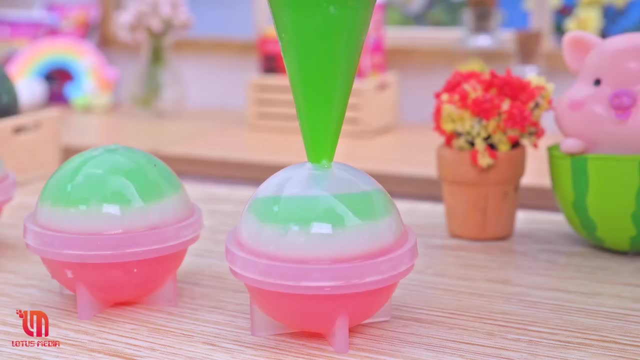 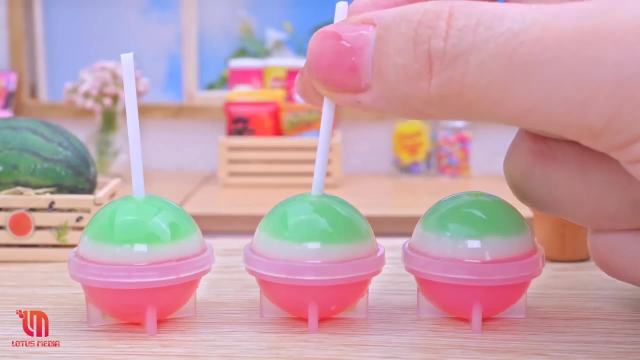 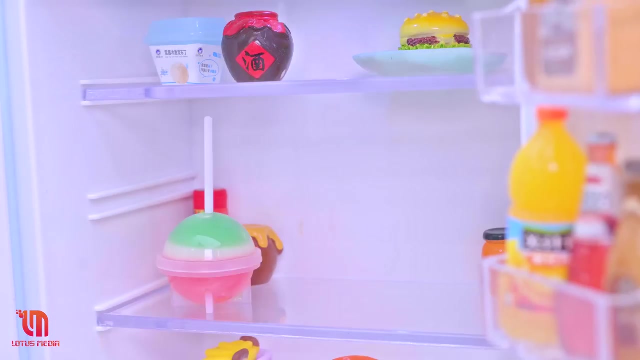 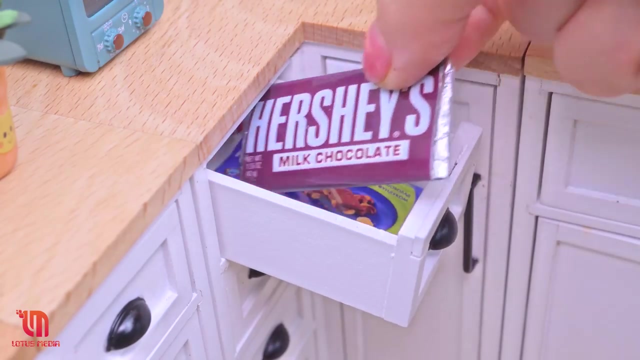 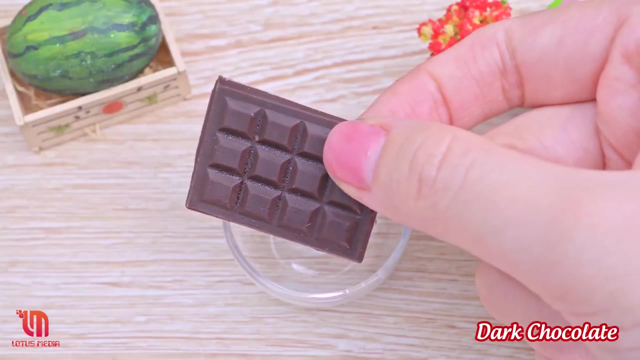 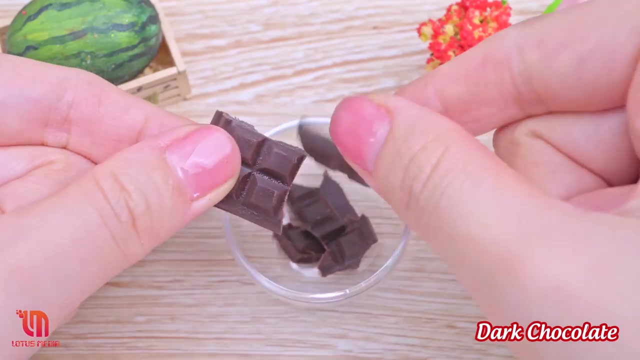 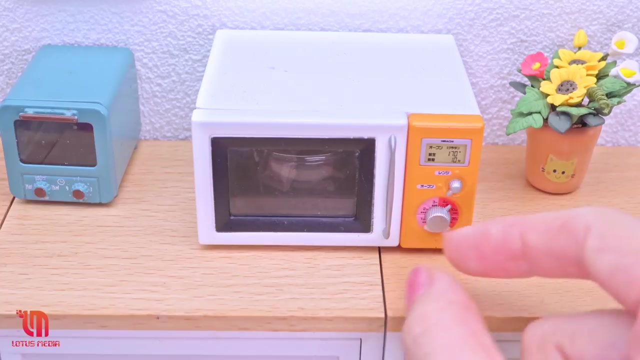 I'm going to cut it into small pieces and put it in the refrigerator for about an hour. I'm going to make a cake: 1 egg, 1 cup of milk, 50 grams of sugar, 1 tablespoon of wheat flour. 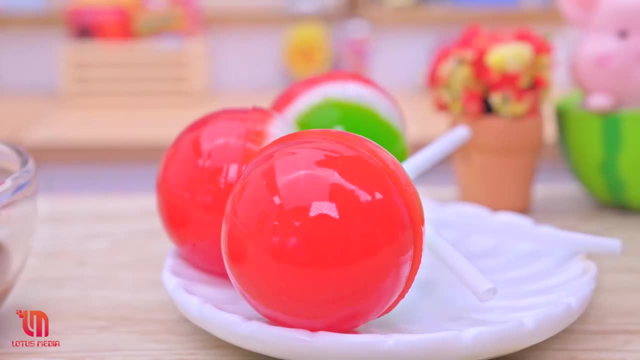 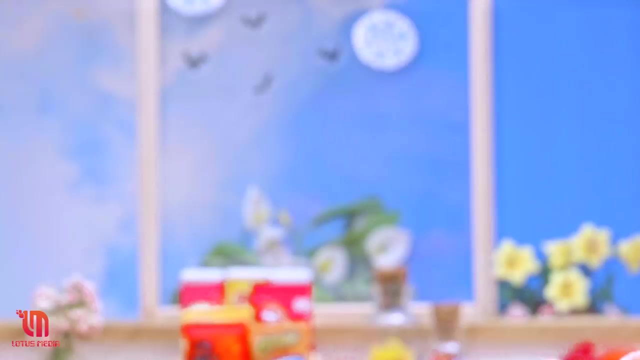 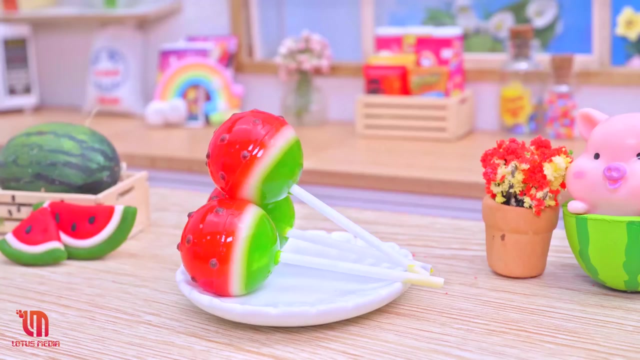 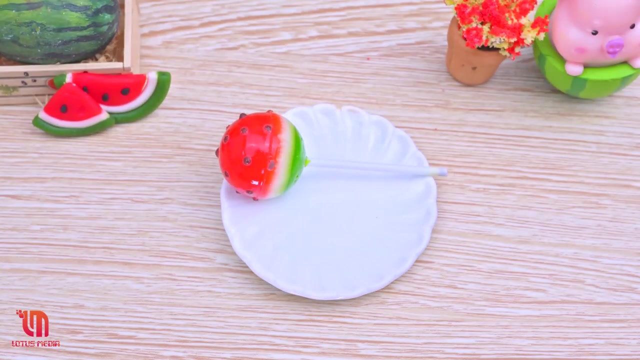 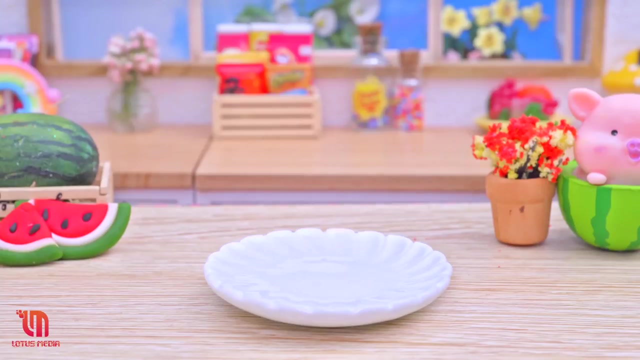 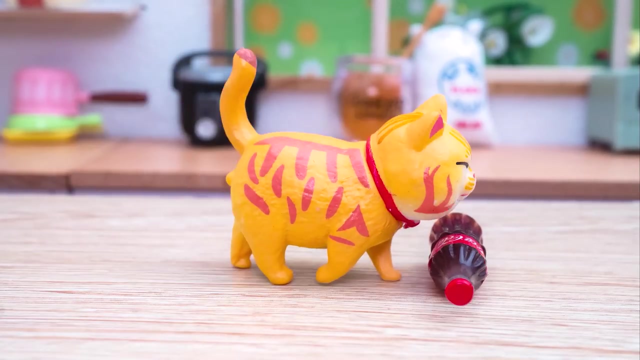 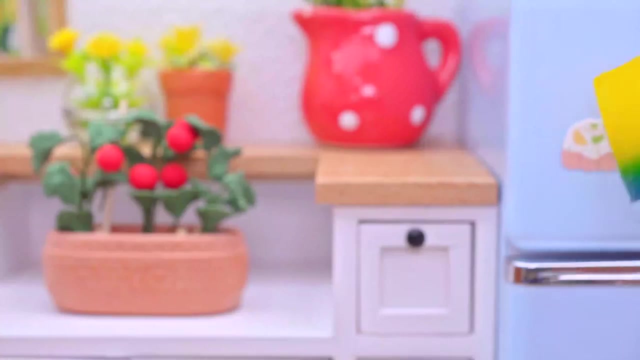 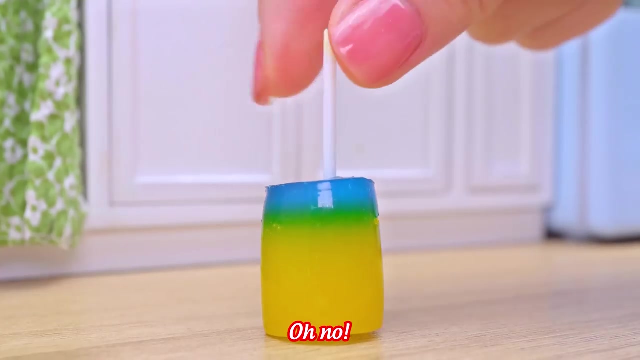 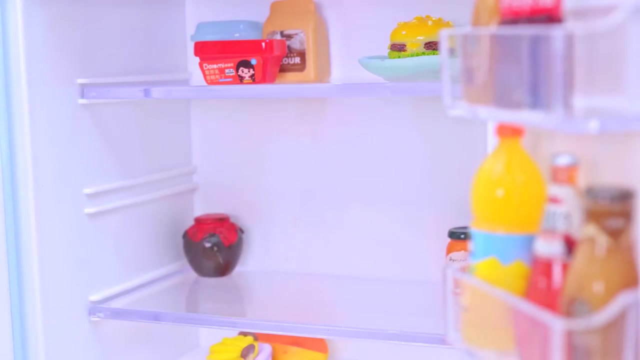 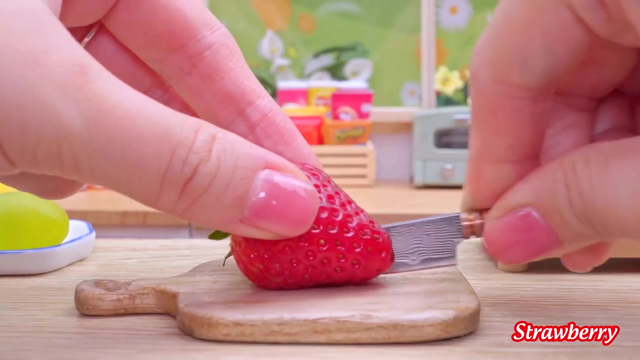 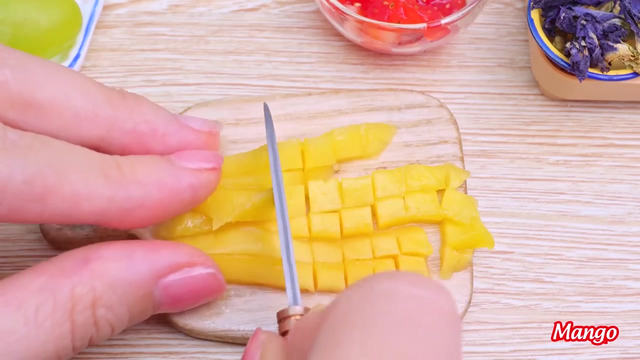 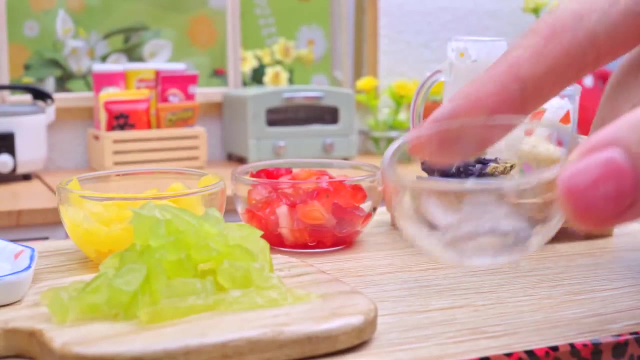 10 grams of salt: 1 teaspoon of salt. 1 tablespoon of sugar. 1 thousand grams of flour: 1 tablespoon of flour. Wow, I love it. Delicious Yummy. Oh no, Oh no, Oh no. 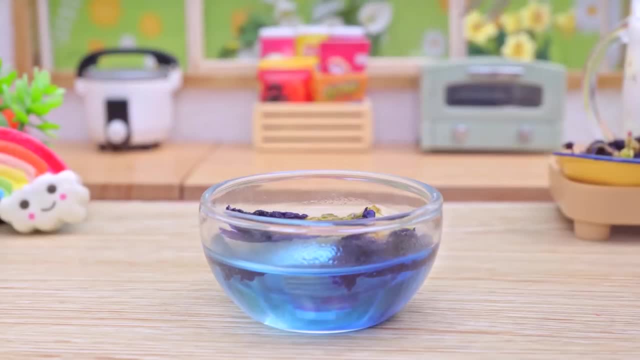 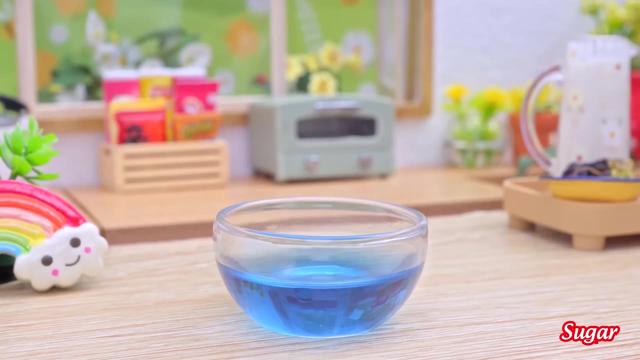 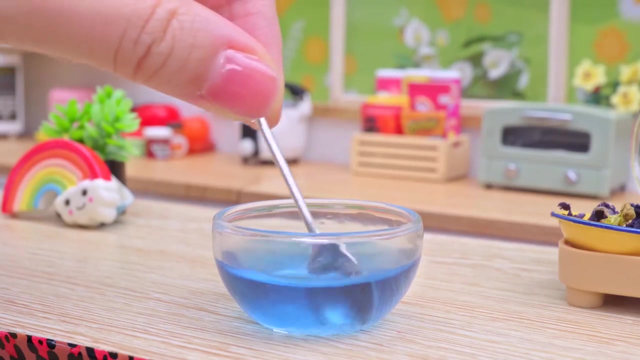 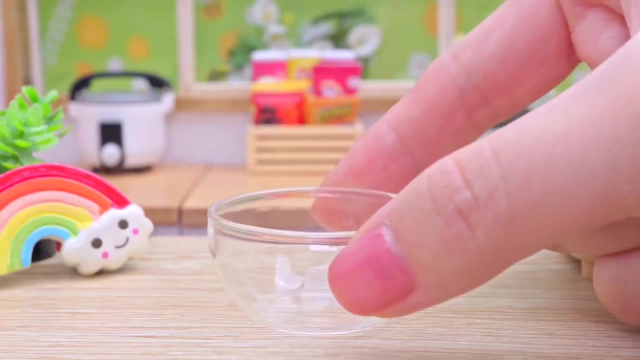 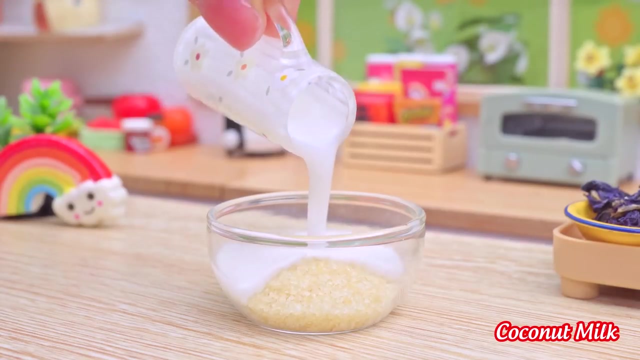 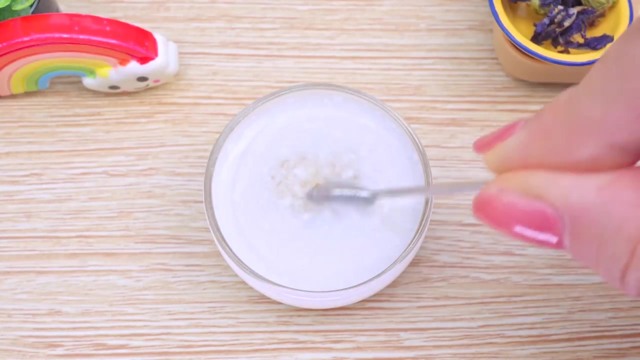 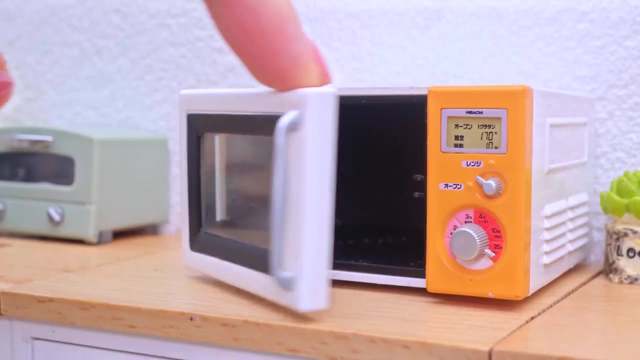 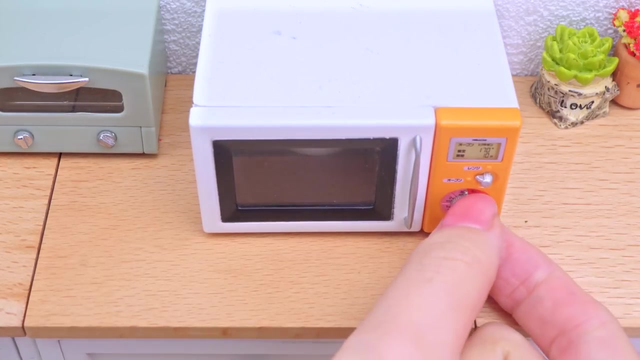 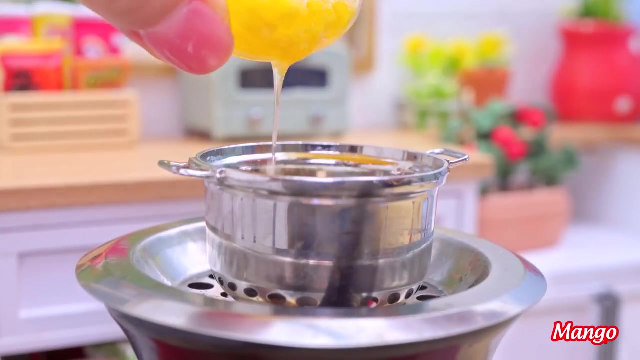 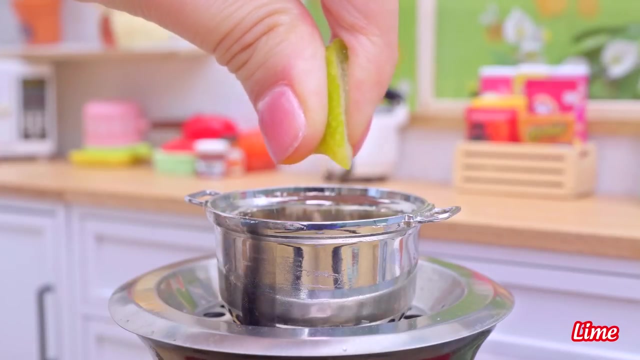 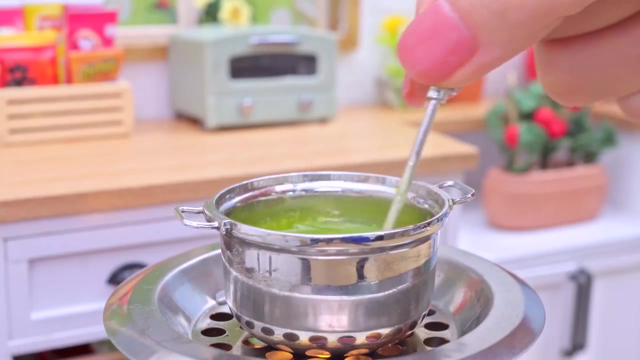 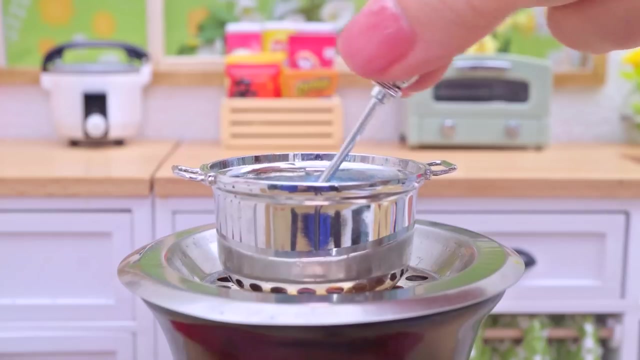 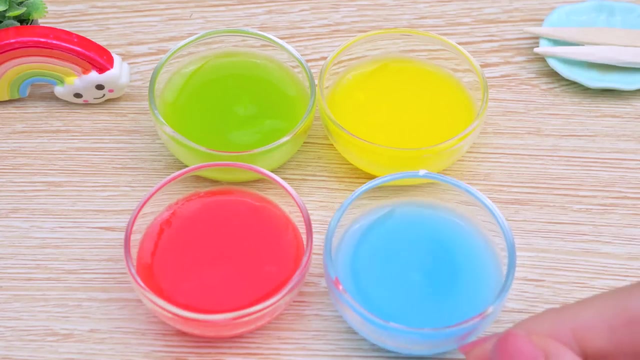 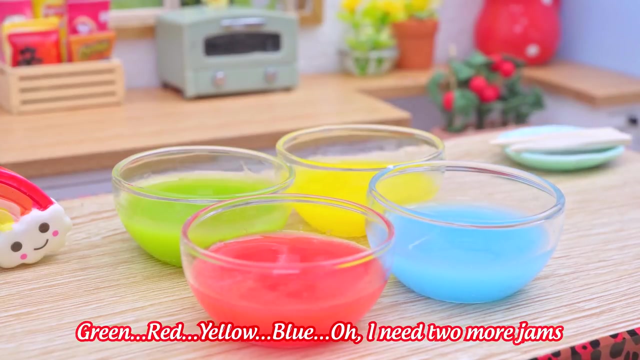 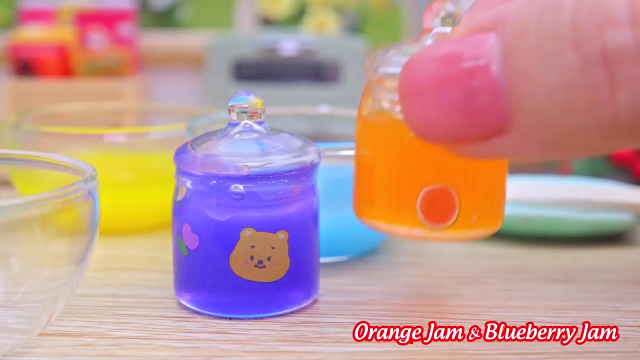 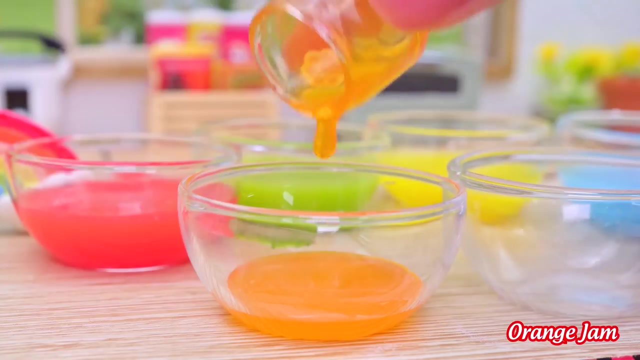 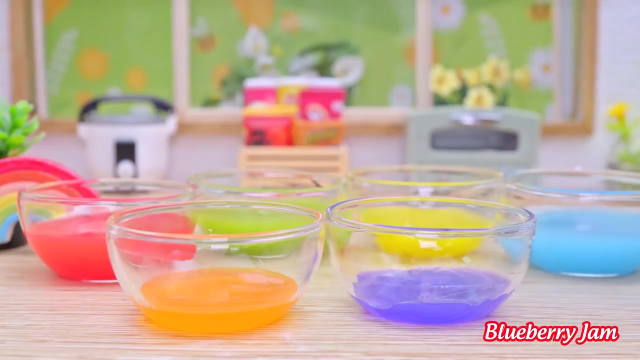 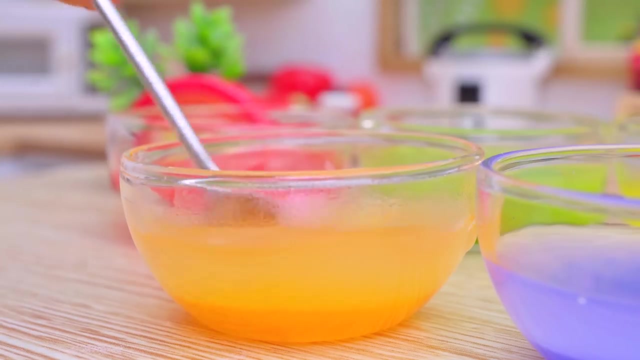 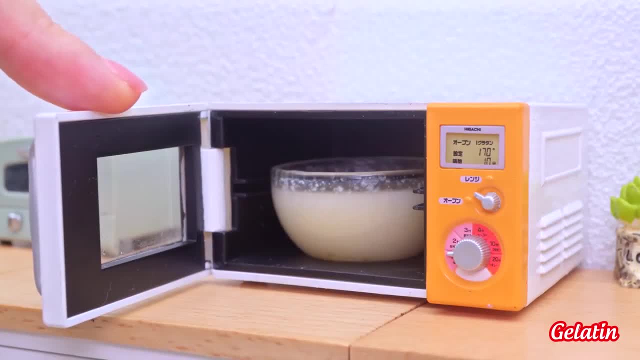 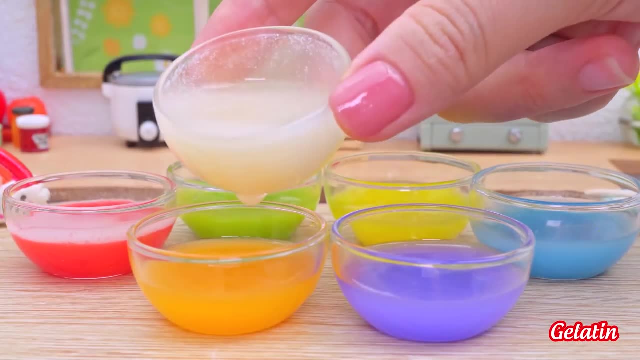 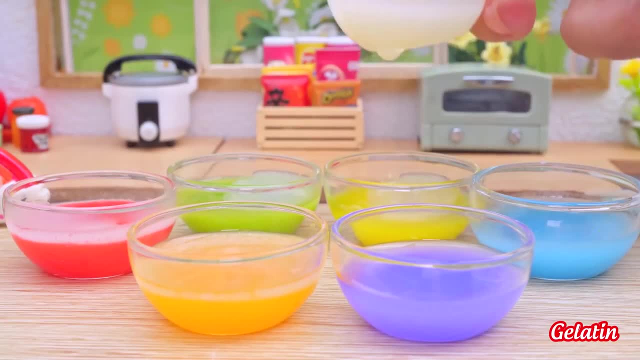 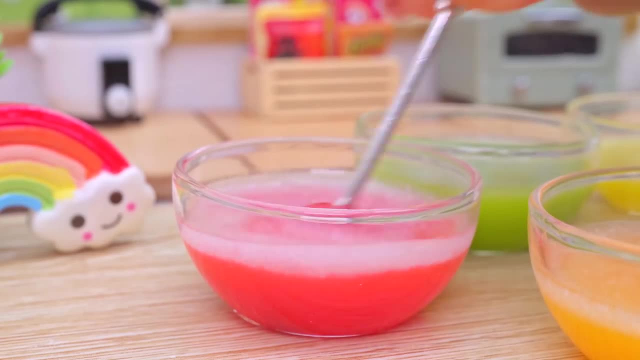 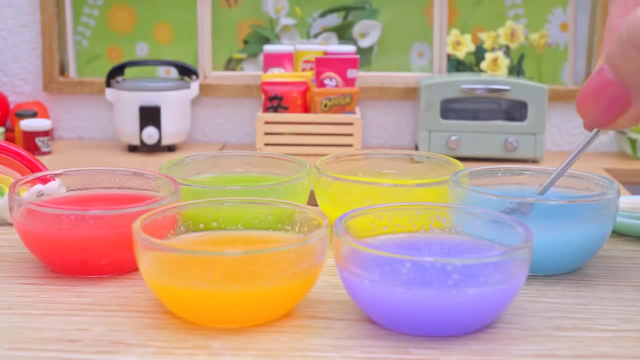 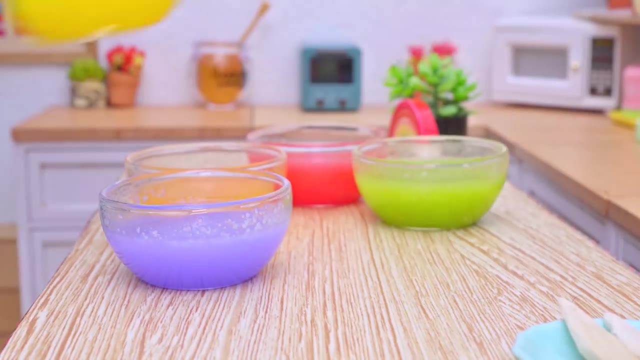 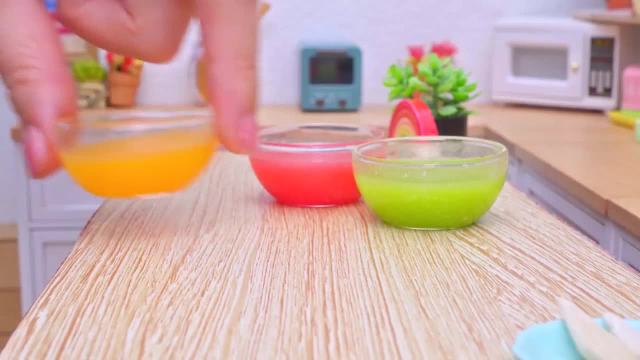 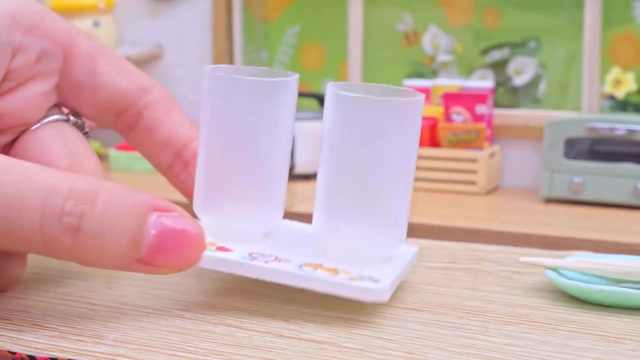 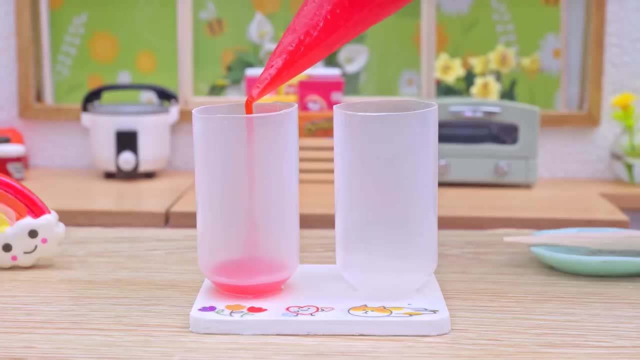 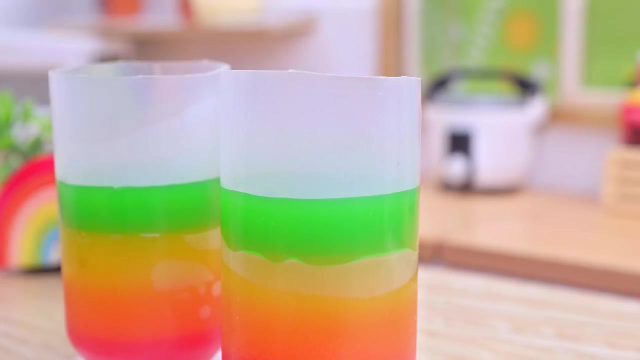 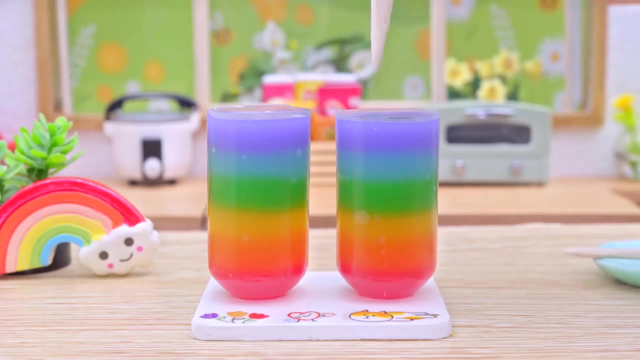 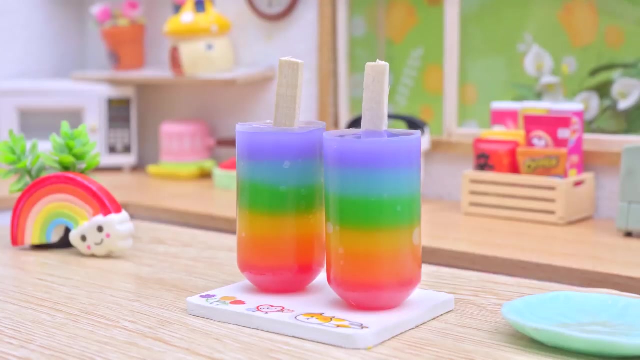 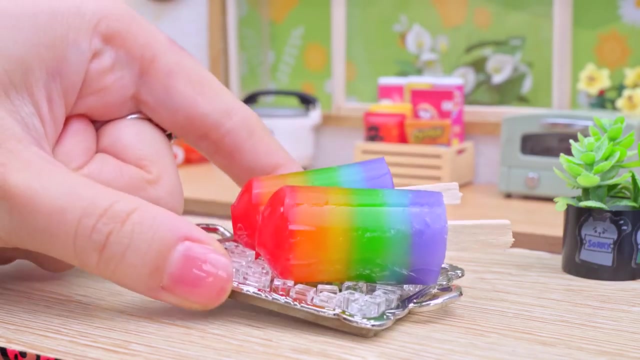 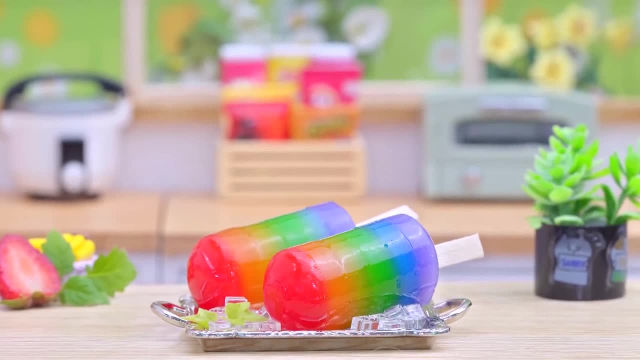 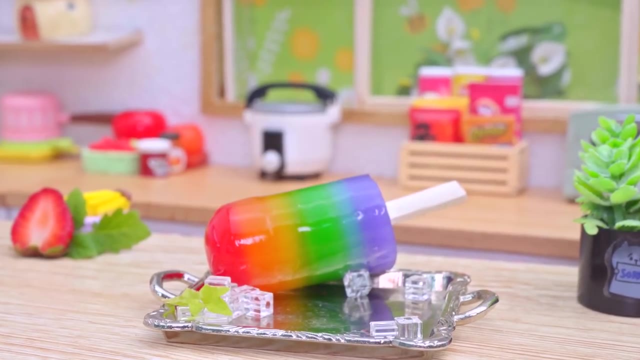 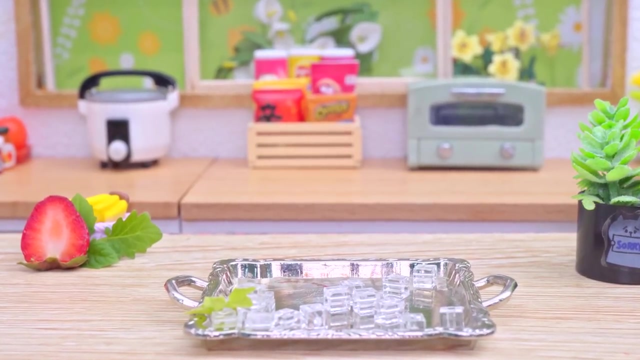 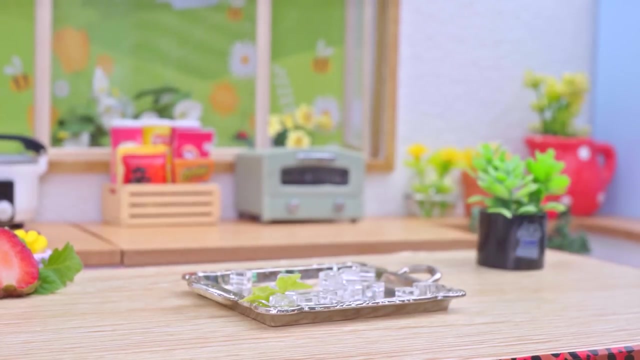 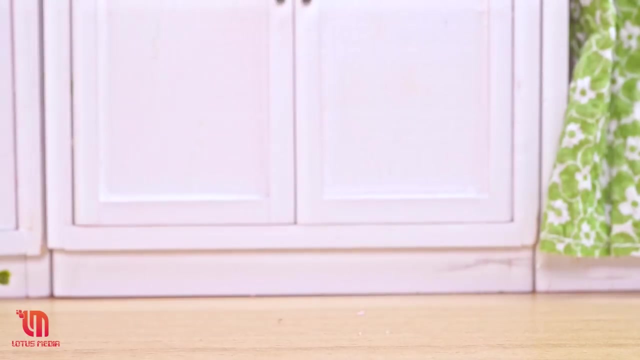 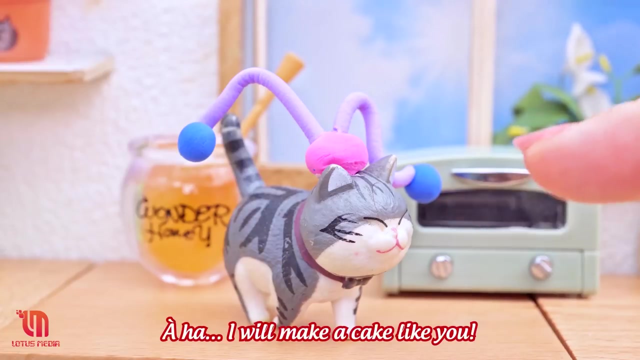 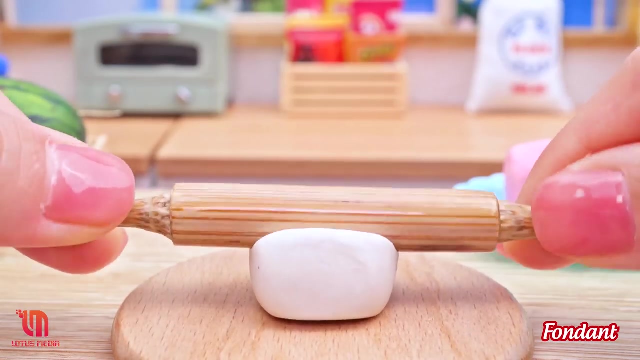 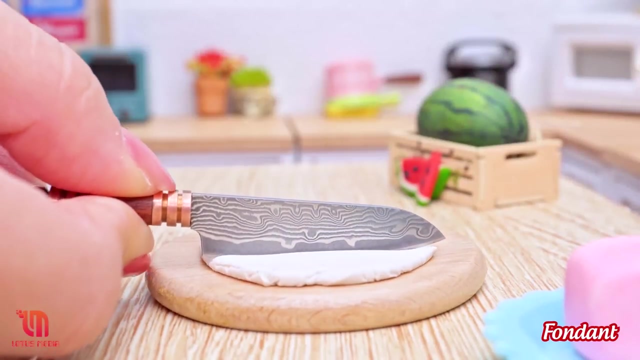 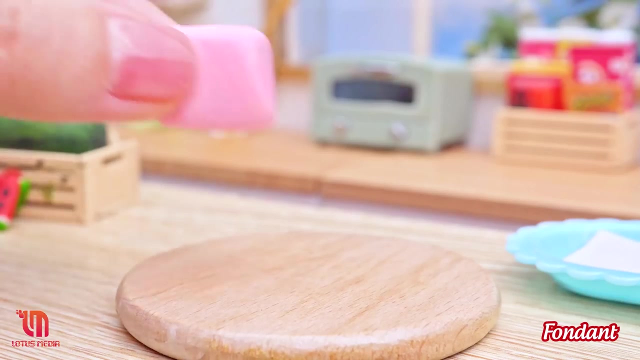 Delicious, Tasty, Wow, Sweet, Yummy. Oh, hello, Here you are. You are so beautiful. Aha, I will make a cake like you. Hi, I'm who you saw on yesterday's video. Same without me. 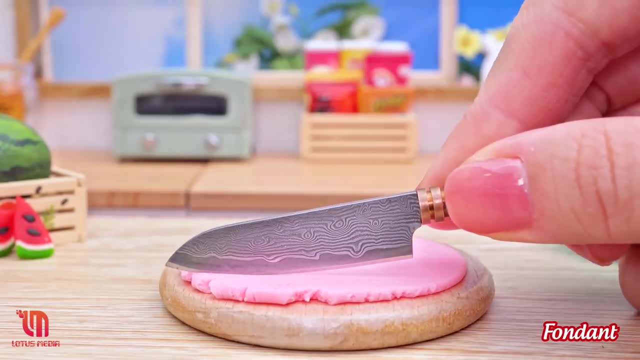 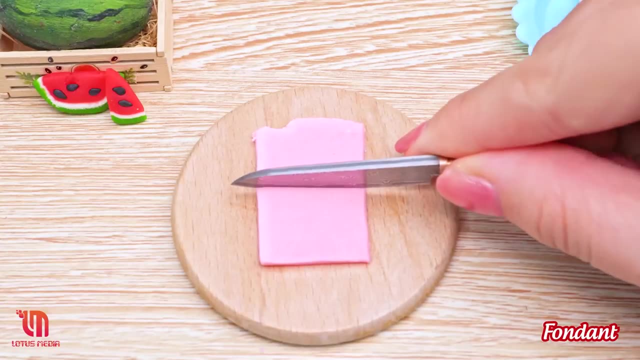 How do you like it So delicious, Wow, Delicious. The recipe is so simple, with a alternative recipe, that the quality of the cake you see today is also amazing, and you will be tastedきた by us. Thanks a lot, And now I'd like to see. 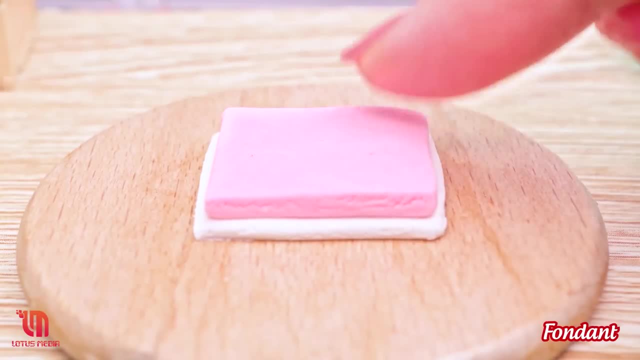 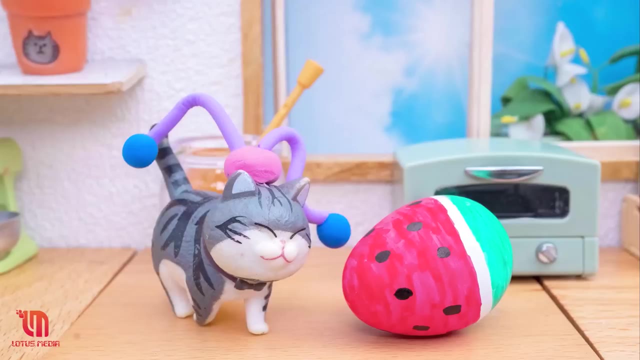 your questions. OK, Let's start. Huh, Ah, the kicker helps me surviving. And am I right? Is this okay? Pastries, Hm, Right, What? No, thank you. Yes, Oh, thank you. 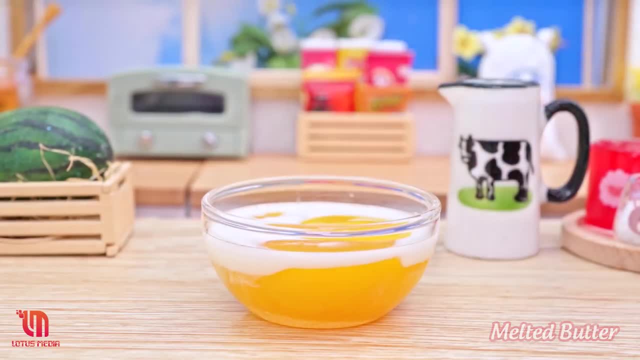 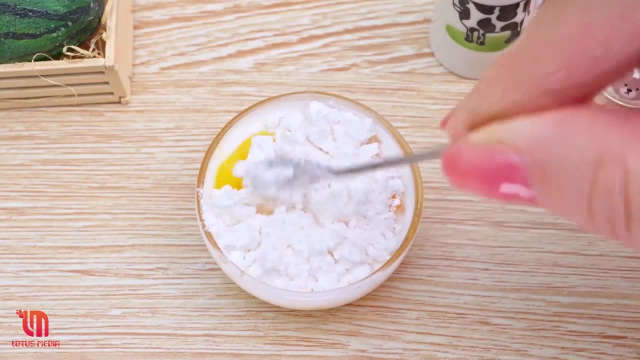 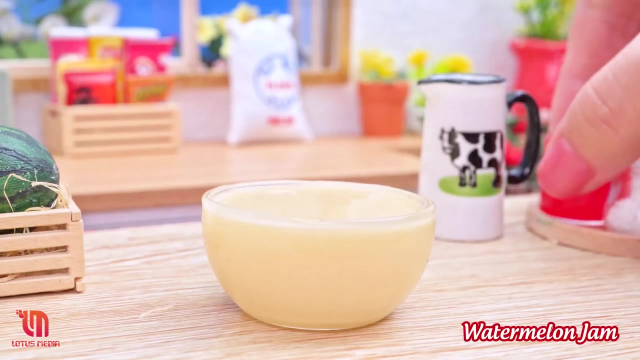 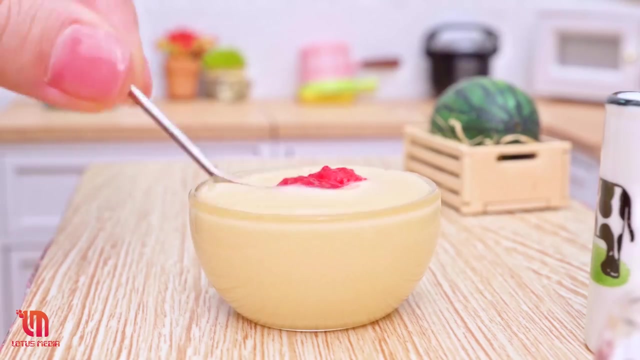 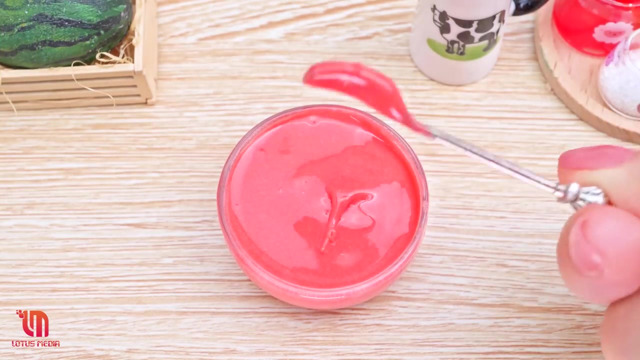 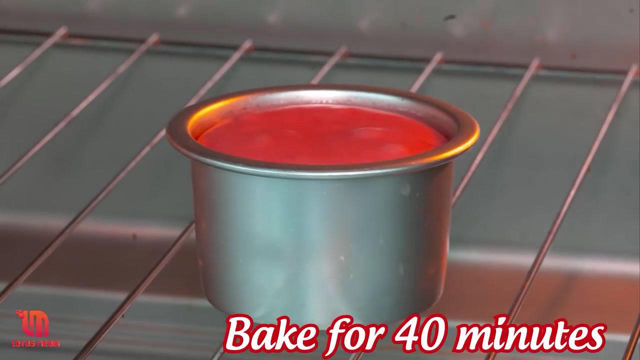 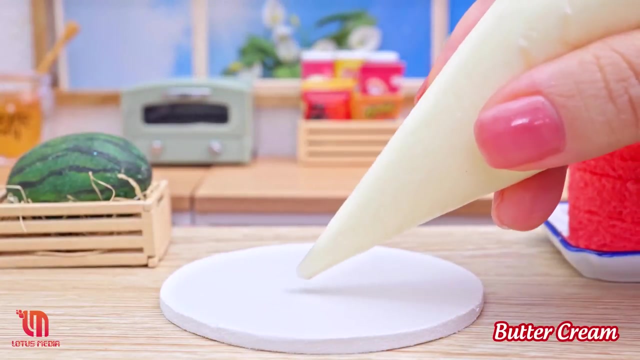 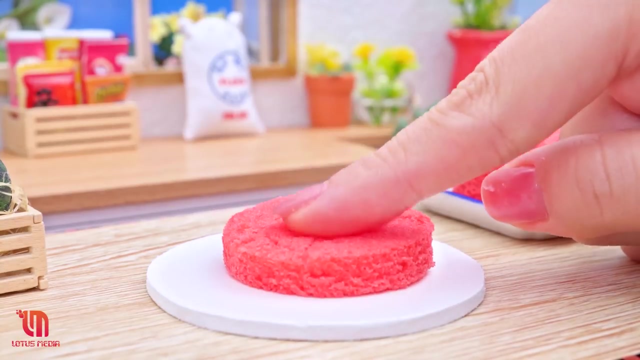 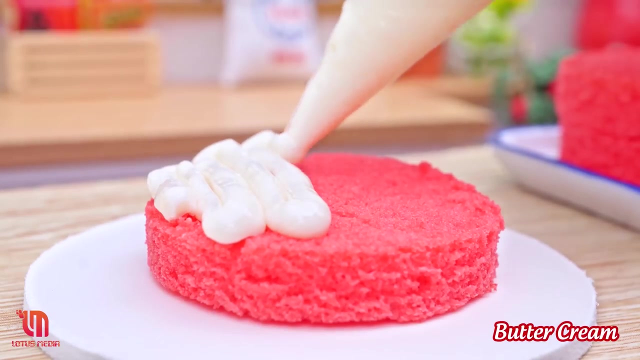 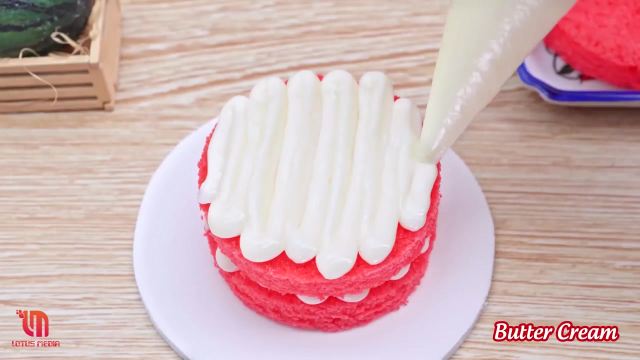 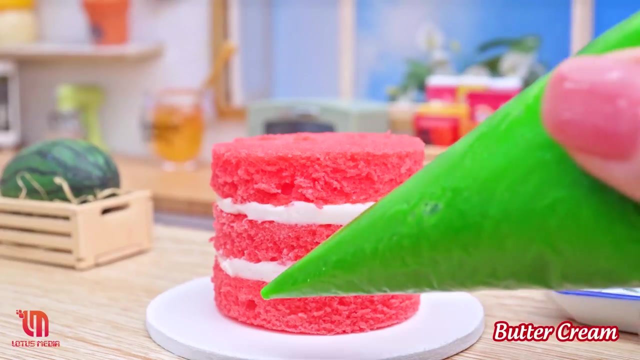 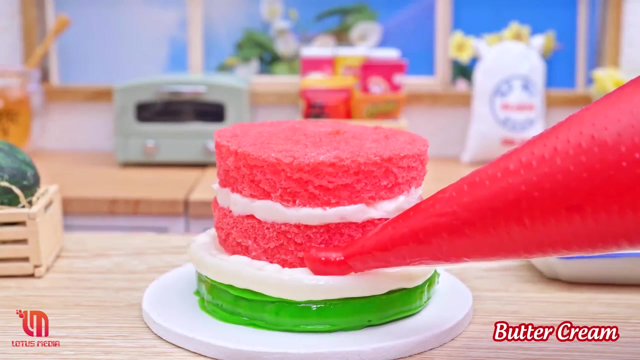 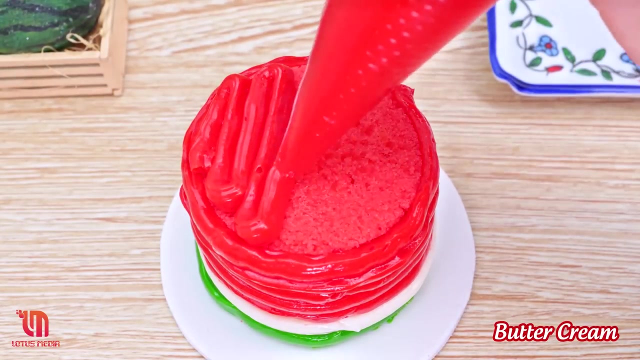 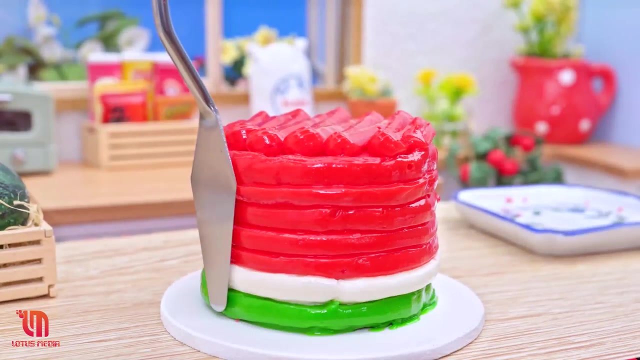 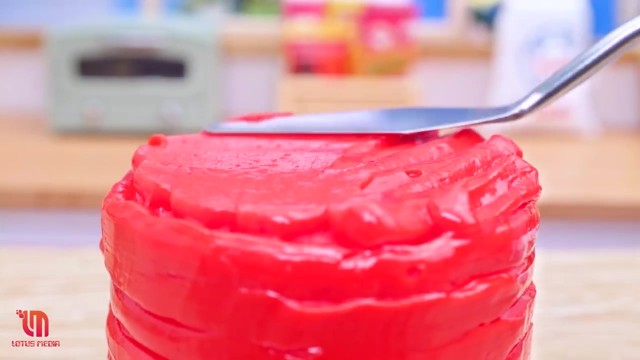 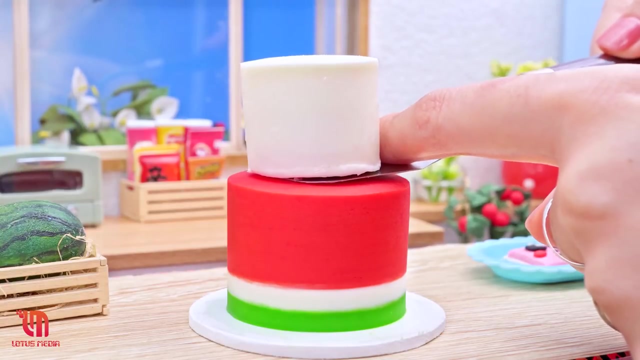 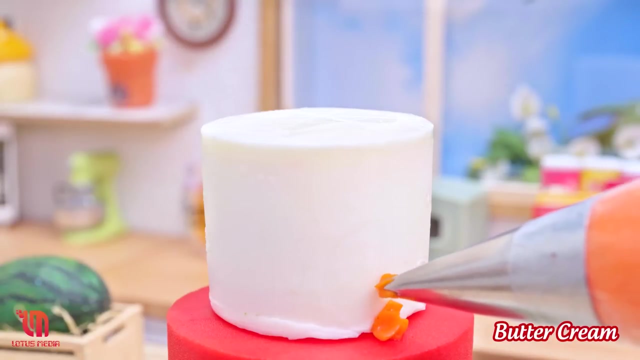 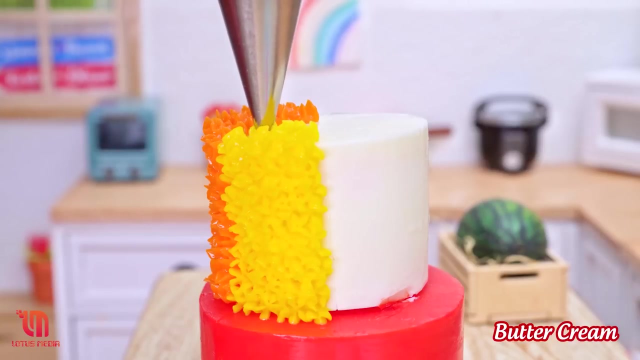 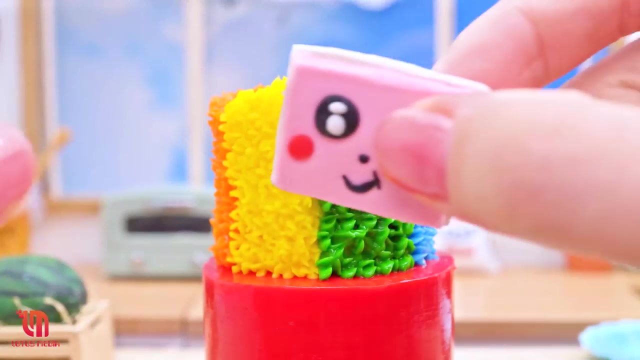 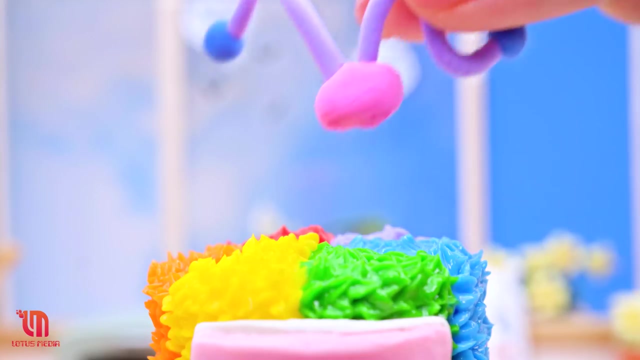 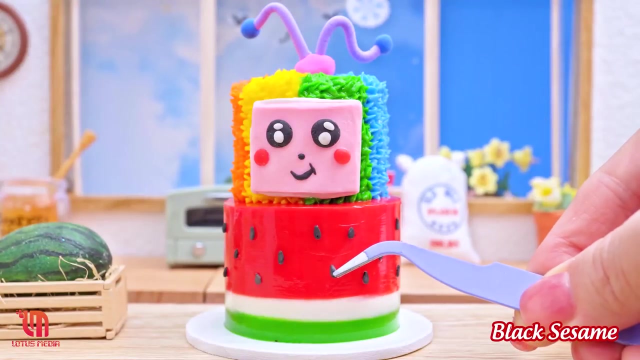 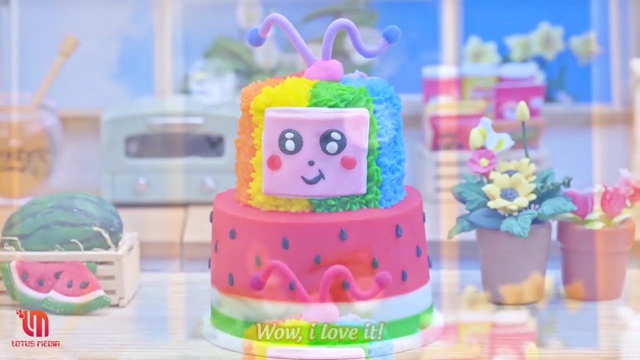 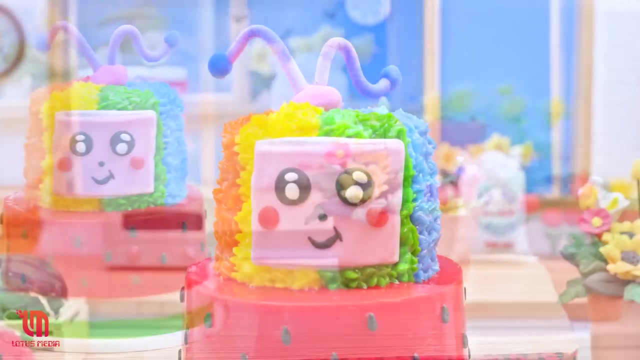 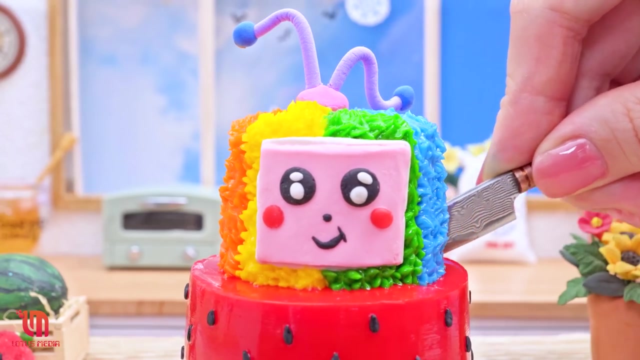 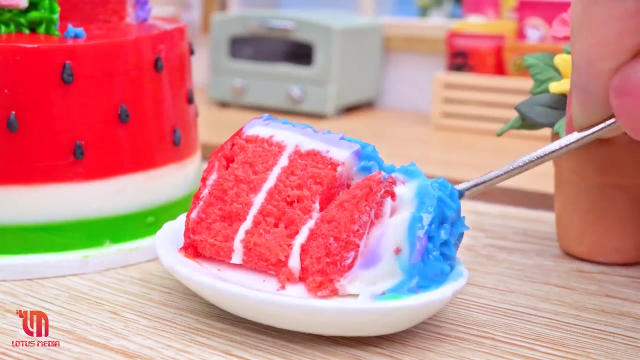 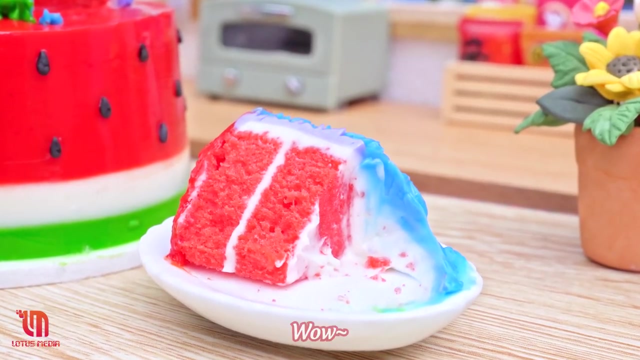 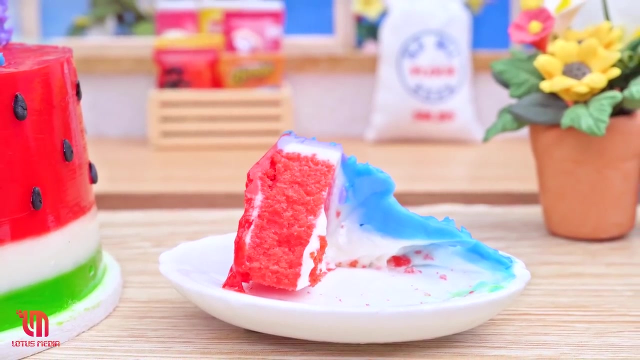 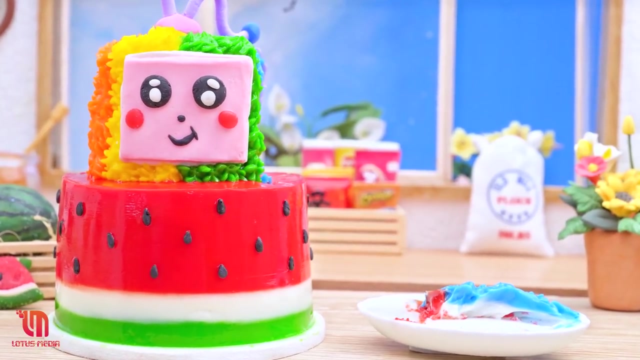 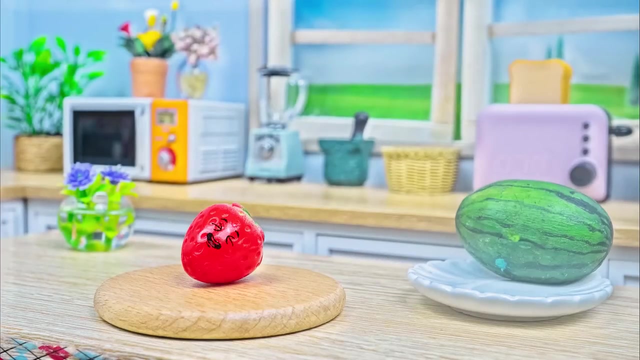 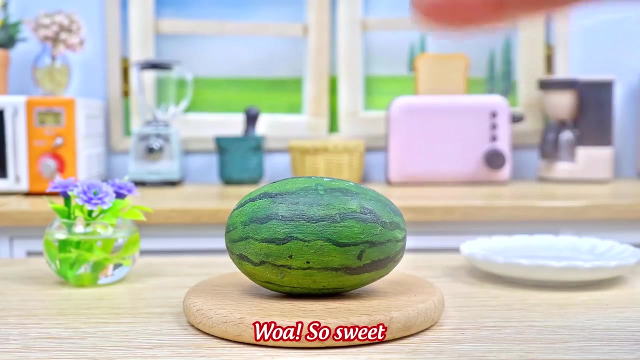 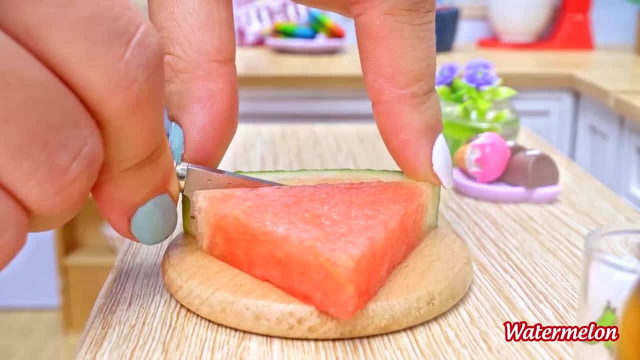 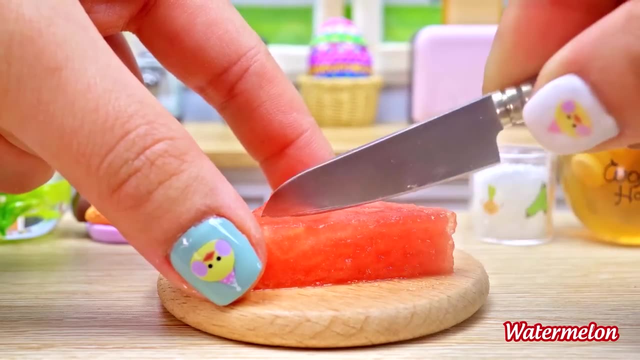 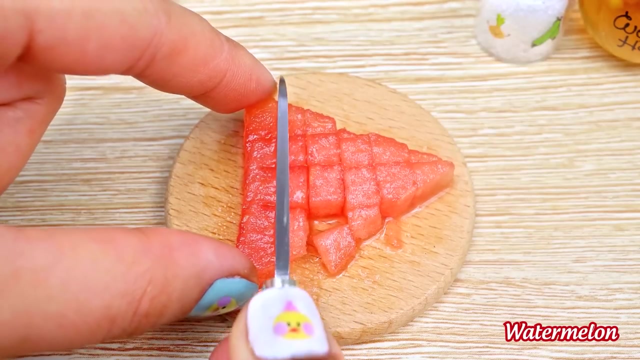 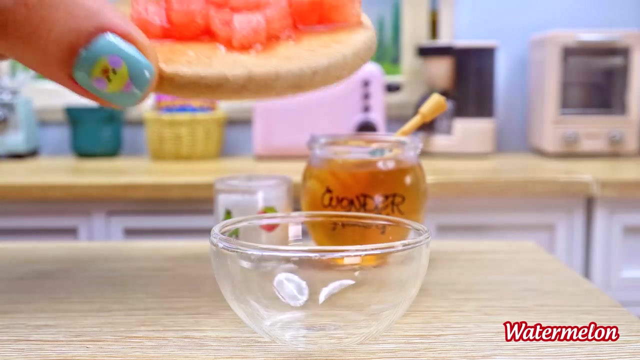 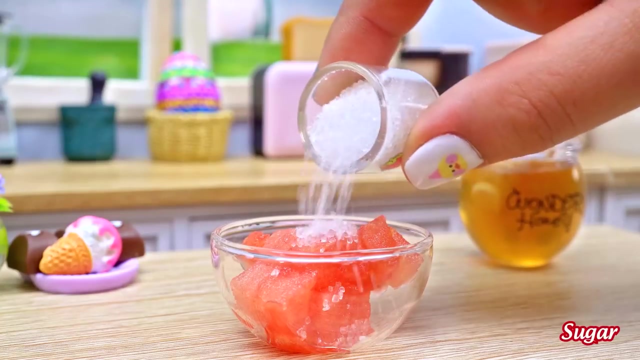 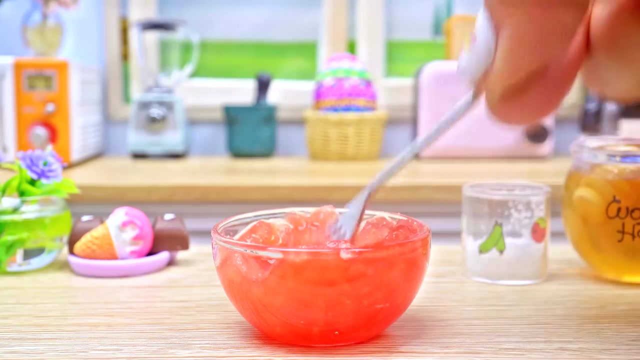 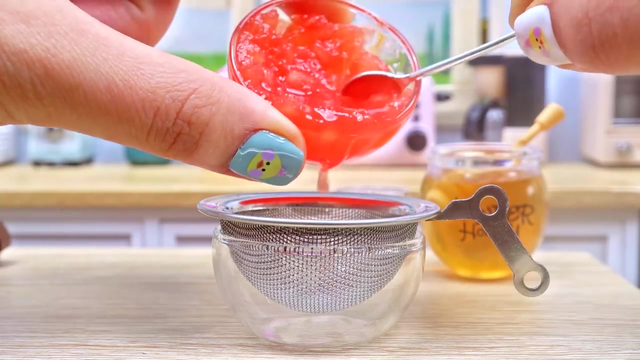 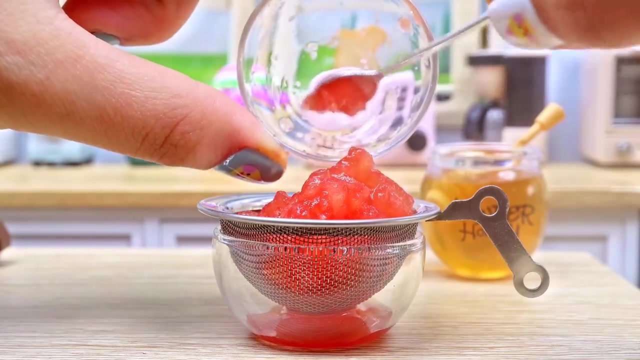 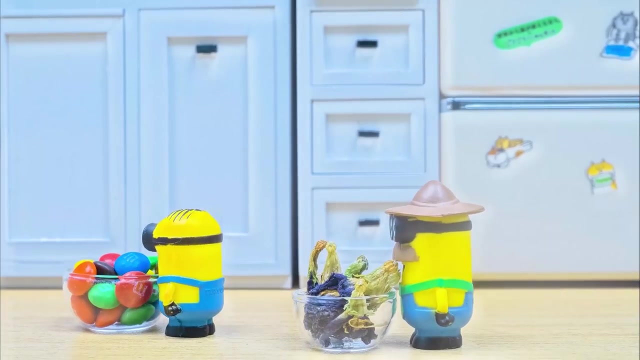 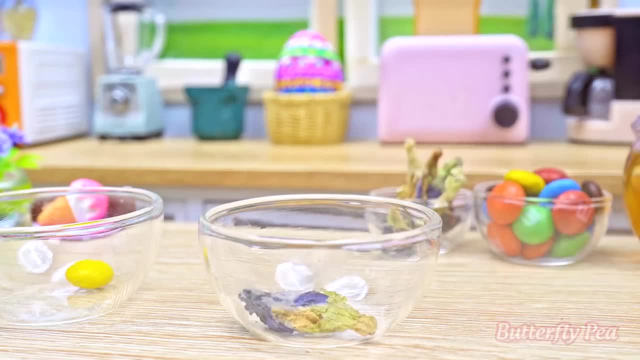 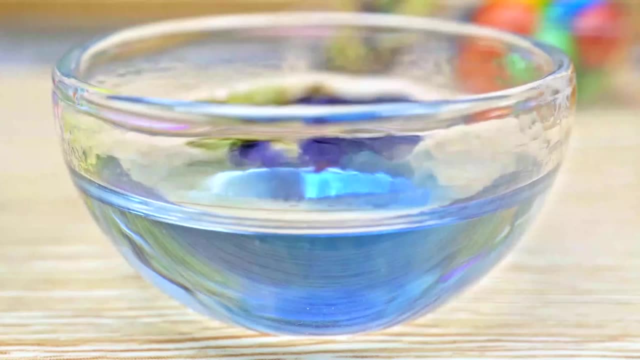 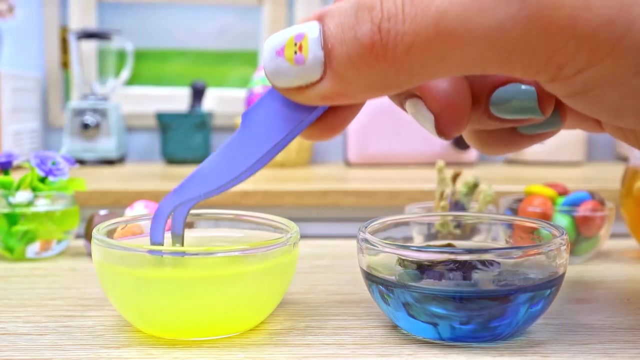 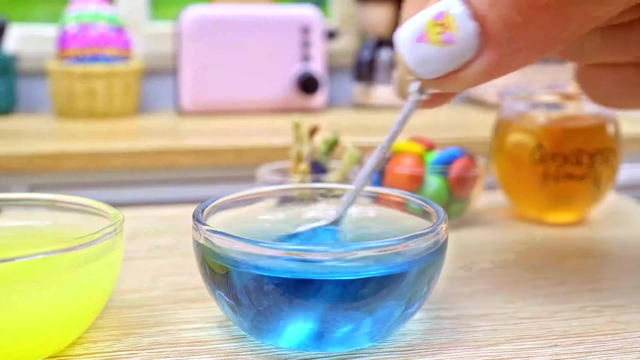 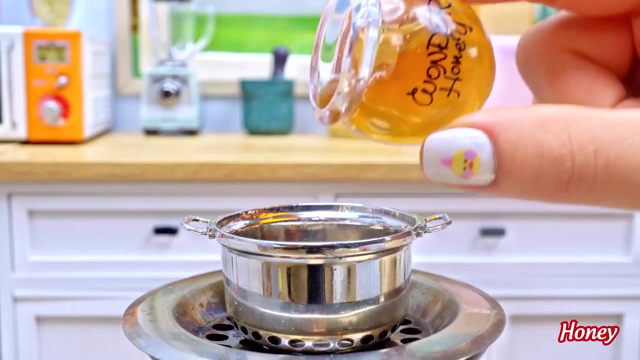 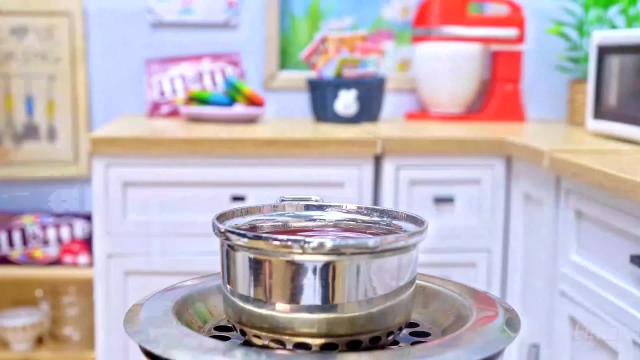 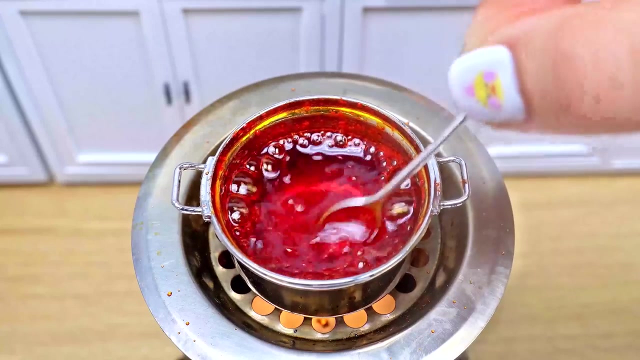 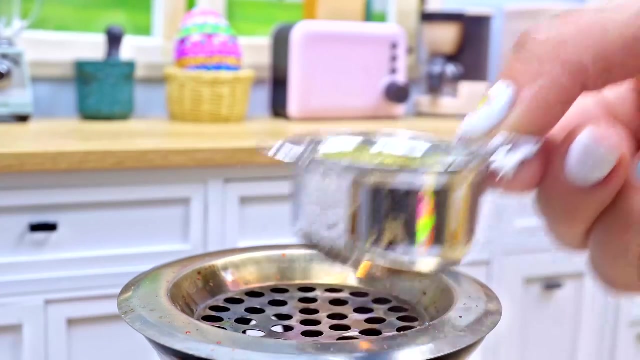 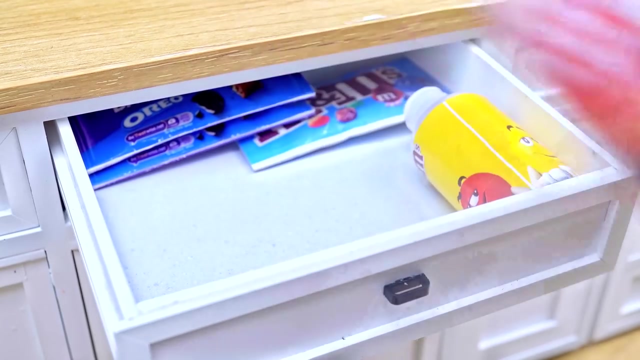 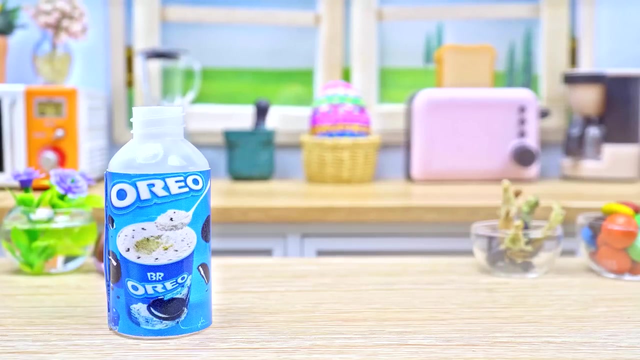 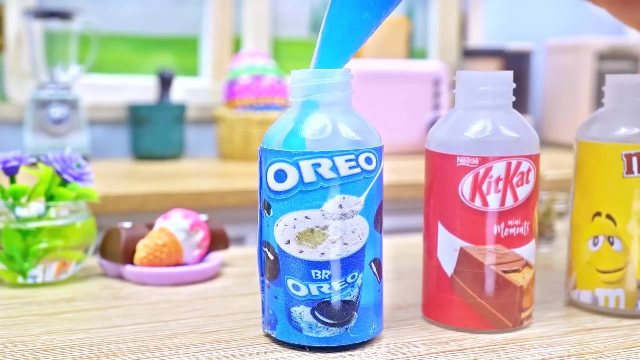 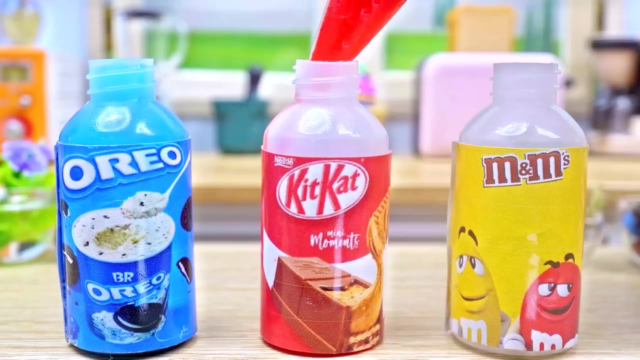 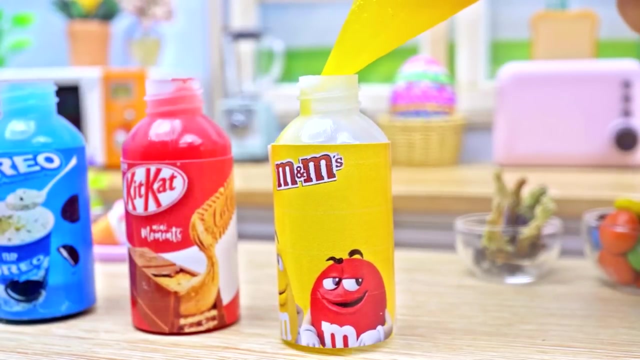 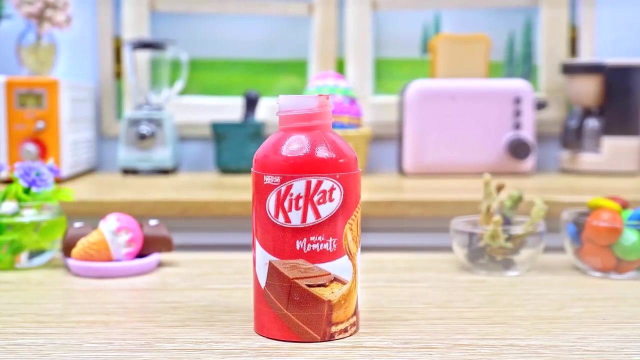 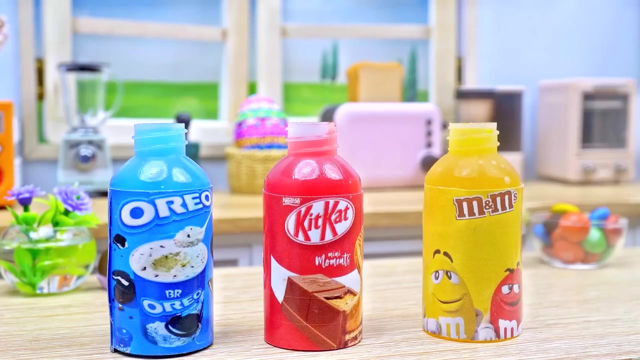 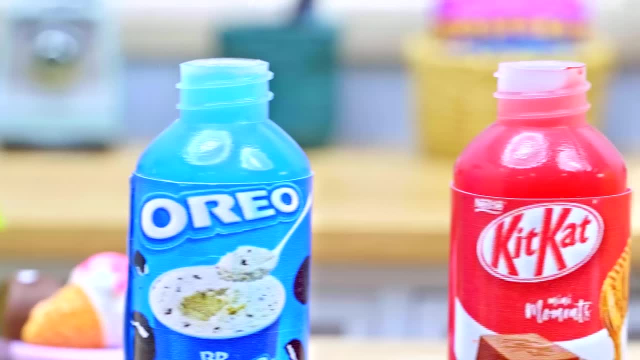 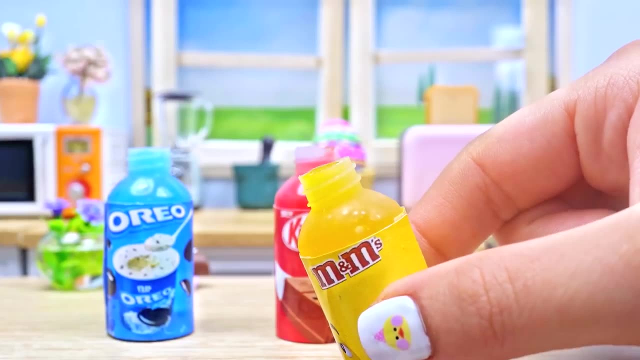 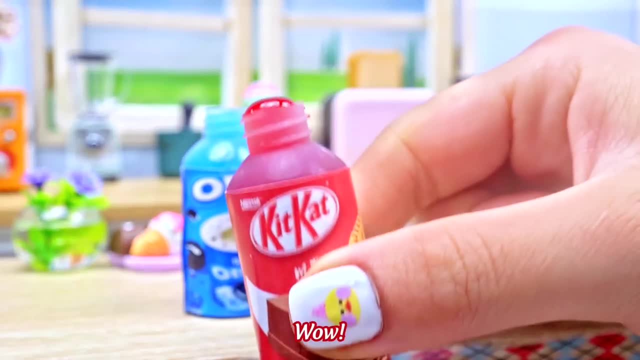 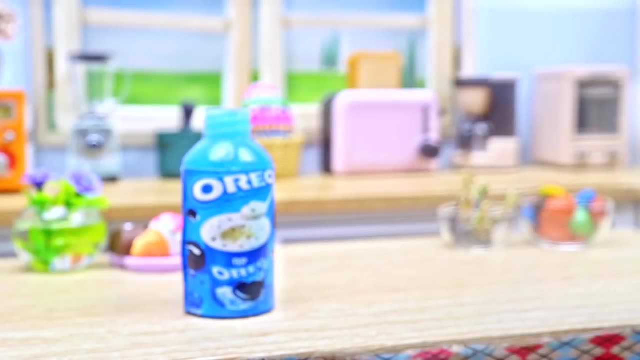 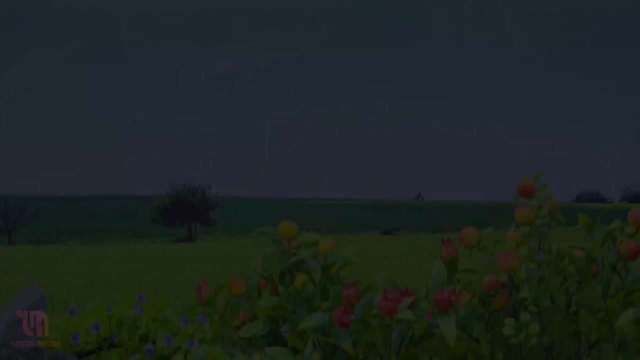 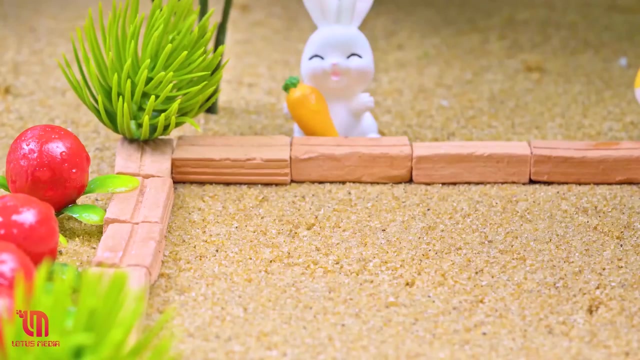 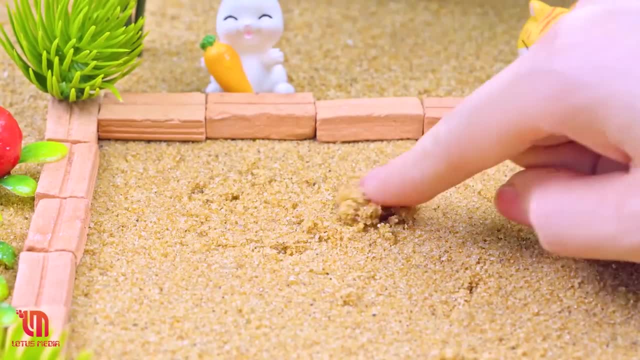 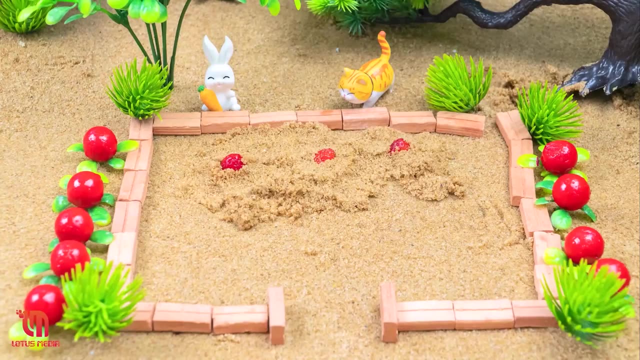 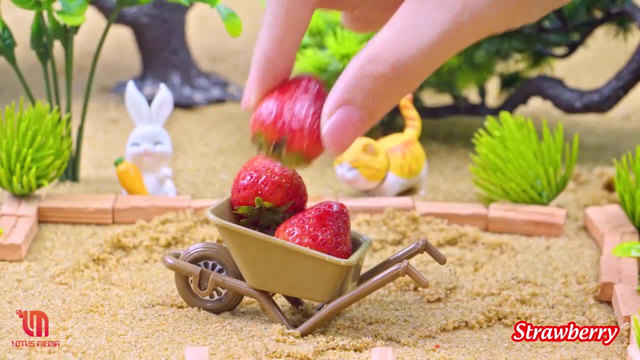 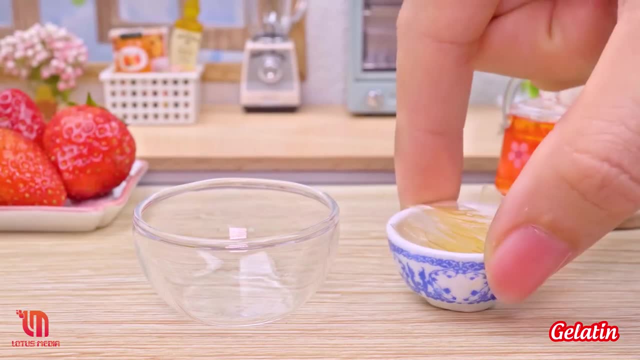 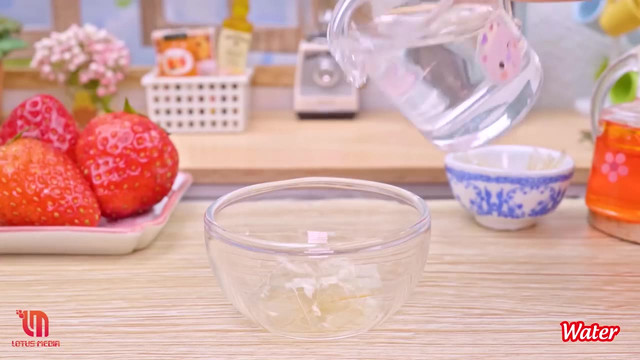 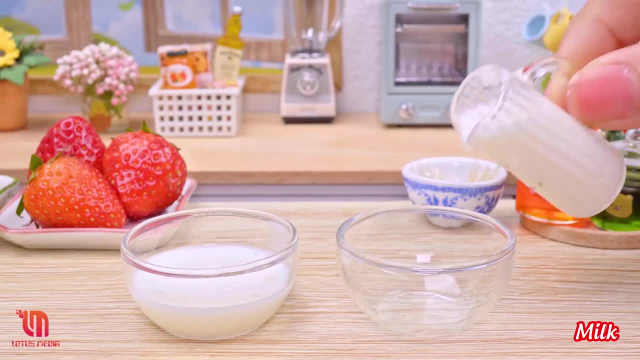 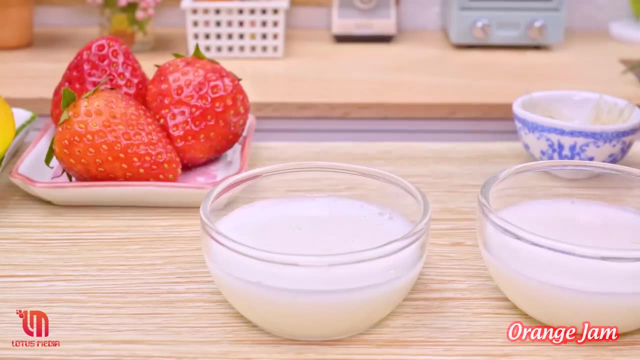 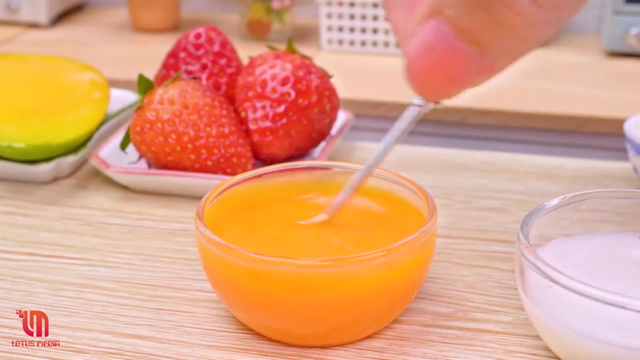 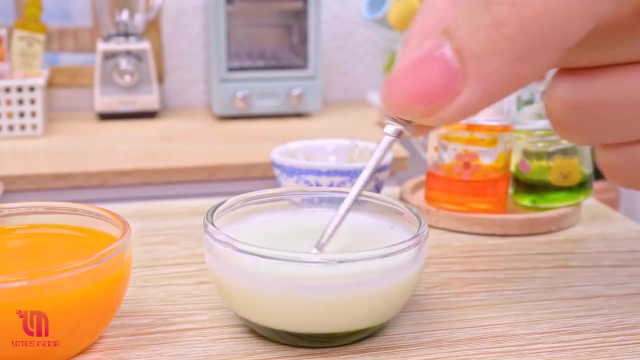 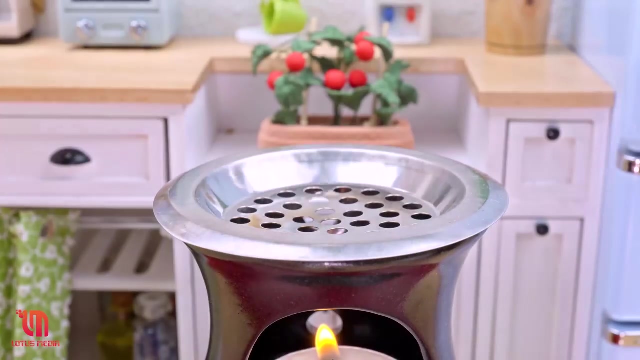 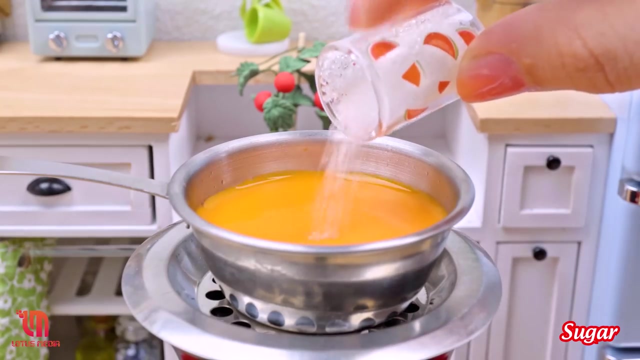 Add 1 tablespoon of salt, pepper and water to the pot and bring to a boil. then turn off the heat and let it simmer for about 10 minutes. Sift all the flour into a realize and add all the eggs. Toss over softened butter at low speed. 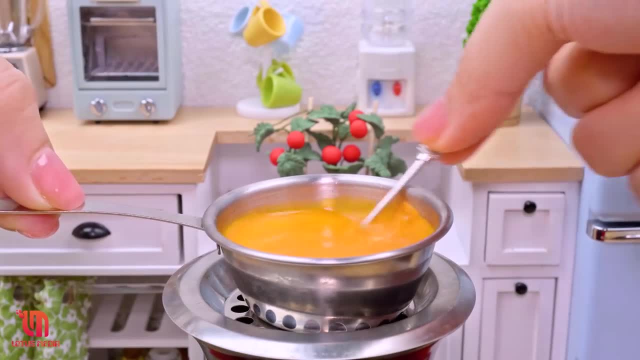 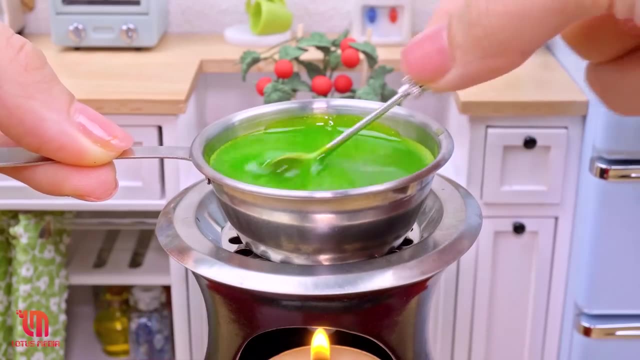 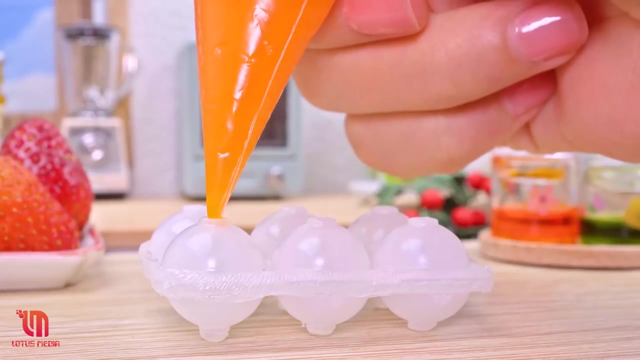 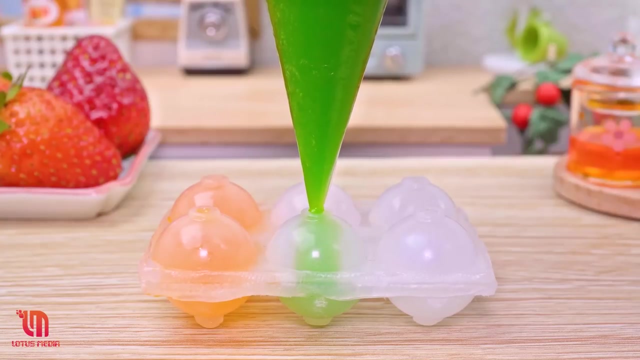 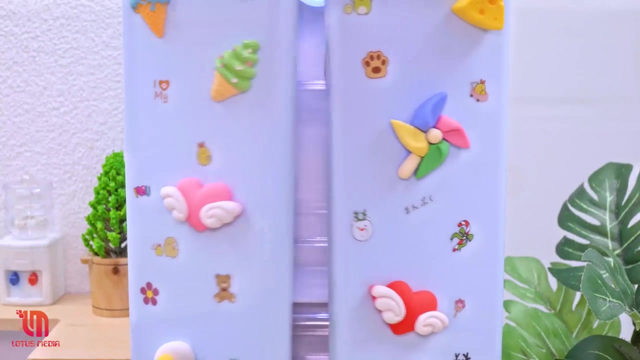 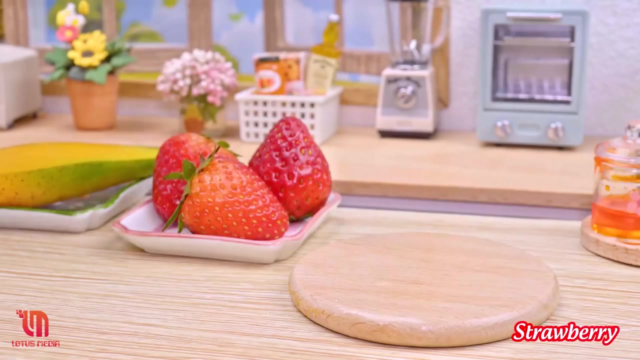 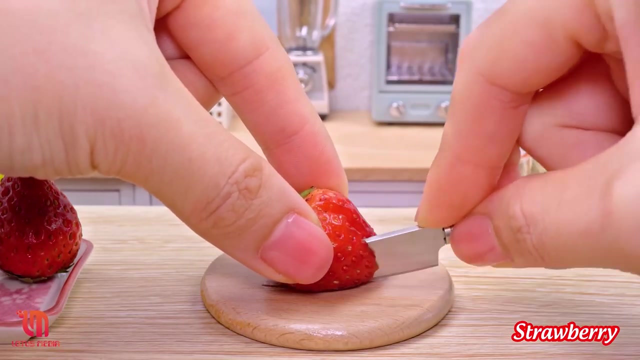 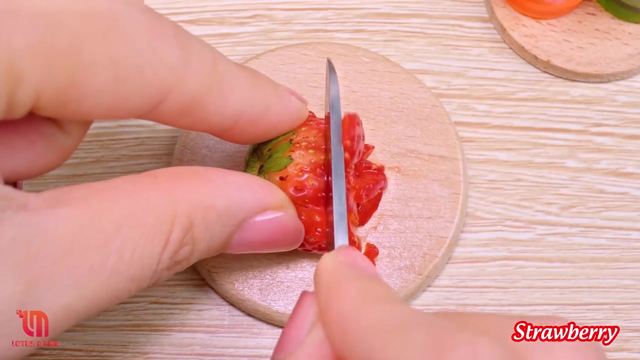 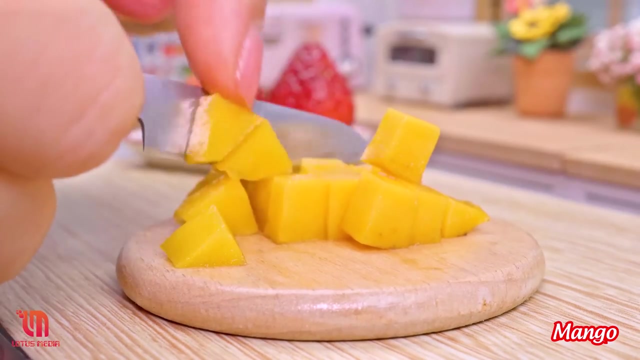 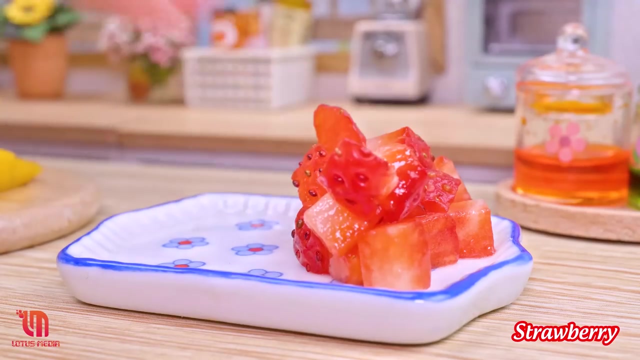 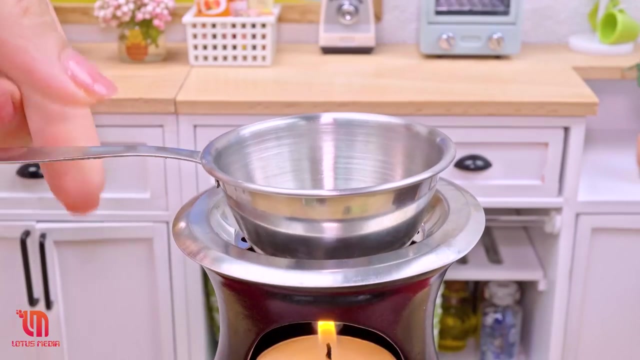 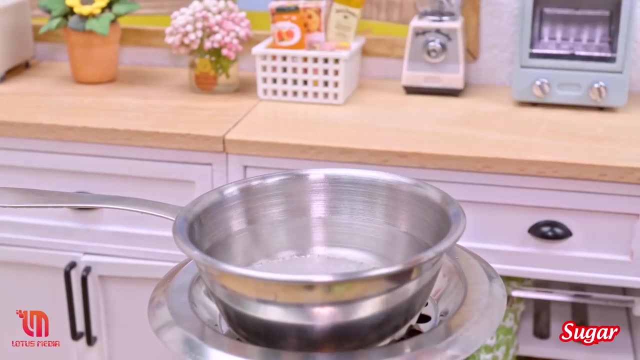 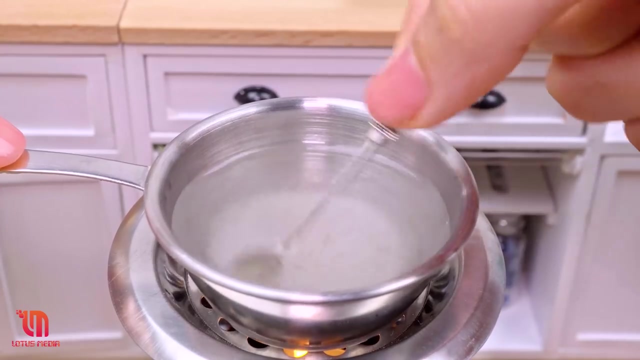 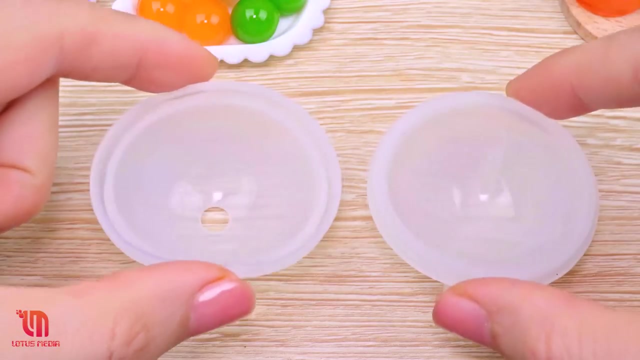 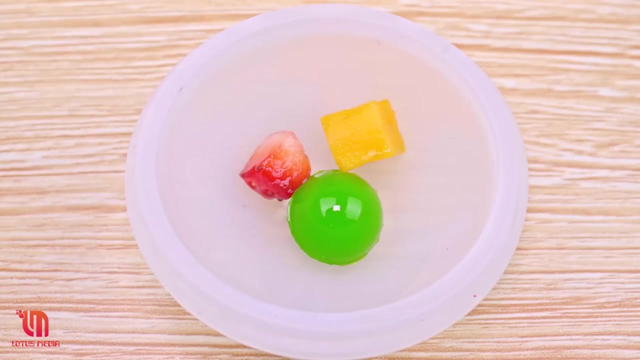 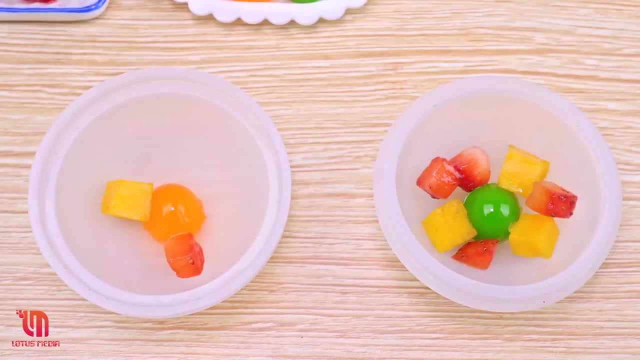 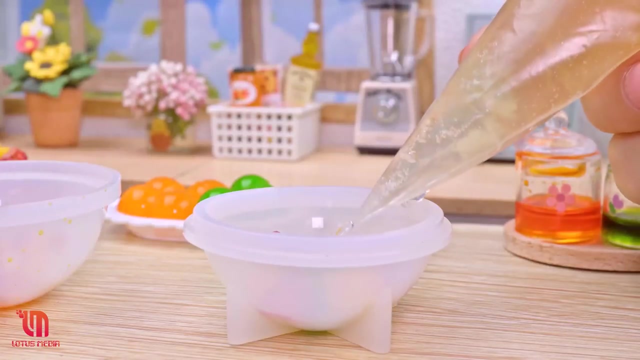 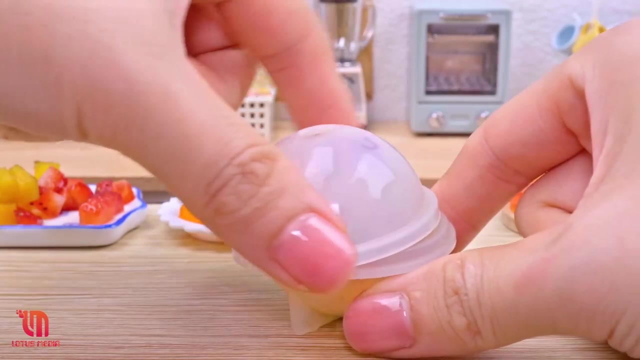 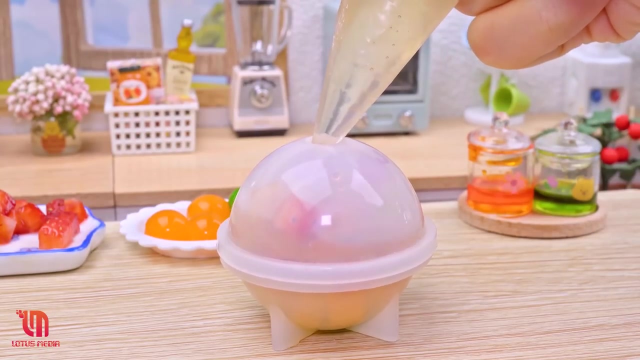 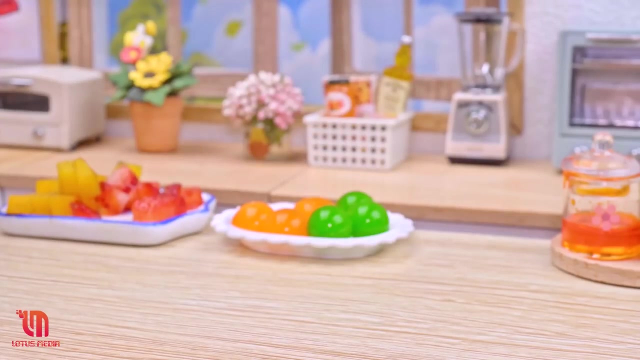 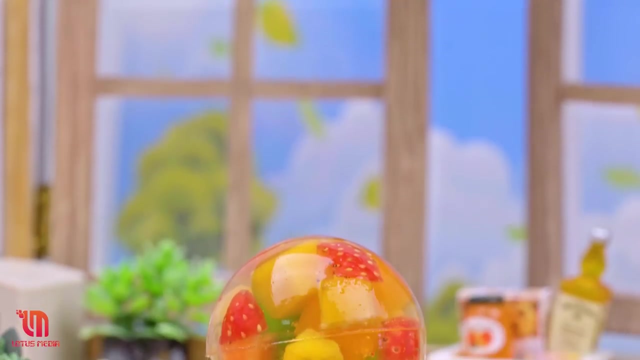 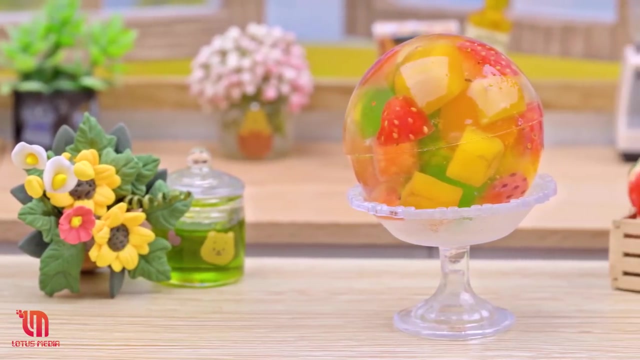 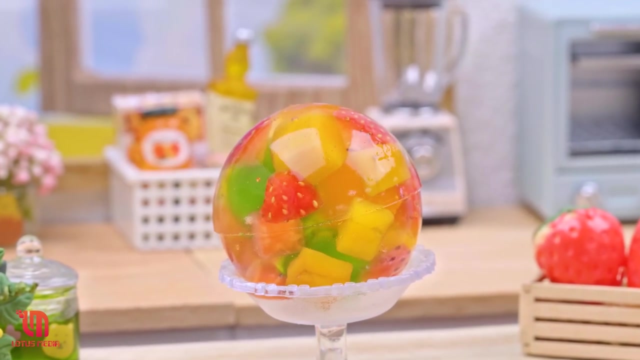 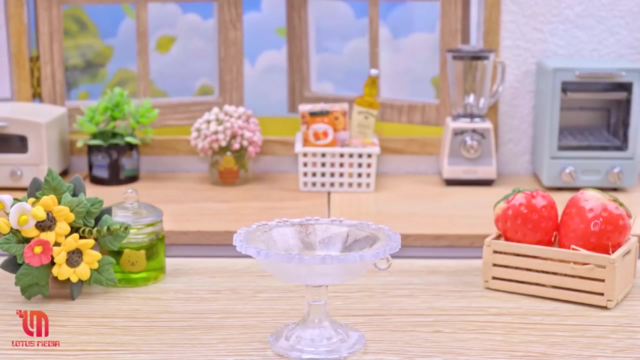 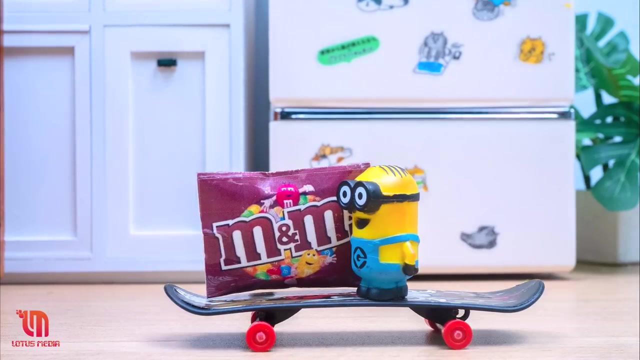 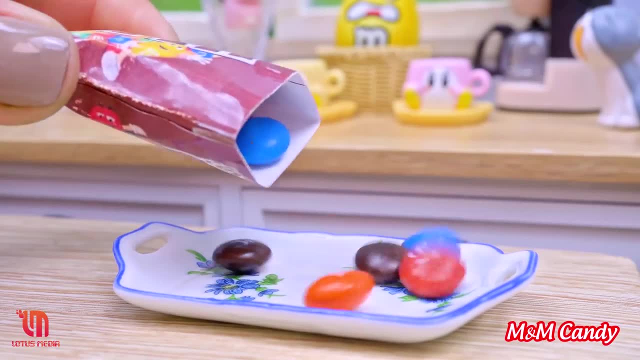 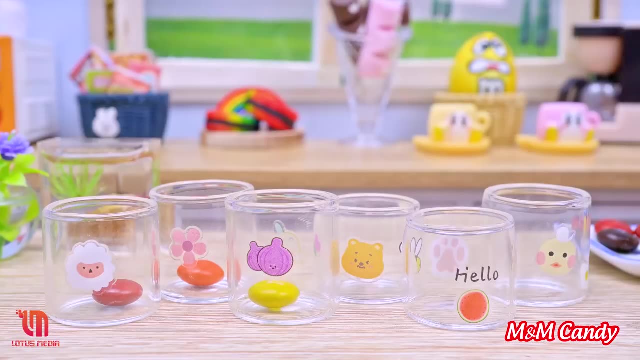 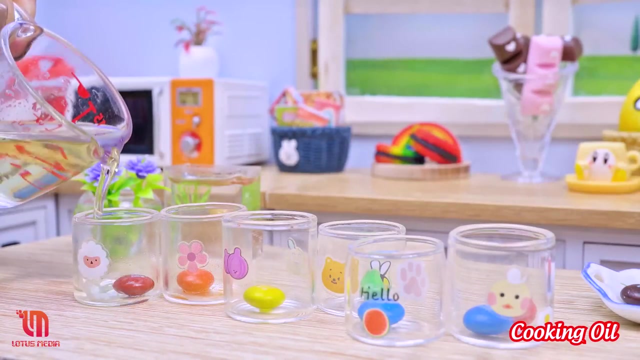 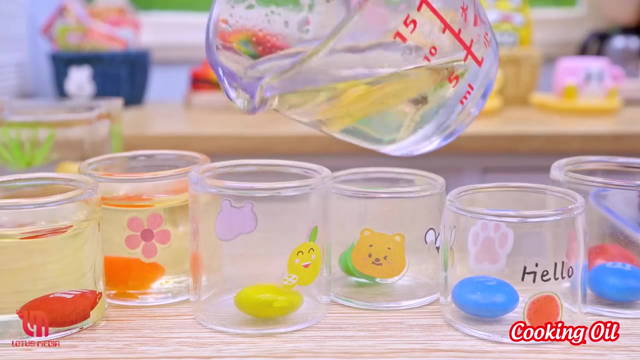 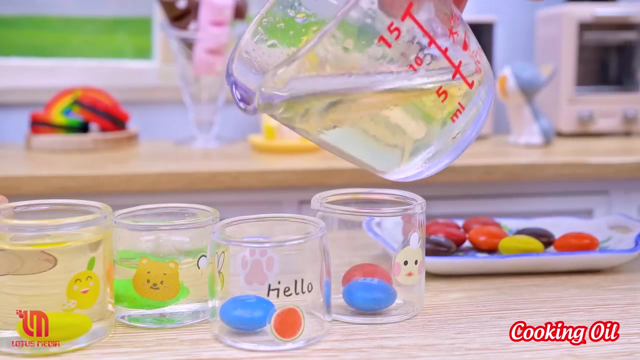 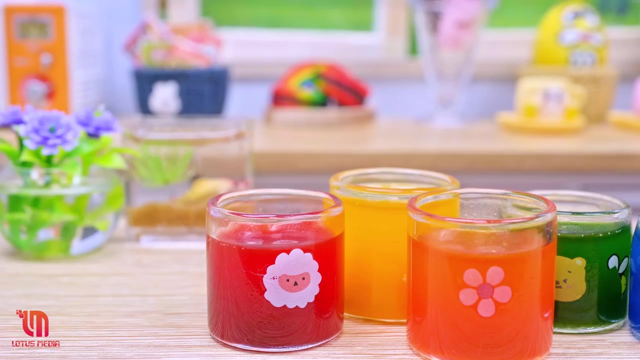 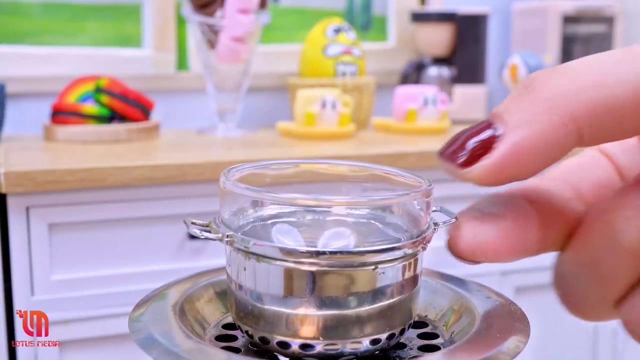 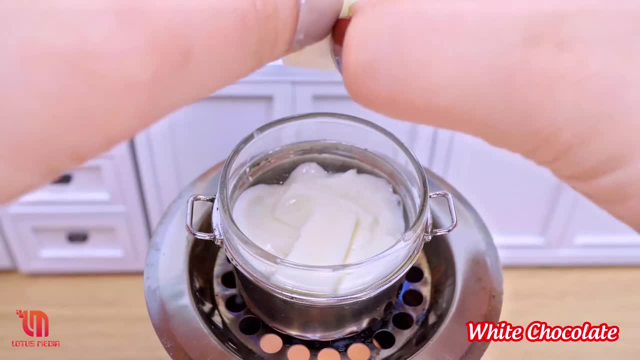 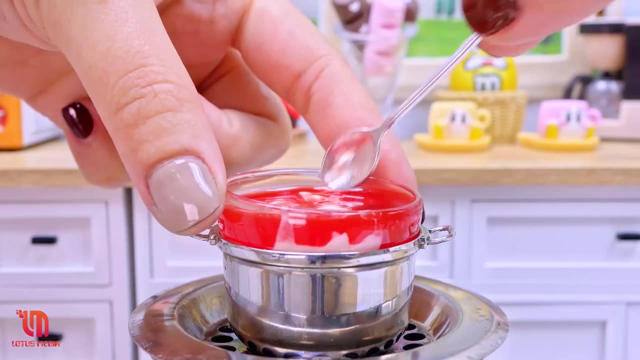 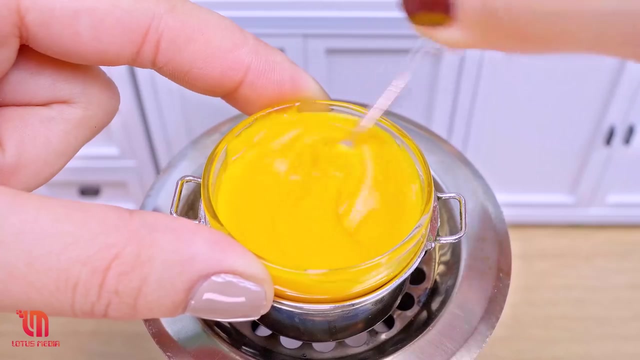 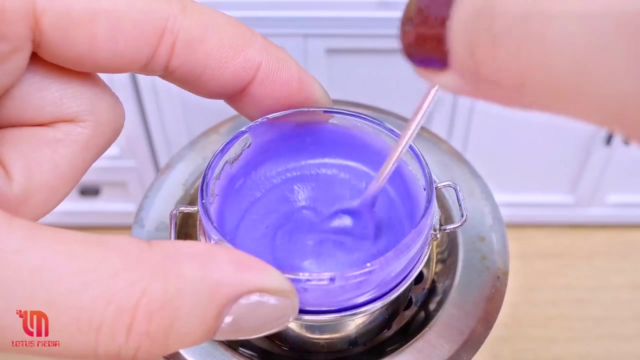 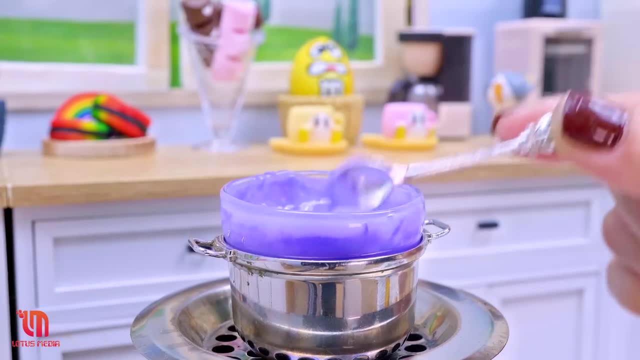 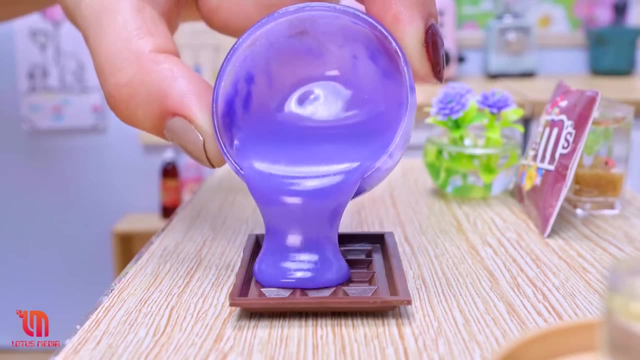 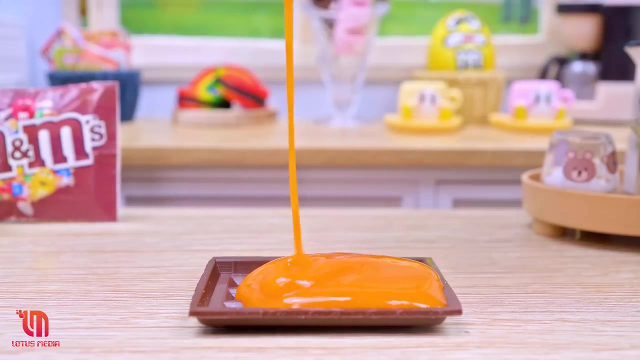 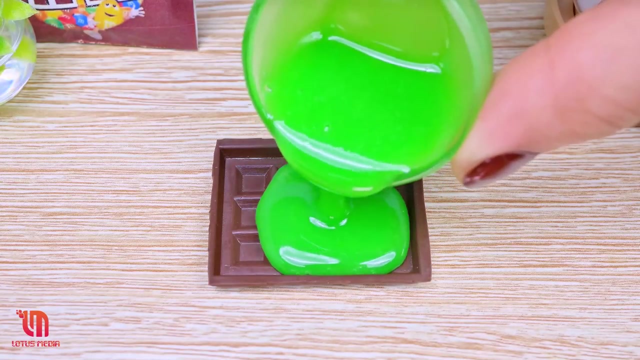 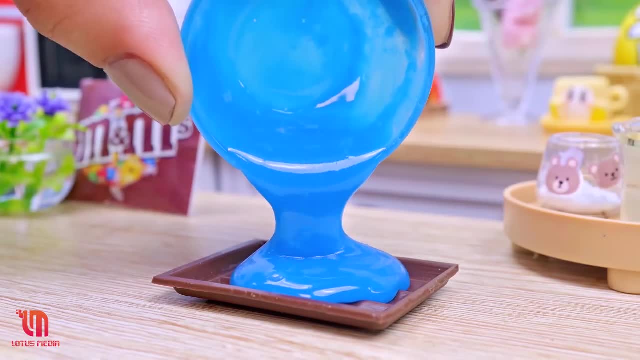 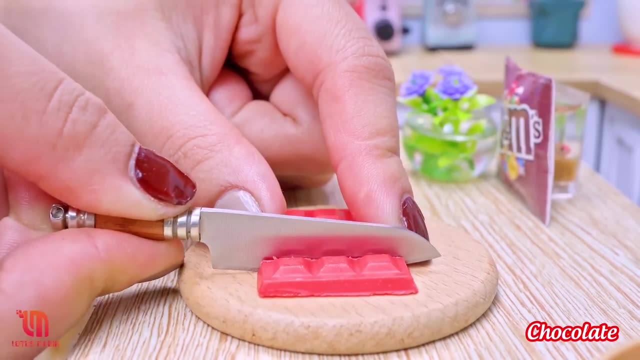 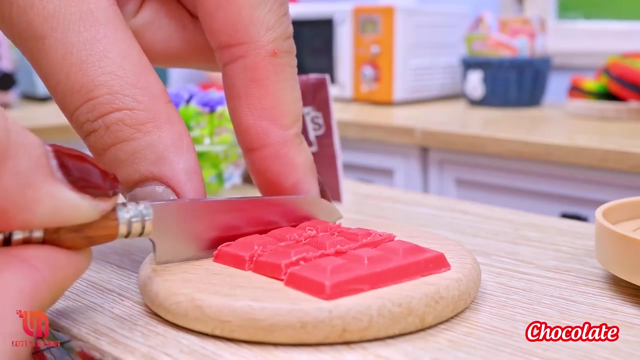 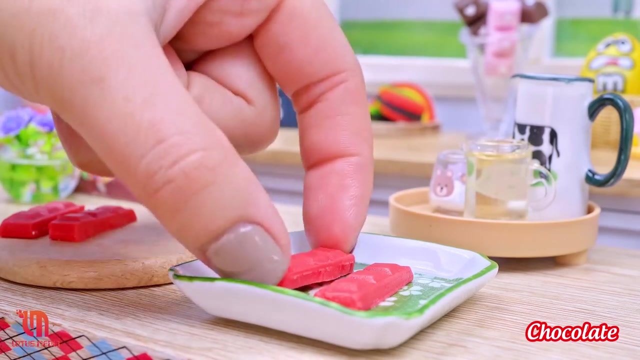 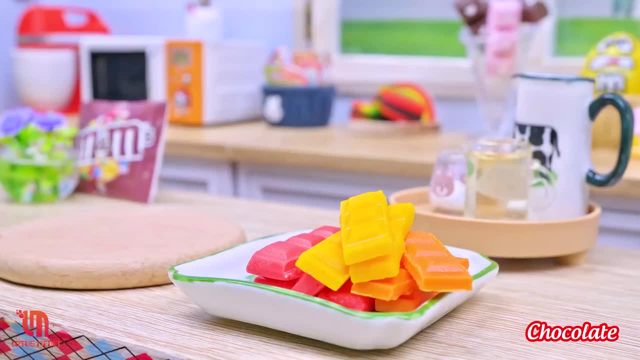 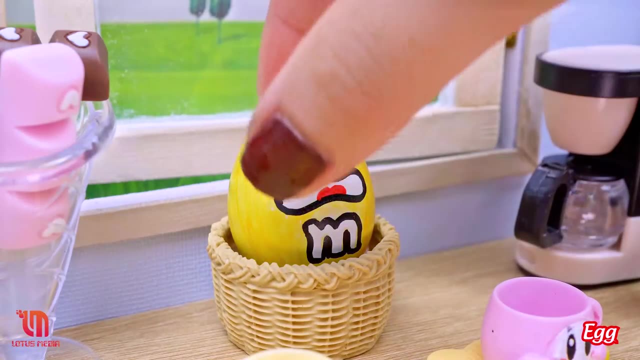 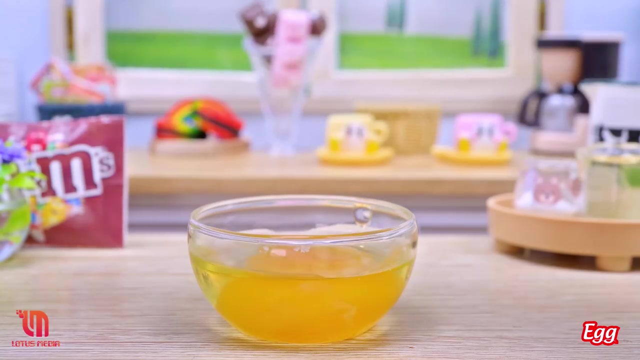 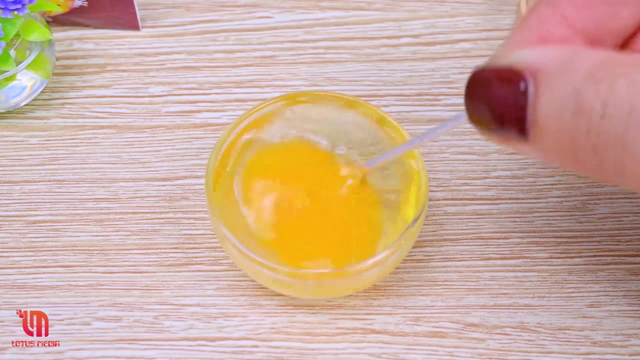 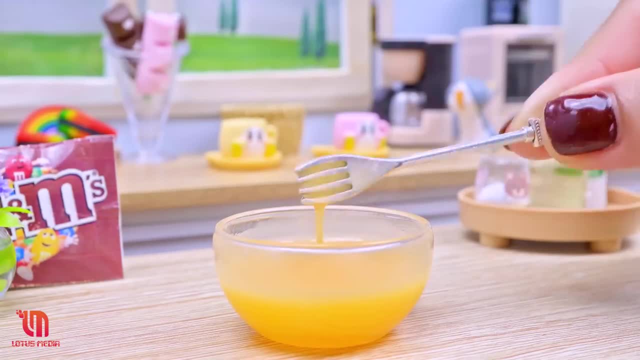 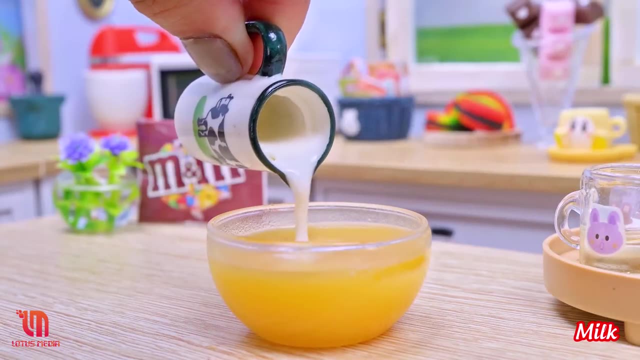 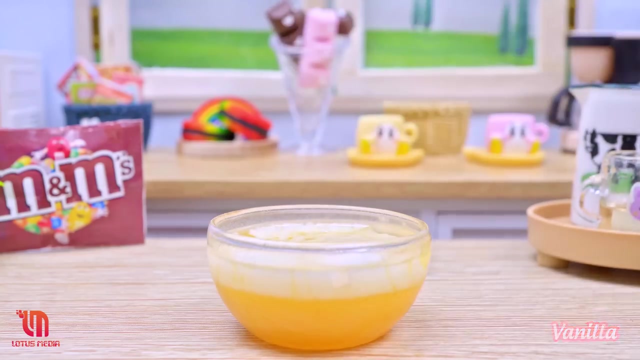 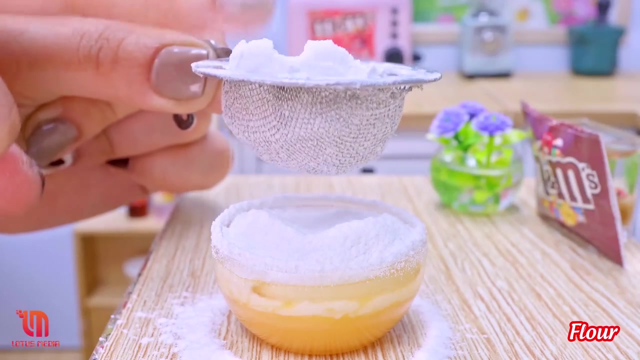 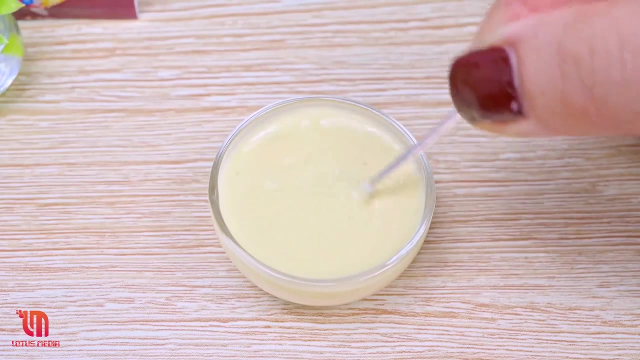 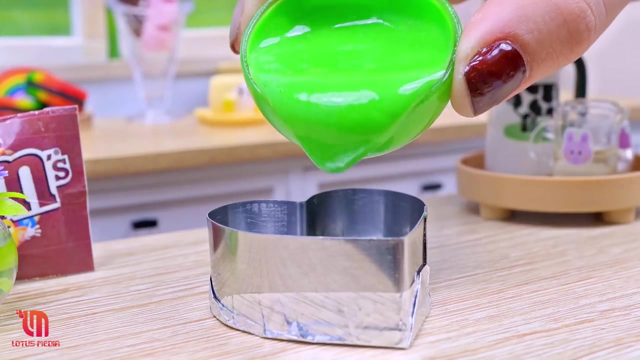 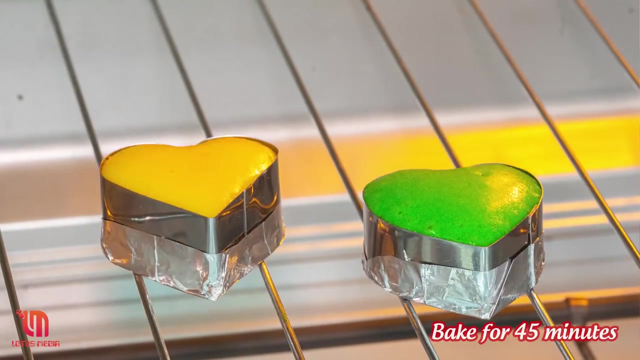 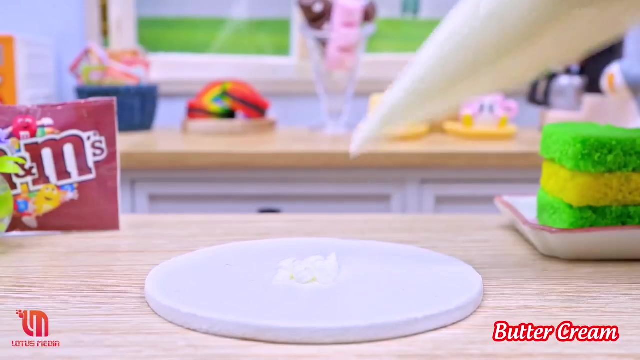 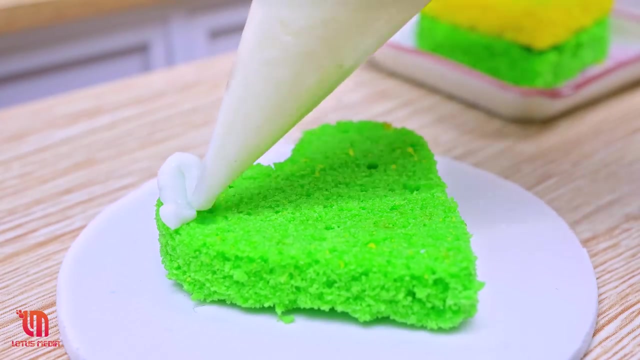 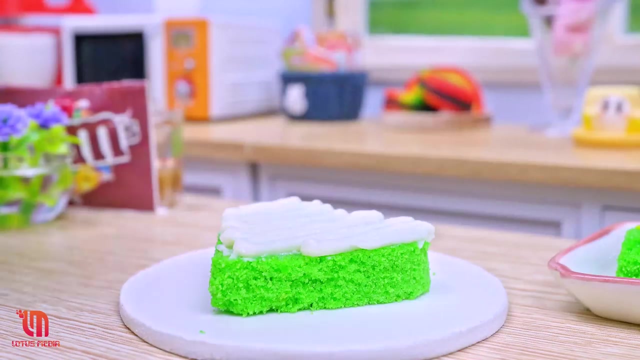 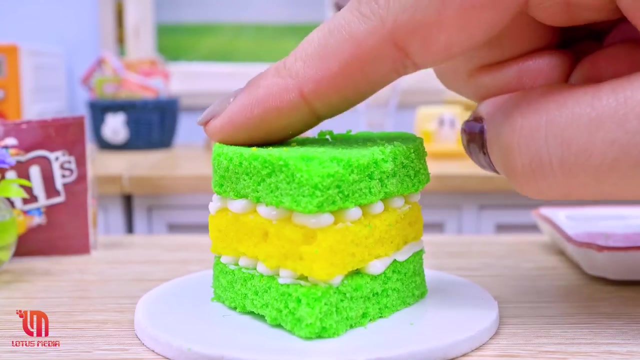 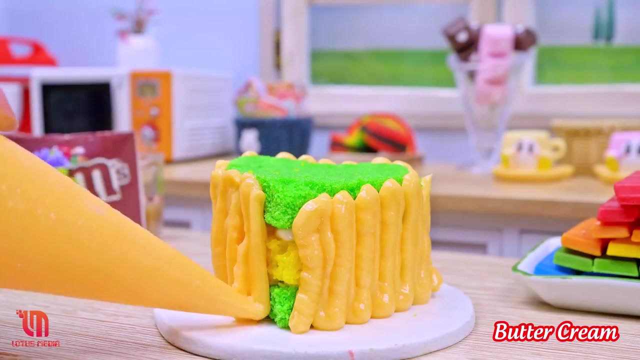 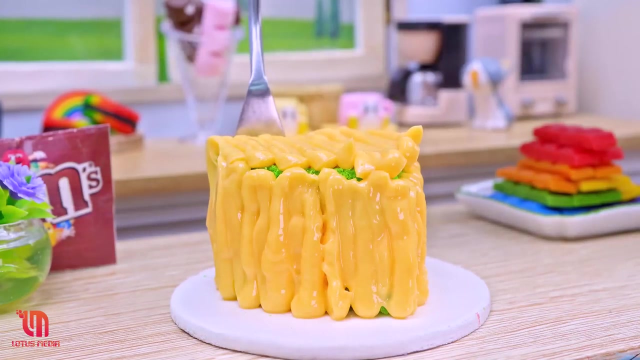 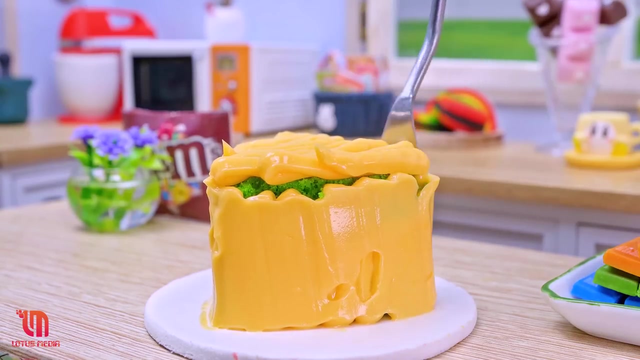 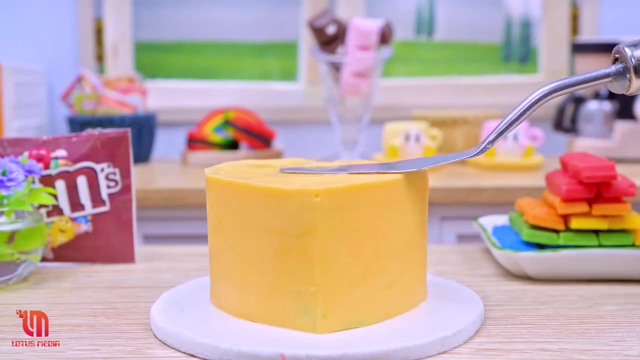 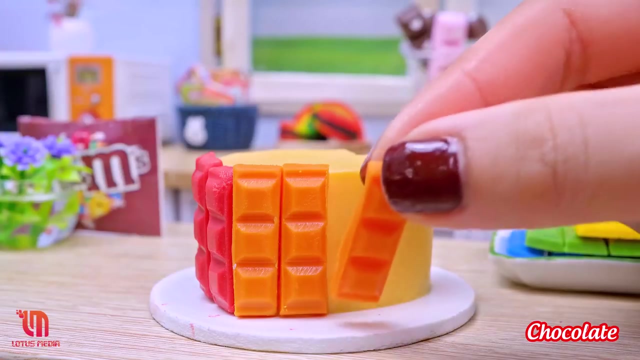 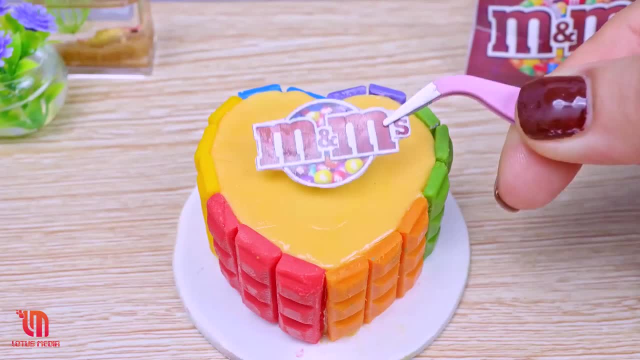 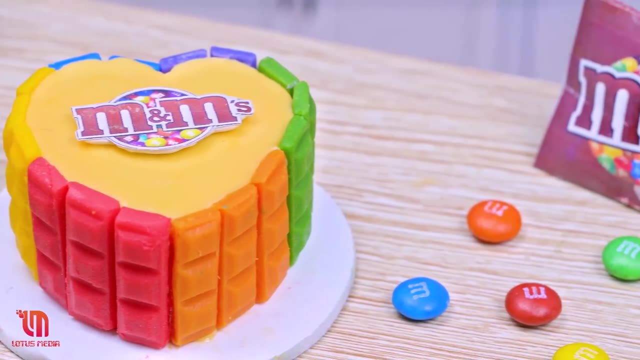 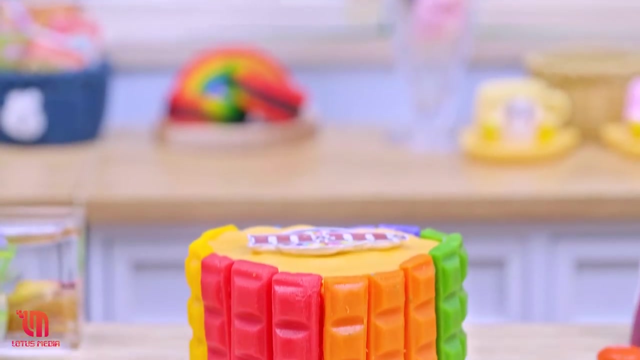 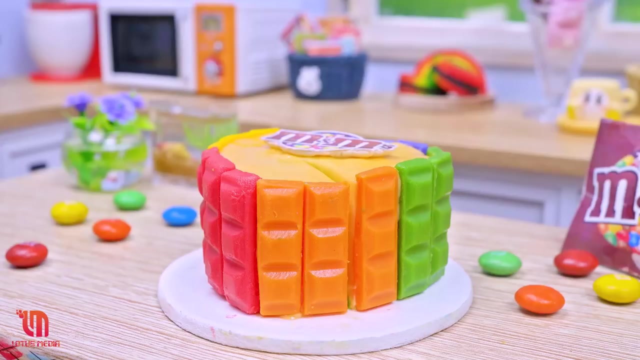 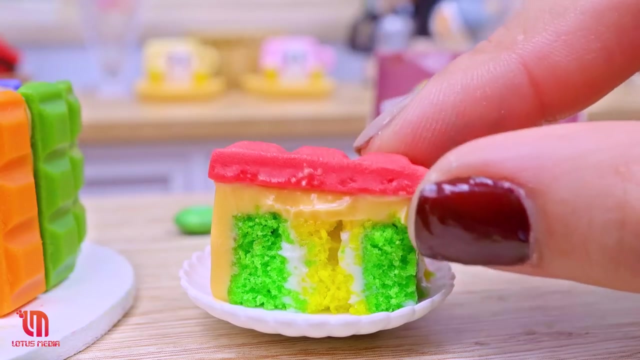 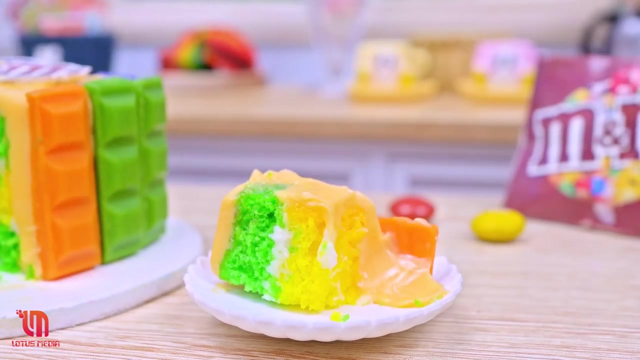 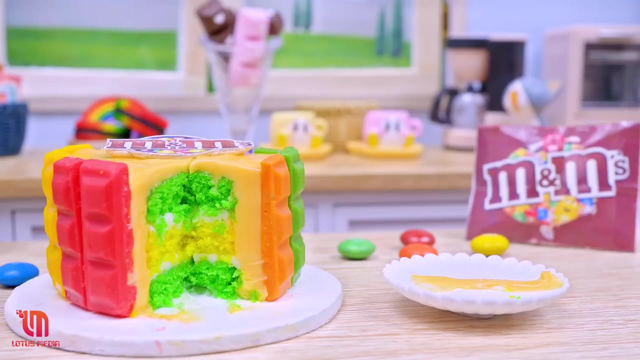 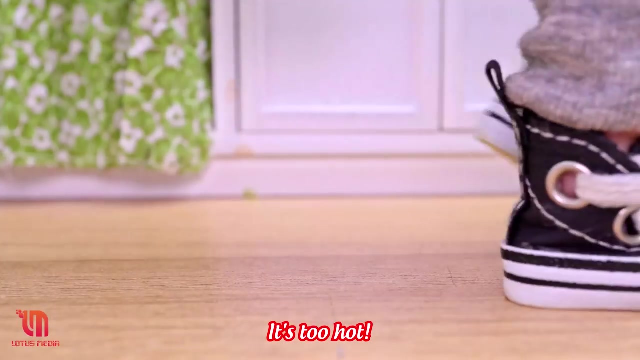 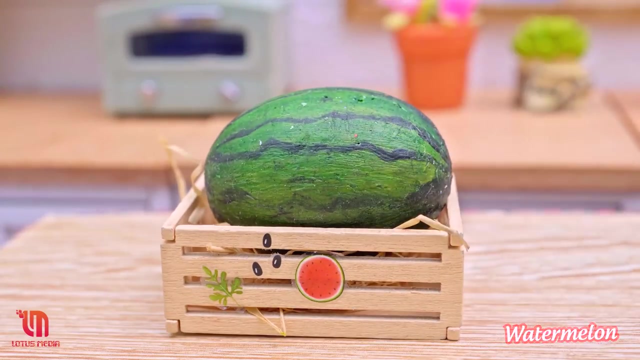 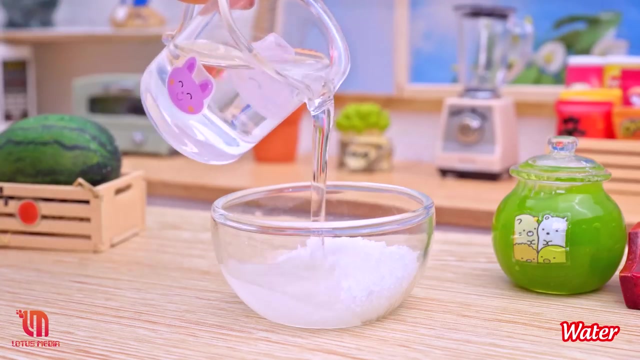 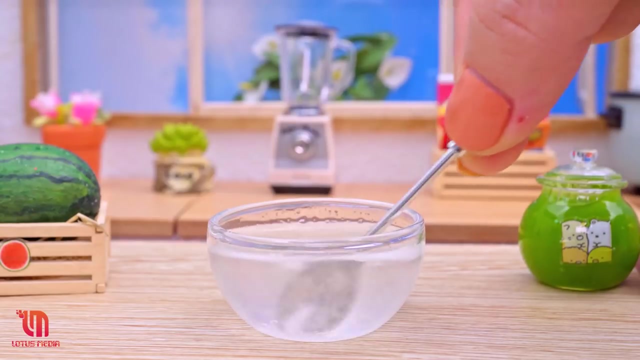 Wow, I love it. Delicious, Tasty, Wow, Sweet, Yummy, It's too hot. Oh, we have watermelons. Let's cook some cool sweets. Let's go, I'm going to make a little cake. 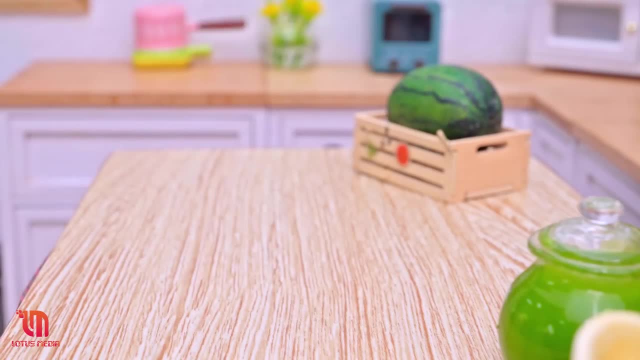 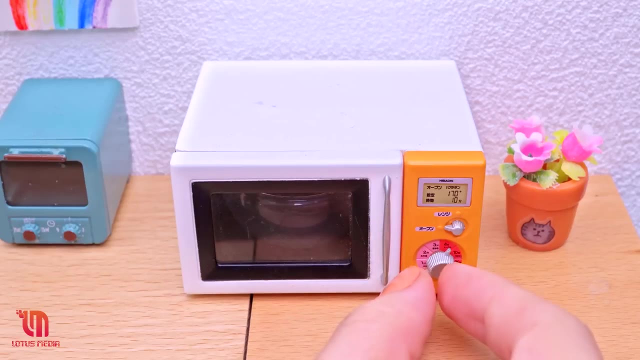 Gonna make a cake with this. I'm going to make a cake with this. This is cool. This is cool. Hello, where are you from? I'm fromiras. I'm going to make a cake. I'm going to make a cake. 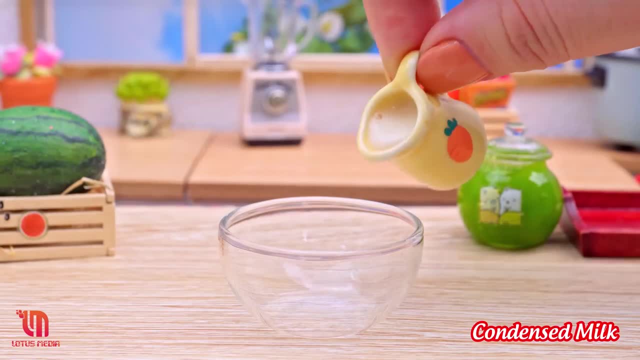 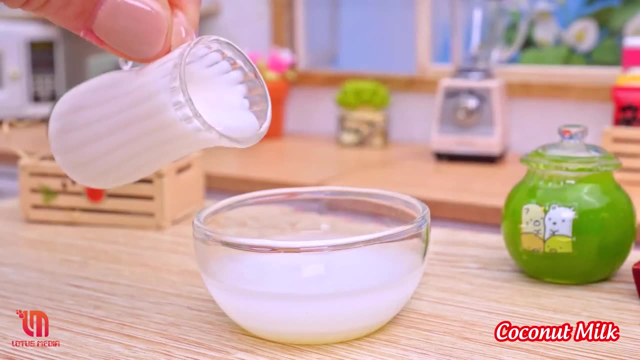 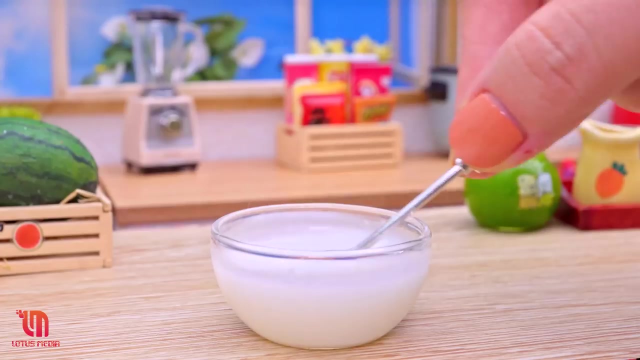 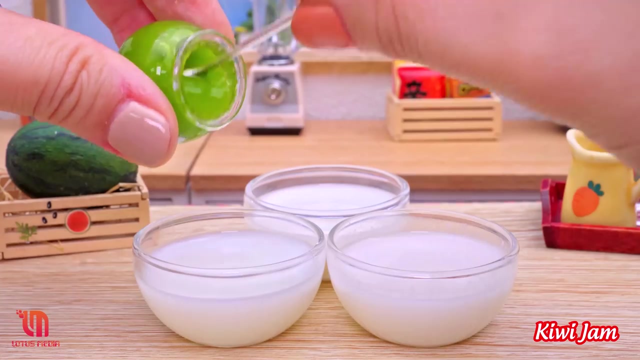 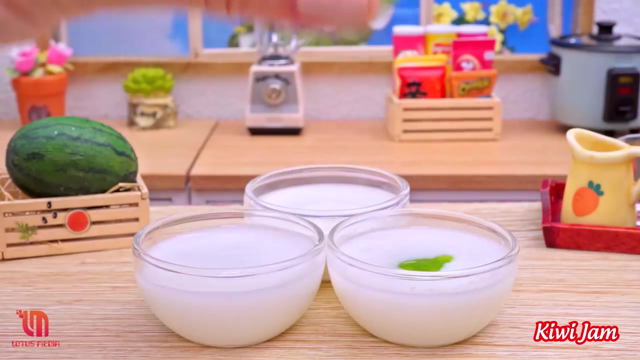 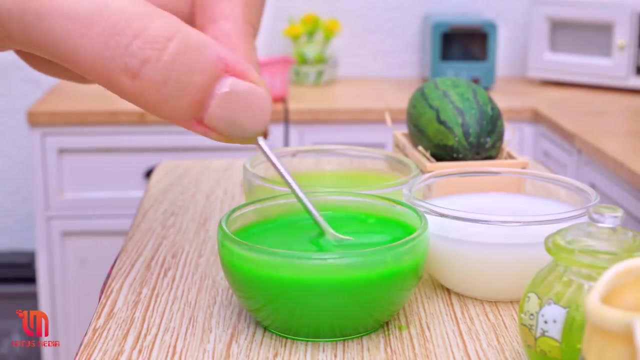 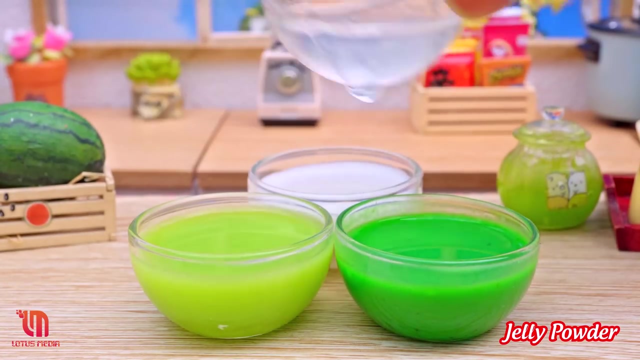 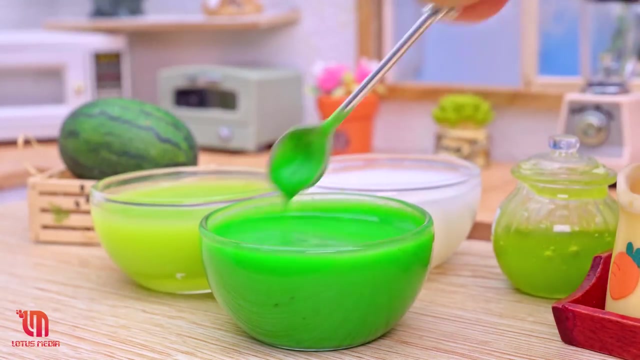 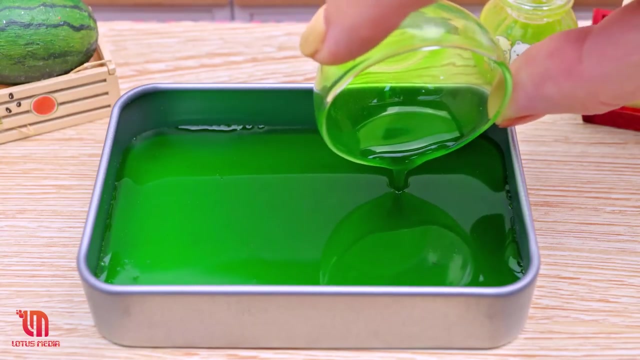 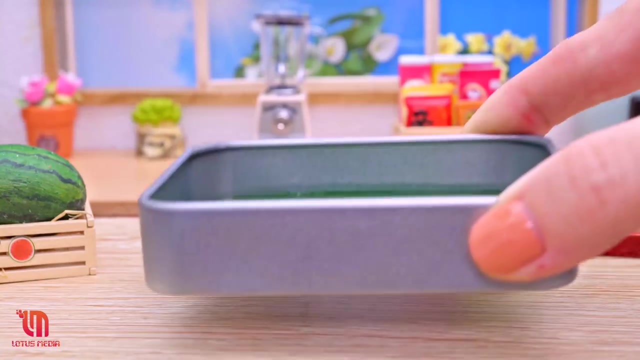 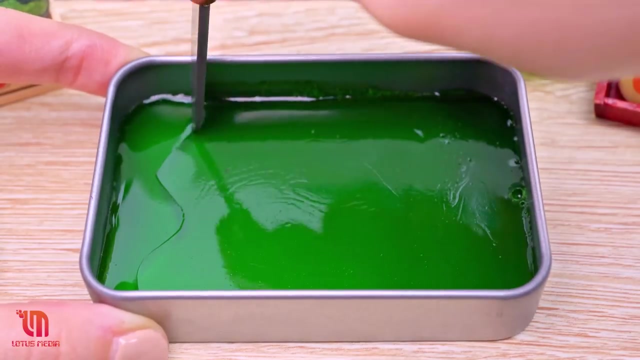 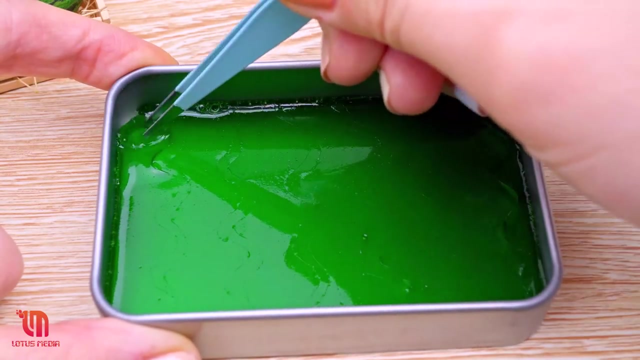 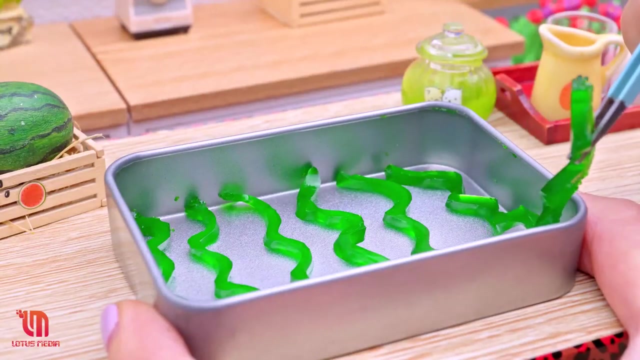 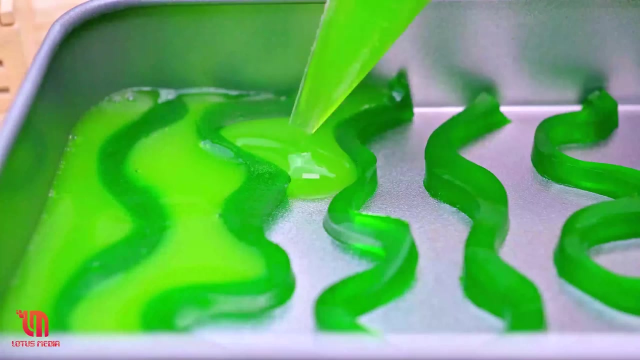 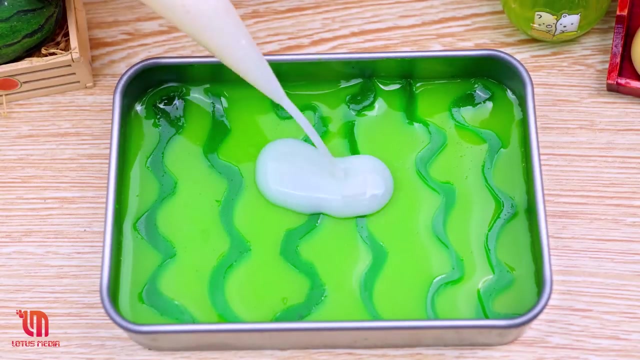 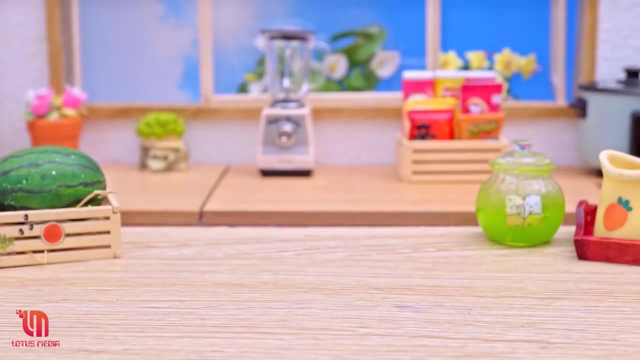 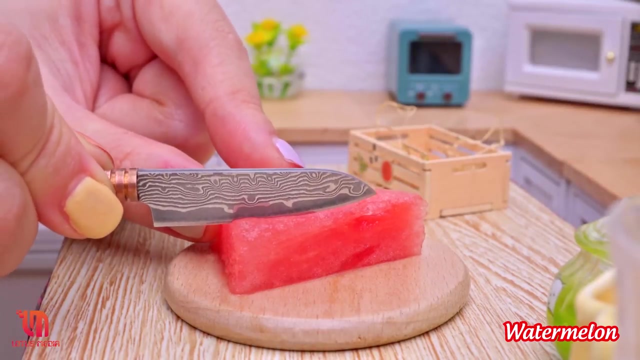 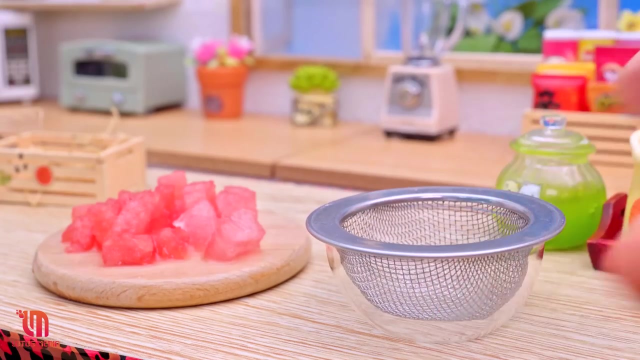 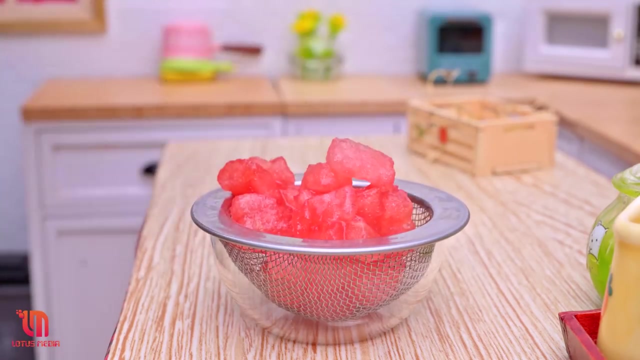 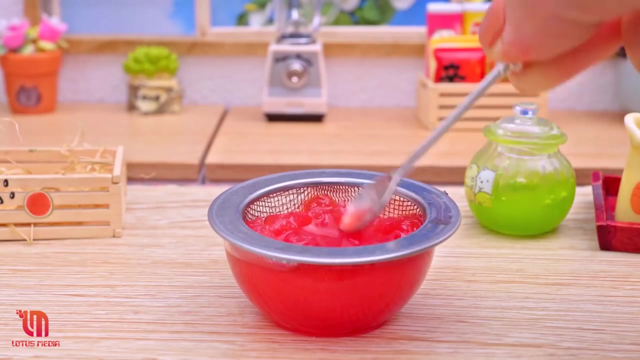 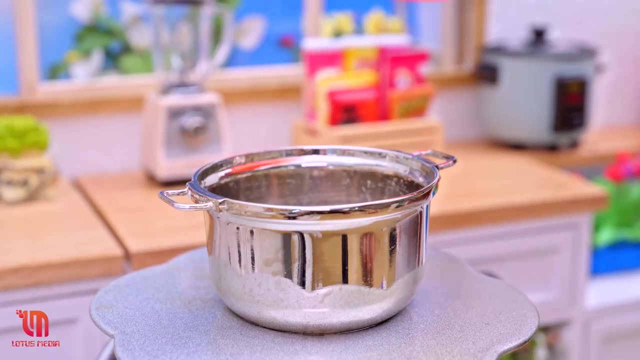 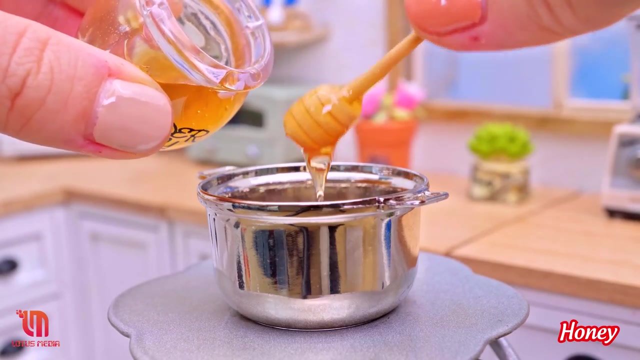 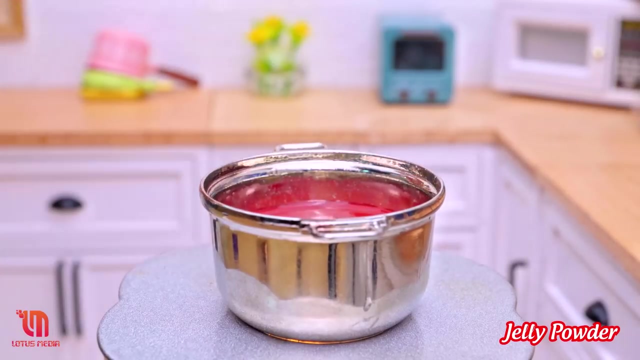 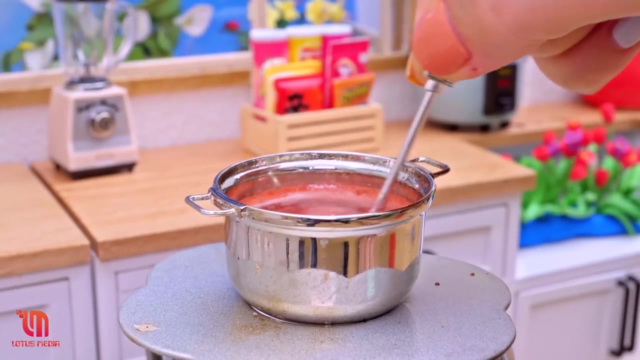 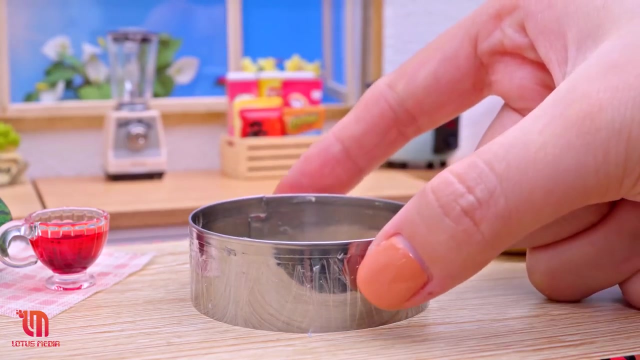 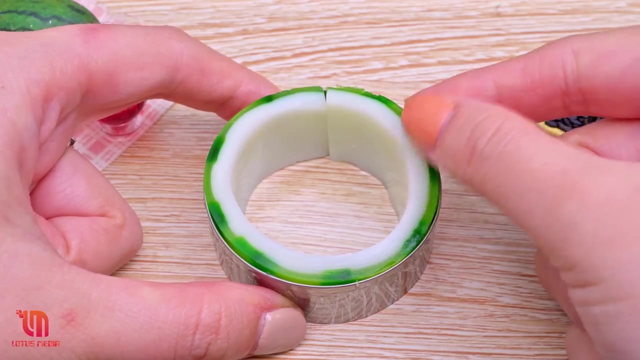 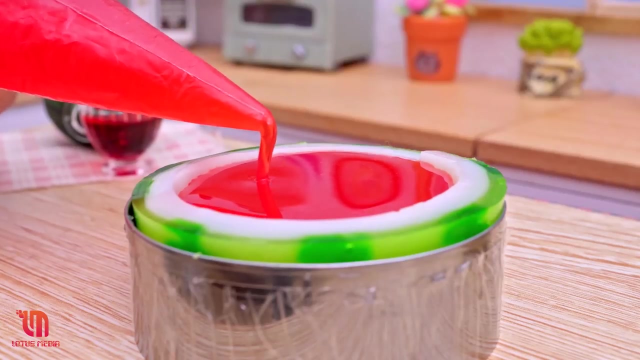 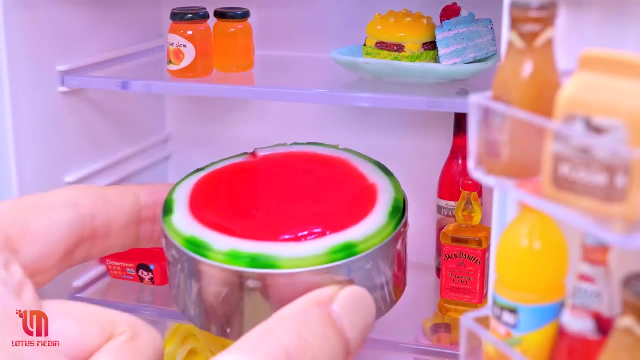 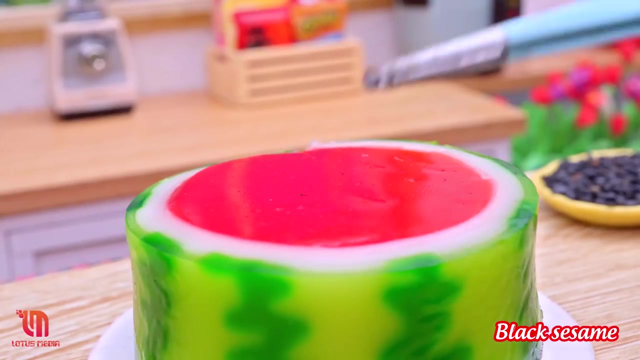 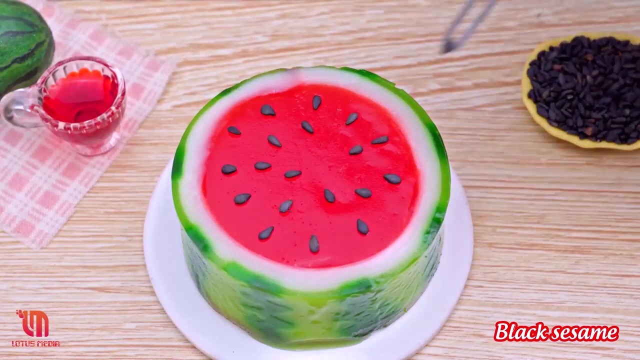 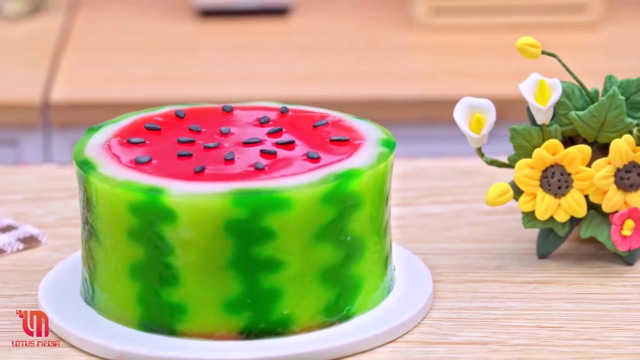 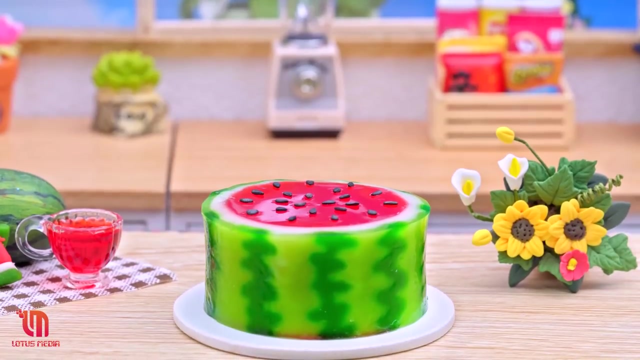 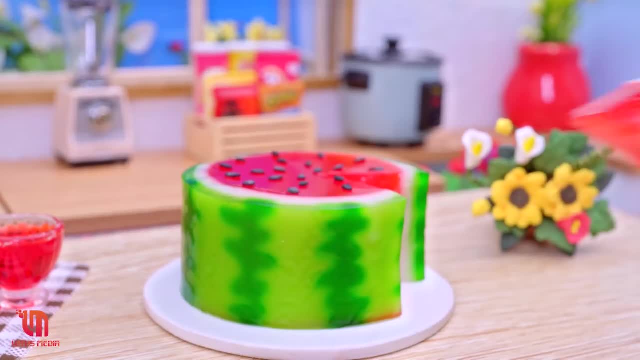 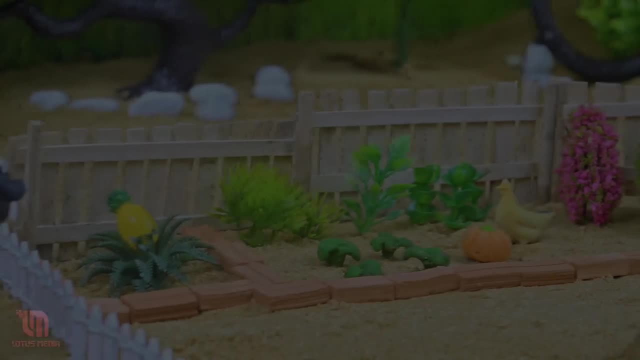 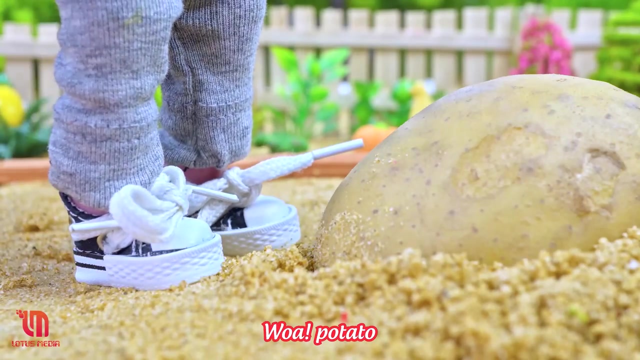 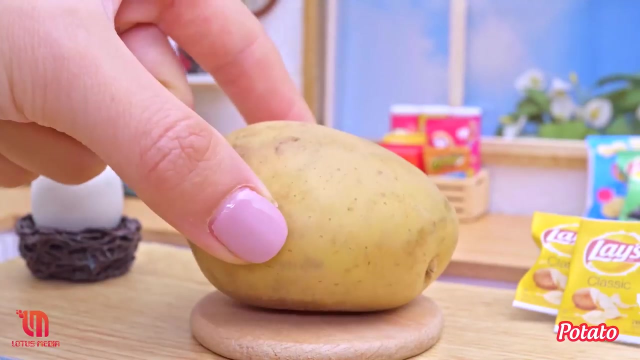 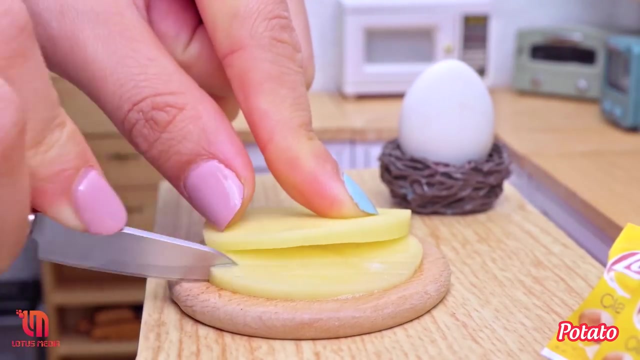 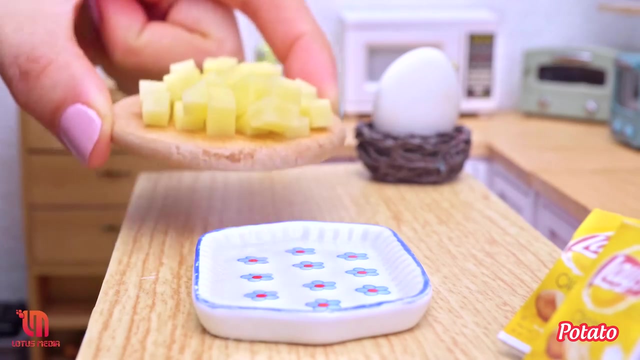 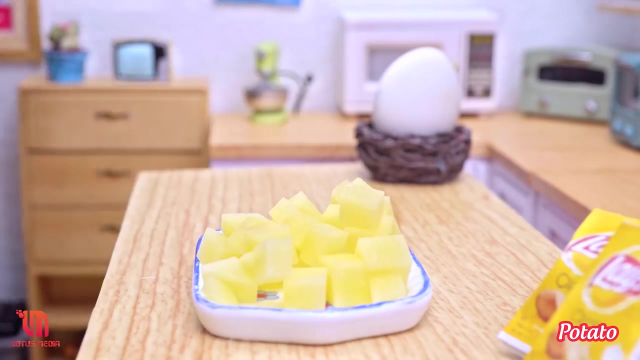 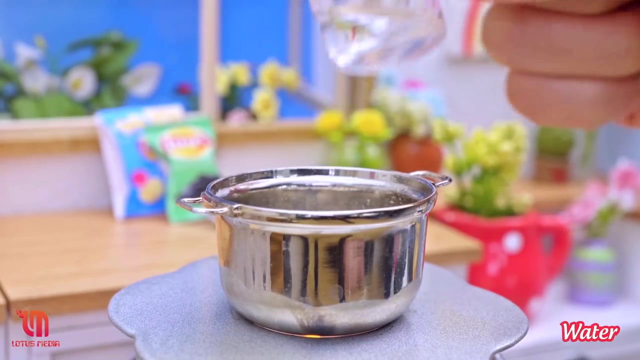 Tasty. Oh wow, Oh wow, Oh wow. Cut the chicken into small pieces. Cut the chicken into small pieces. Cut the chicken into small pieces. Put the chicken in a bowl, Add water, Add salt, Add pepper. 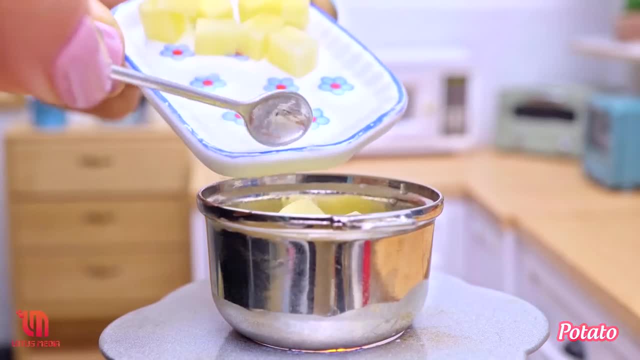 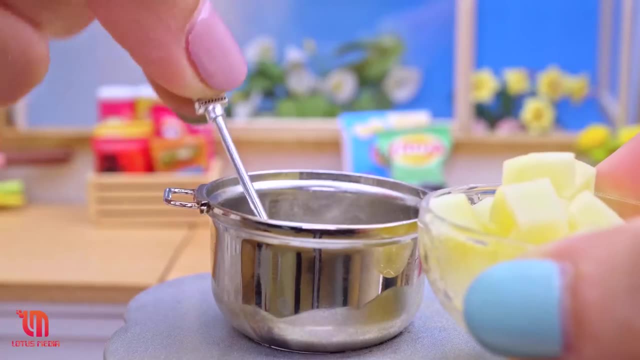 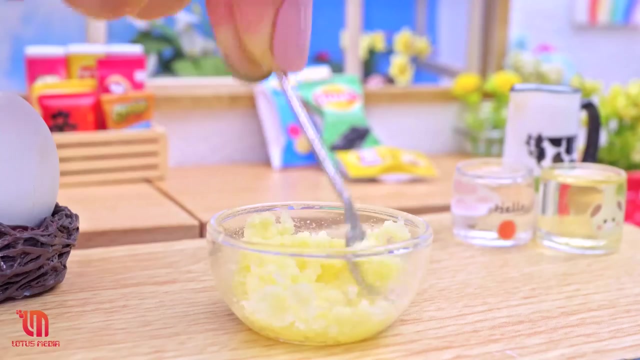 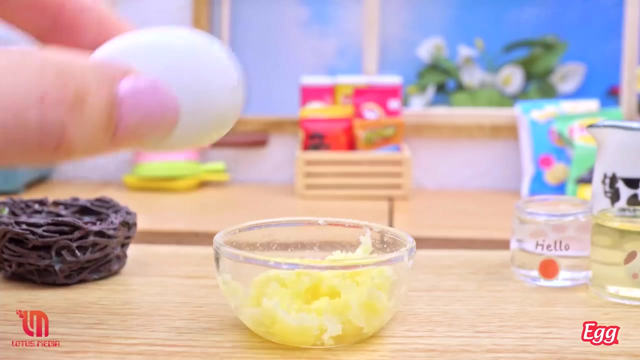 Add pepper. Mix three times, Mix one more time. Mix three times. Boil the chicken in a pot and pour in a little water. Add the tomatoes and season them. Add oil, Add eggs, Add rice as well. Add red pepper. 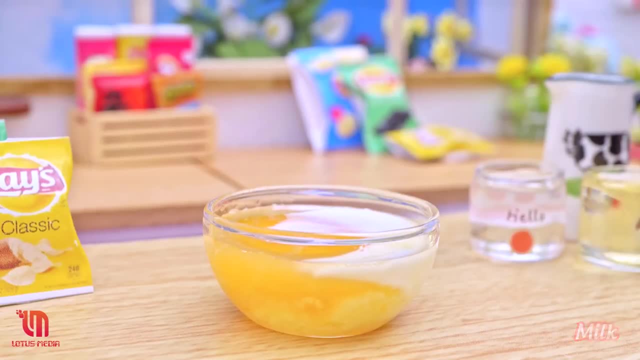 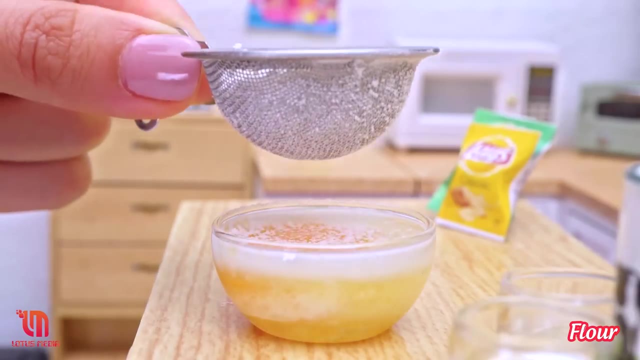 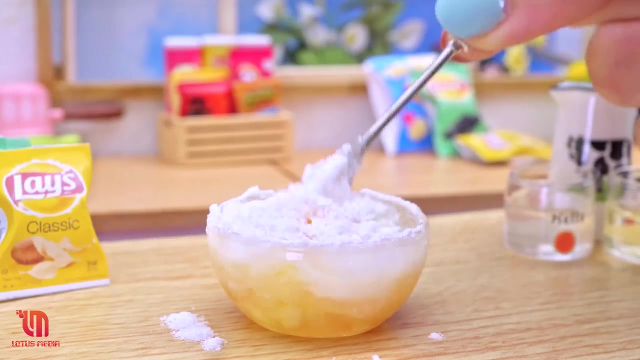 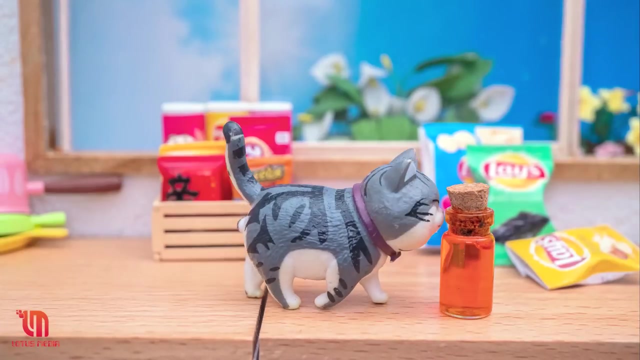 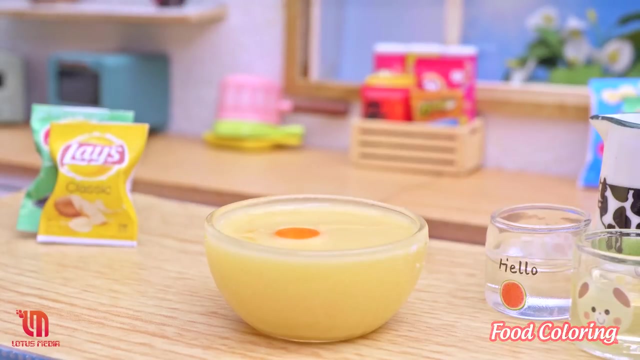 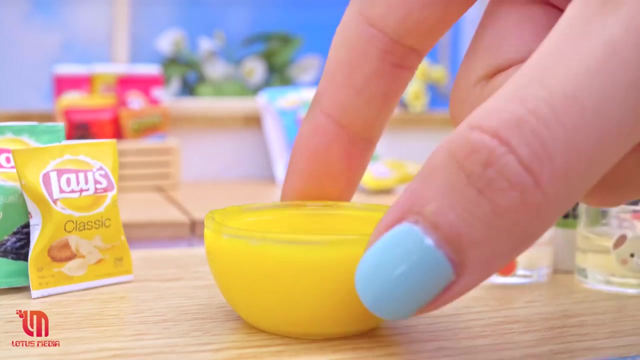 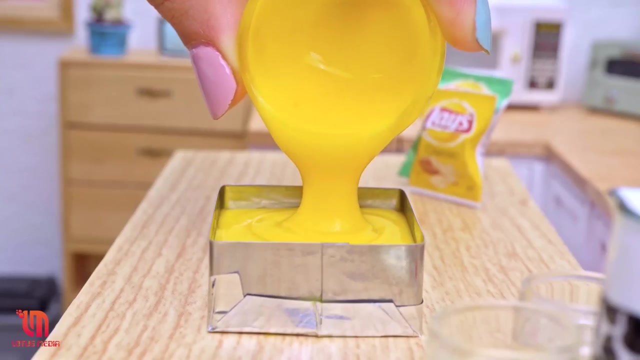 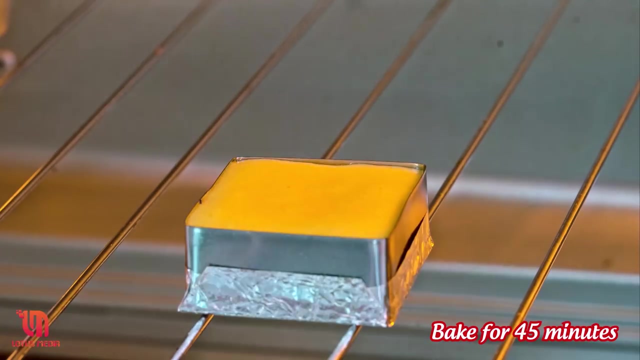 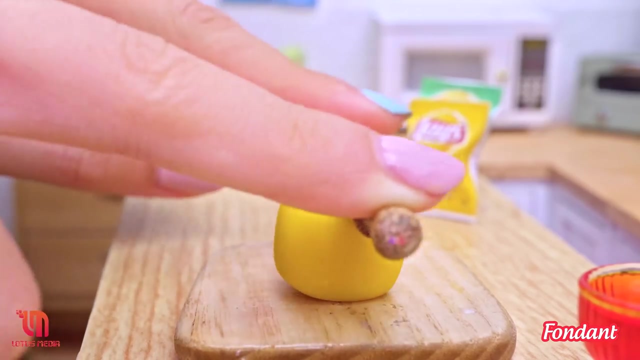 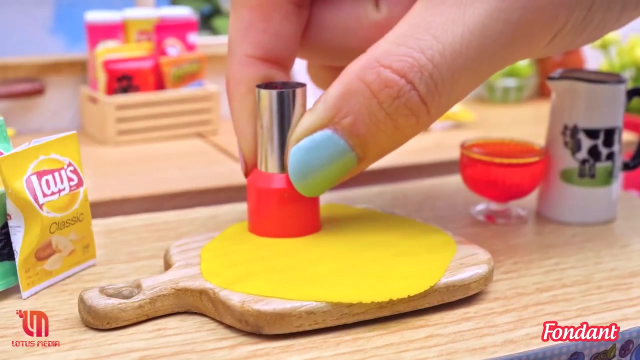 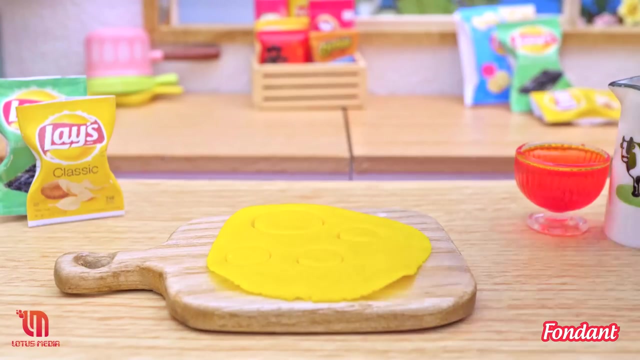 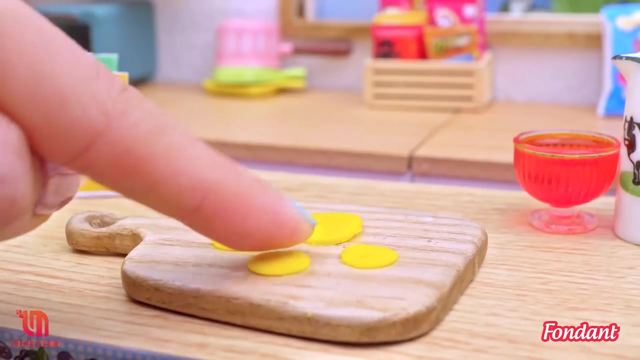 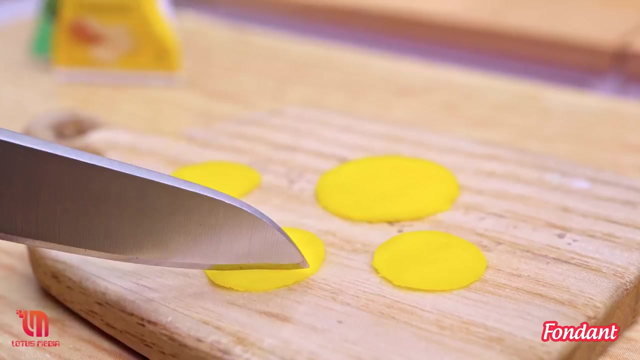 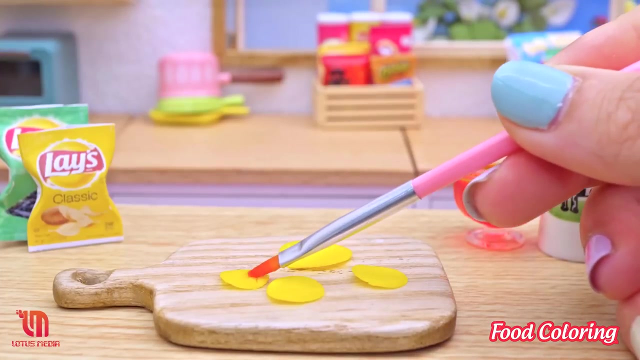 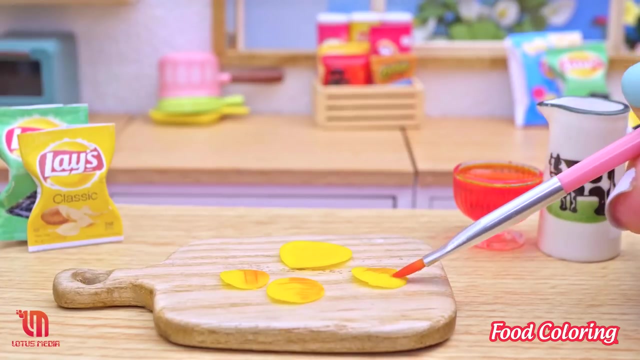 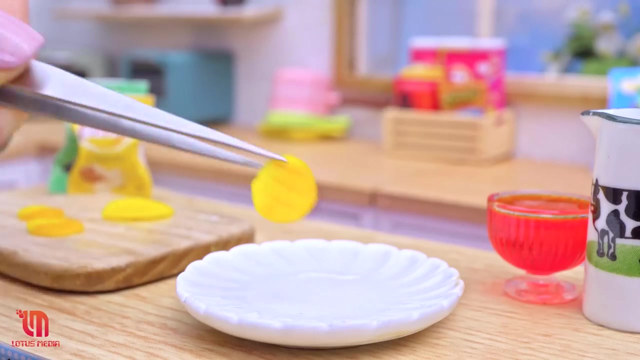 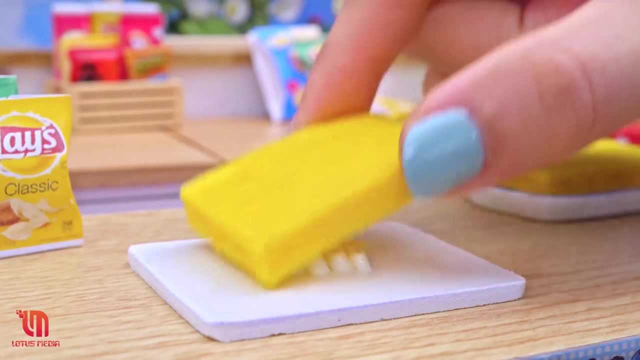 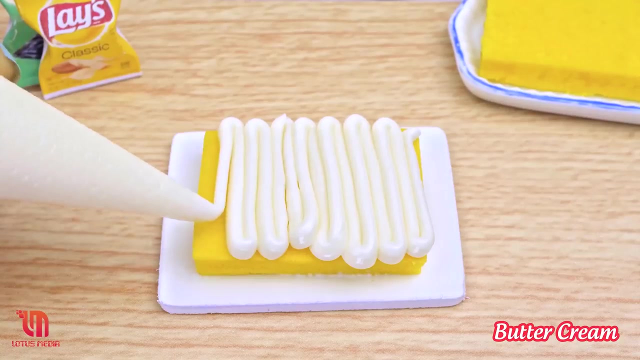 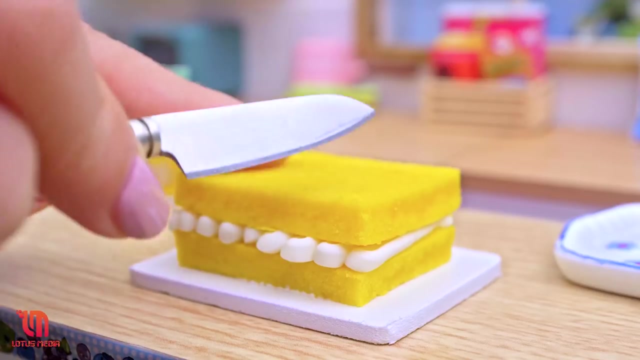 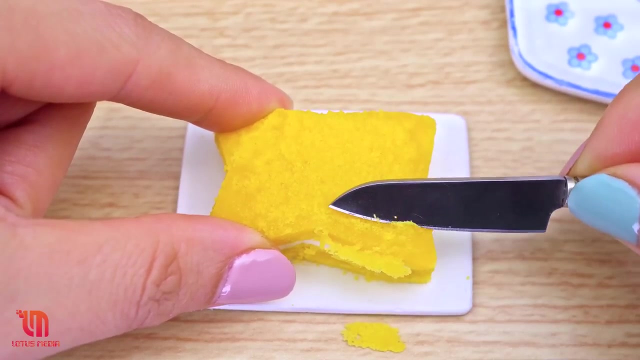 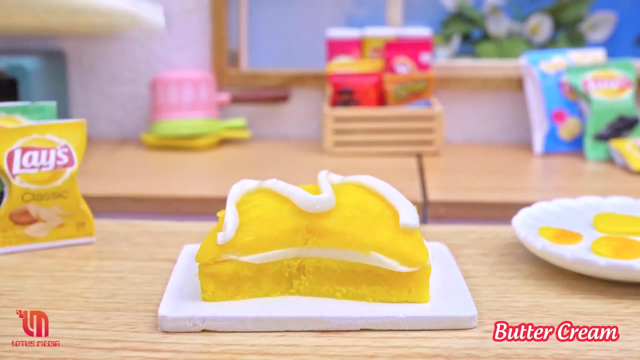 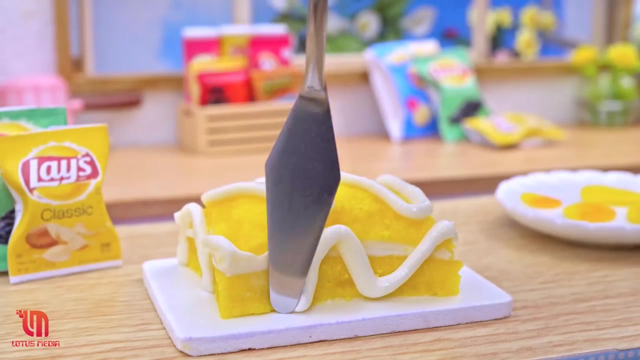 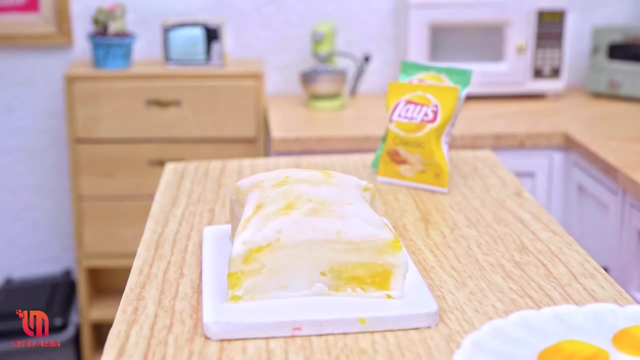 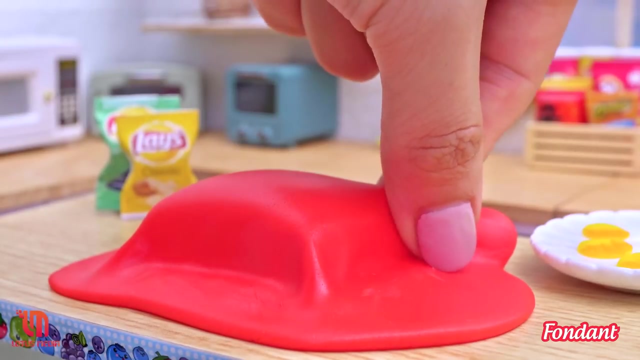 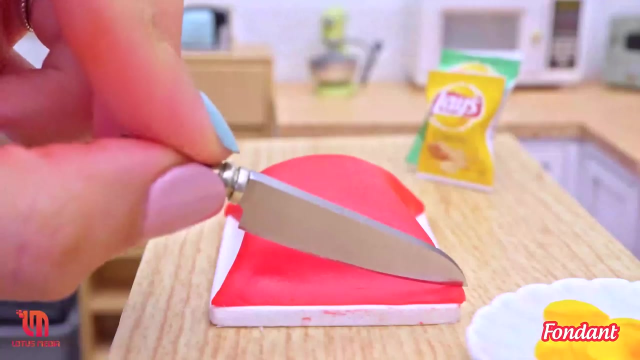 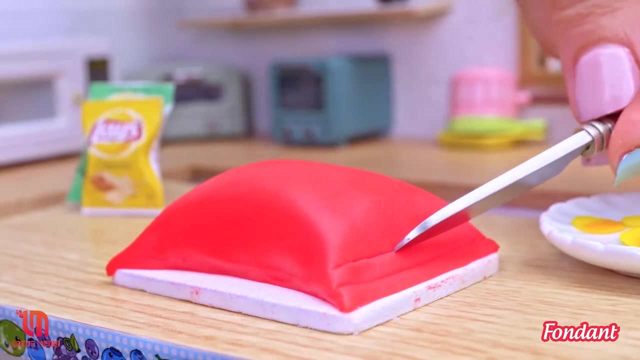 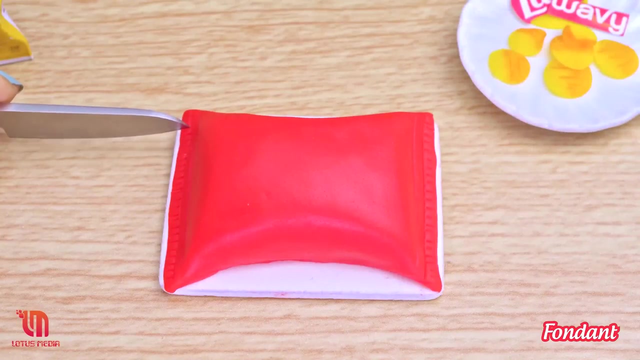 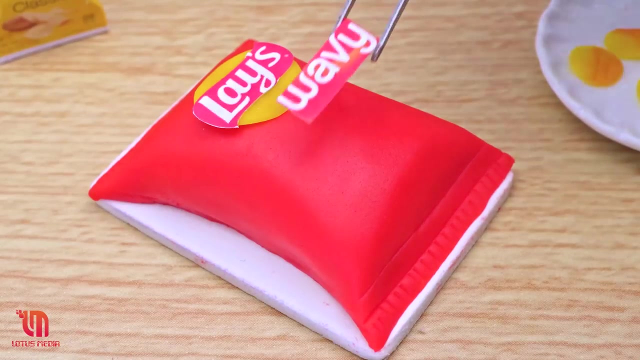 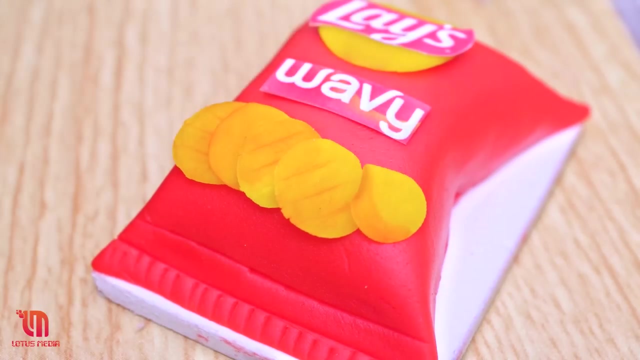 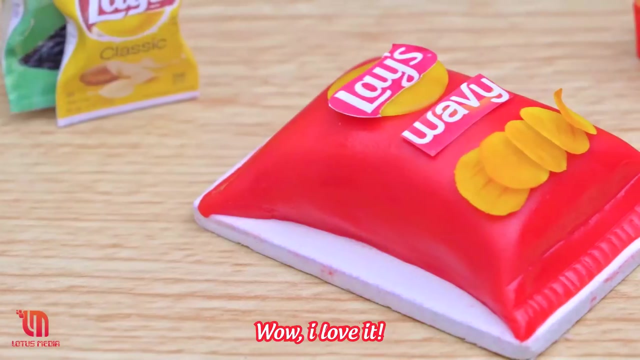 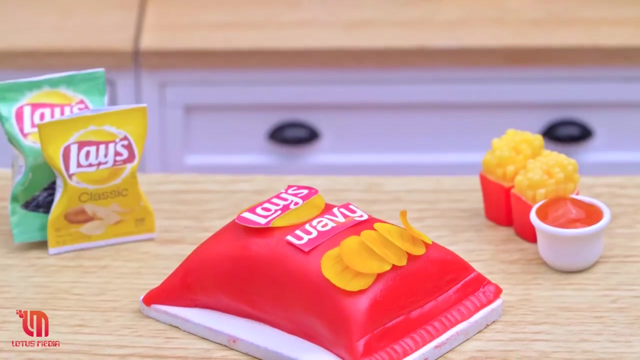 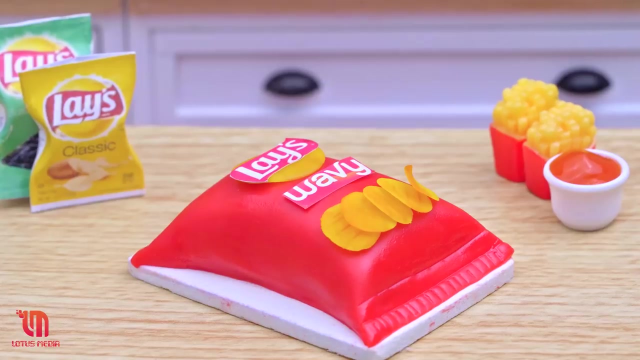 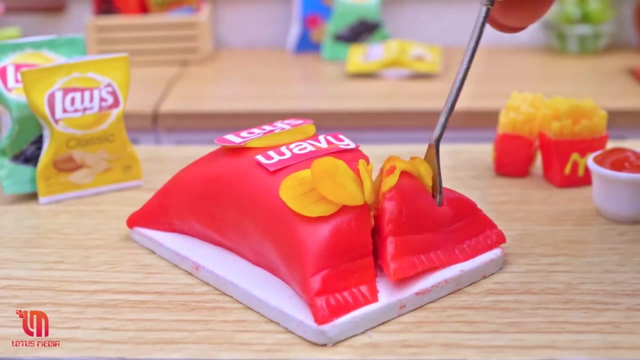 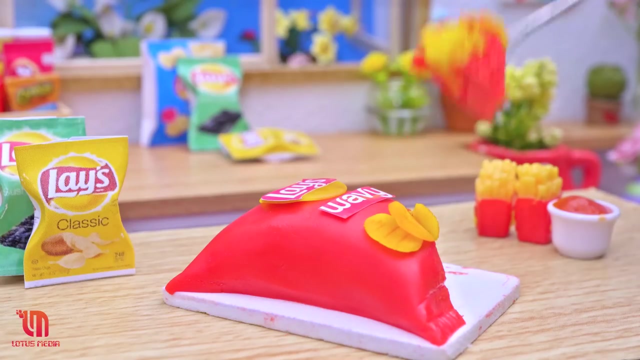 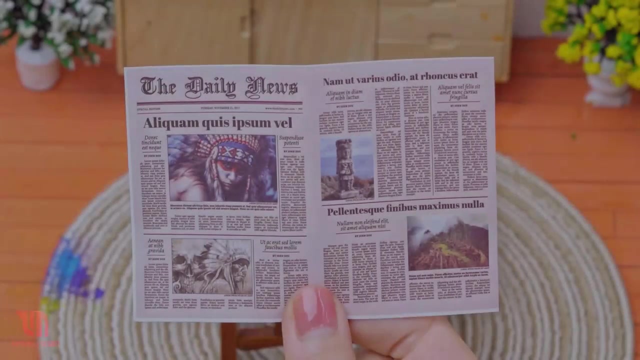 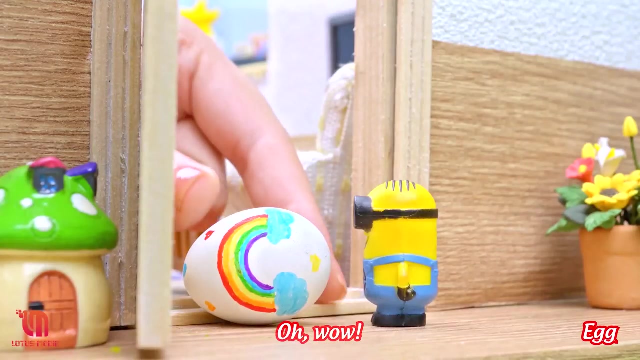 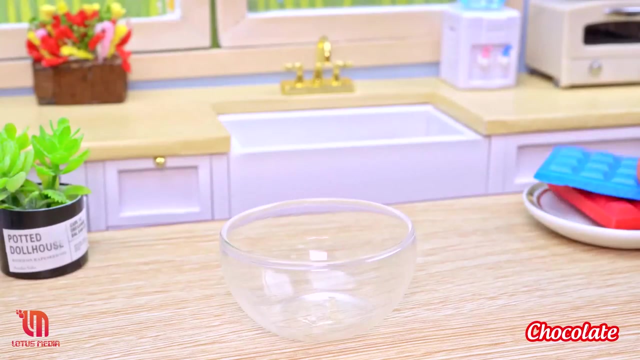 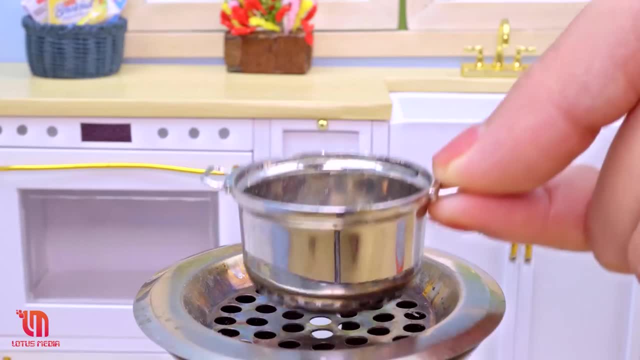 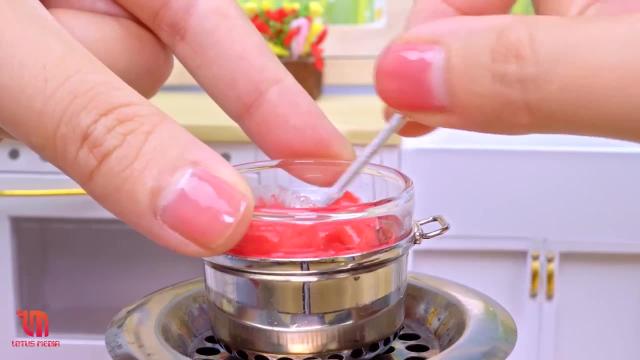 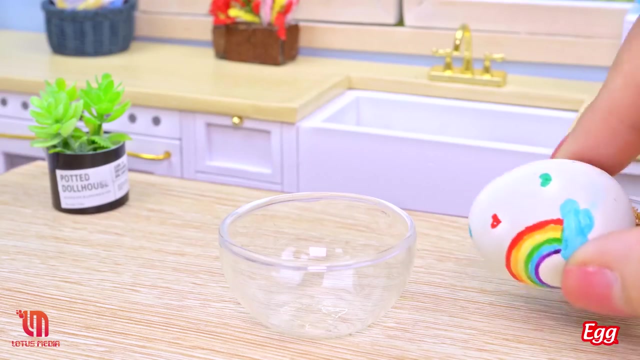 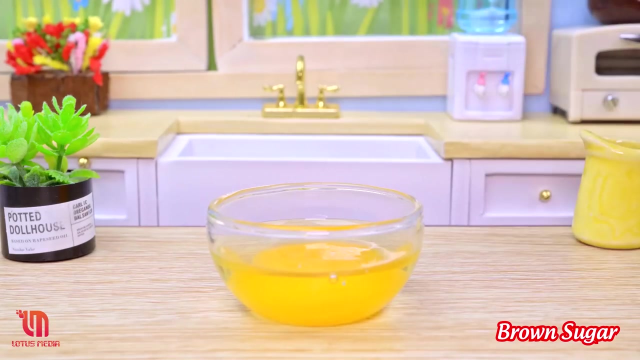 Thank you, You're welcome. Bye-bye. Add 1 tablespoon of soy sauce and 1 tablespoon of cooking wine to the pan and stir-fry over medium heat. Add 1 tablespoon of soy sauce and 1 tablespoon of cooking wine and stir-fry over medium heat. 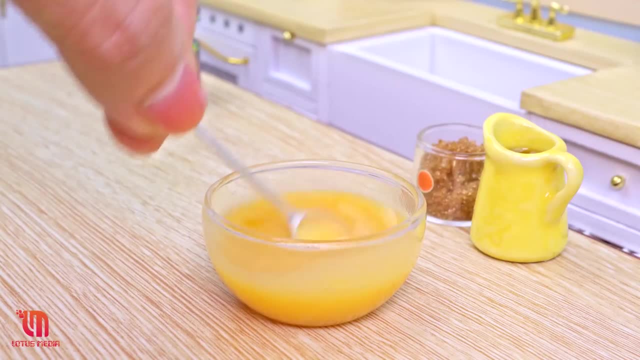 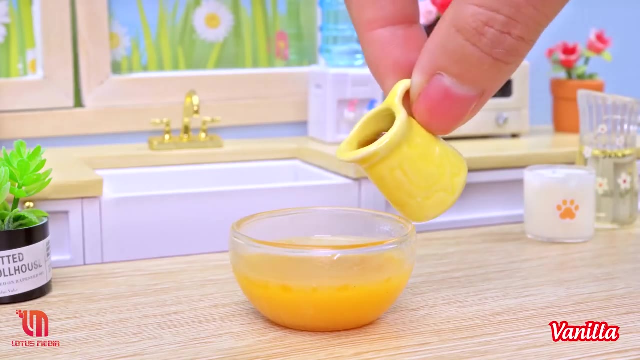 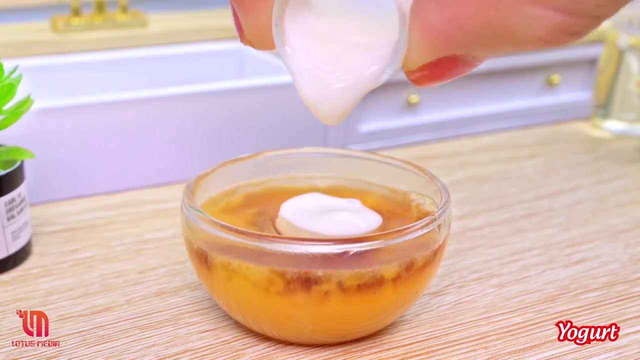 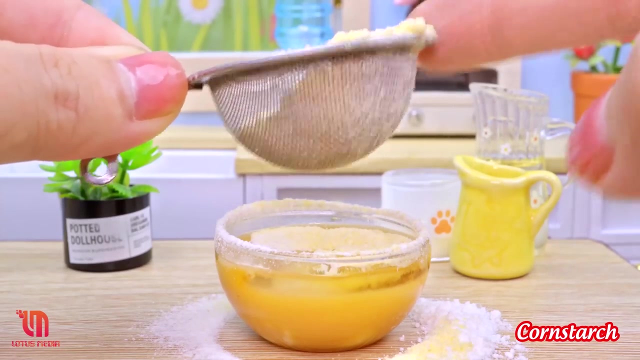 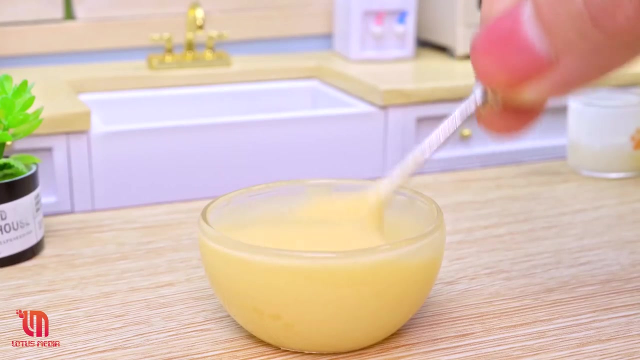 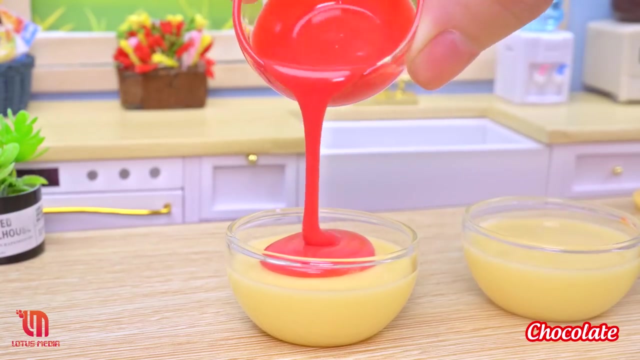 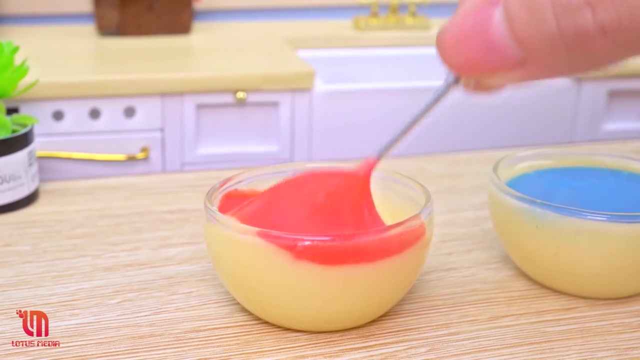 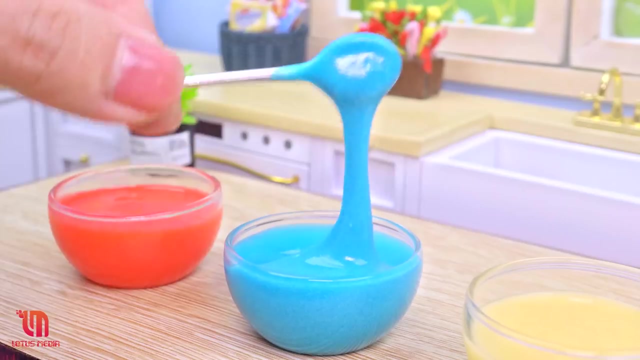 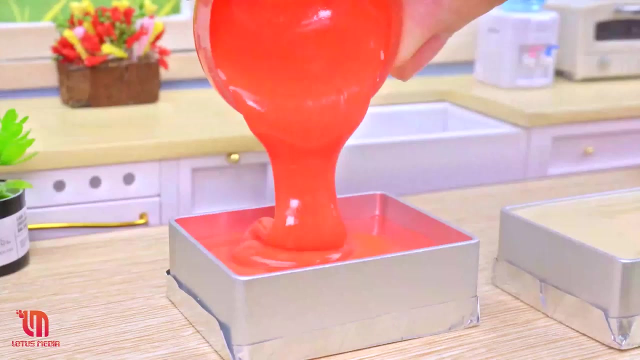 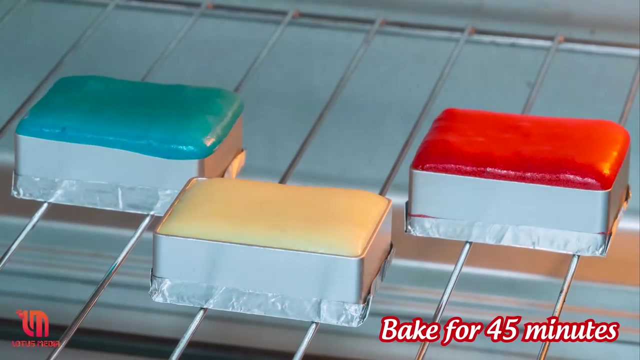 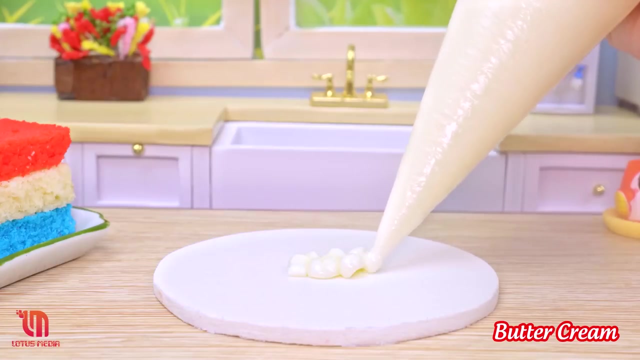 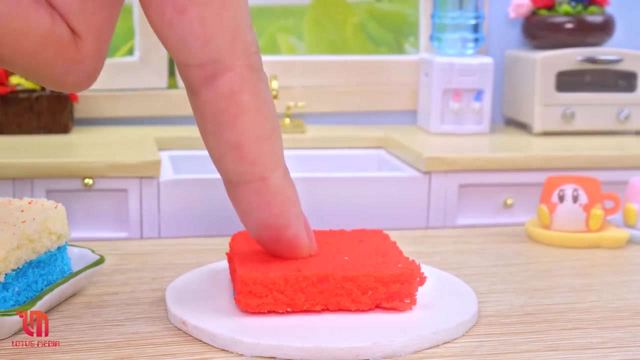 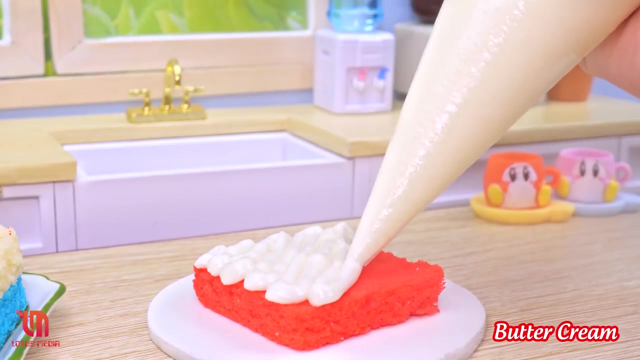 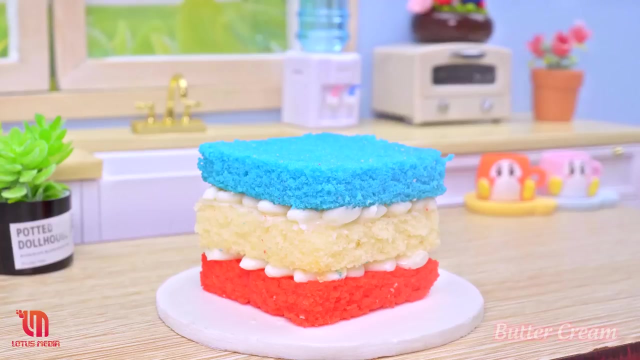 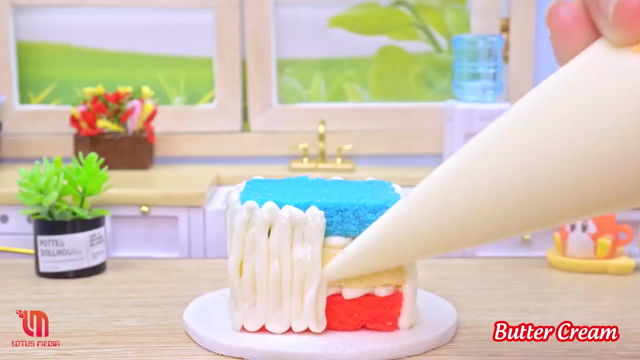 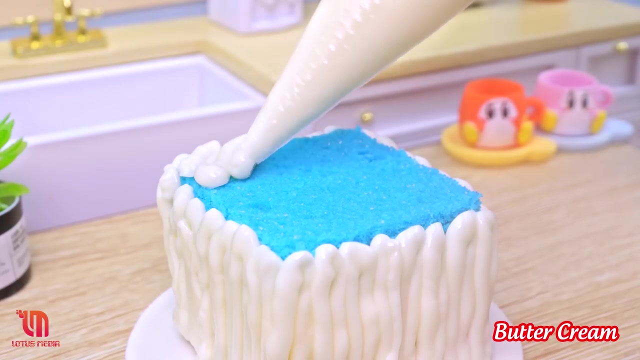 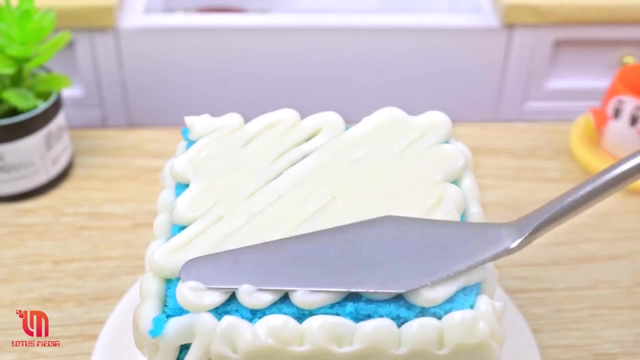 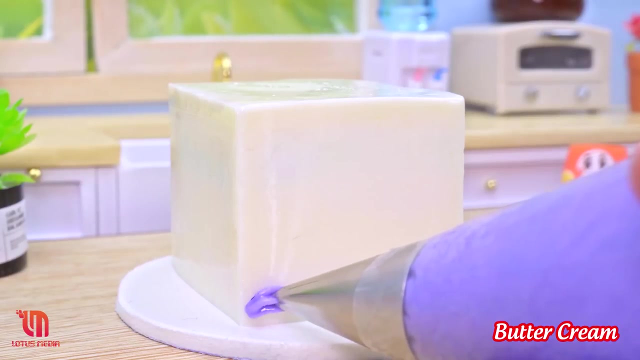 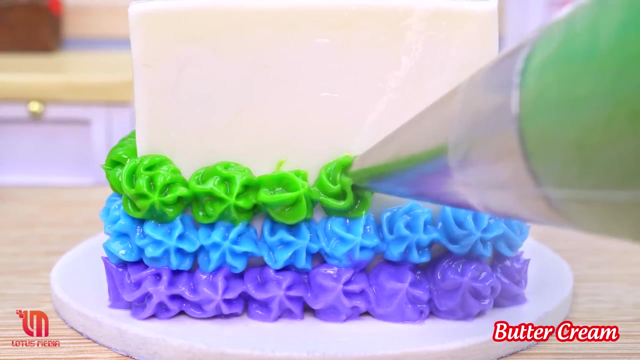 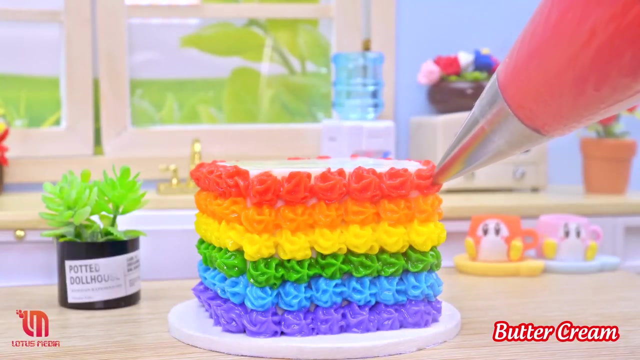 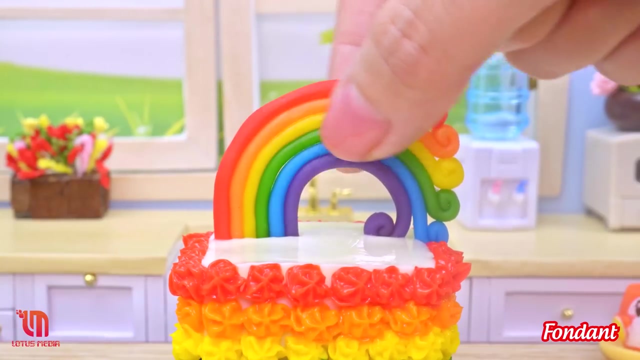 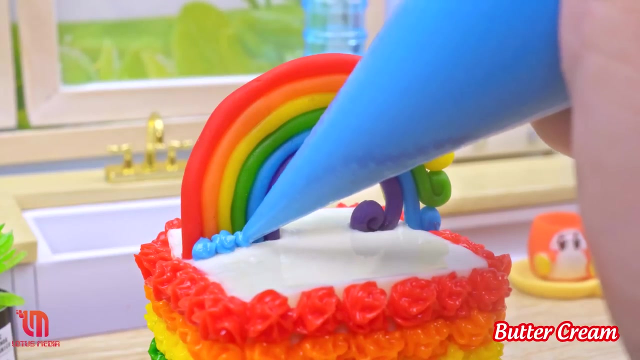 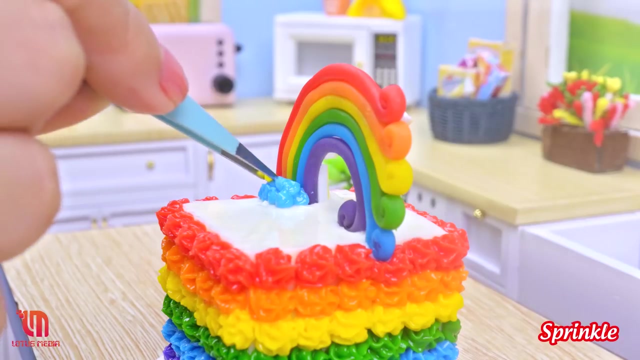 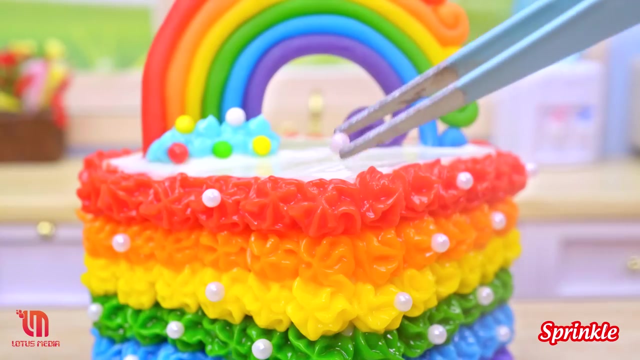 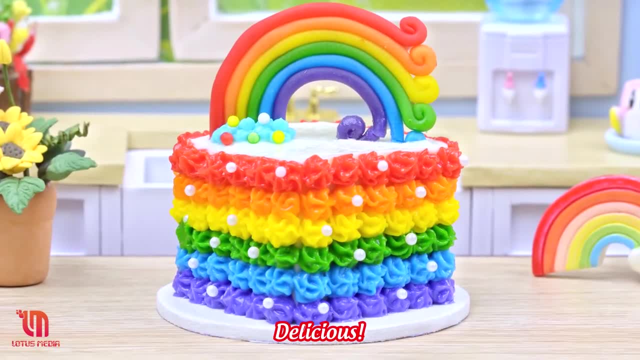 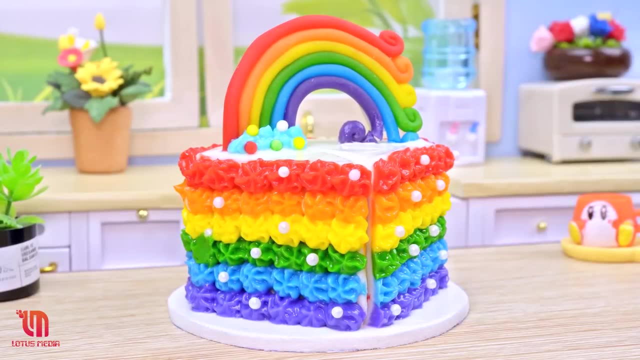 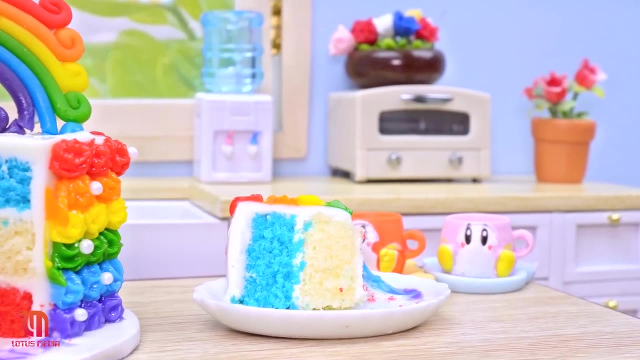 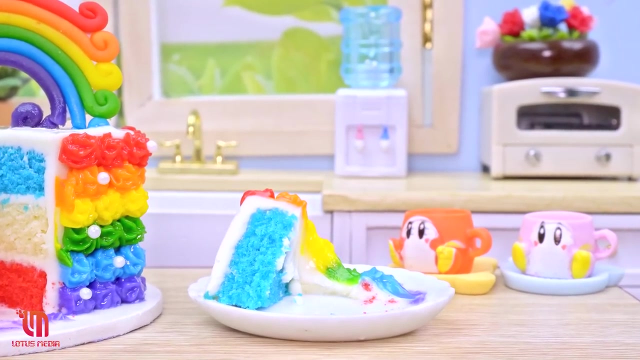 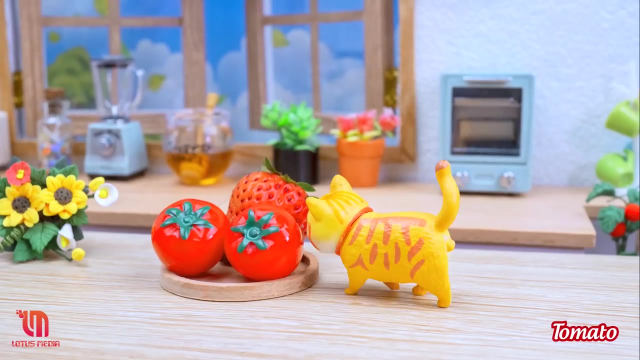 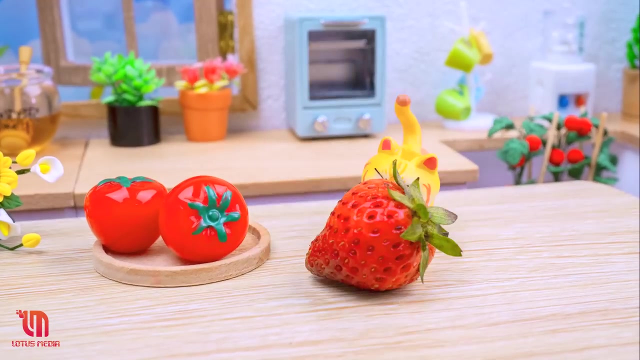 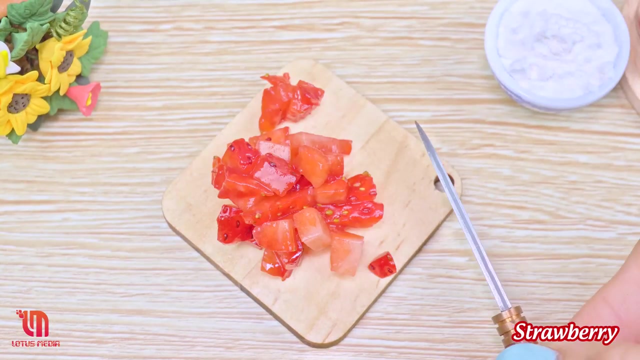 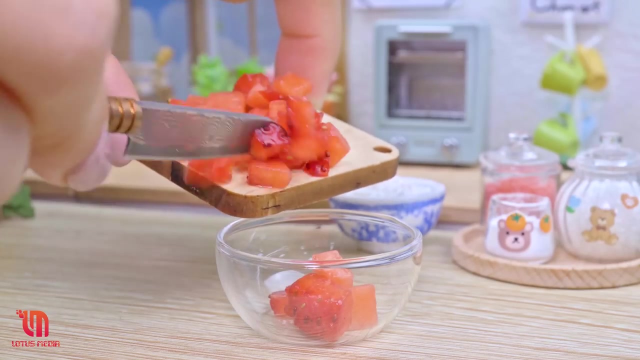 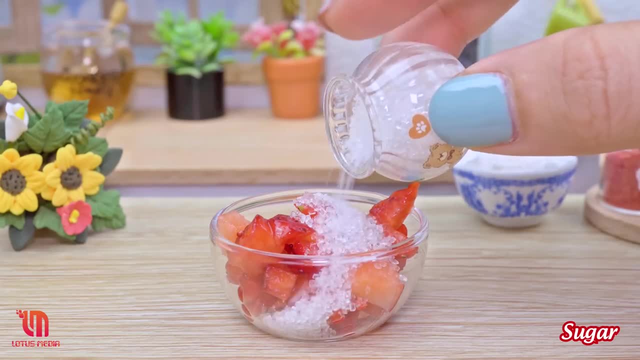 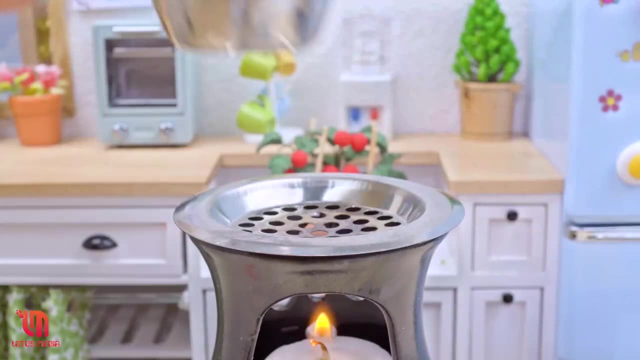 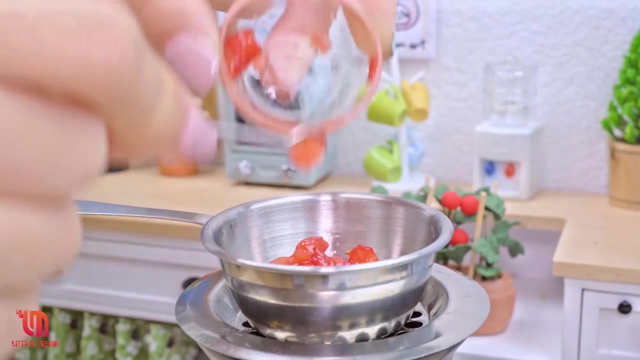 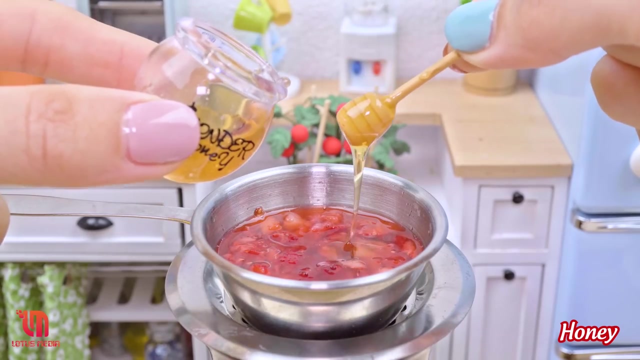 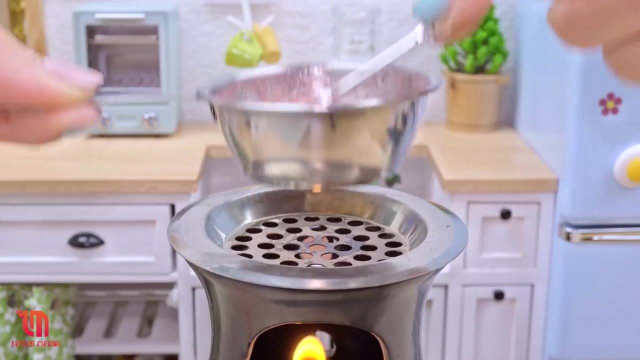 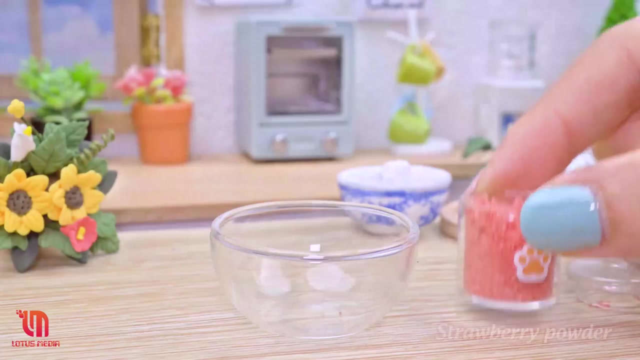 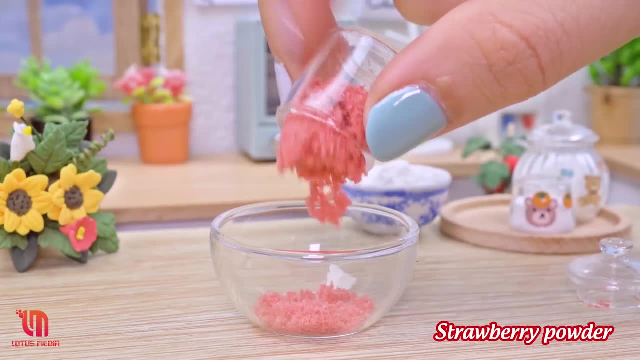 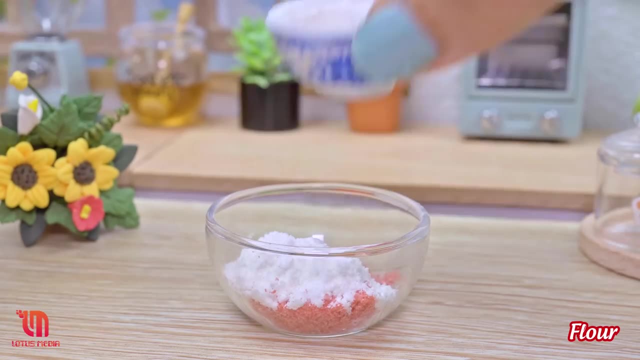 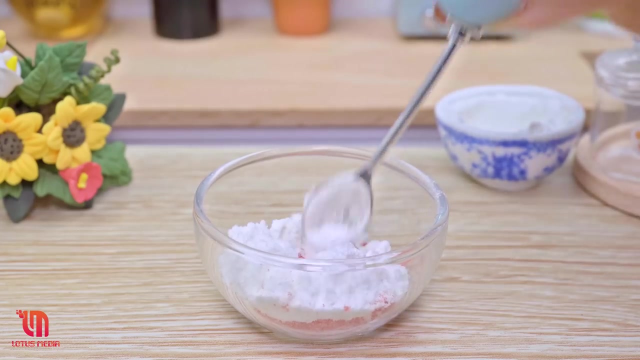 Hello, No doubt, Strawberry, You can use your finger to make it easier to open the lid. The lid is very hard, so it is recommended to use a wooden spoon. You can use a chopstick to make it easier to open the lid. 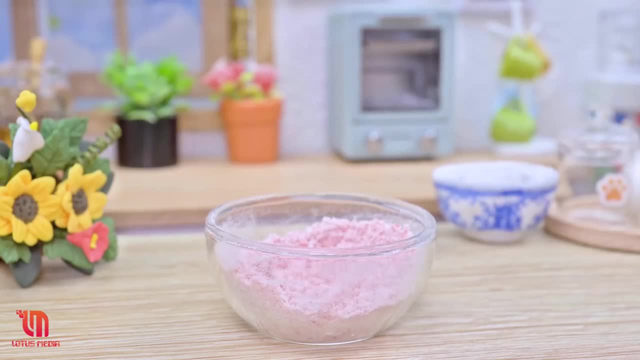 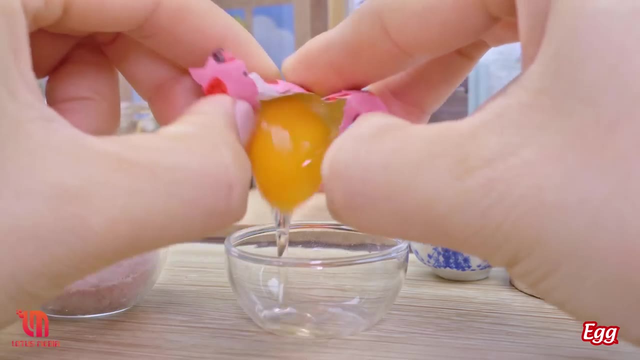 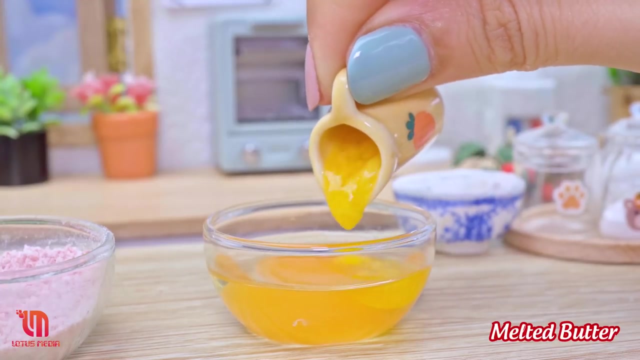 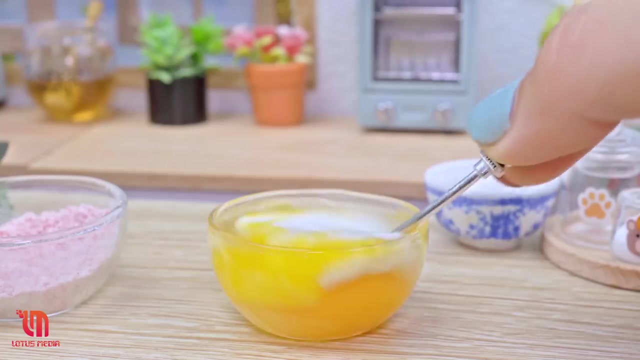 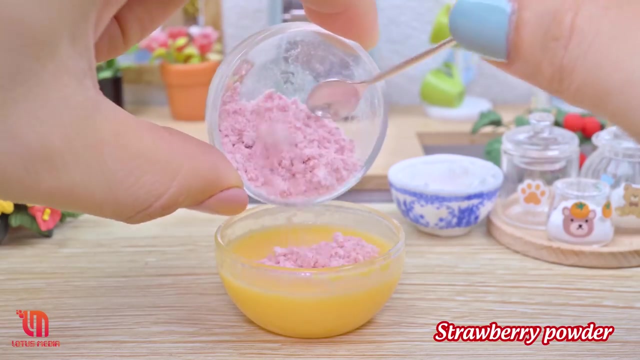 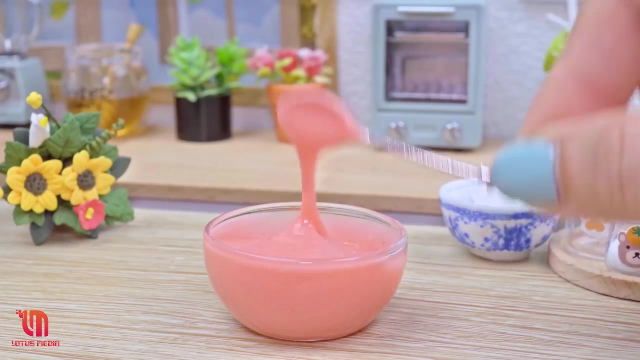 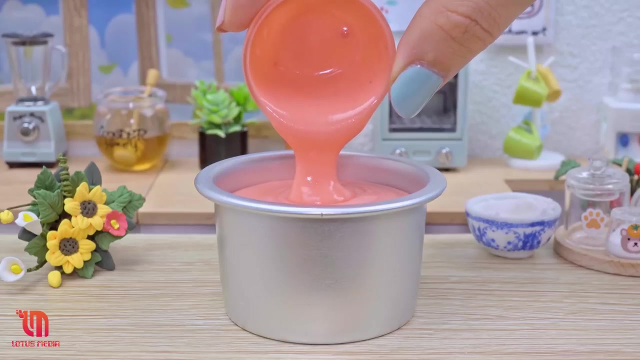 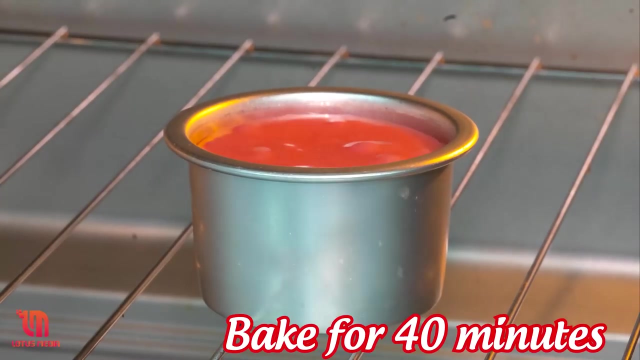 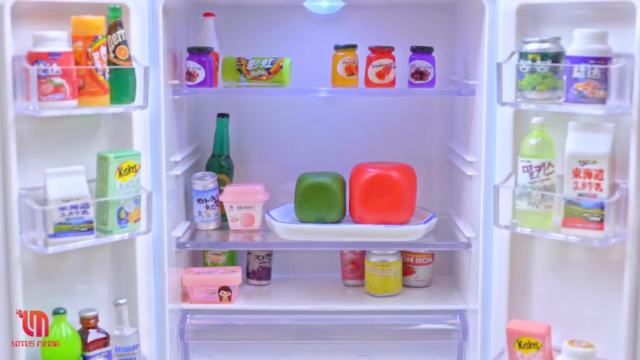 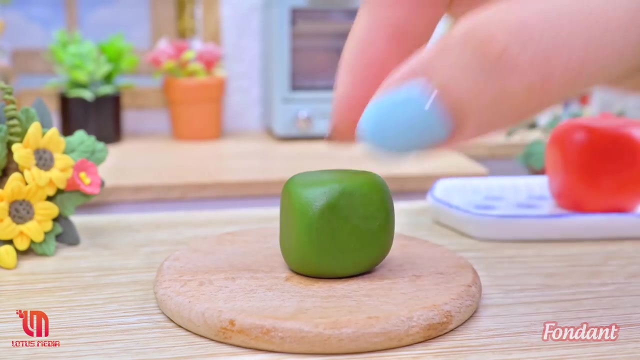 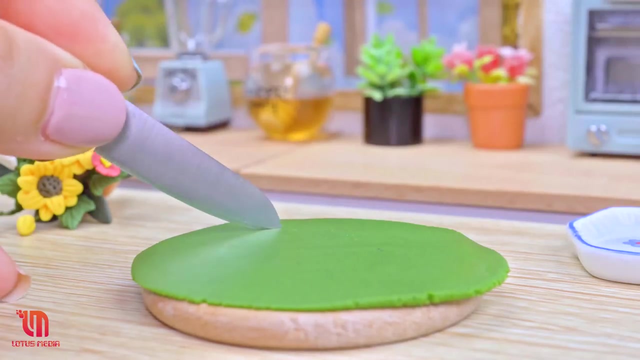 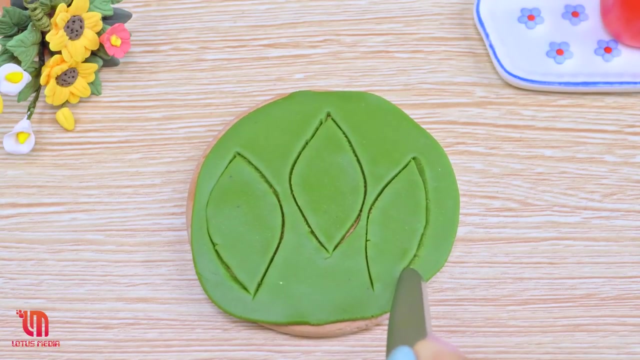 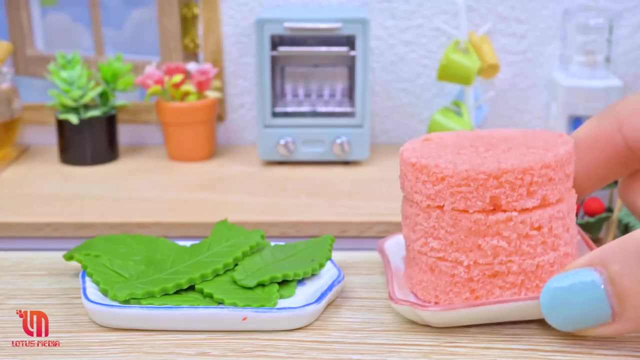 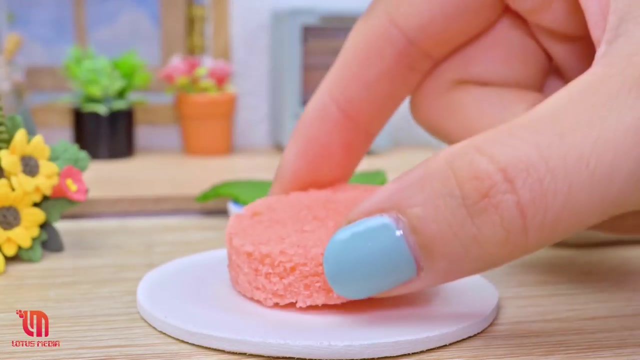 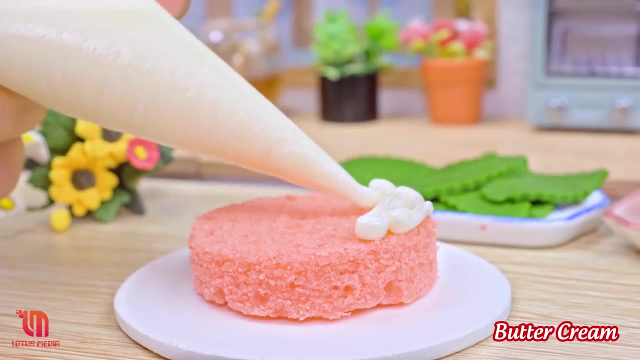 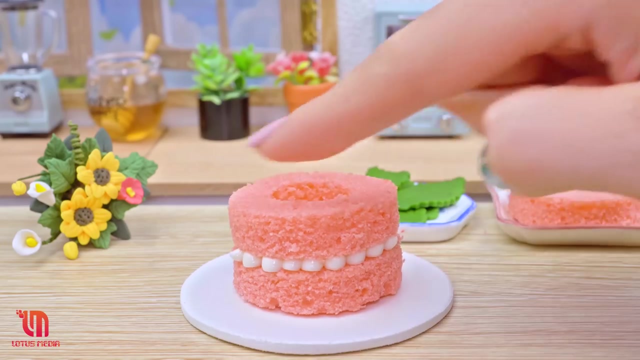 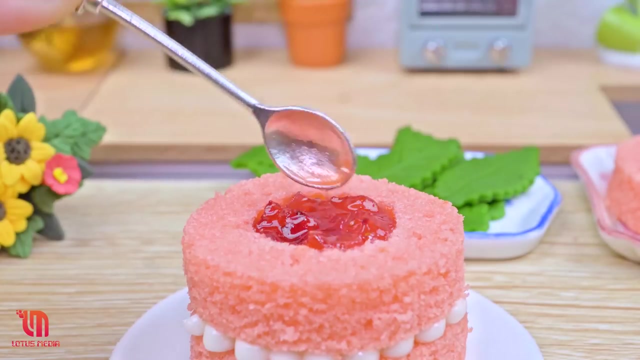 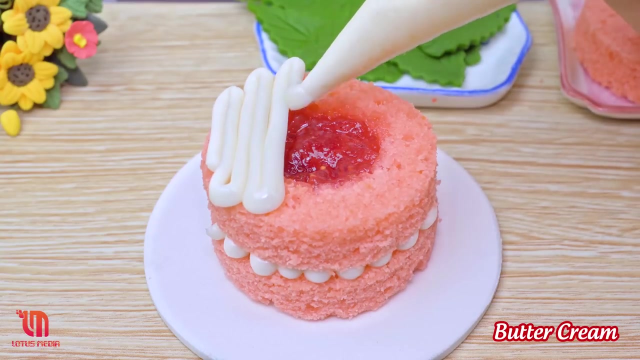 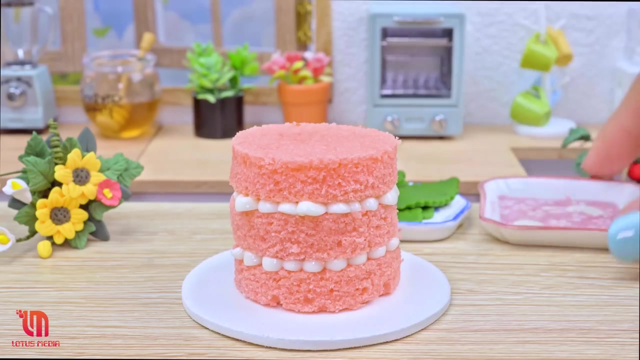 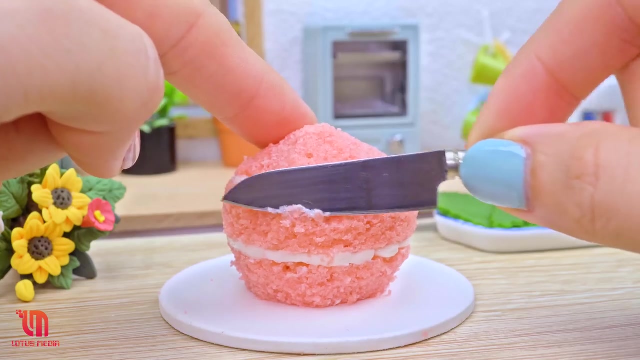 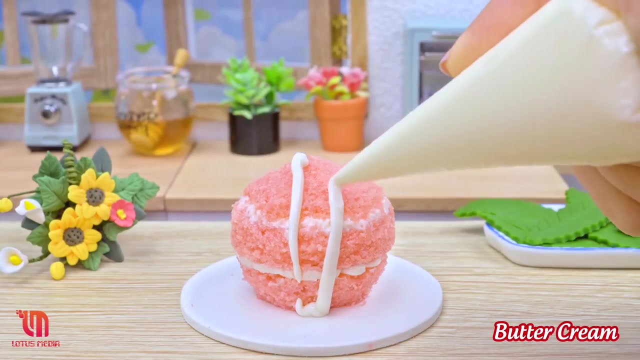 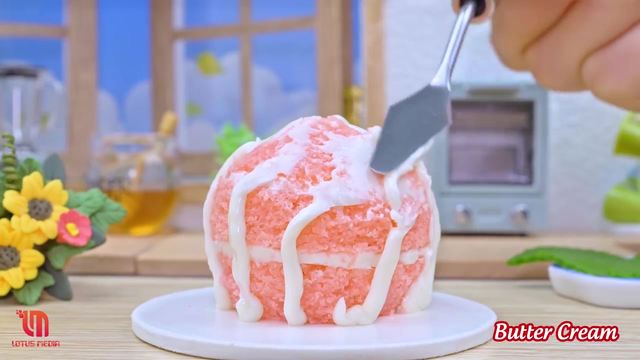 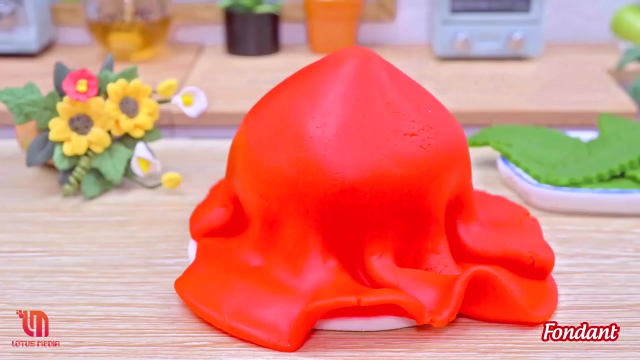 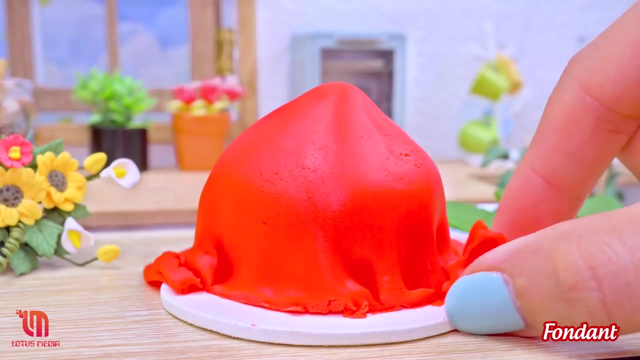 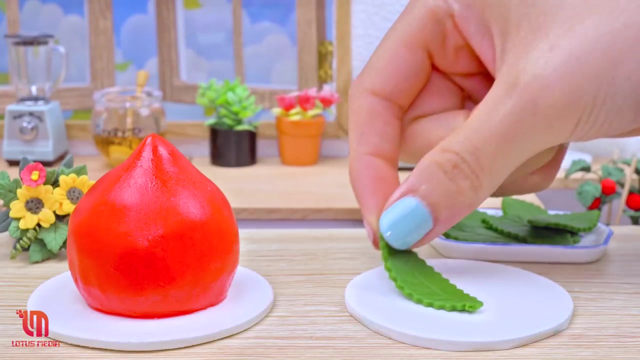 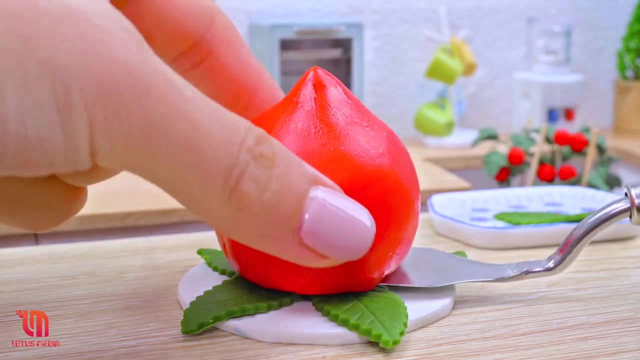 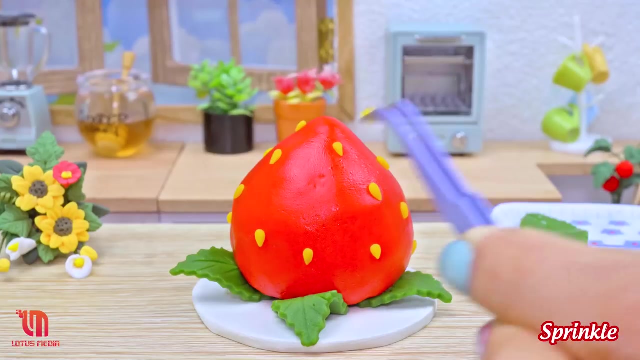 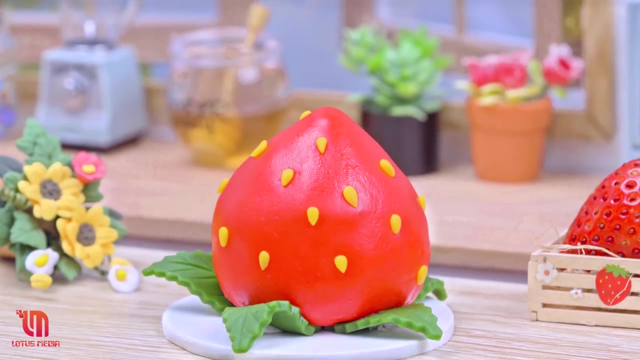 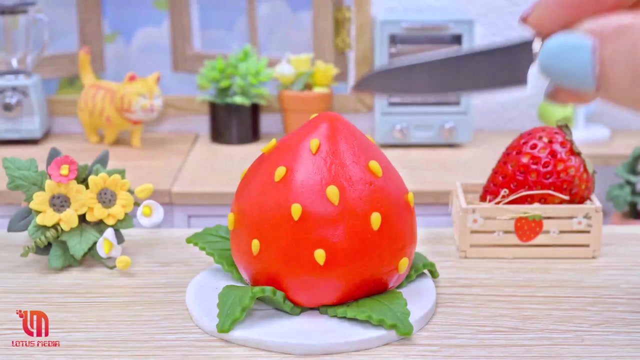 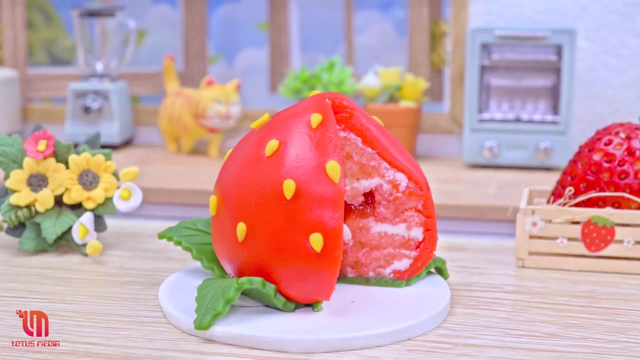 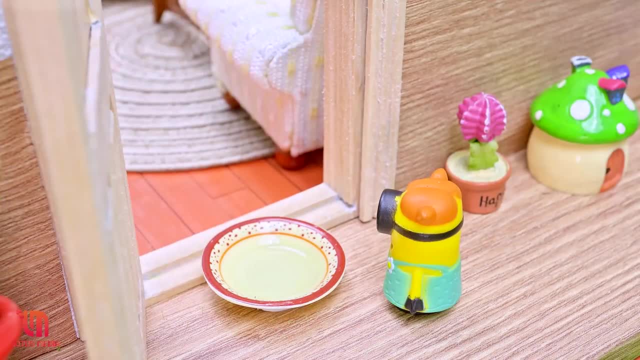 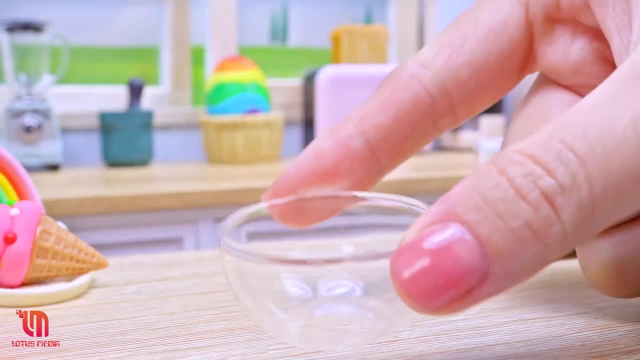 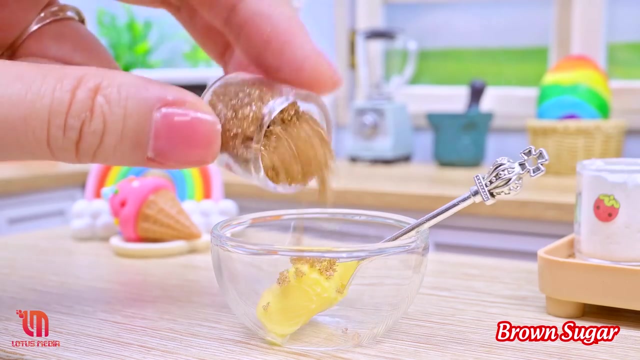 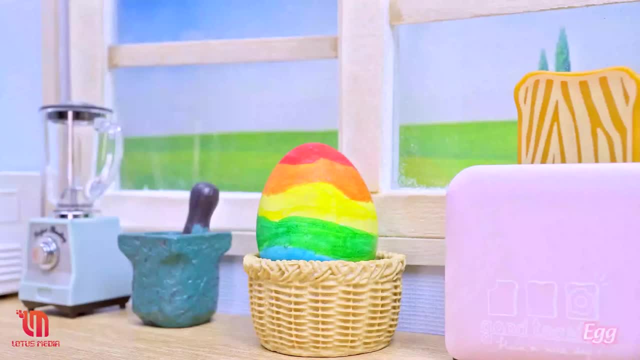 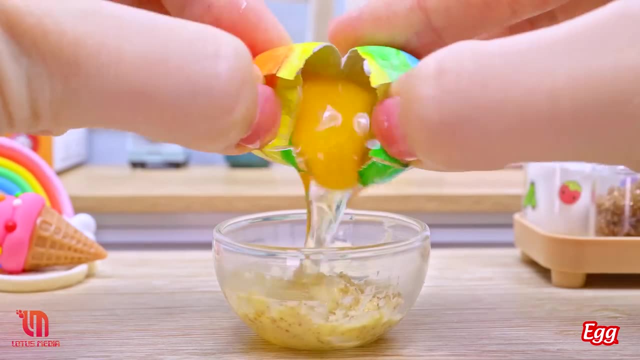 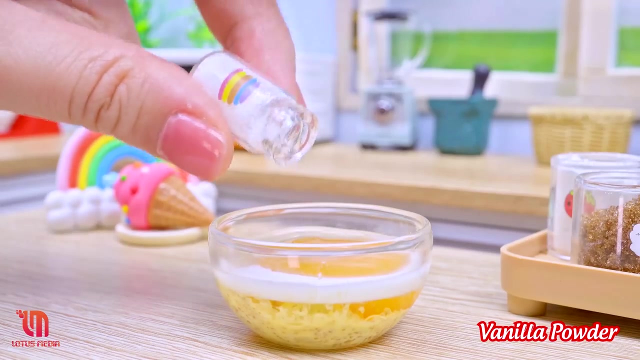 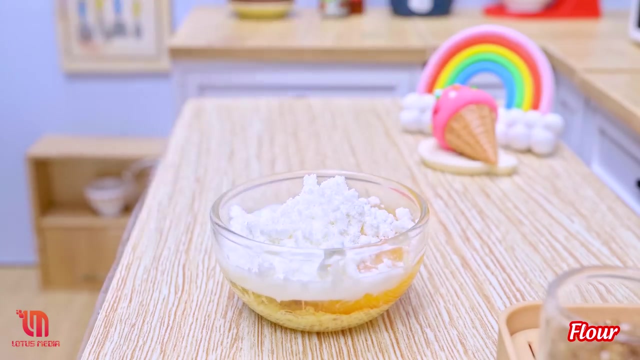 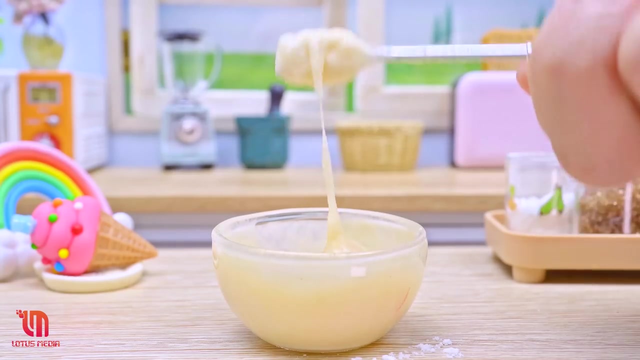 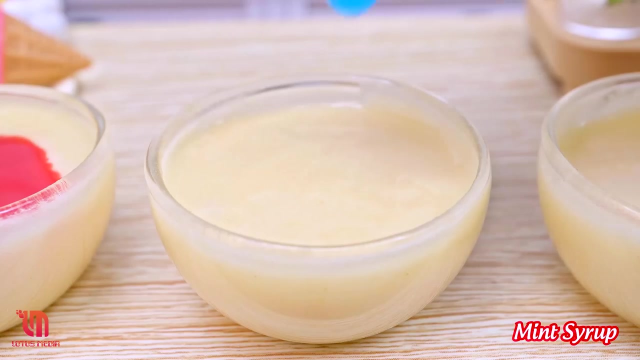 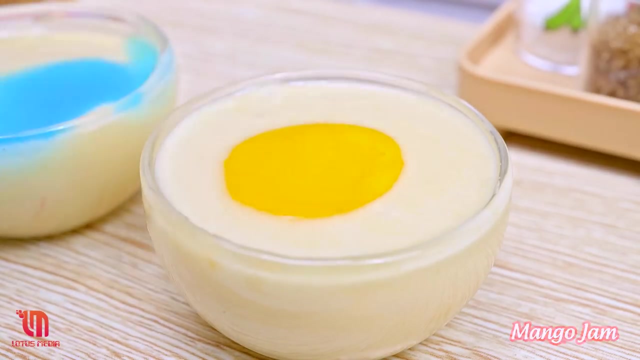 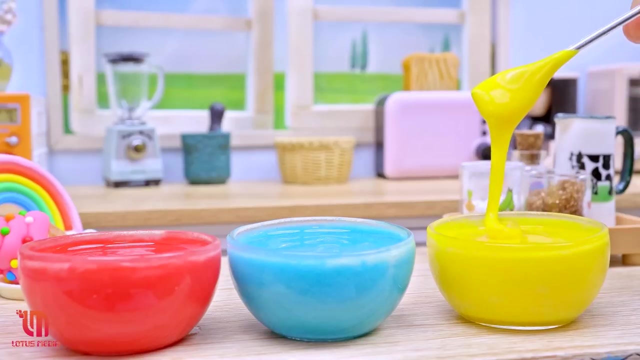 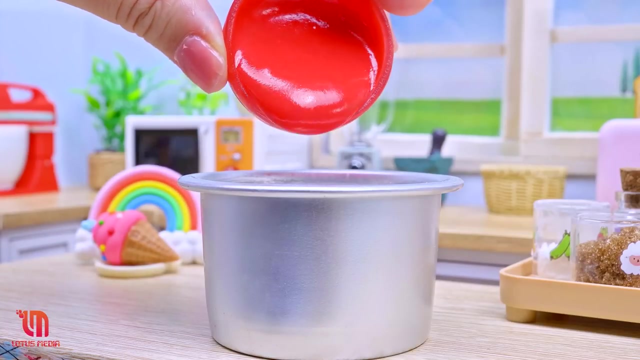 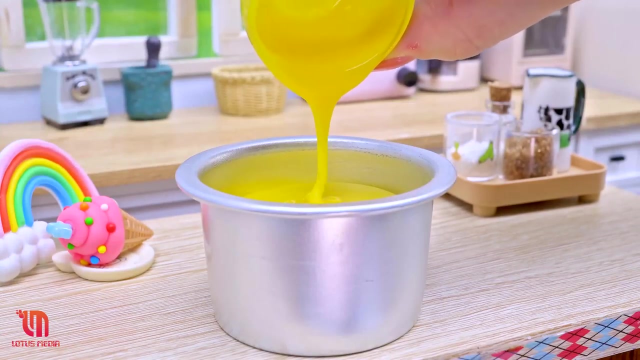 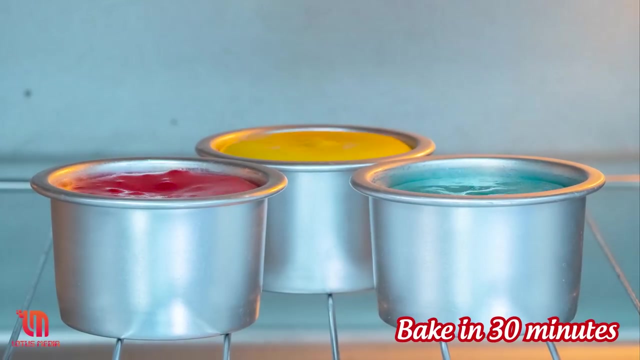 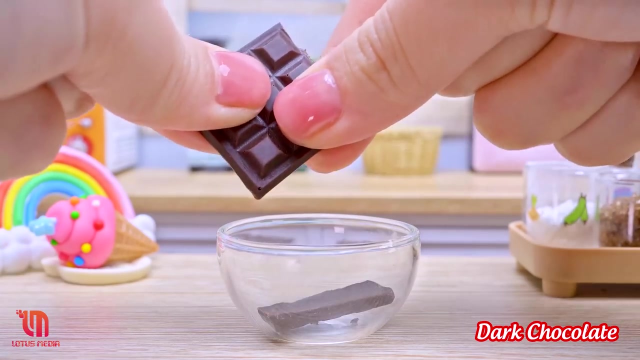 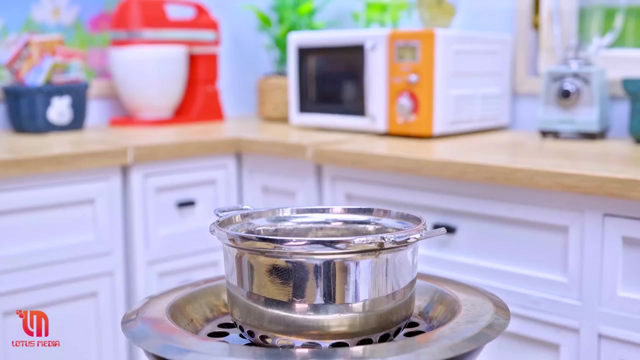 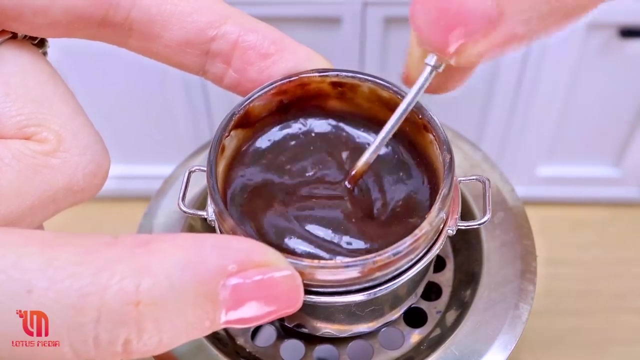 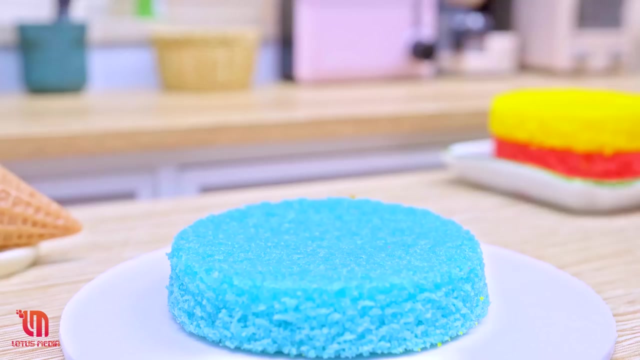 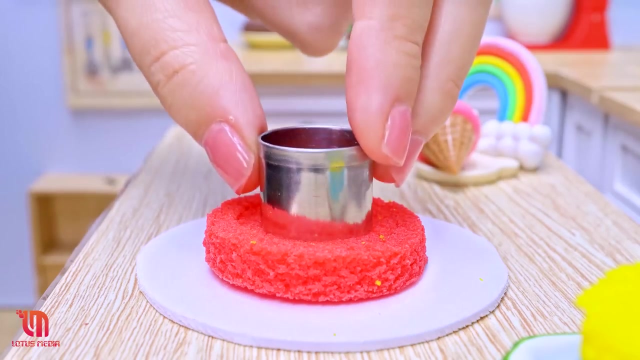 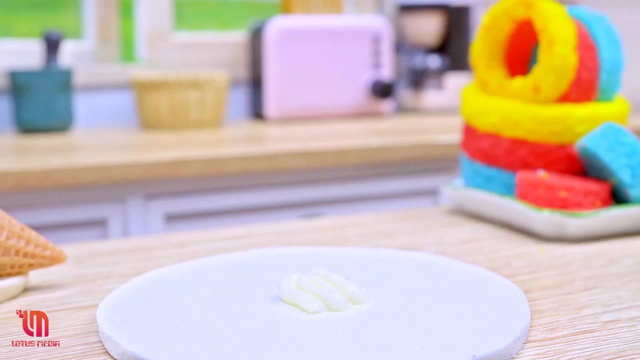 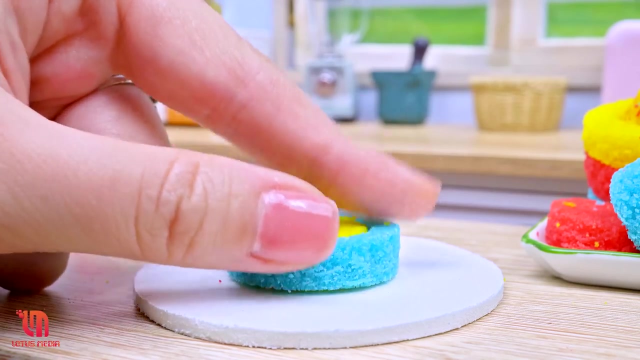 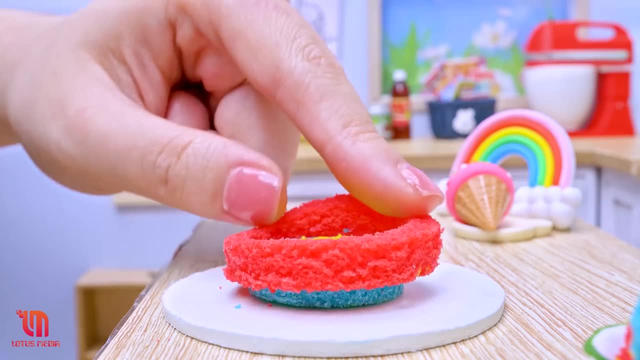 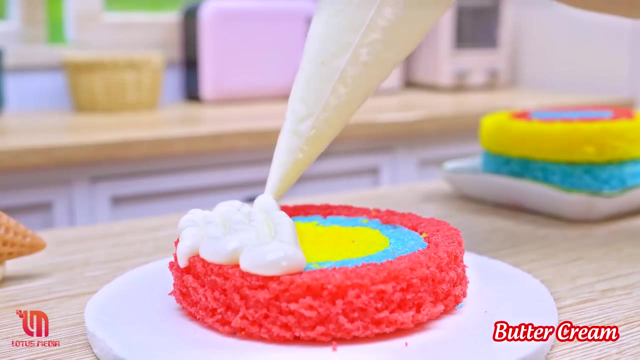 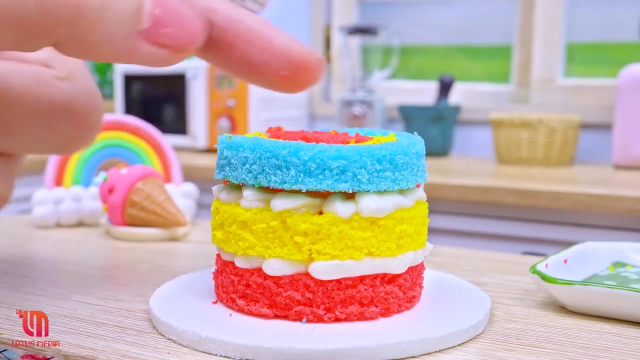 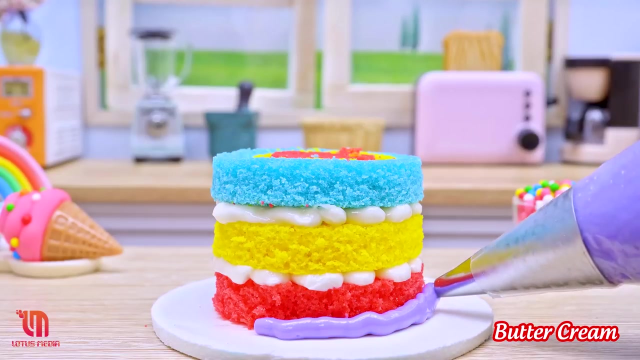 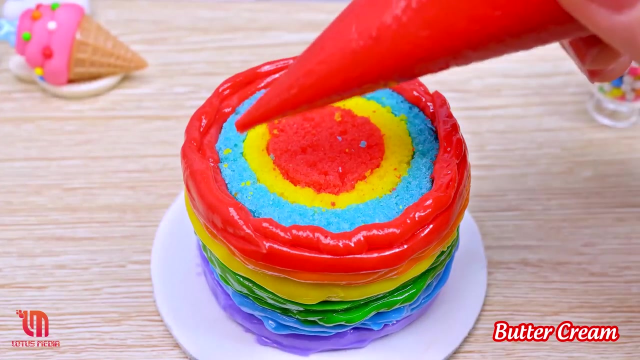 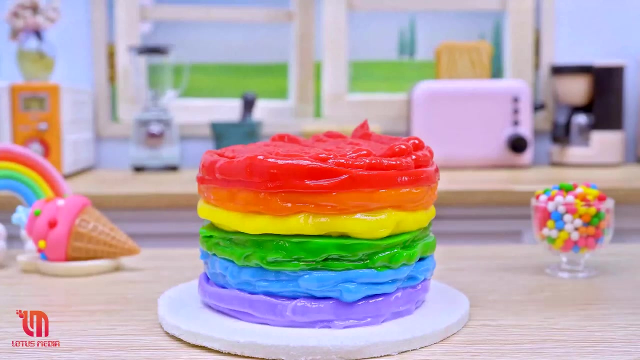 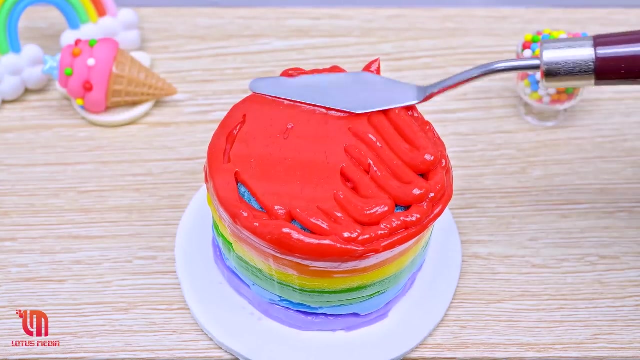 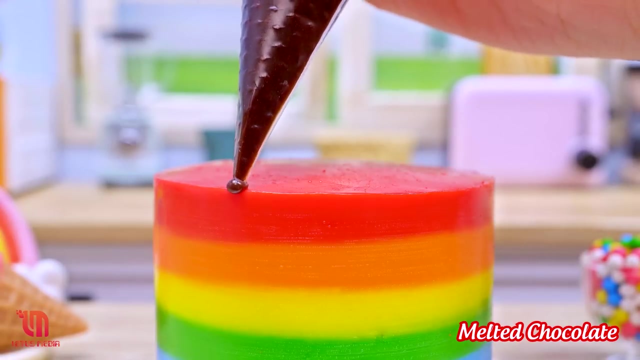 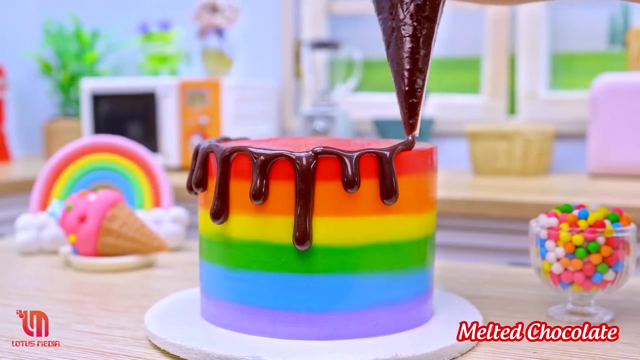 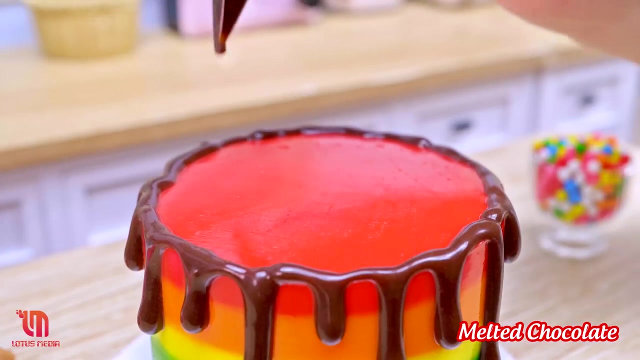 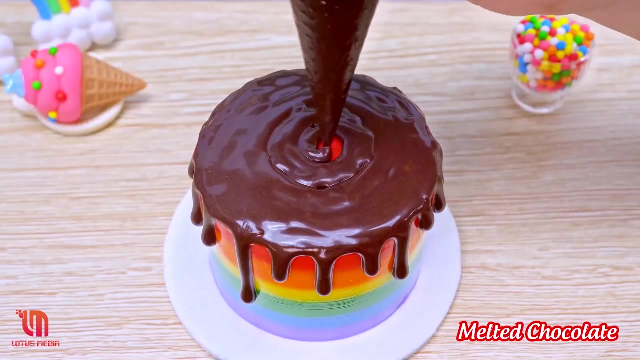 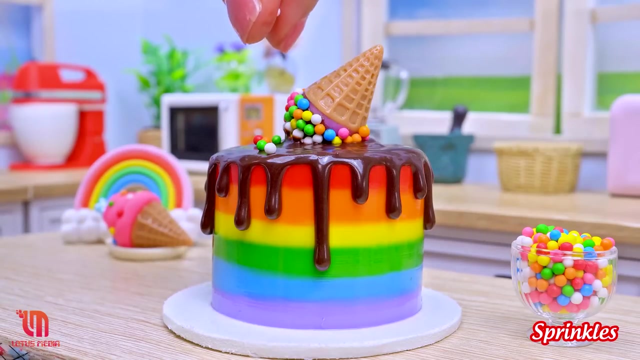 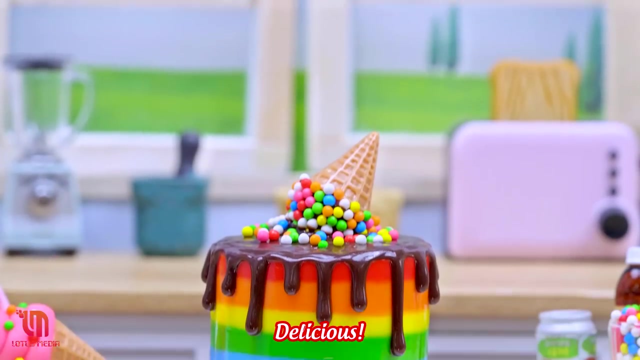 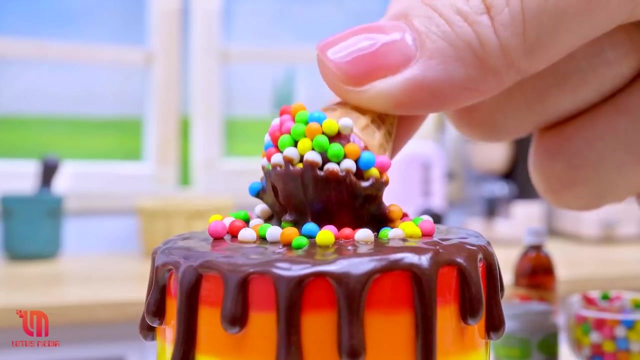 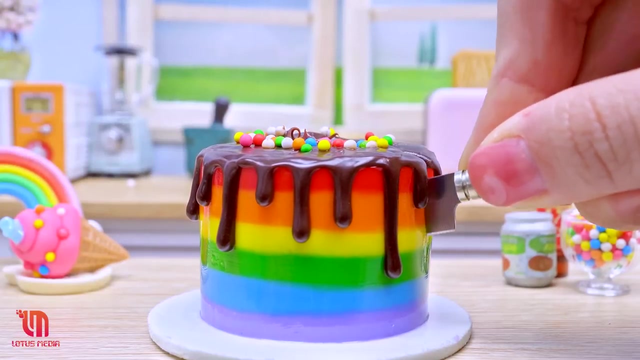 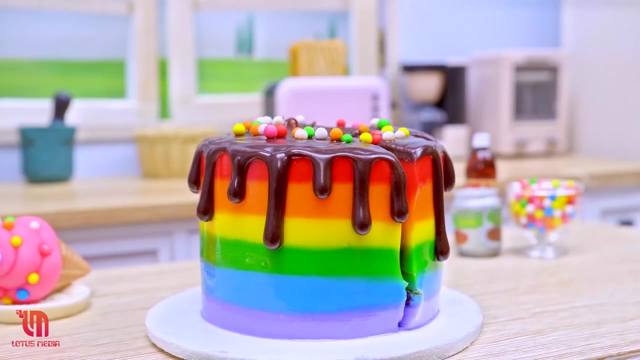 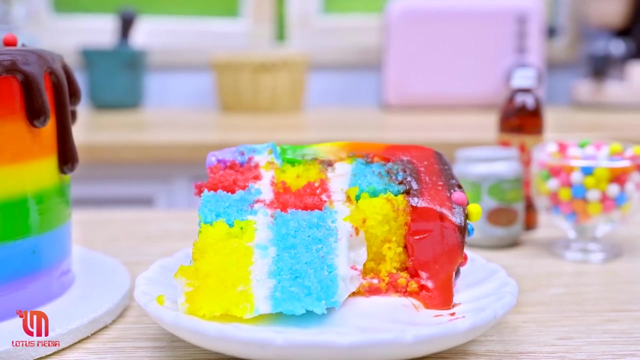 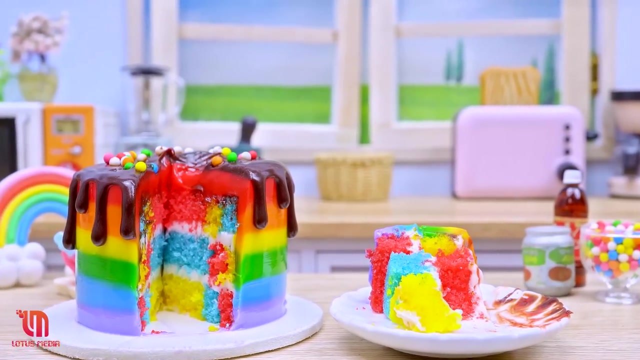 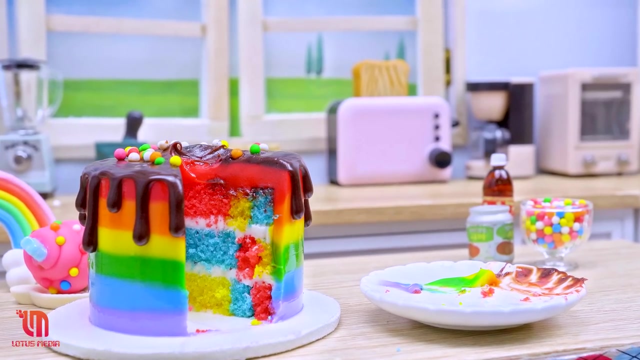 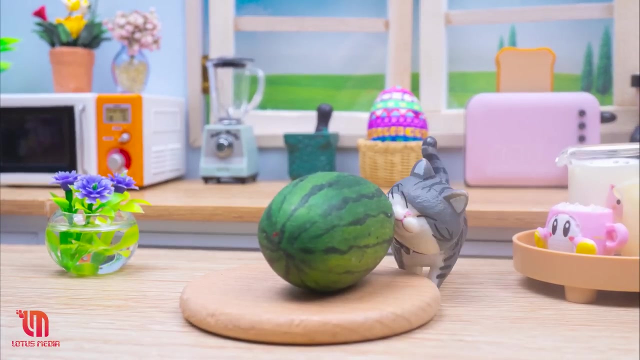 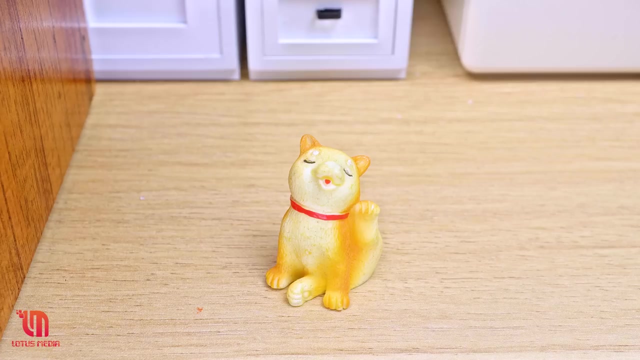 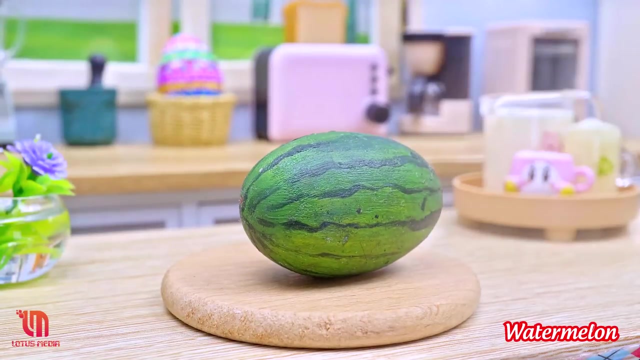 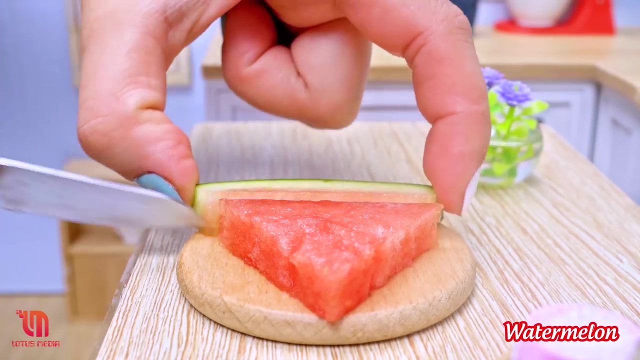 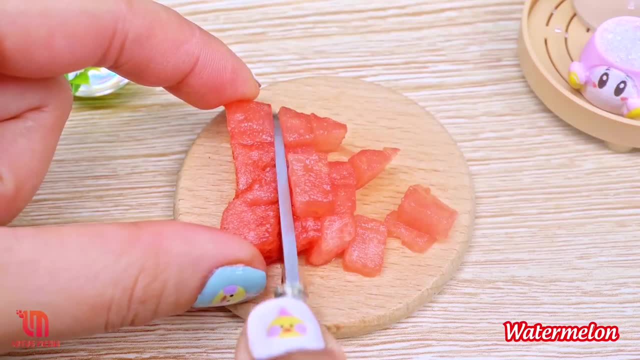 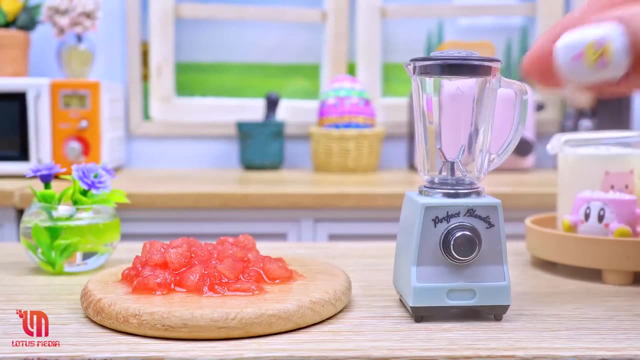 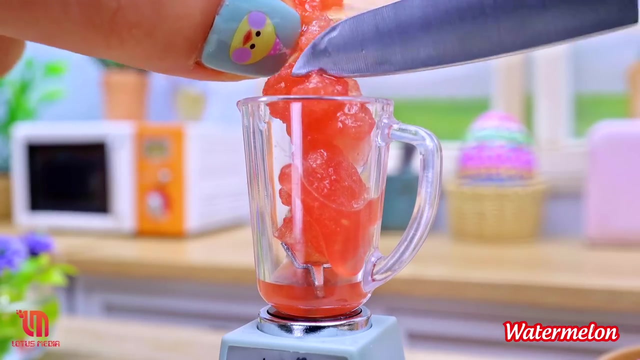 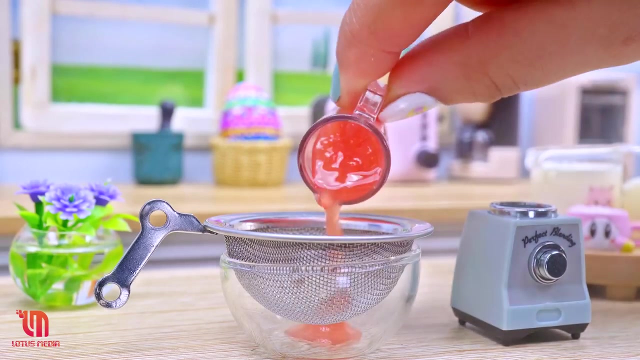 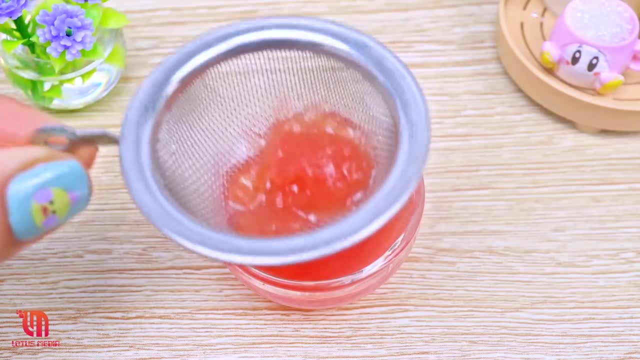 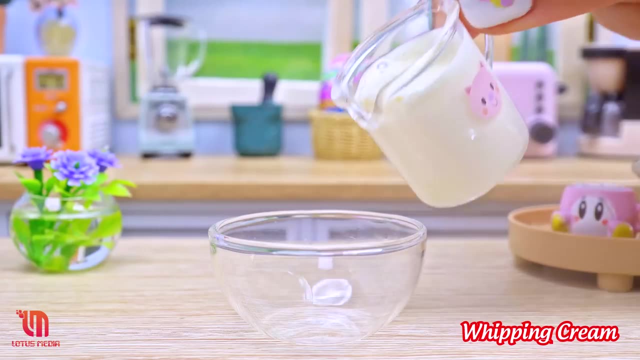 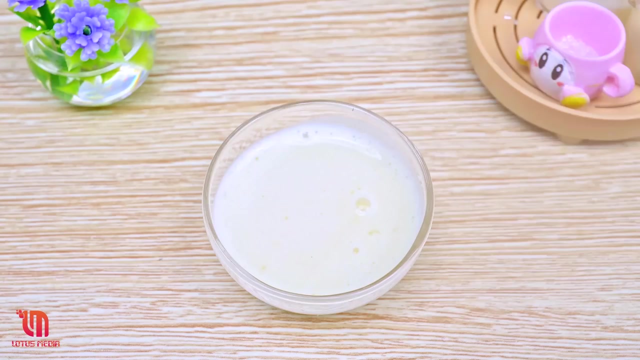 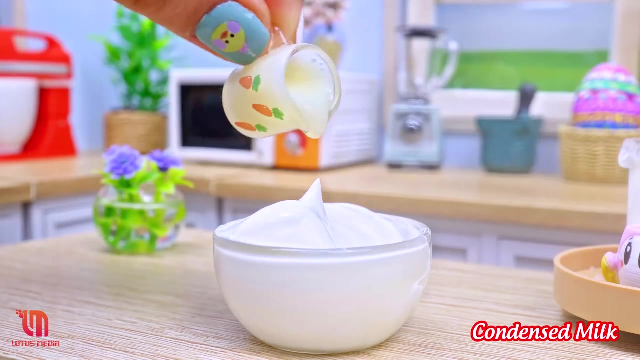 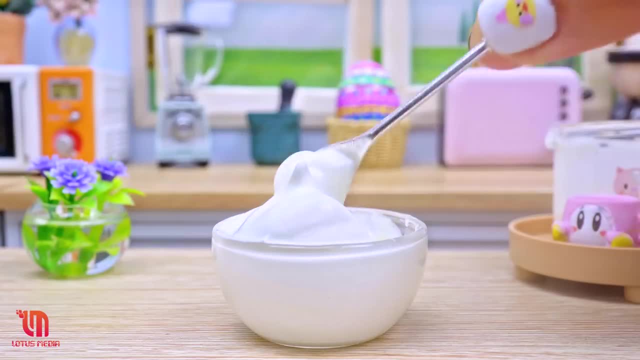 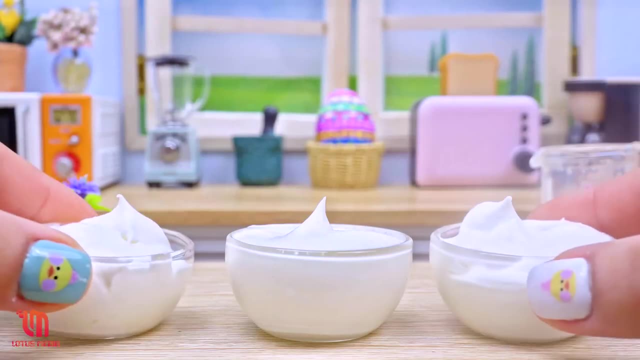 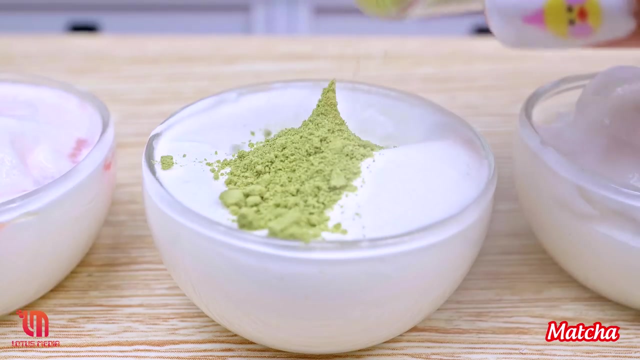 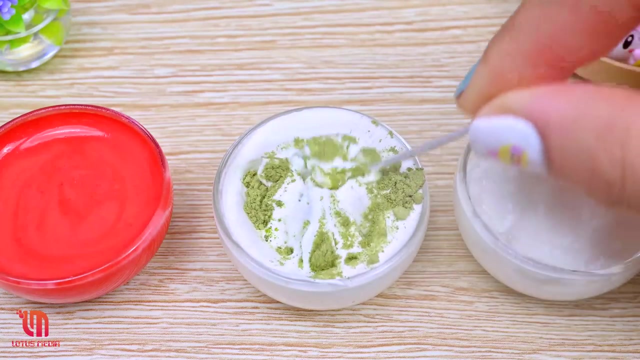 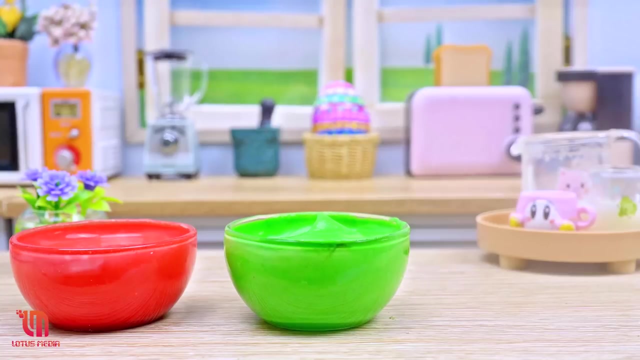 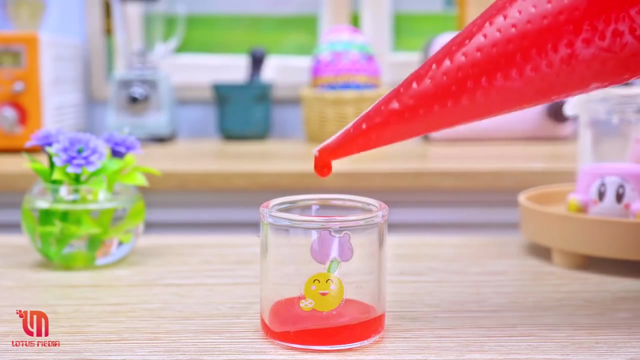 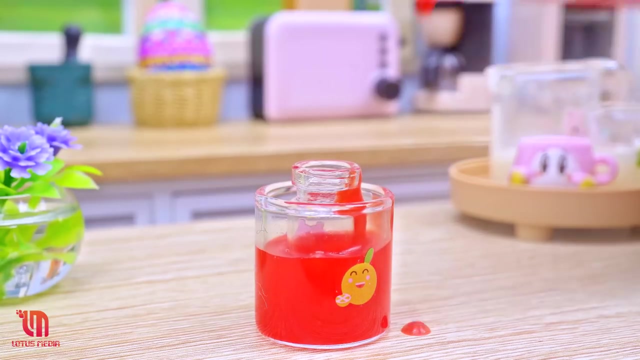 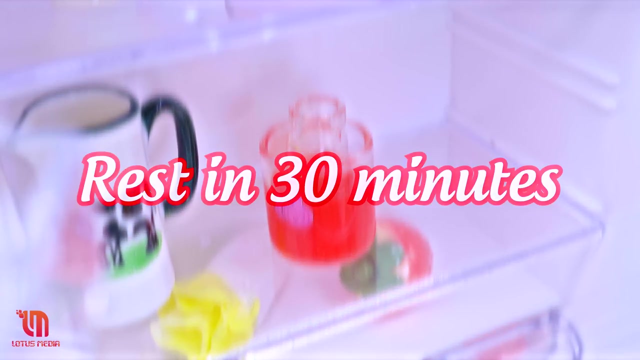 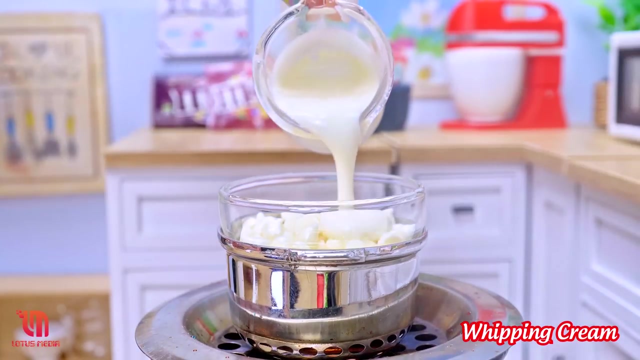 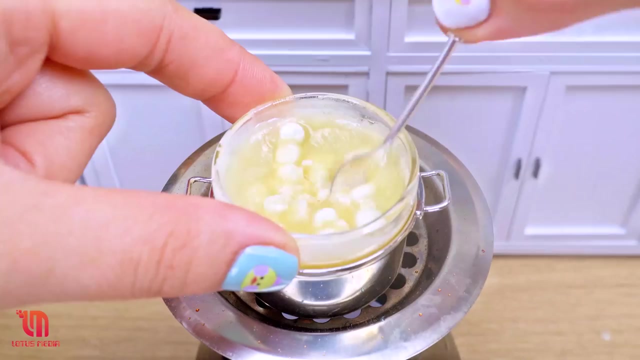 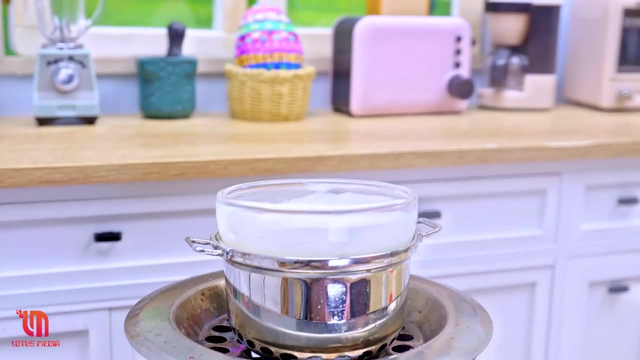 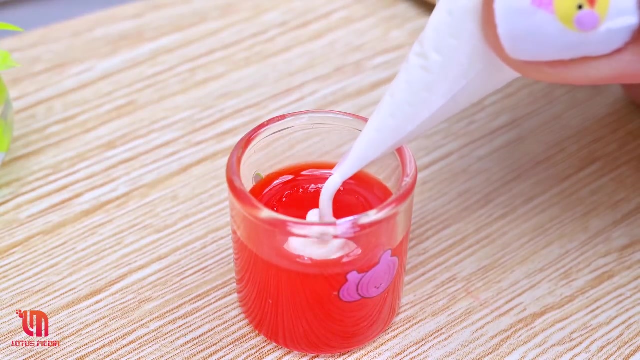 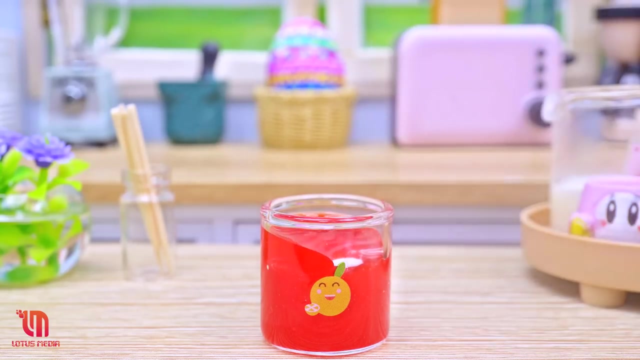 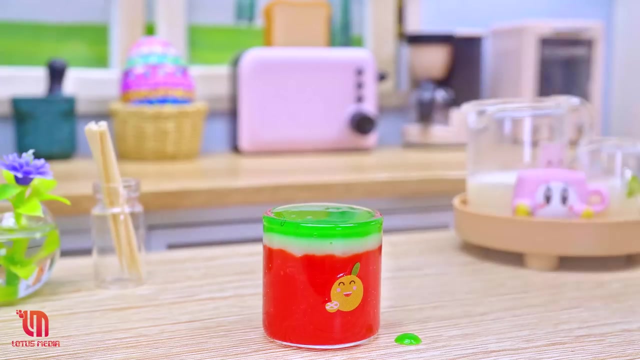 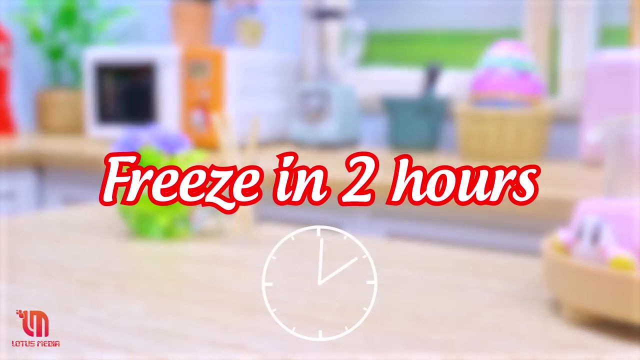 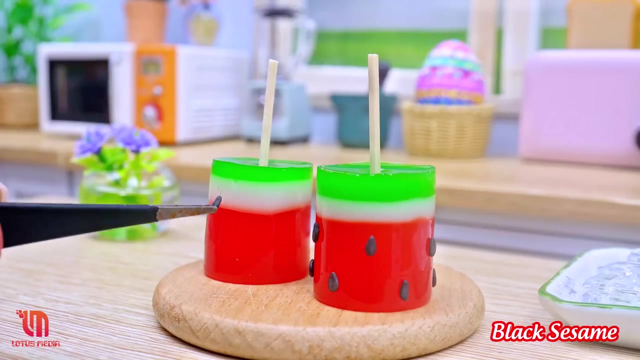 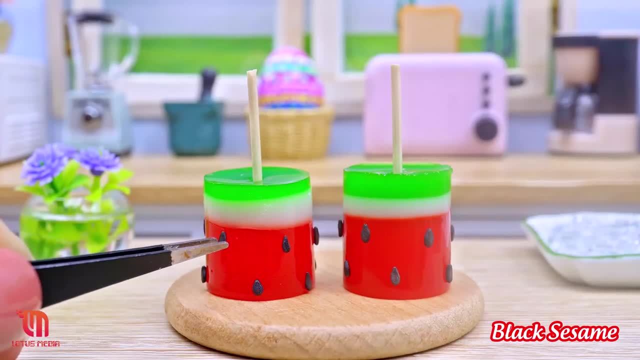 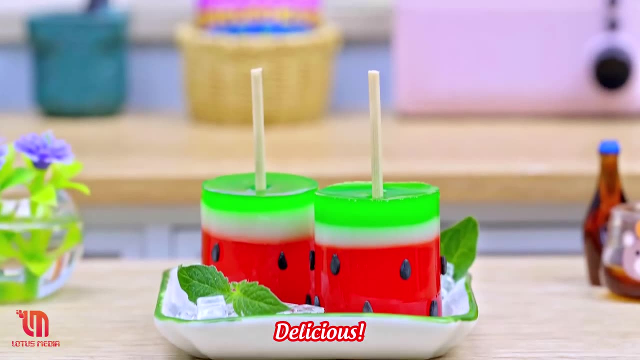 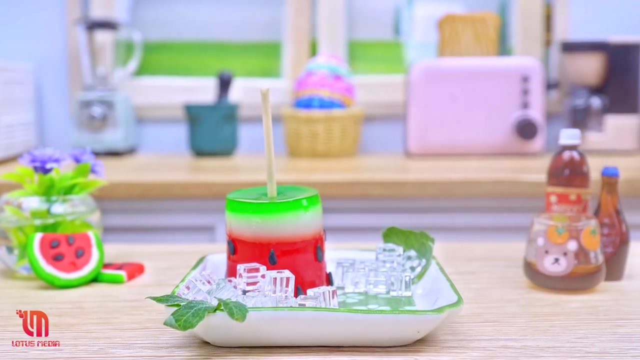 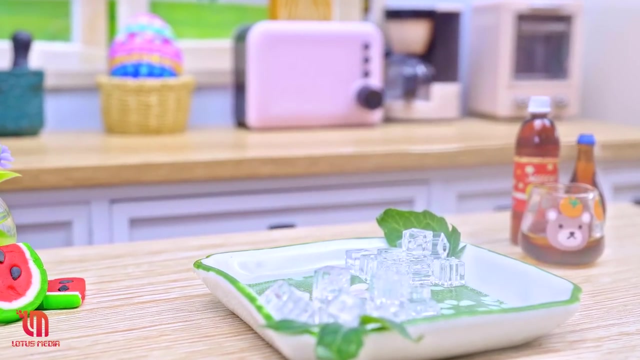 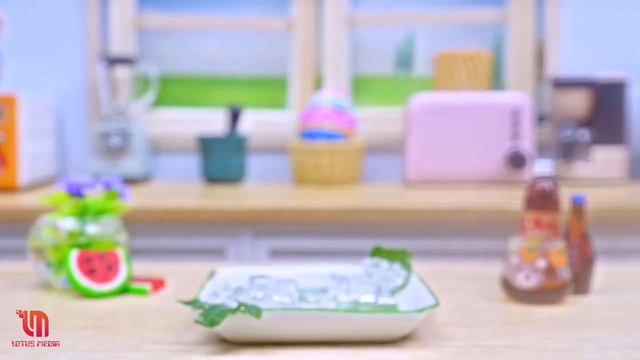 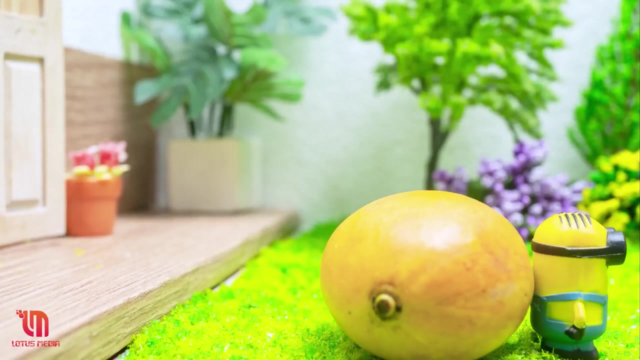 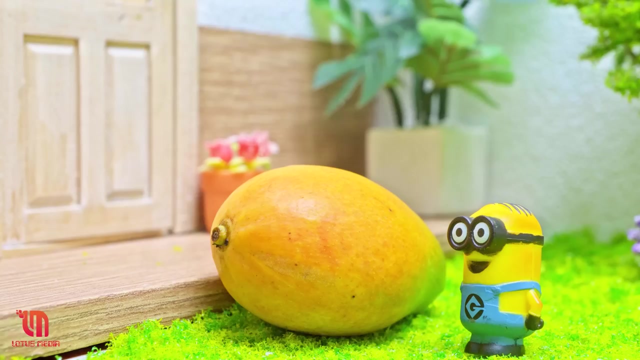 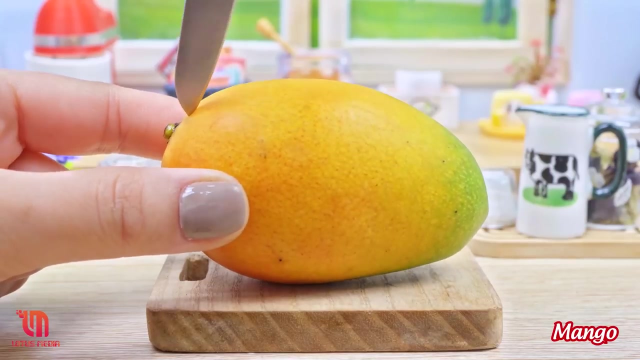 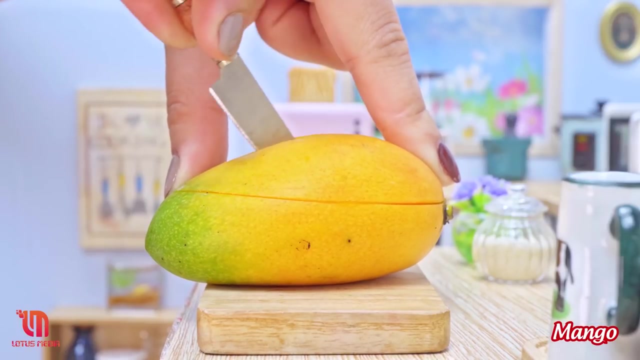 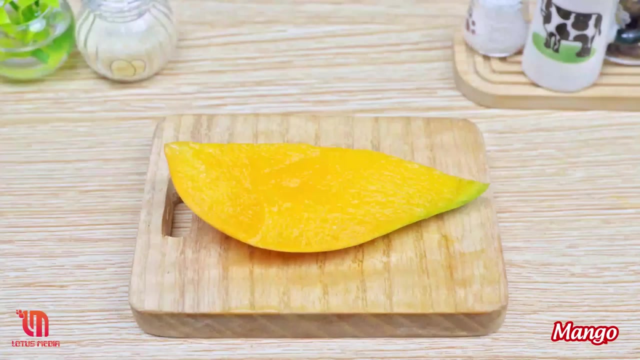 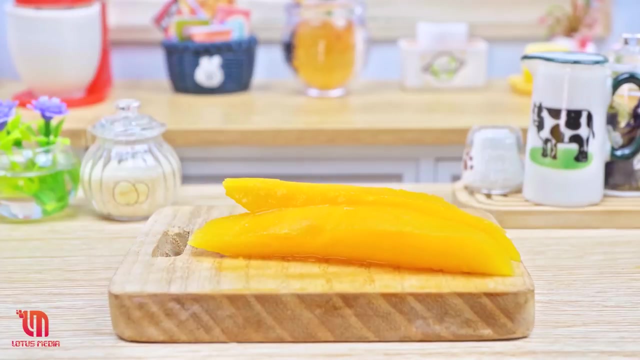 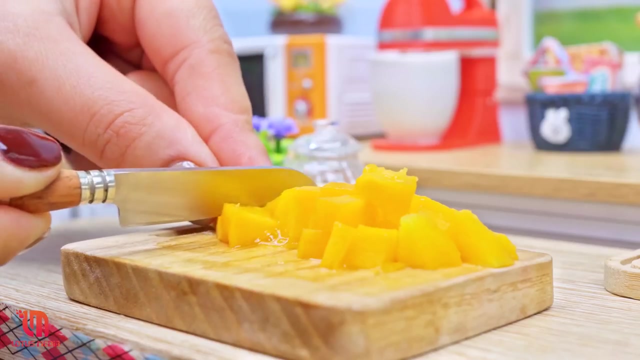 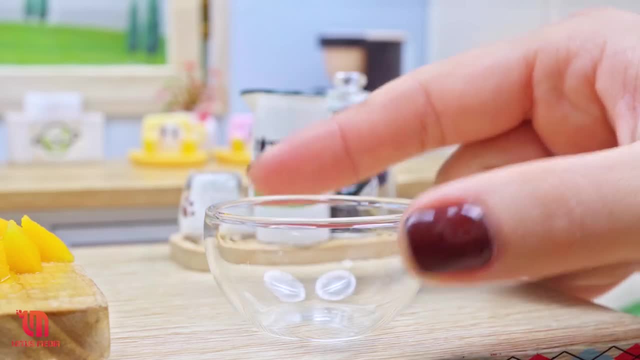 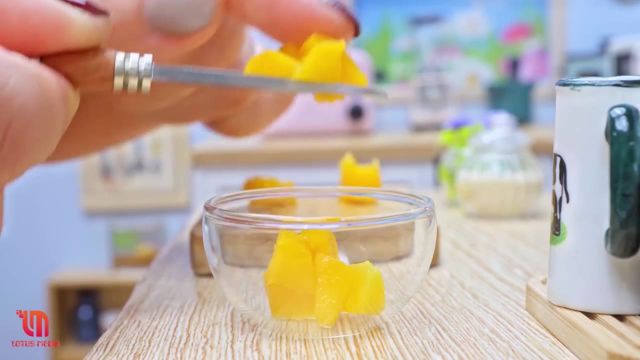 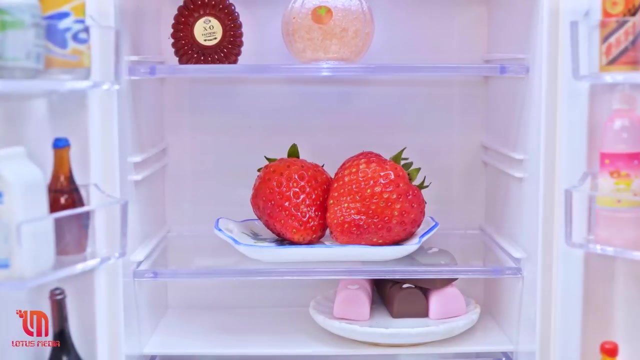 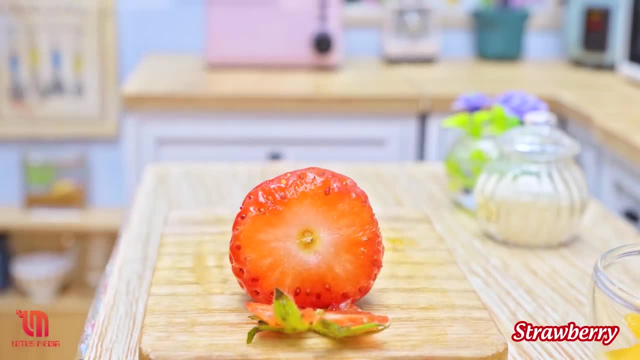 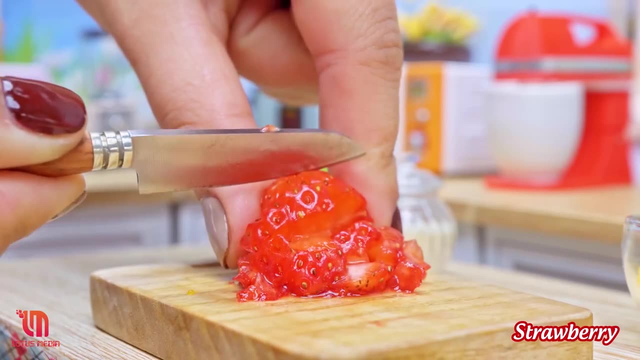 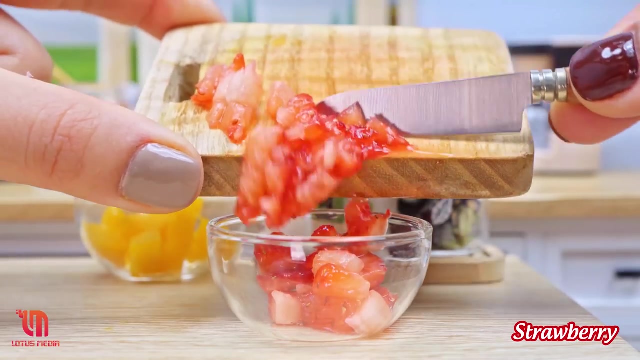 Oh, can I help you? Oh, can I help you? Oh, can I help you? Oh, Oh, I haven't seen you. You have my bulk requests, but You have my bulk requests, but You have my bulk requests, but. 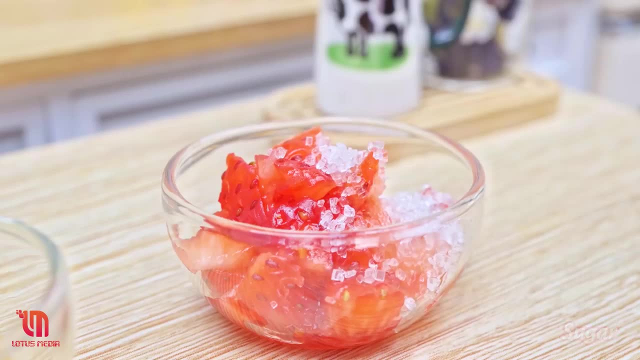 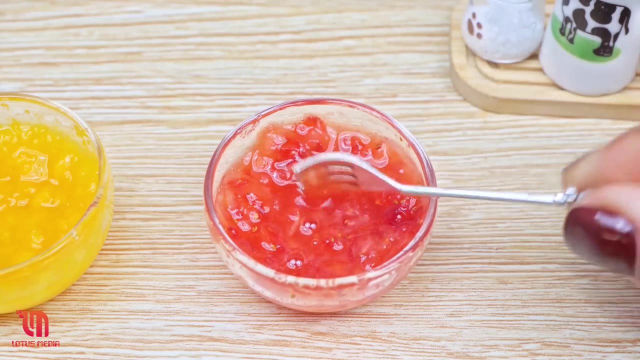 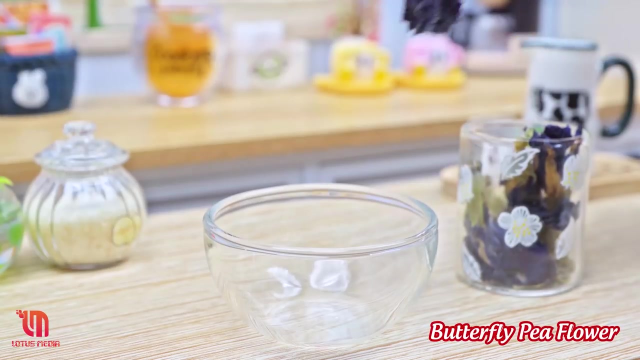 Heat it up in the microwave. Add 100ml of water. Add the egg. Add 1 cup of water. Add 1 tablespoon of salt. Add 1 tablespoon of sugar. Add 1 tablespoon of vinegar. Add 2 tablespoons of beer. 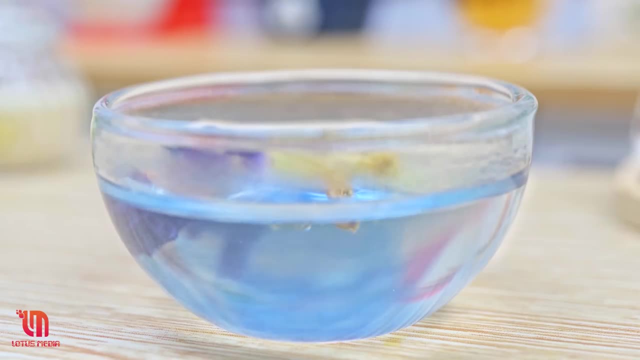 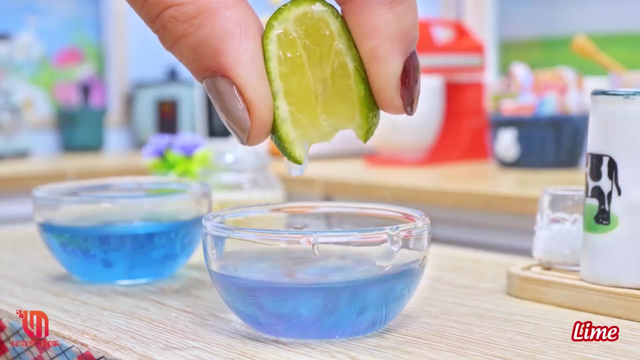 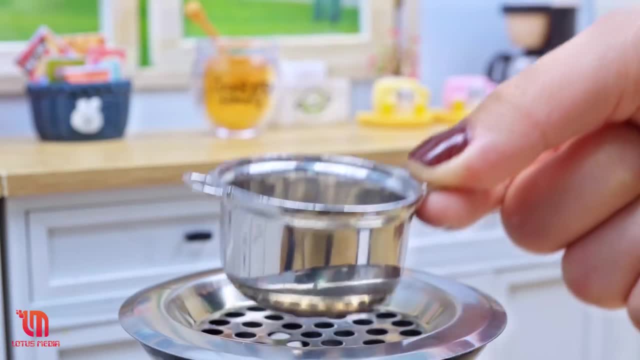 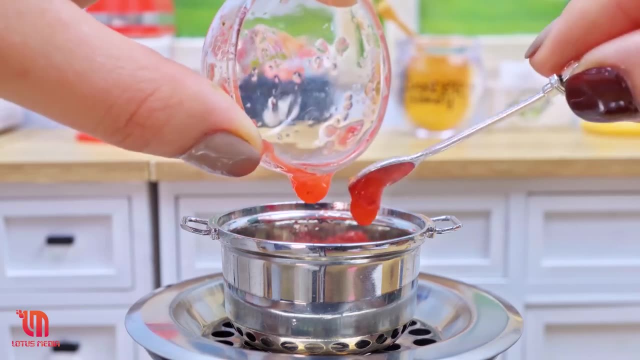 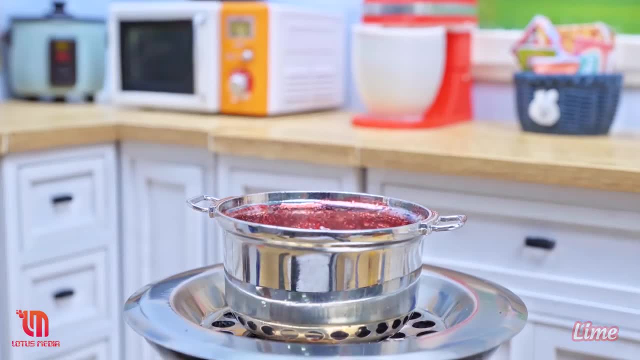 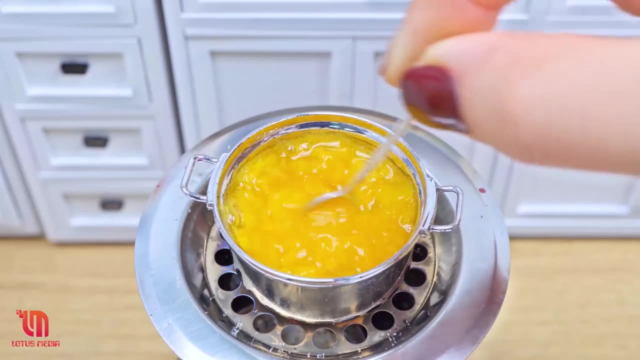 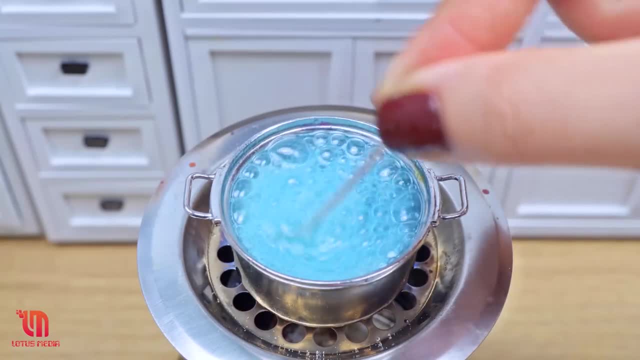 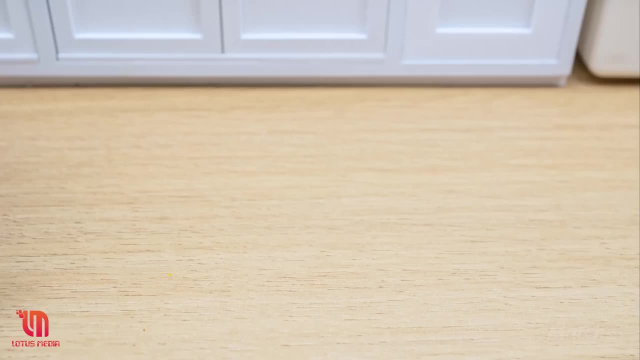 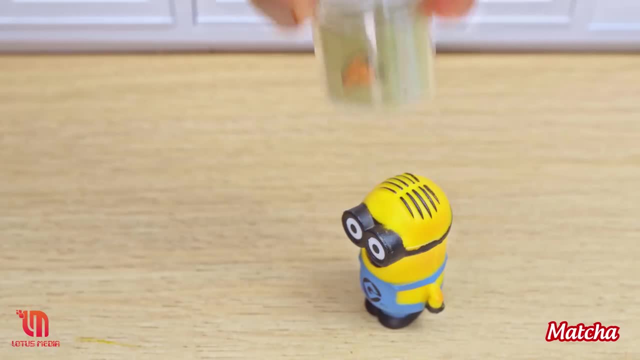 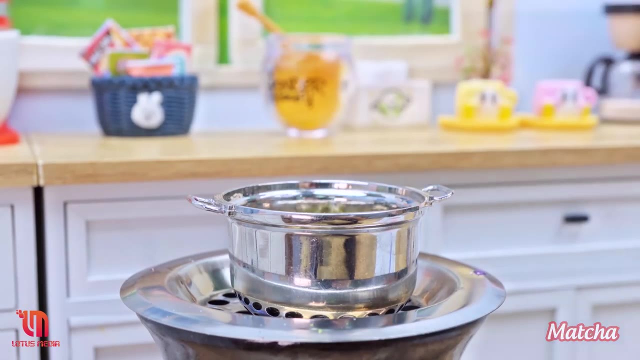 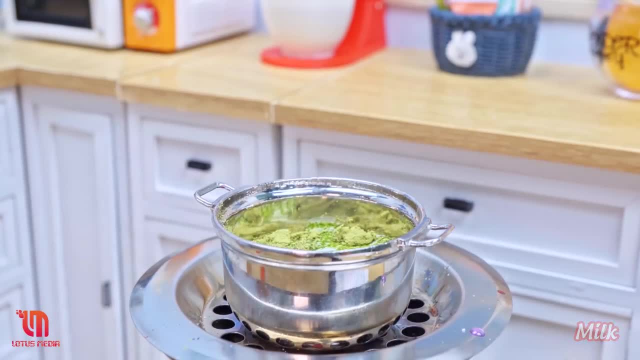 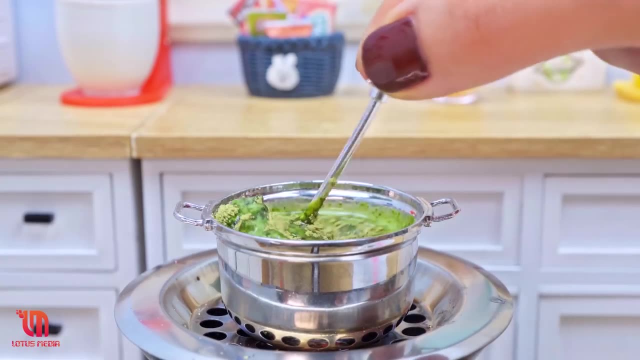 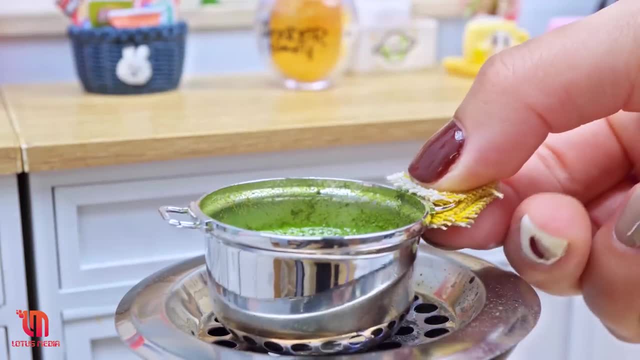 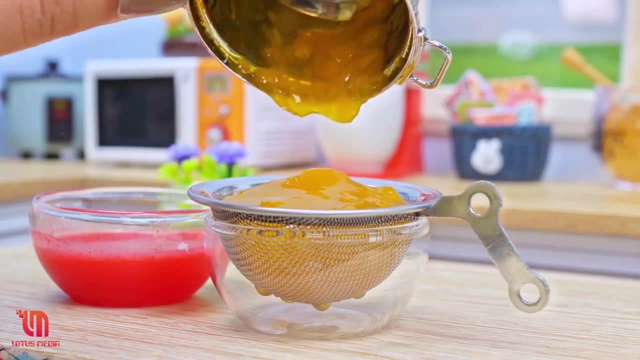 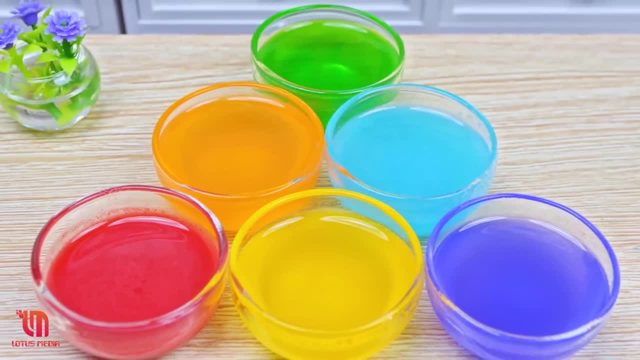 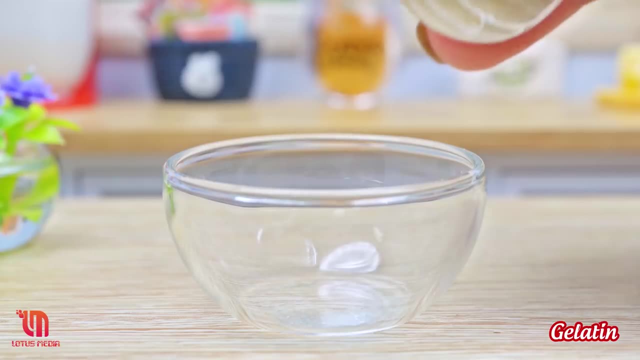 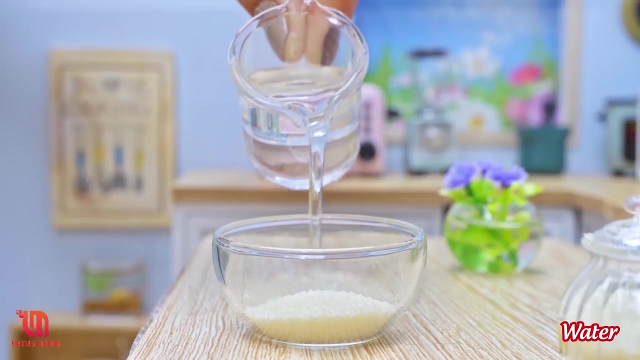 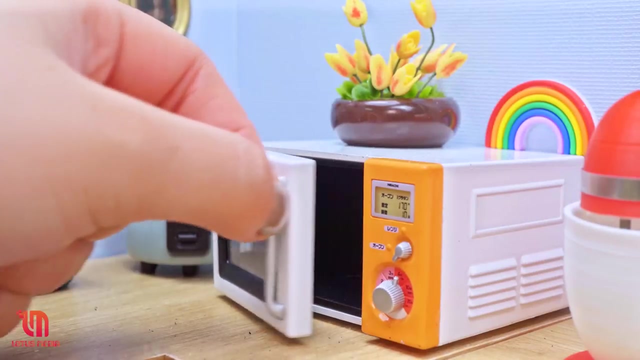 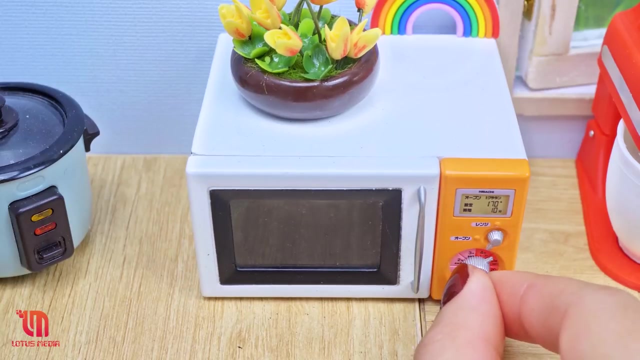 I'm going to drink a cup of water. I'm going to drink a cup of water. hope you enjoyed the video. if you did, please add a like and subscribe to the channel. Now let's prepare the sauce: 1 Tbsp Soy. 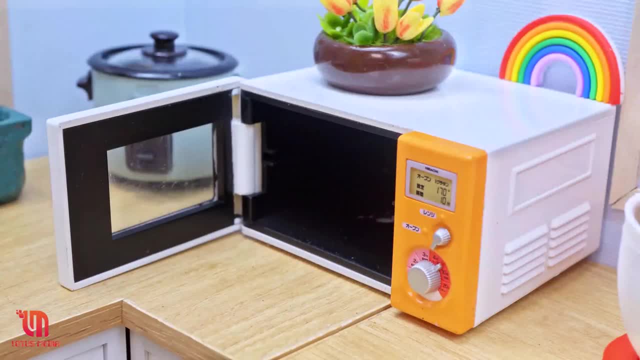 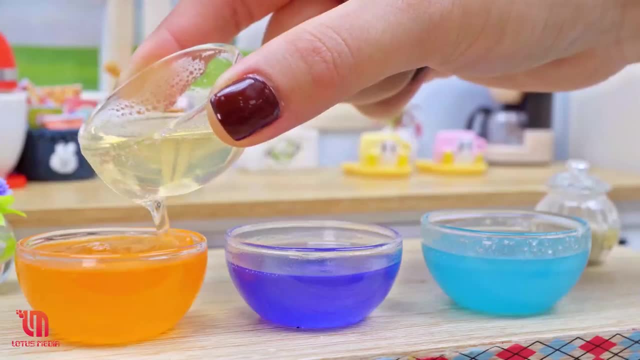 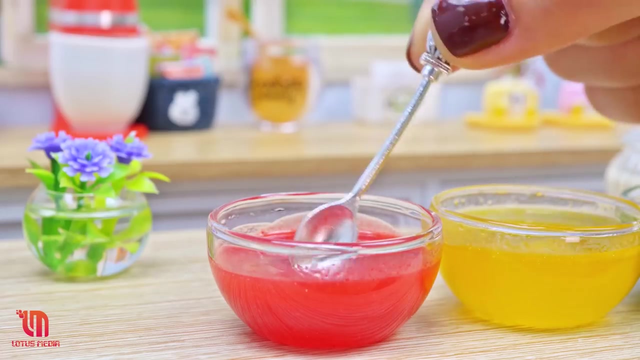 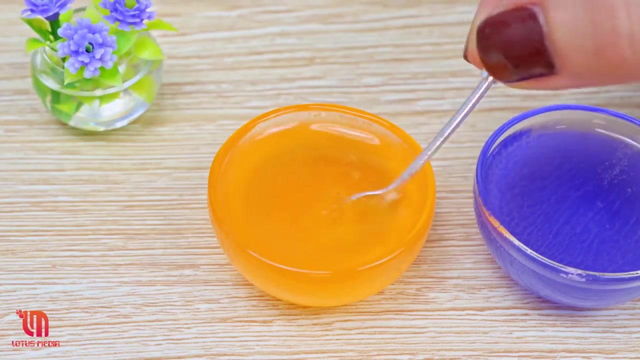 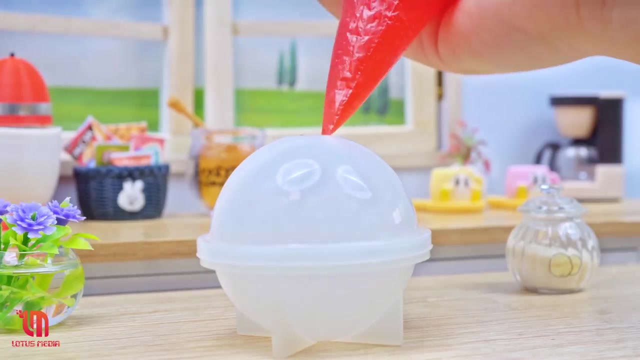 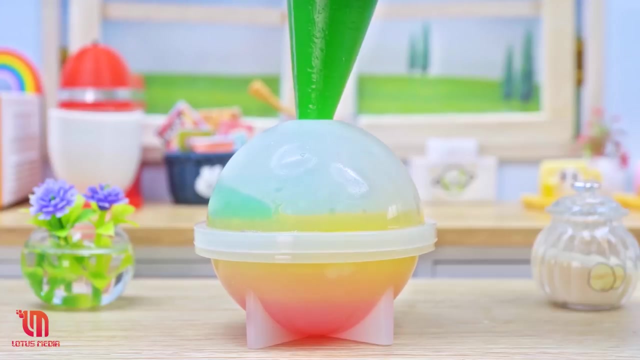 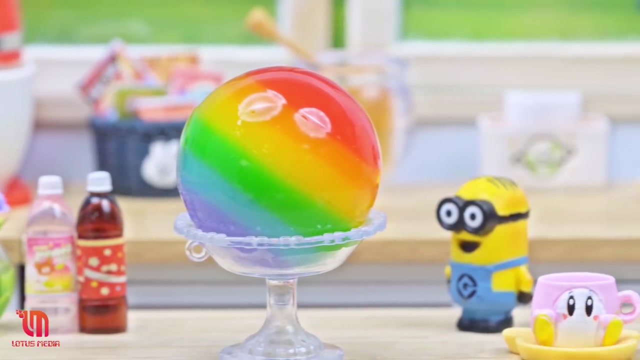 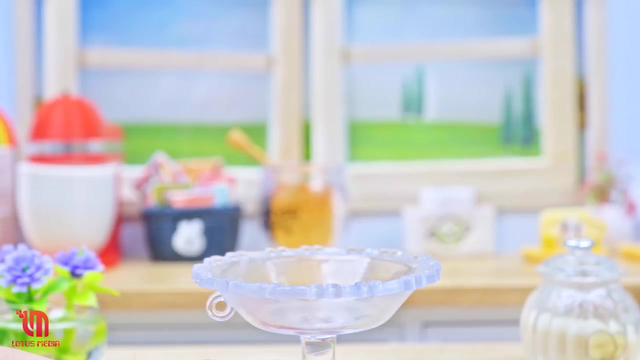 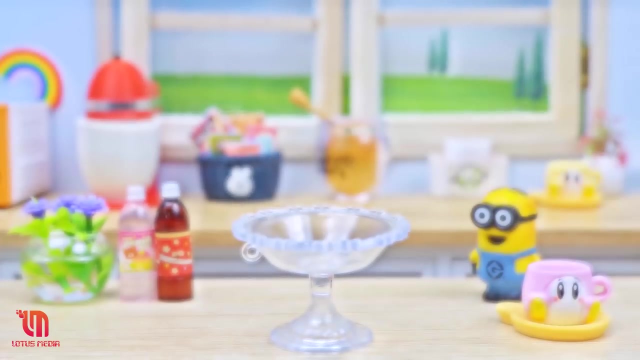 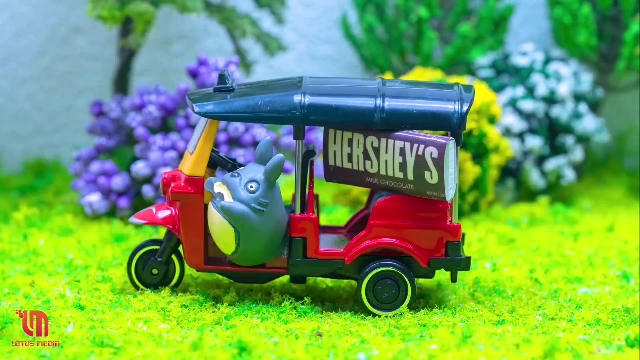 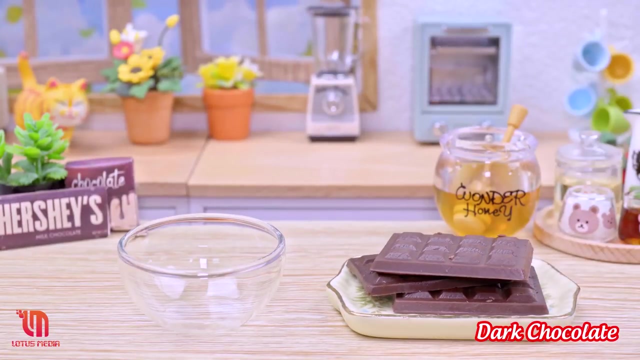 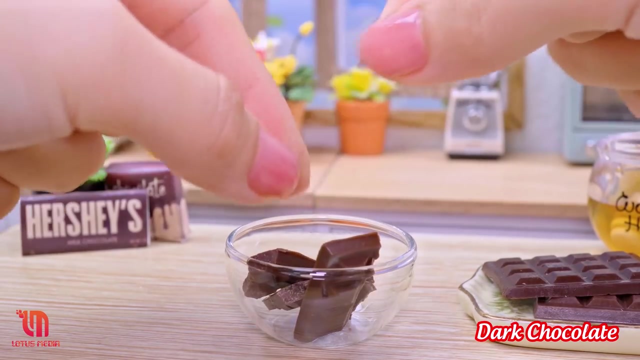 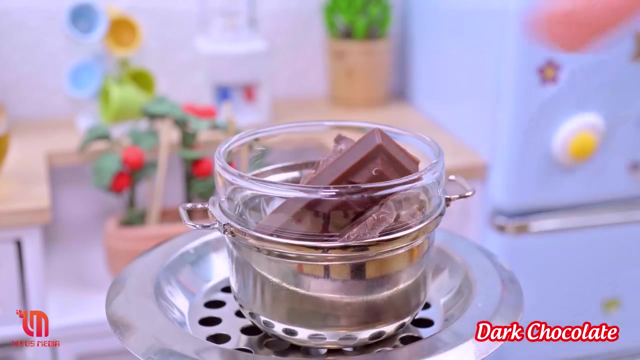 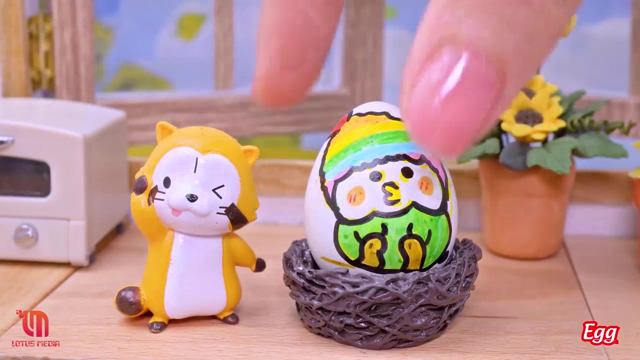 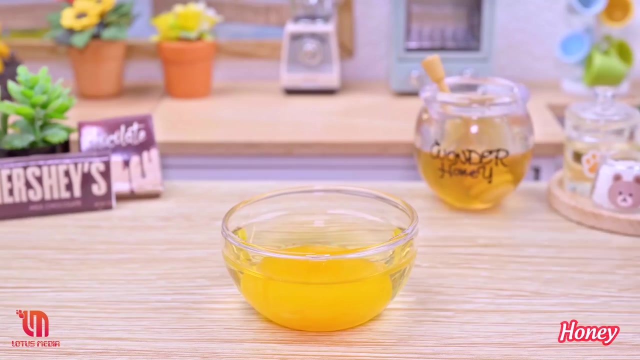 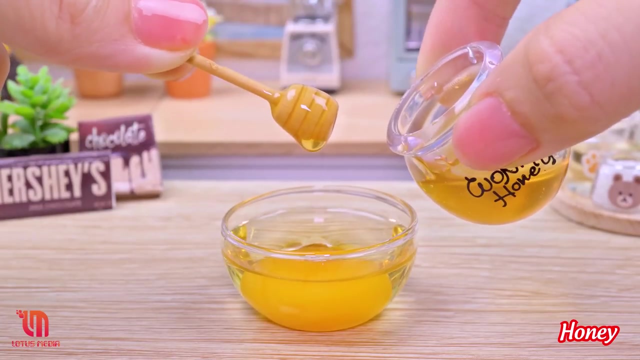 2 tablespoons of cold water, 2 tablespoons of water, 1 tablespoon of salt, 2 tablespoons of starch syrup, 1 tablespoon of cooking wine. Mix it well, Wow, I love it. Delicious, Tasty, Wow, Yummy, I love it. 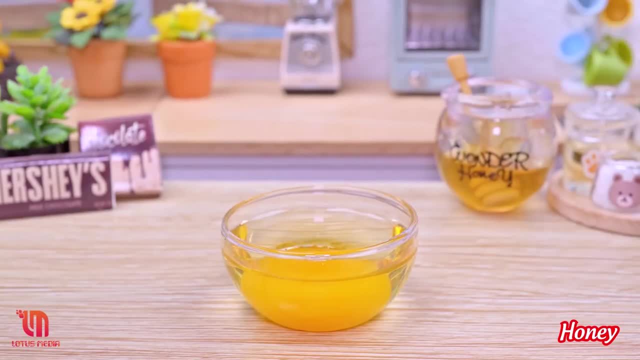 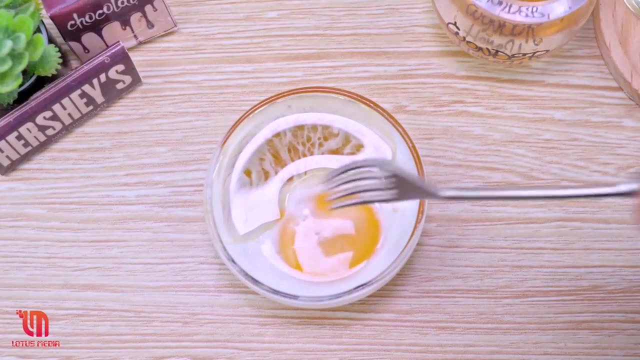 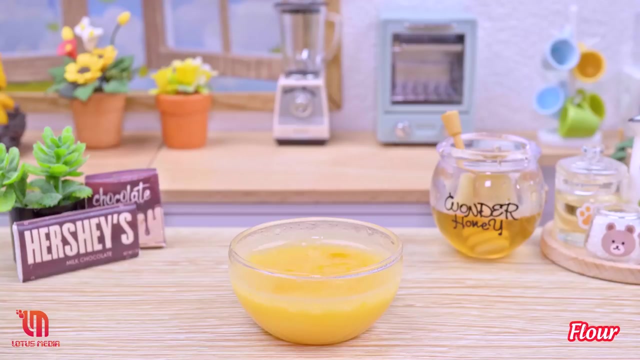 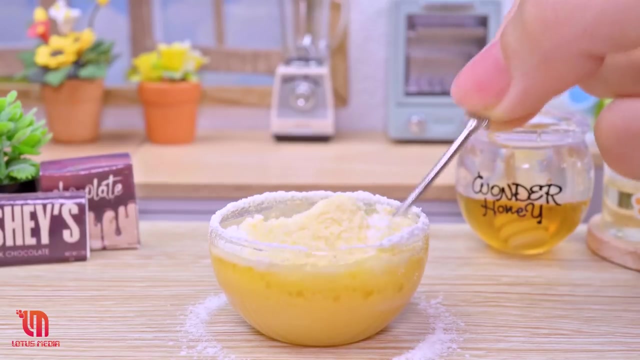 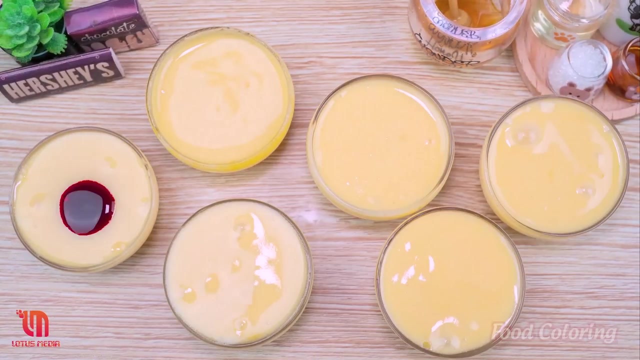 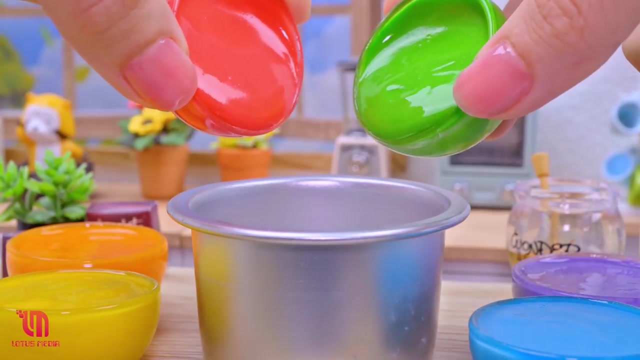 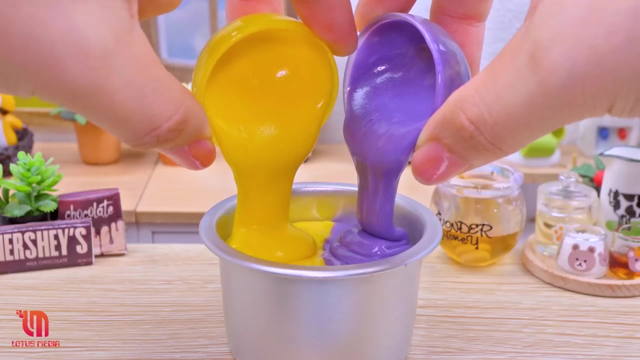 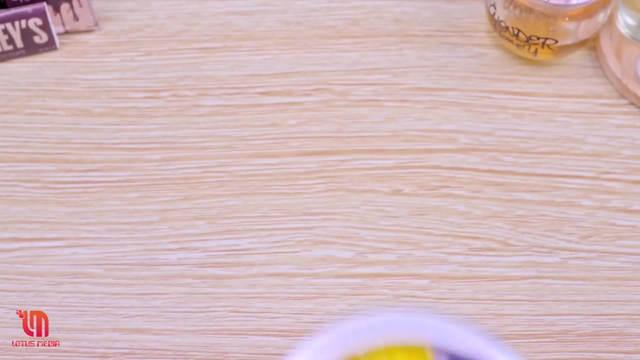 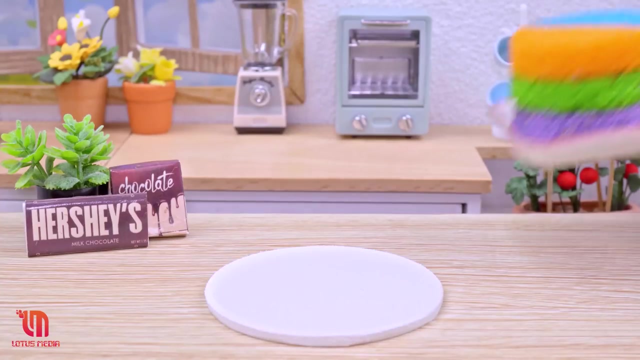 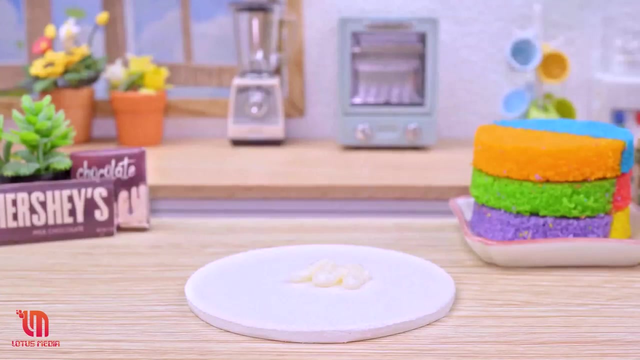 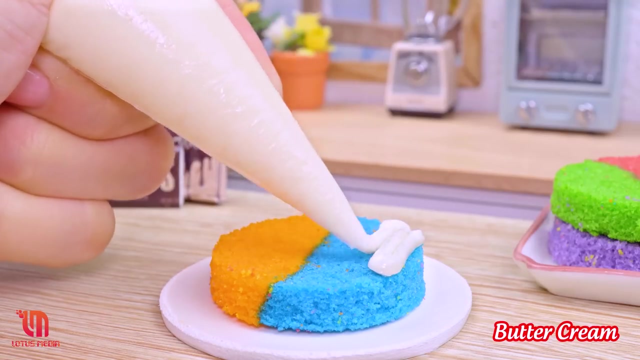 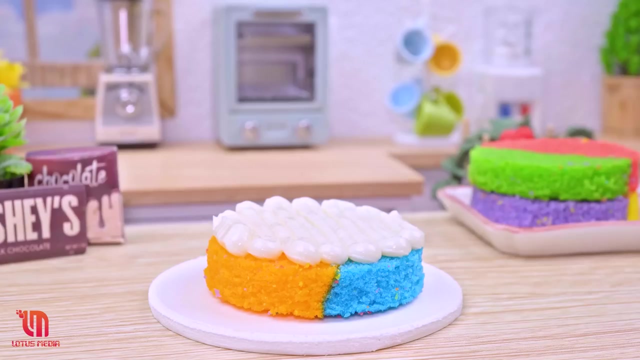 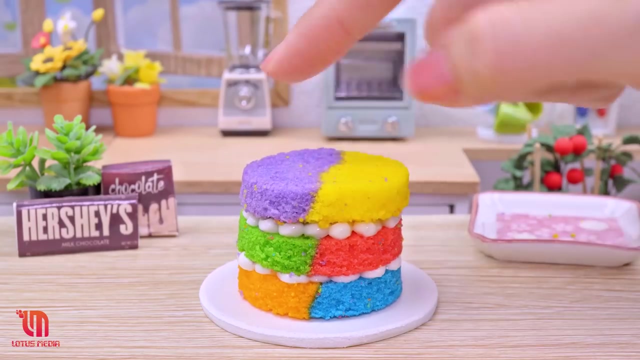 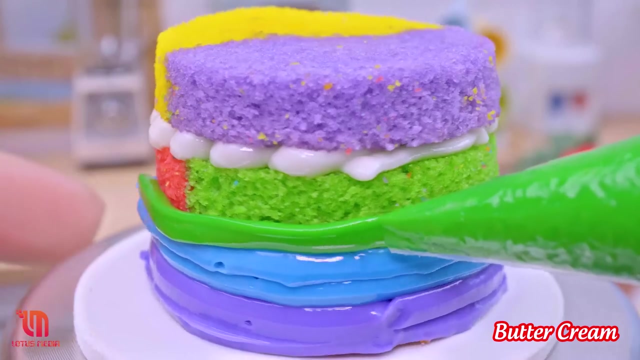 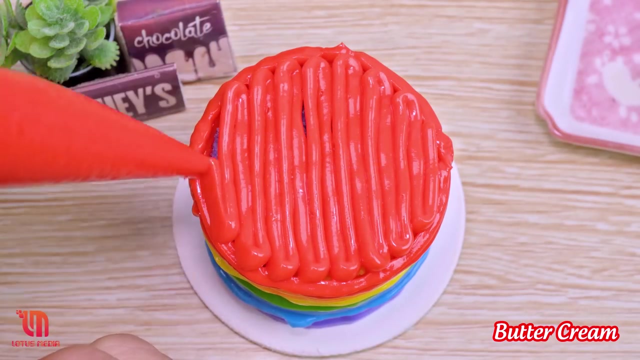 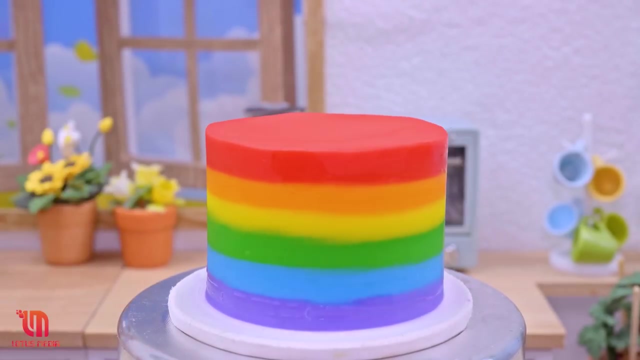 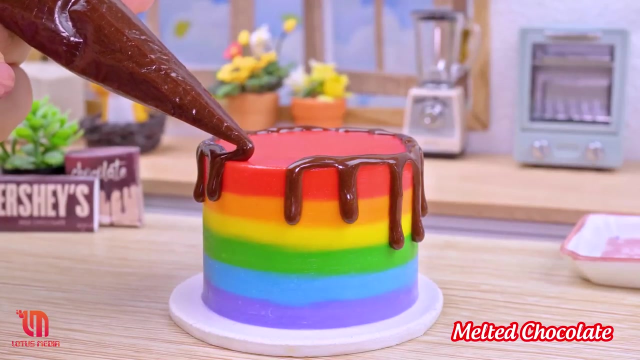 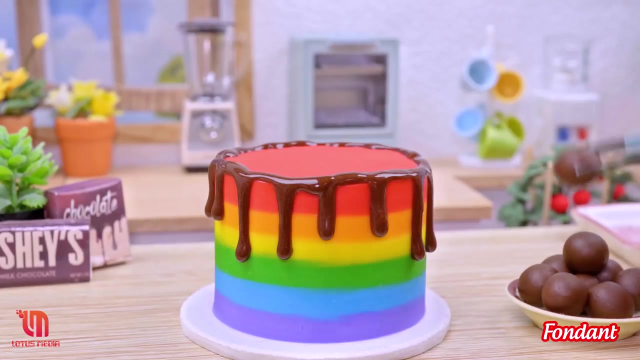 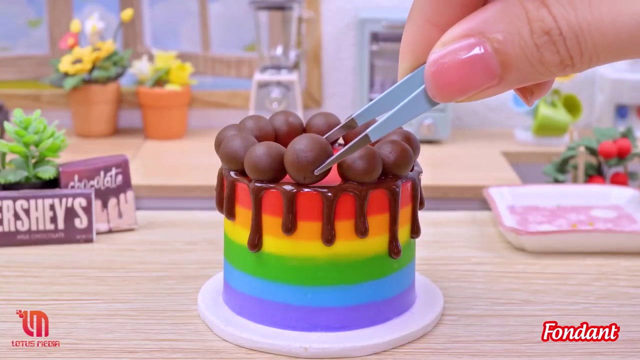 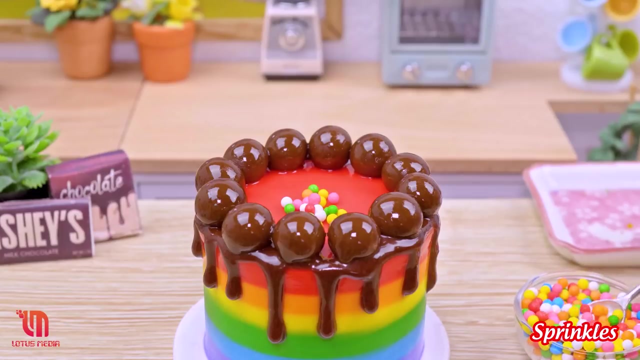 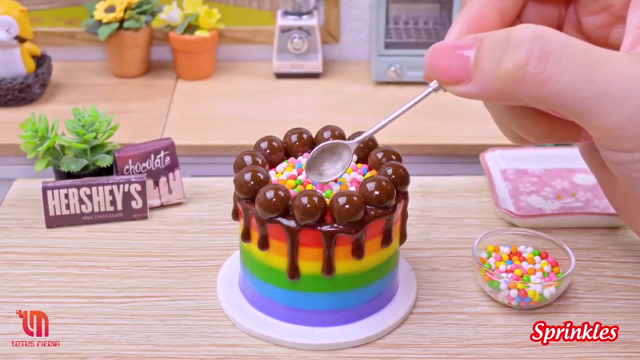 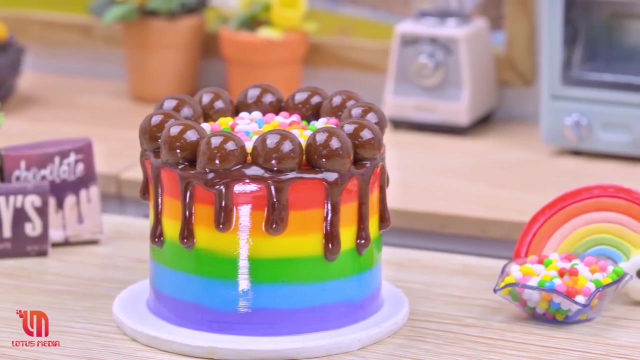 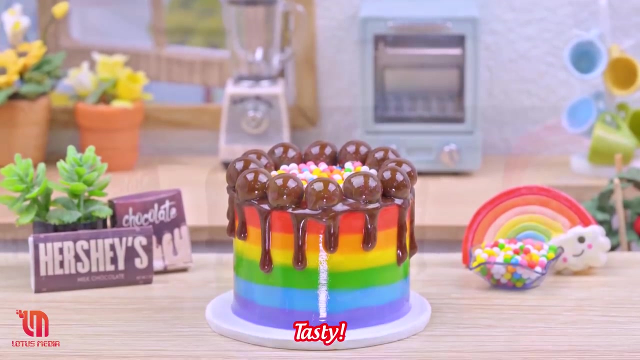 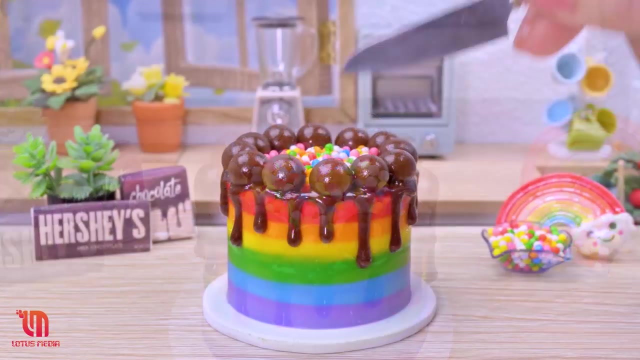 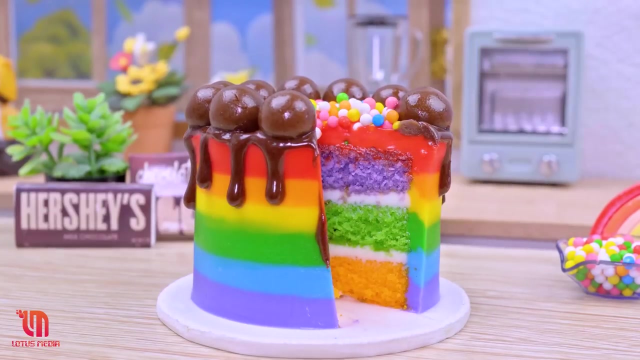 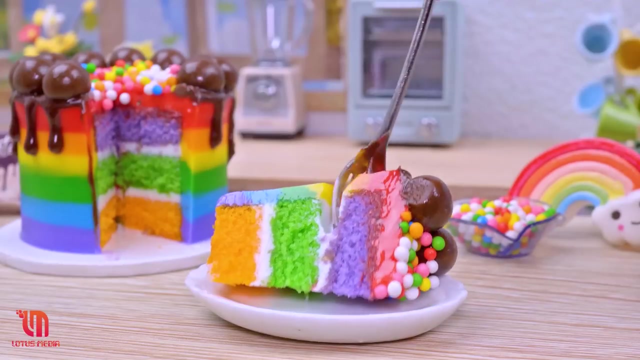 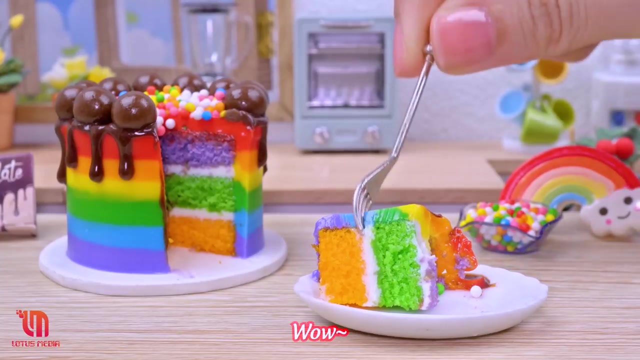 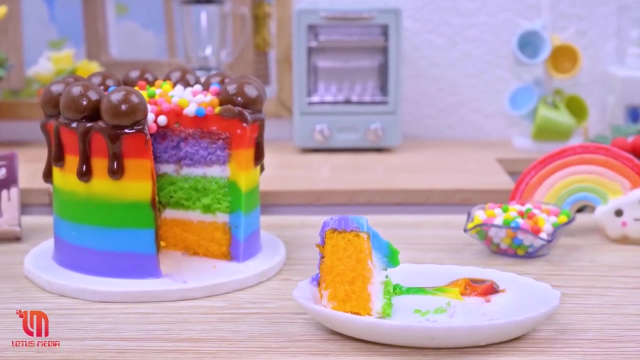 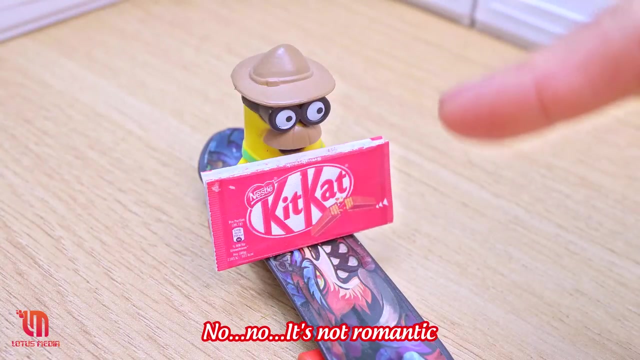 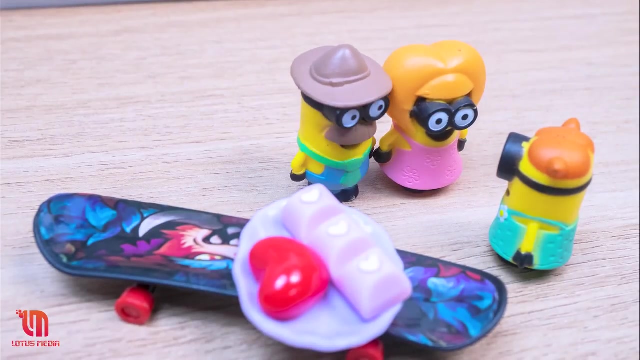 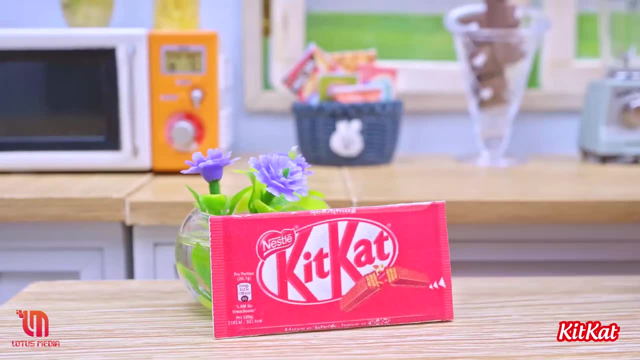 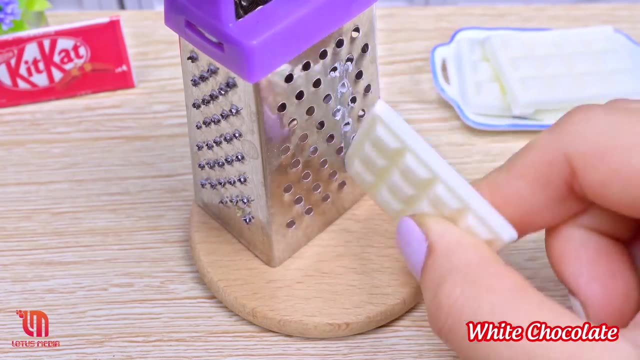 Hi, Hi, Hello. someone is calling Quickly. Who do you want me to be? Do you need a coffee about aання in DOWNTOWN? NO år, You just drink some. We can be together. Yes, yes, 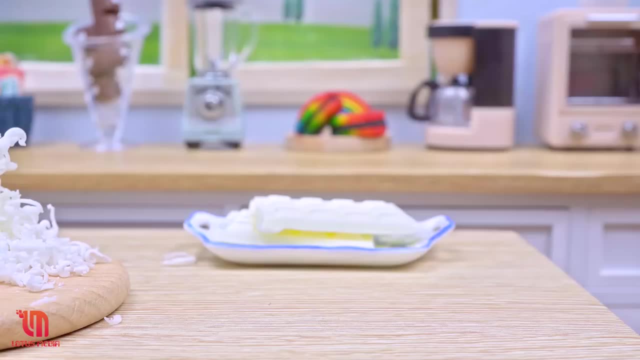 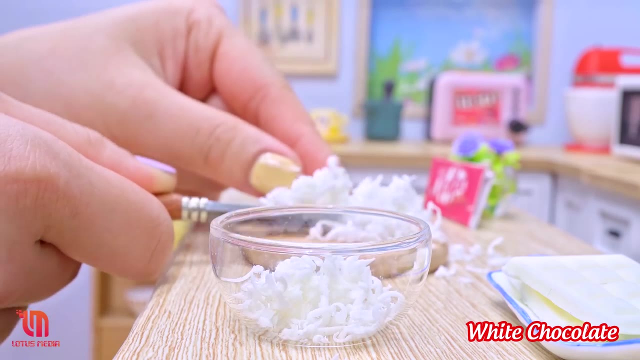 Would you like to have some coffee? We can return tomorrow. Hello, Hello sweet. Hello, Whoパパ, You are decoration for HELLINOISaux. You are decoration for HELLINOISaux. I'm going to make the sauce. 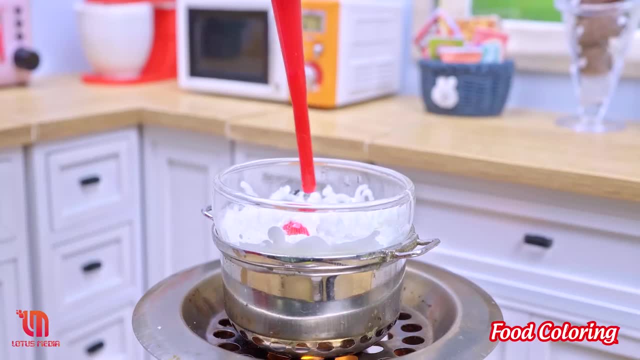 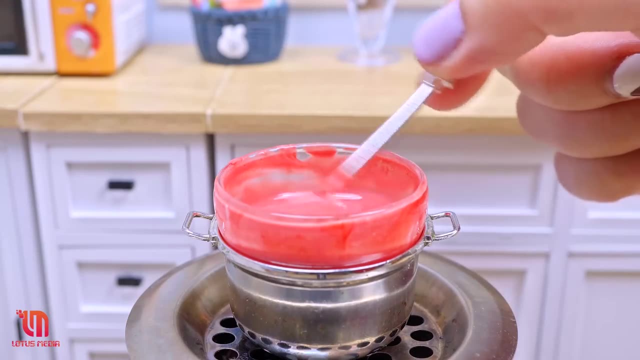 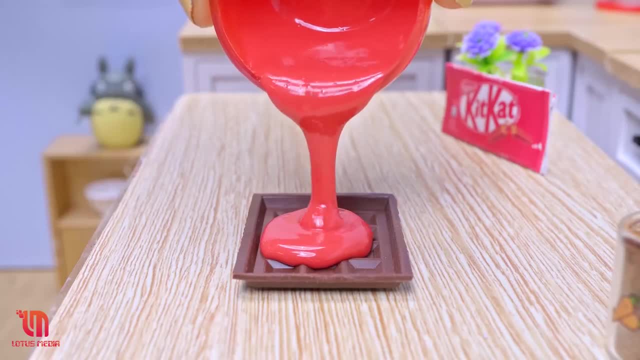 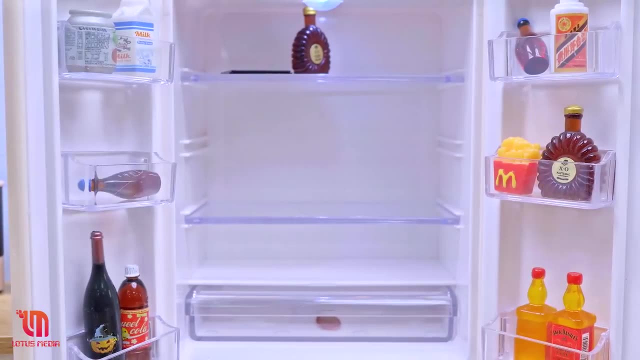 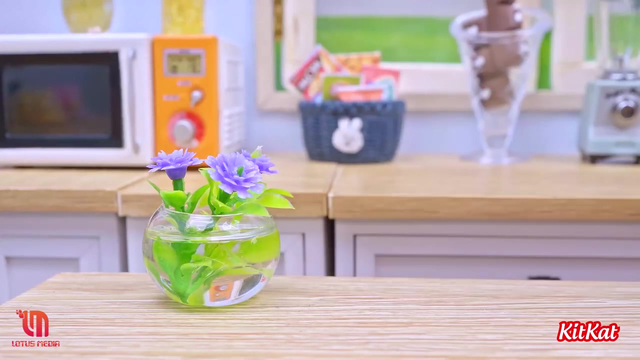 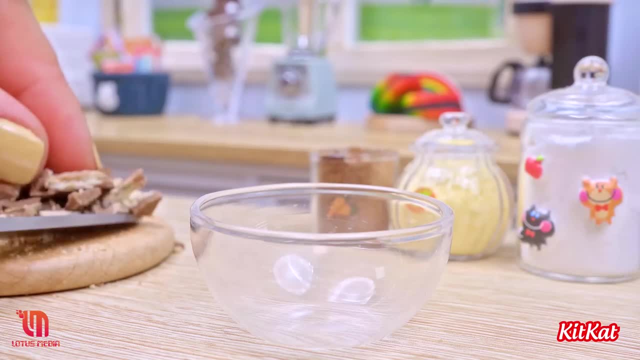 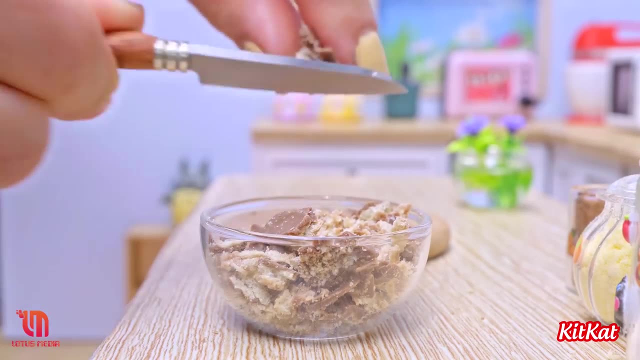 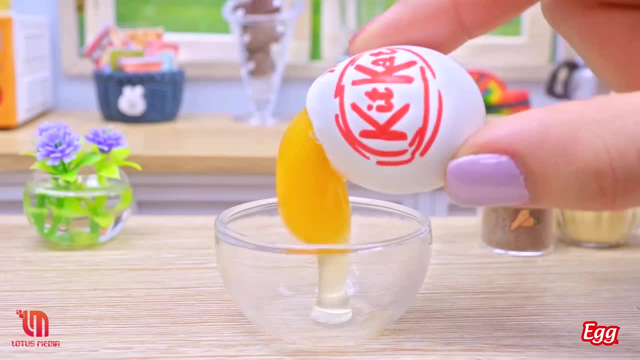 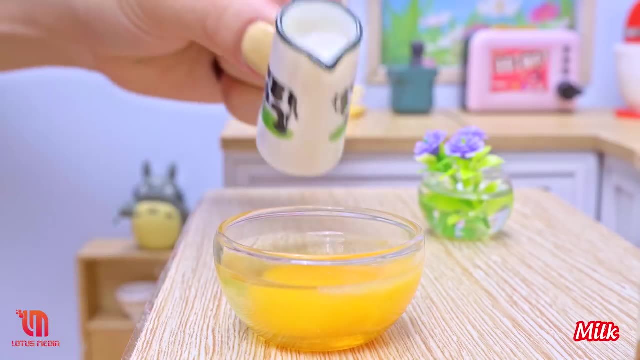 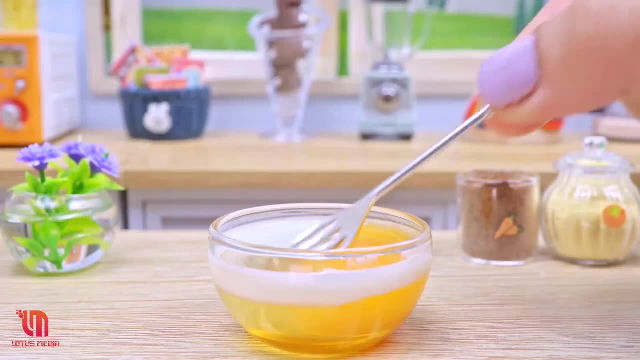 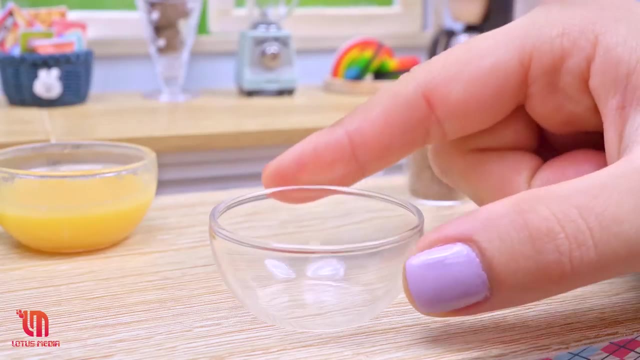 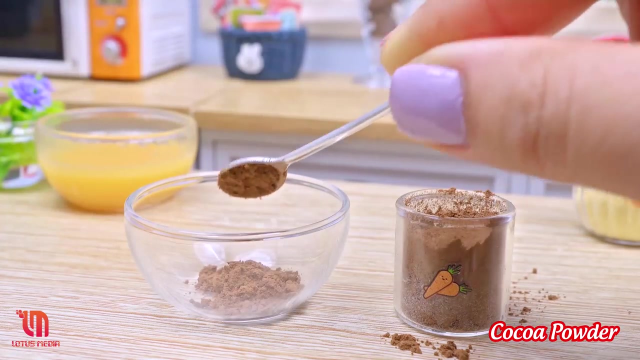 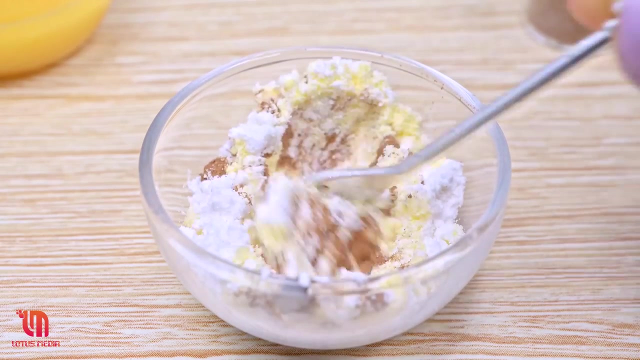 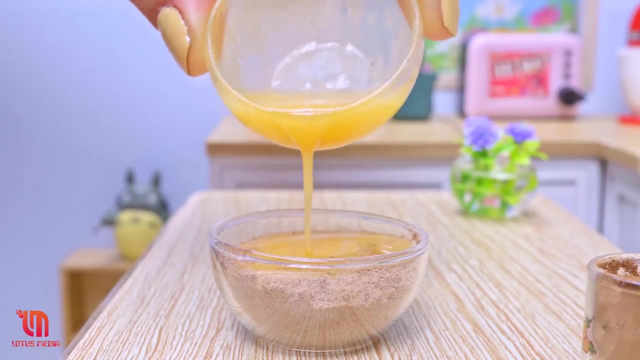 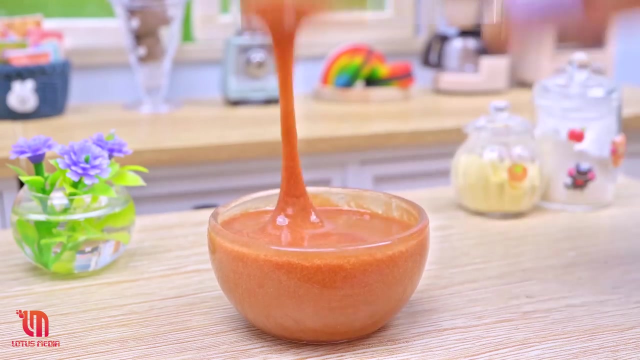 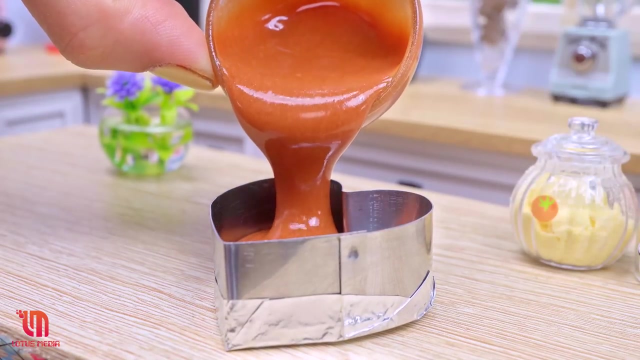 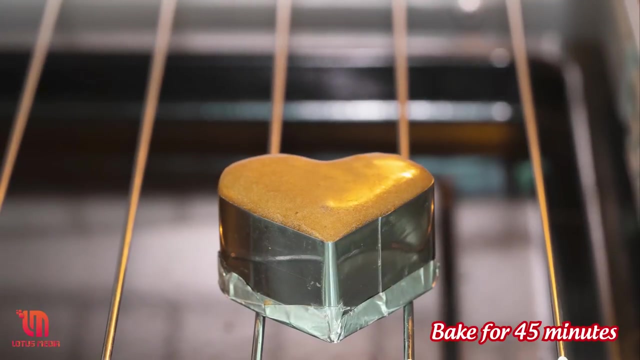 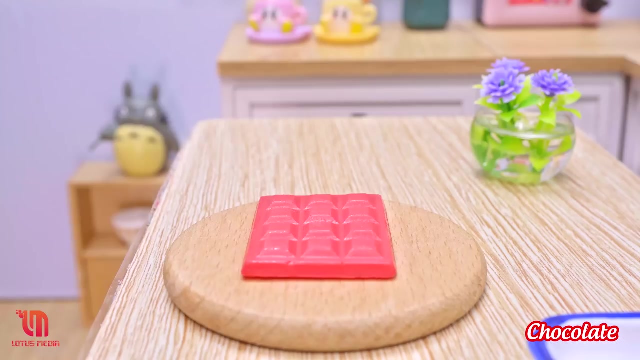 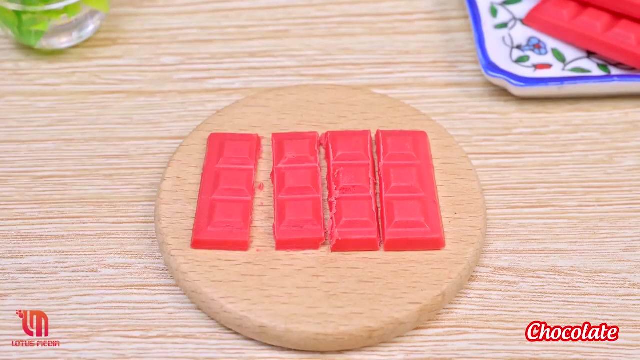 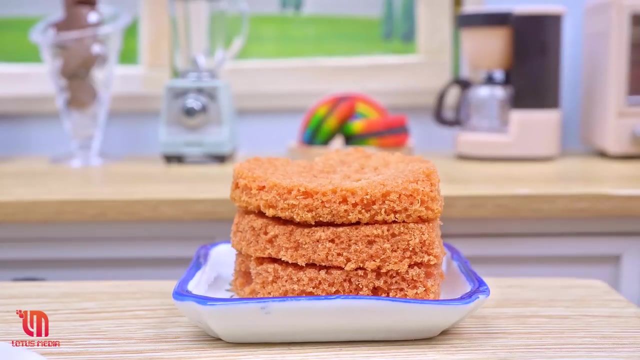 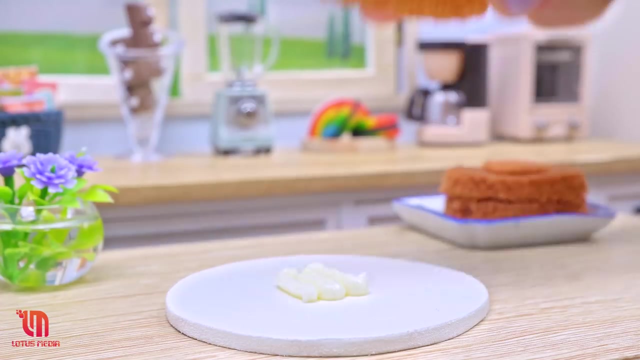 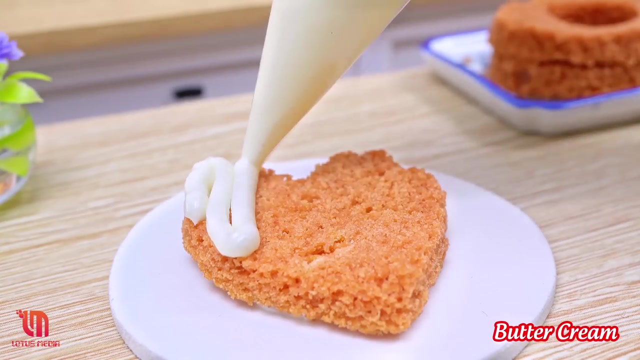 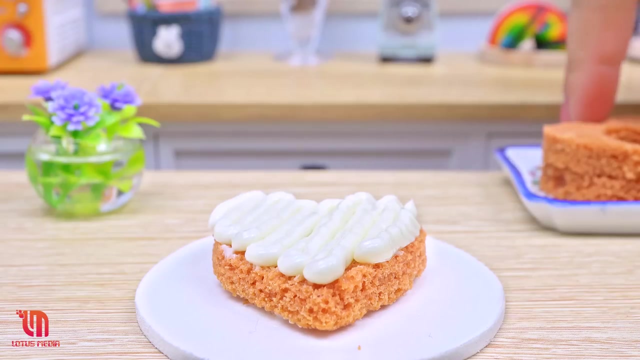 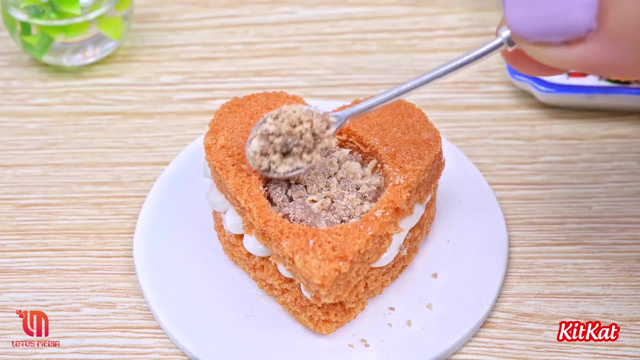 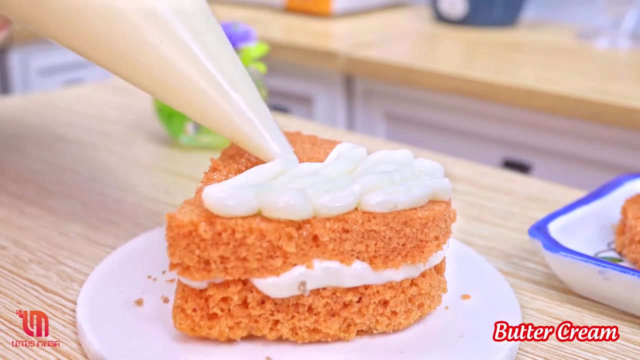 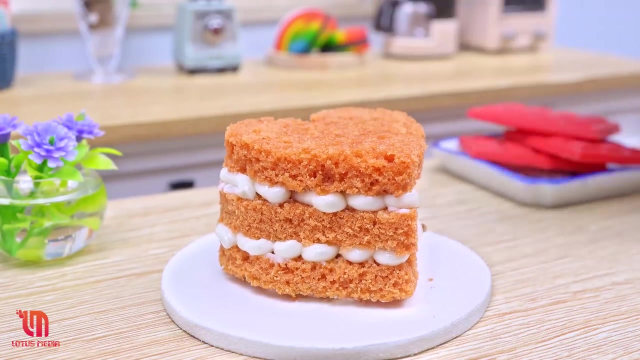 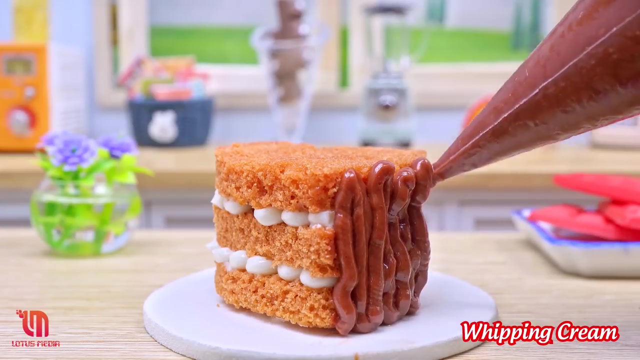 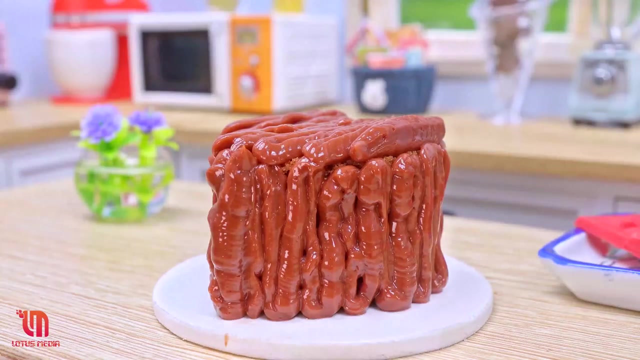 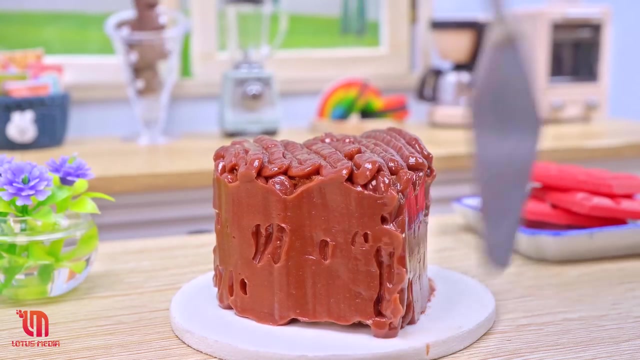 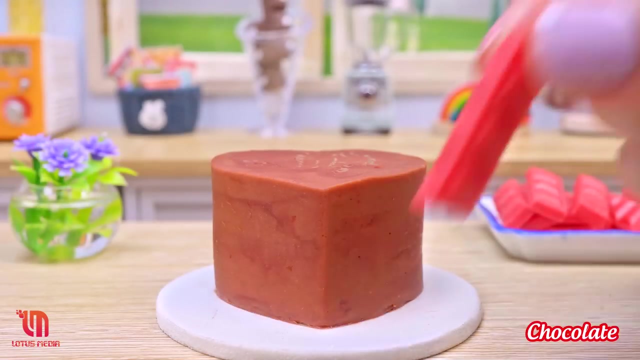 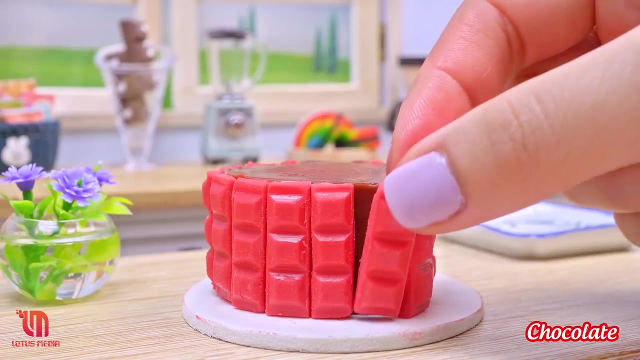 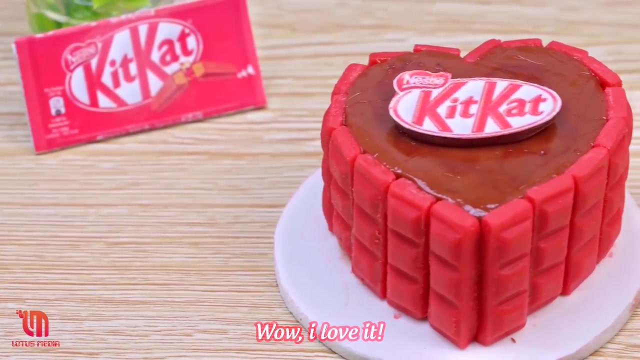 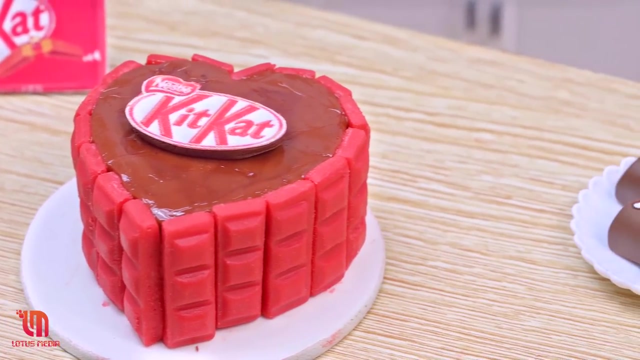 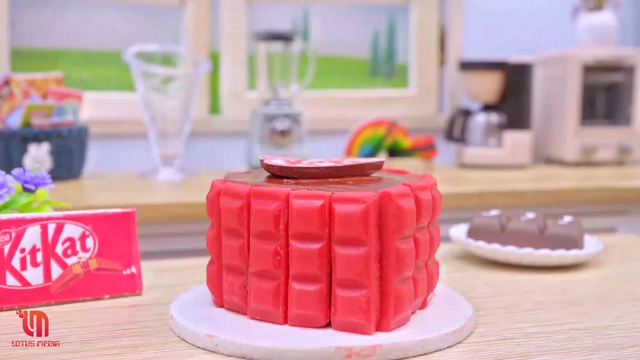 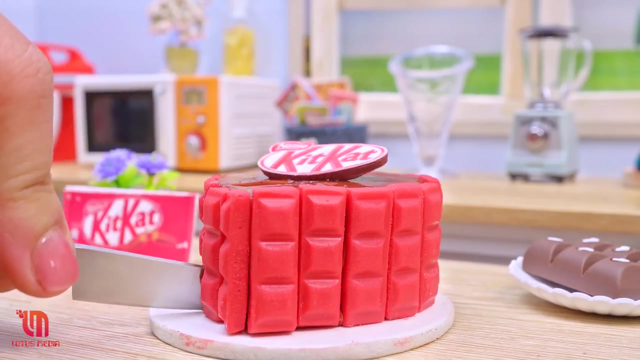 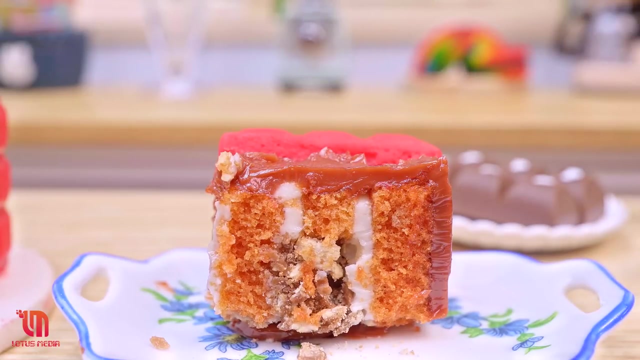 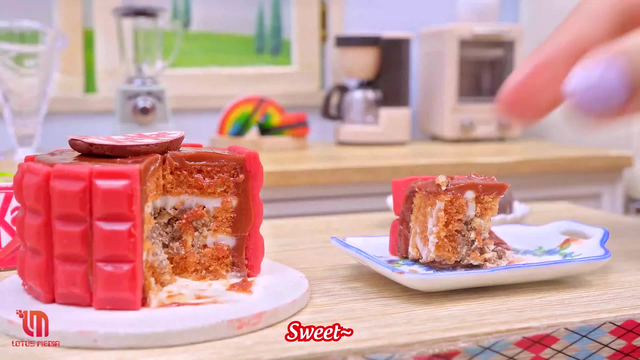 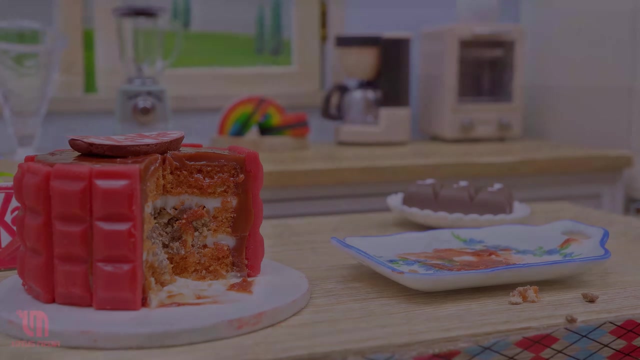 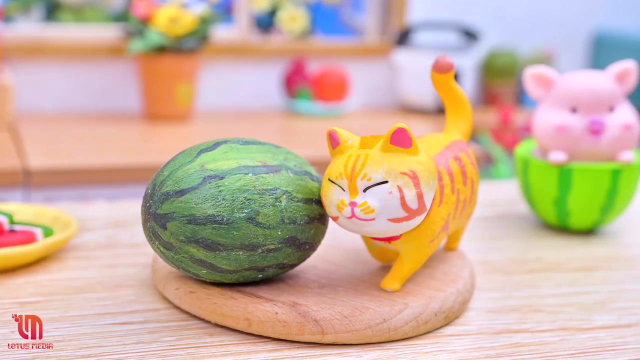 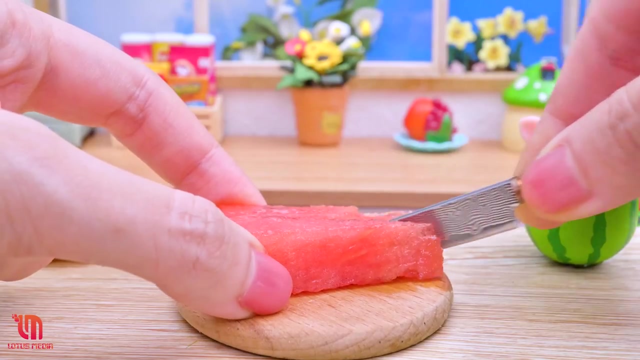 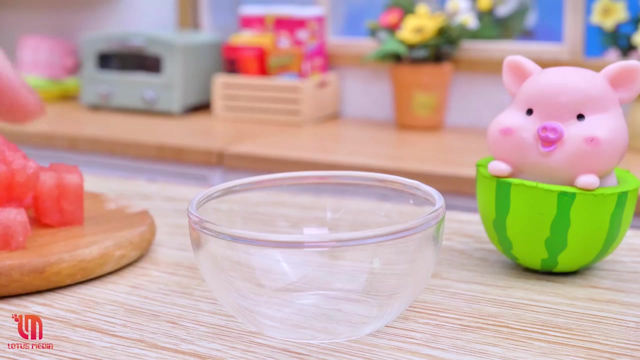 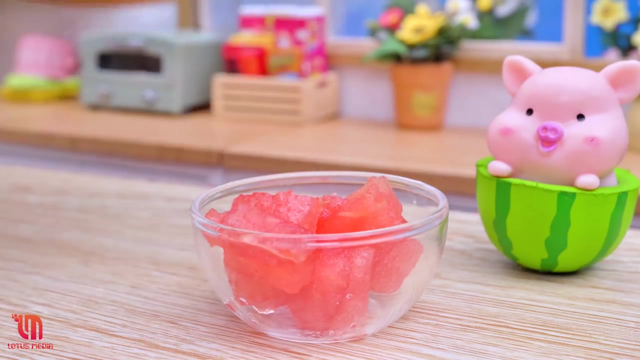 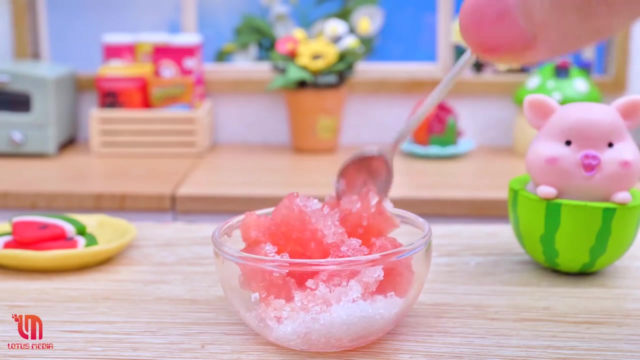 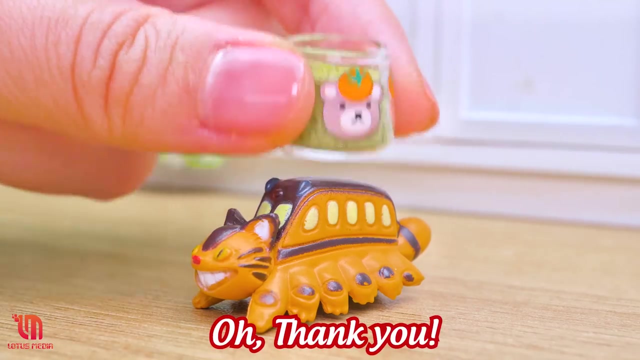 I'm going to make the sauce. Thank you, Thank you. Oh, wow, Thank you, Thank you, Wow, I love it. Delicious, Tasty, Wow, Sweet, Yummy, Wow, Wow, Oh, thank you. 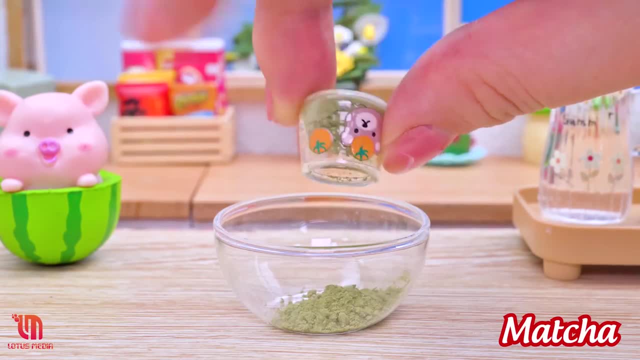 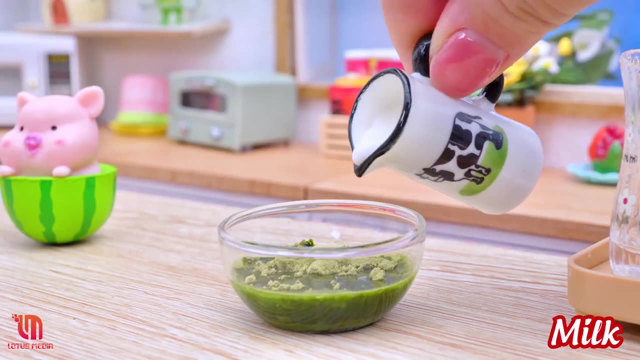 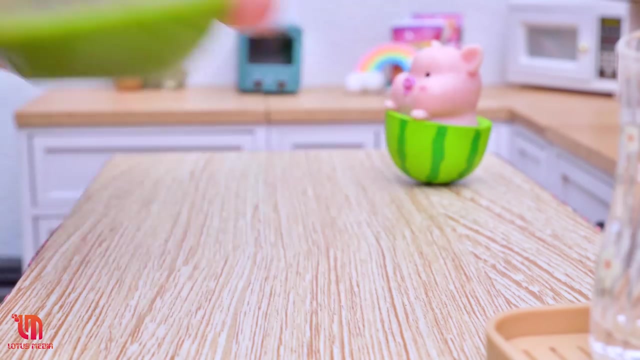 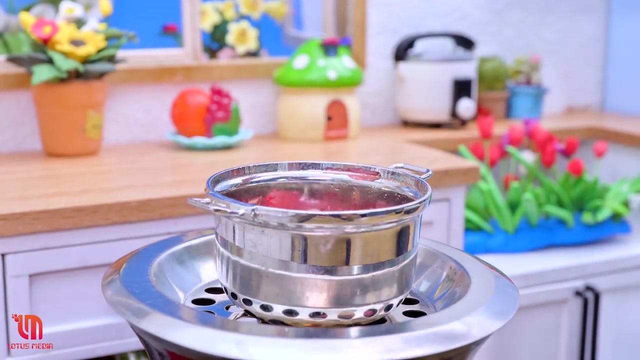 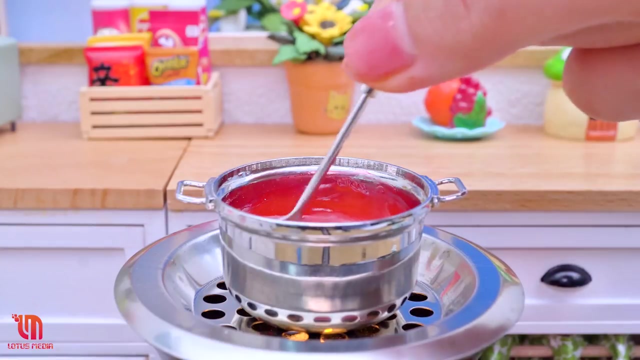 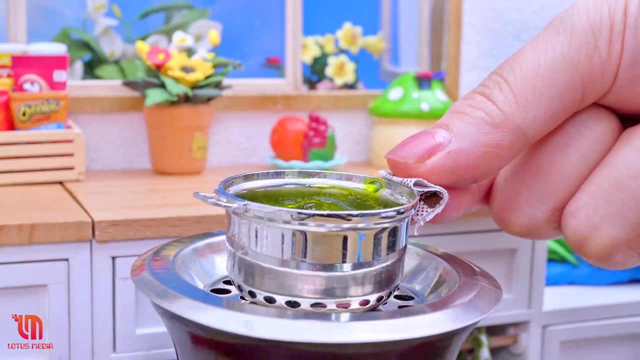 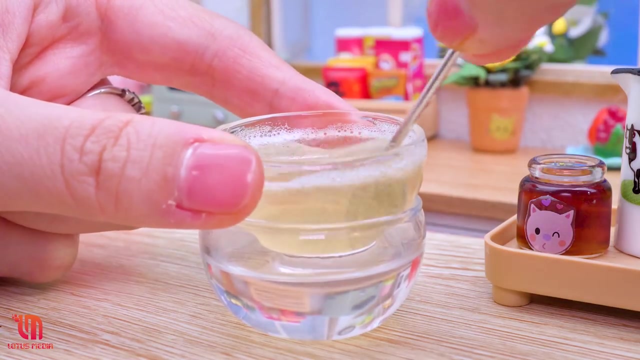 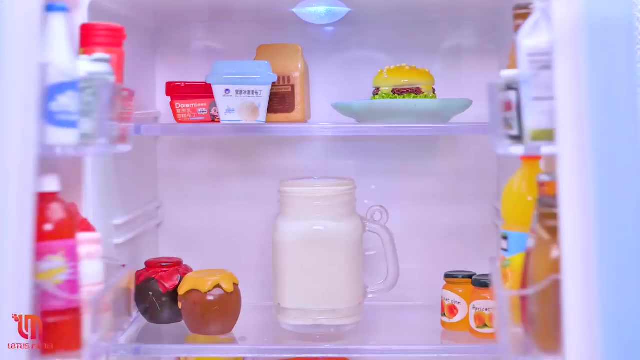 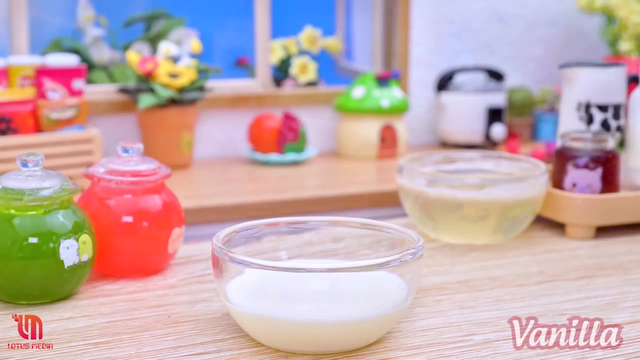 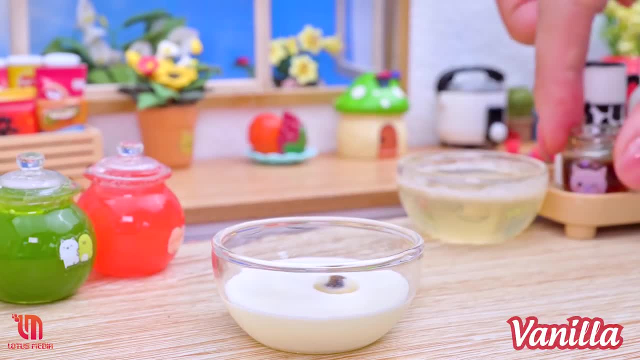 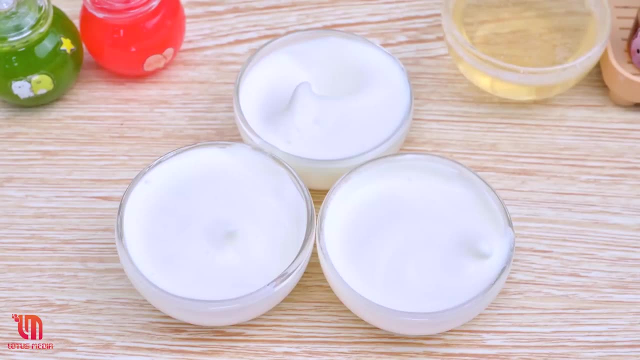 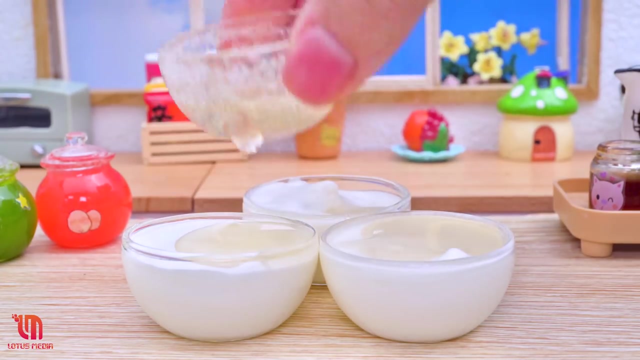 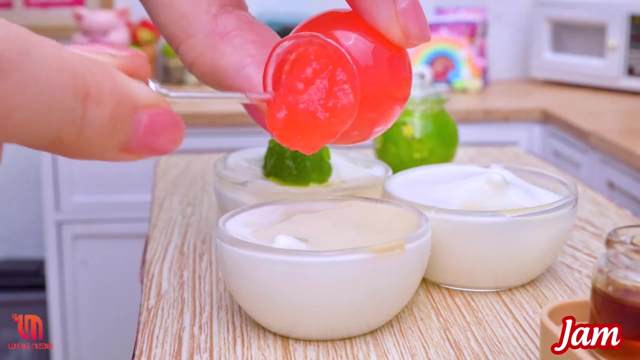 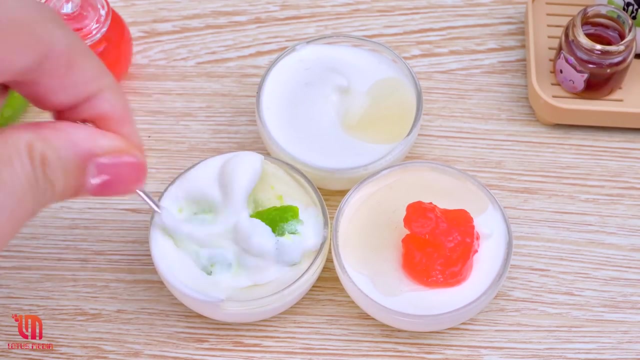 Add 1.5 cups of water to the pot and cook over medium heat. Stir-fry the vegetables: Add 1 cup of rice cake and stir-fry: Add 1 cup of rice cake. Stir-fry the vegetables. I don't like spicy food, so I recommend you try it this way. 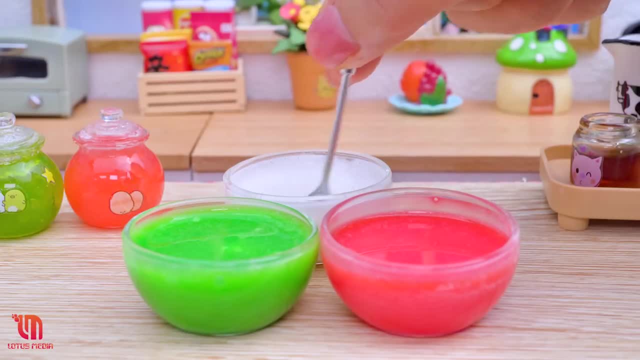 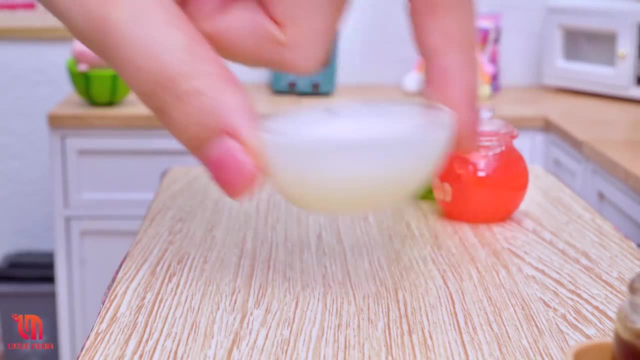 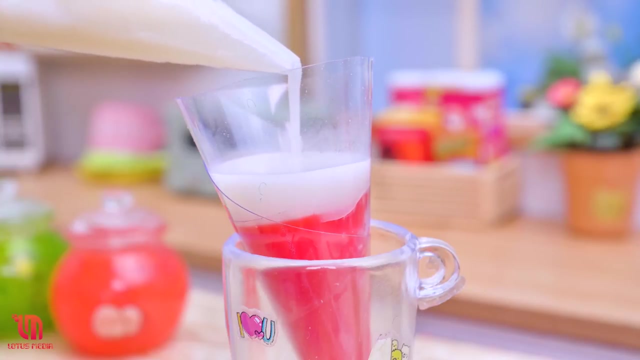 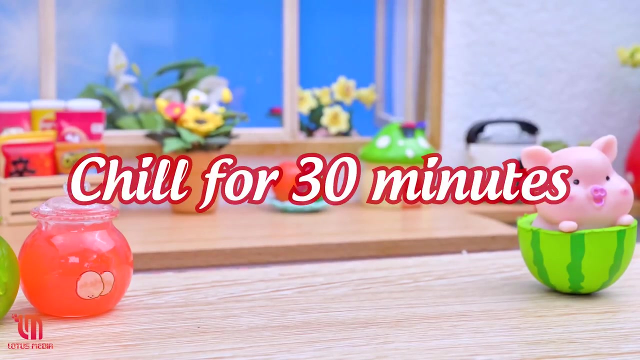 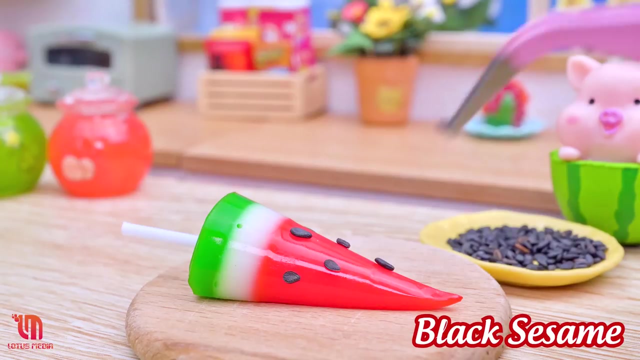 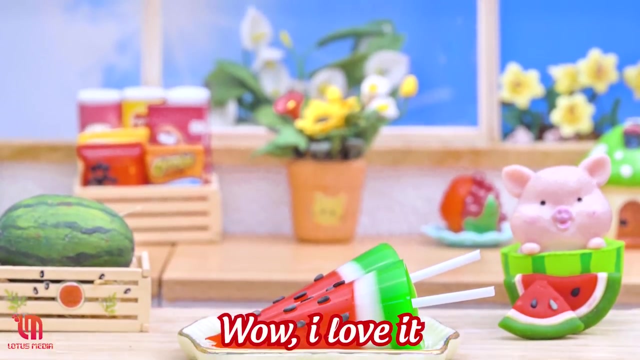 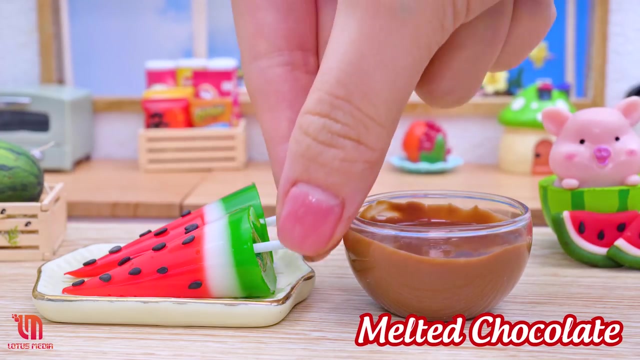 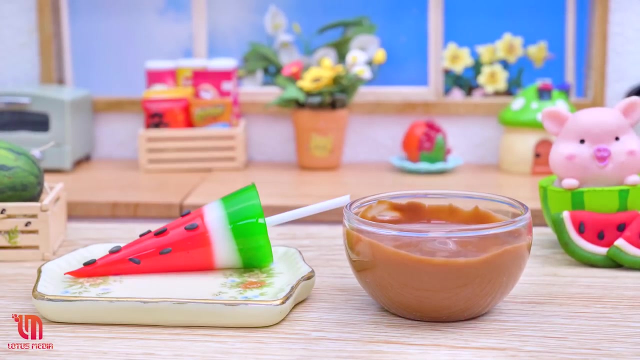 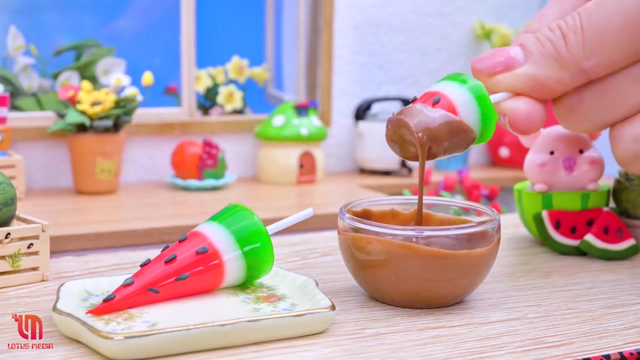 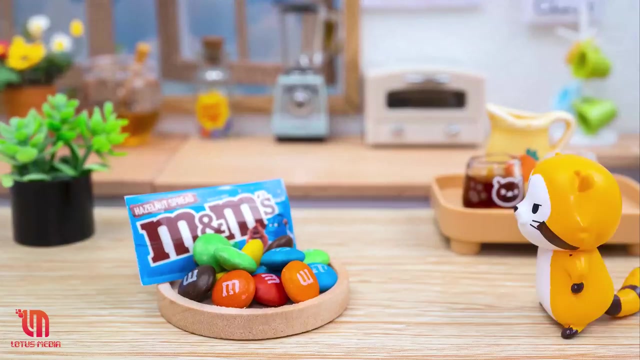 I'll try it with the raw octopus next time. Let's get started, Take the octopus and fry it. Add the sauce you made earlier. Wow, I love it. Delicious, Sweet, Yummy. Oh no, It's not for you. 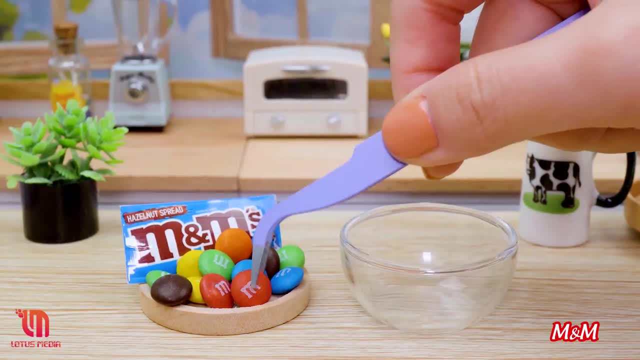 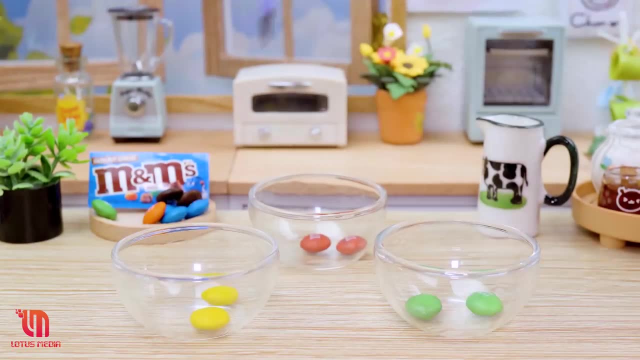 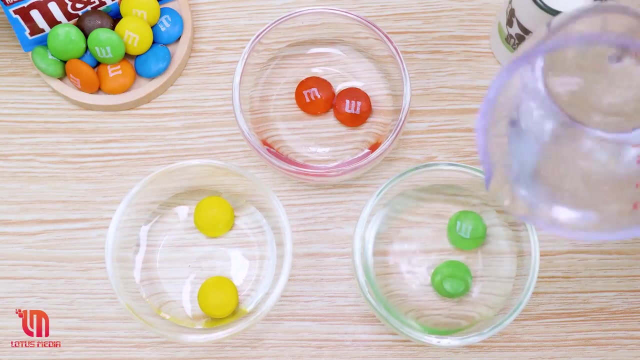 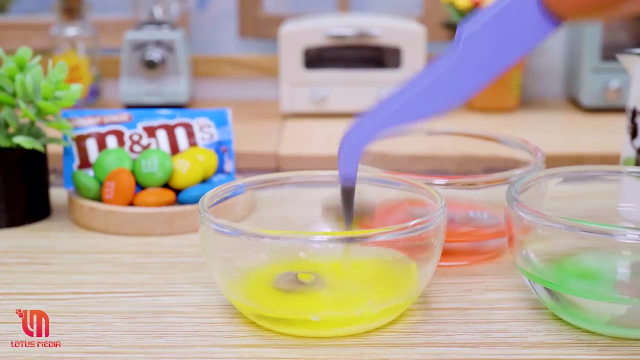 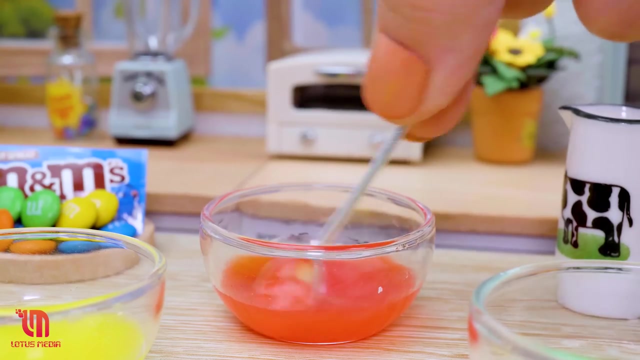 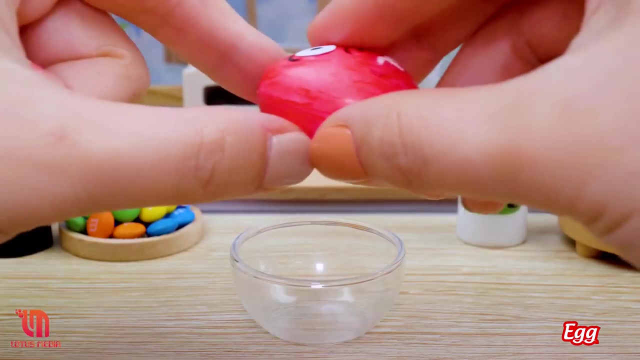 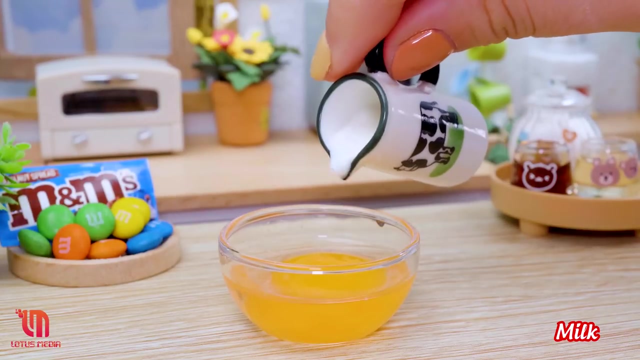 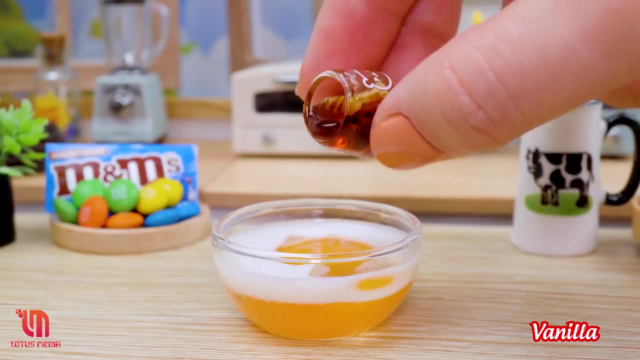 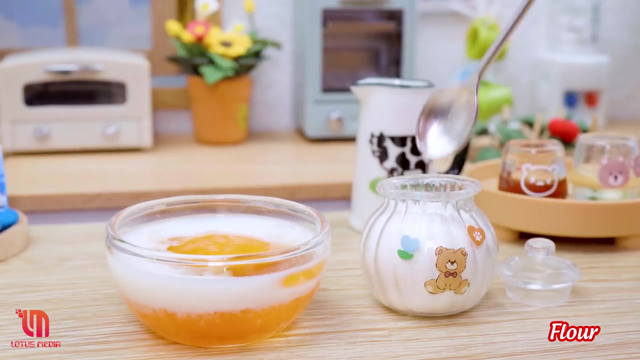 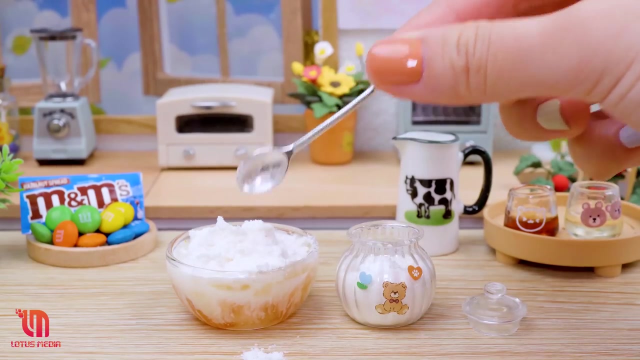 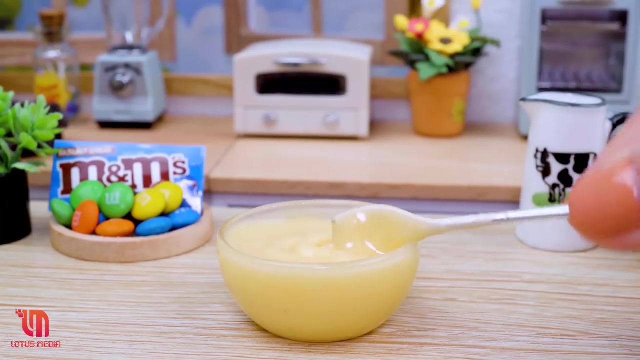 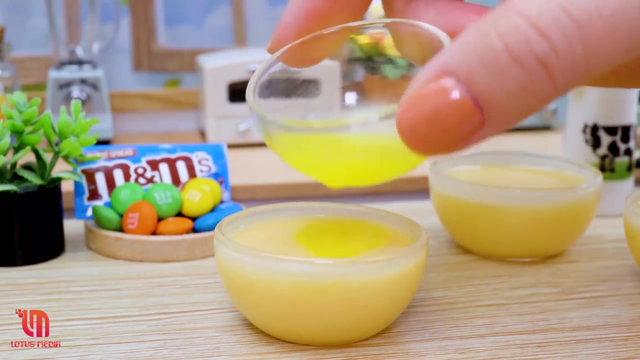 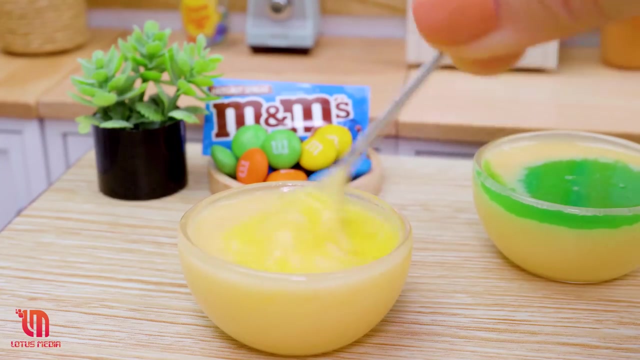 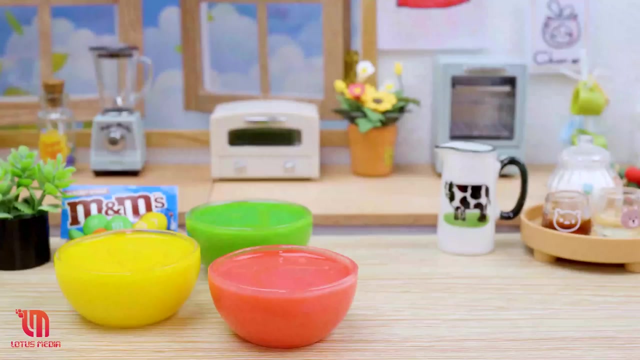 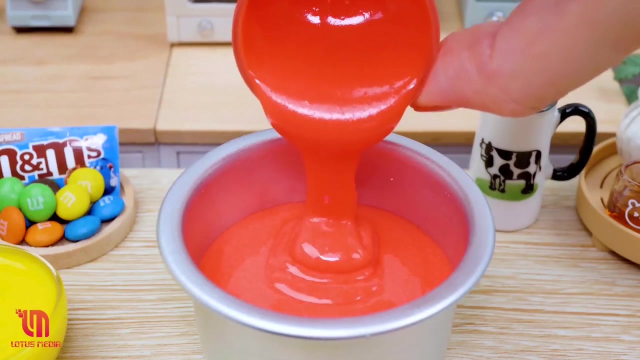 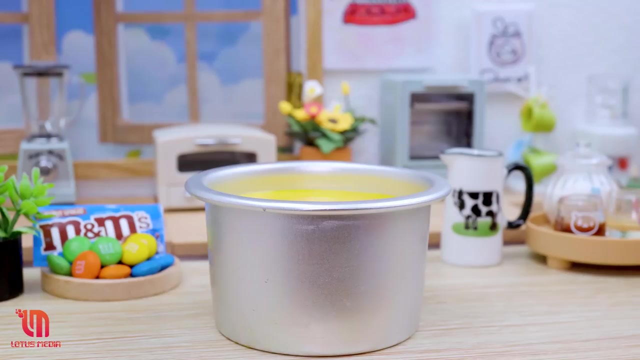 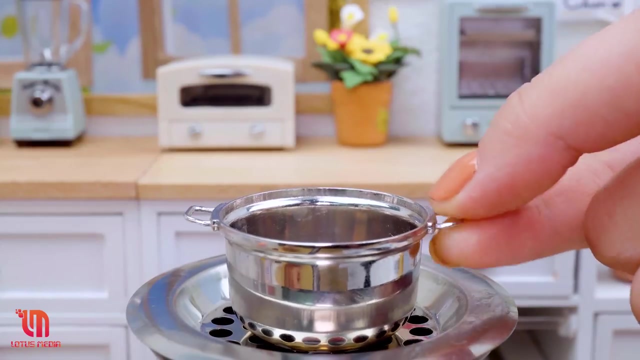 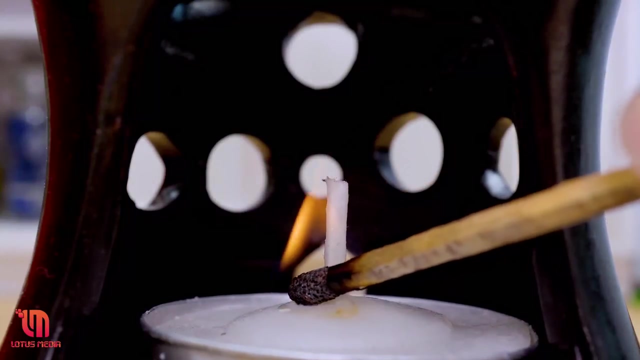 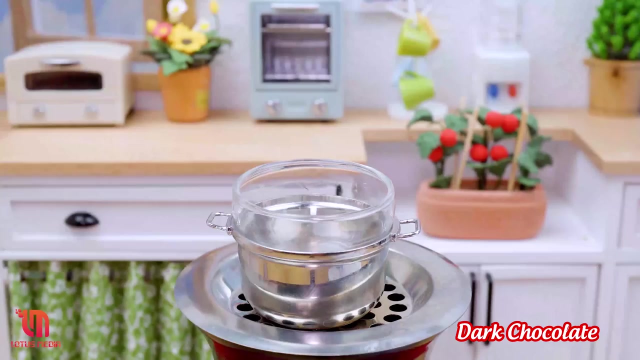 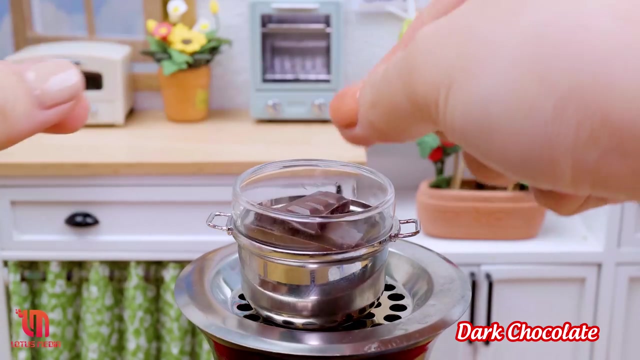 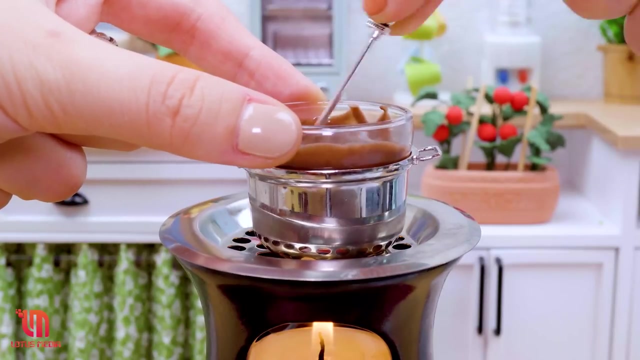 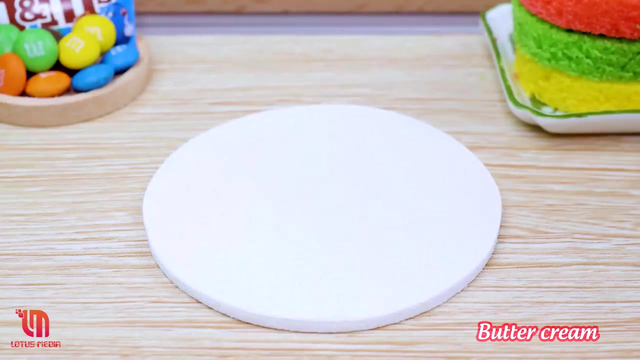 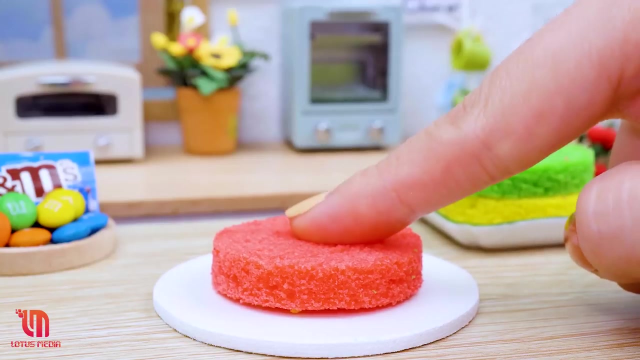 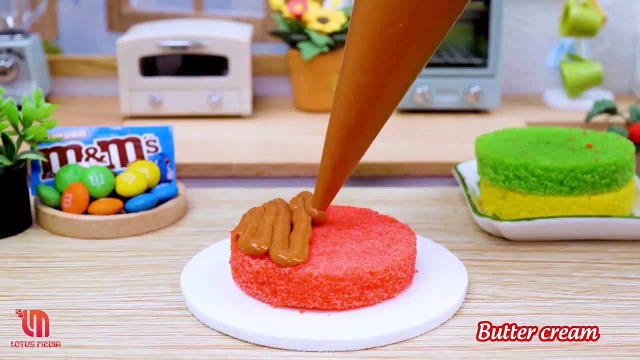 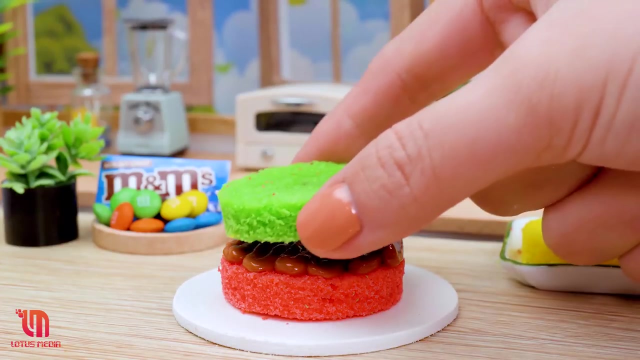 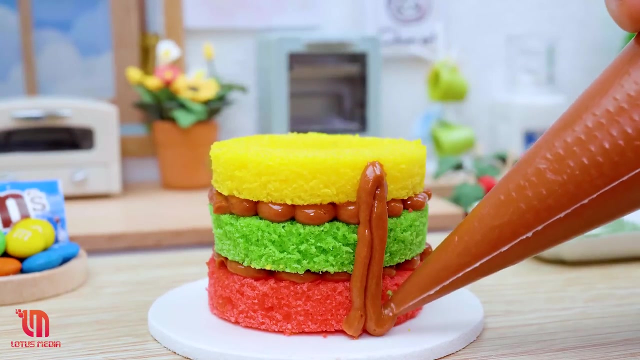 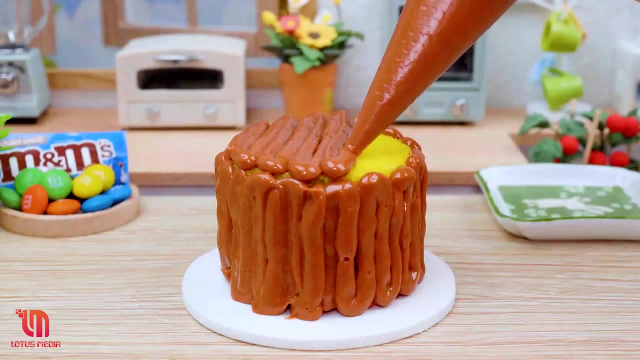 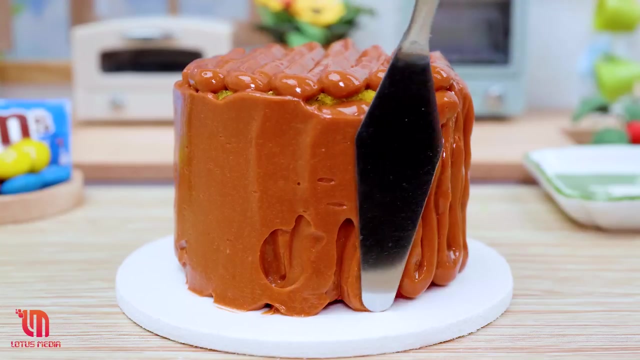 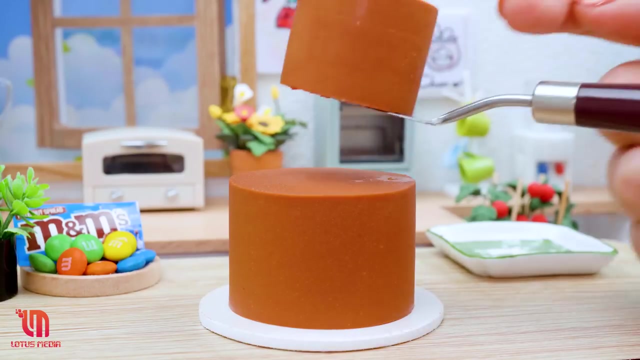 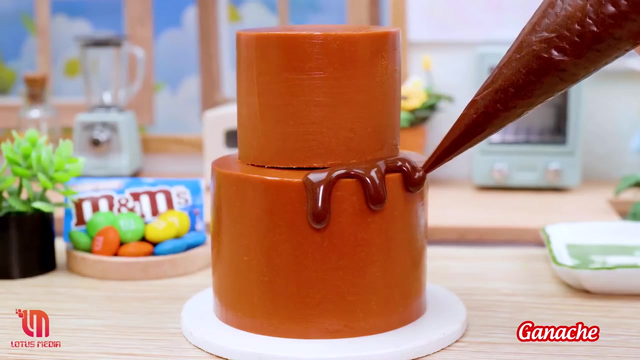 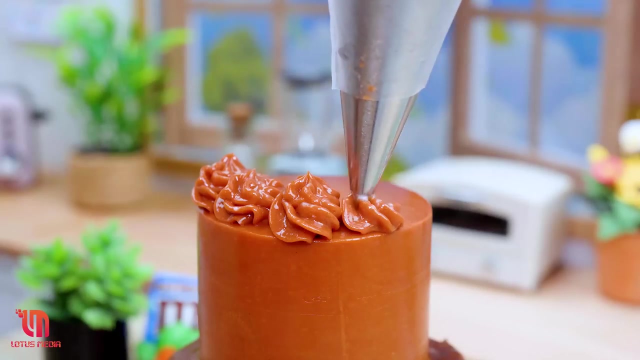 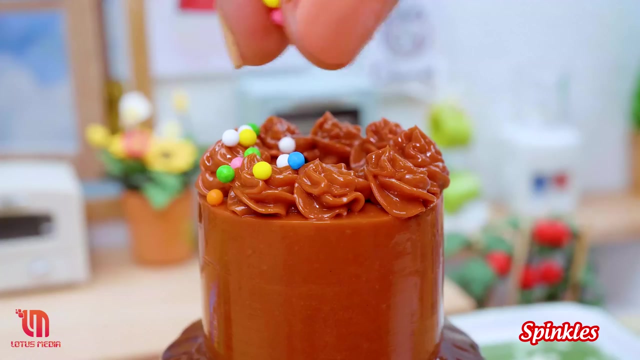 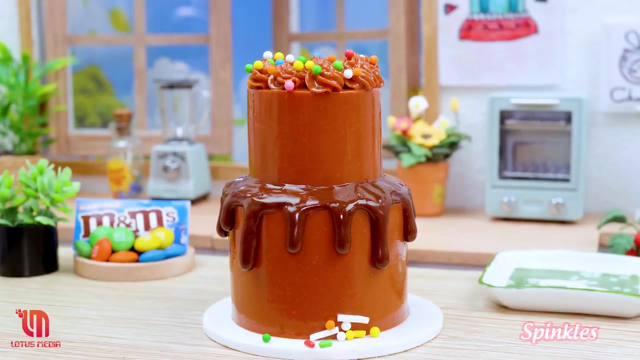 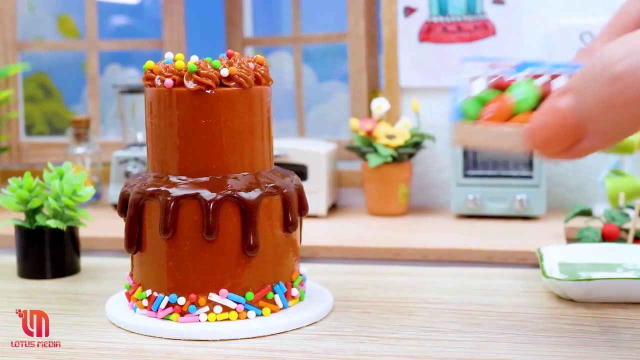 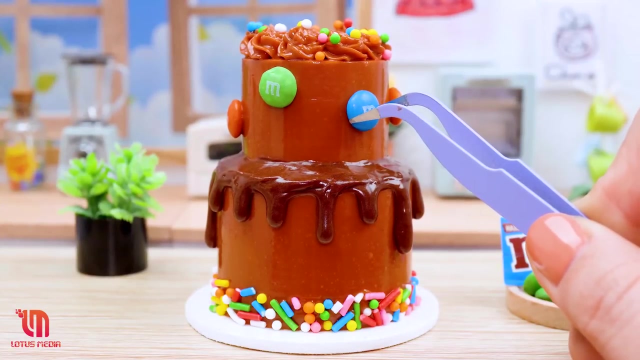 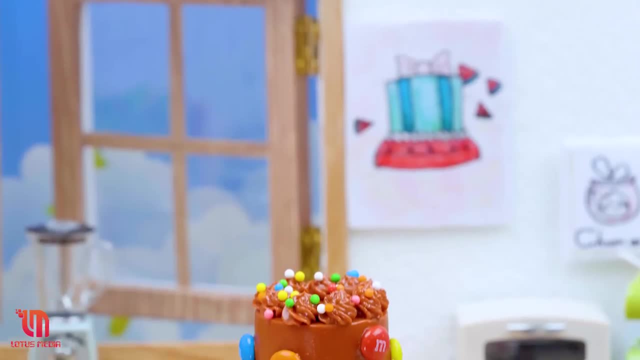 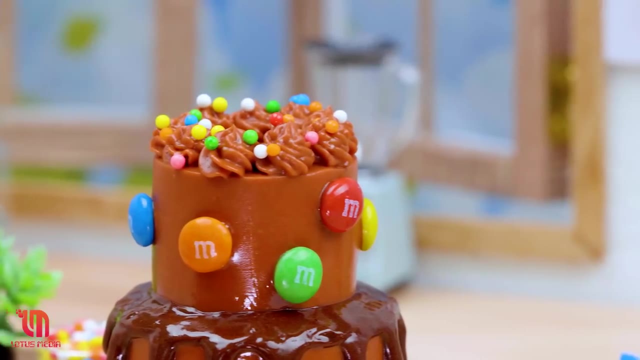 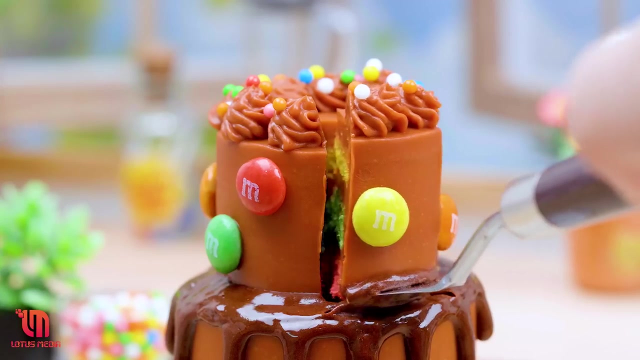 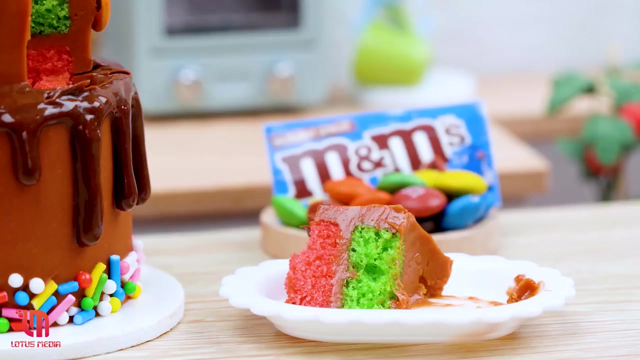 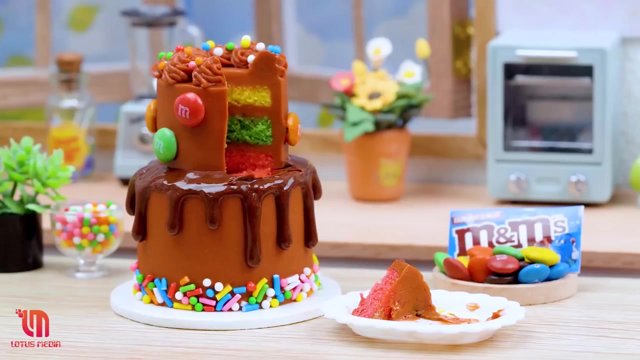 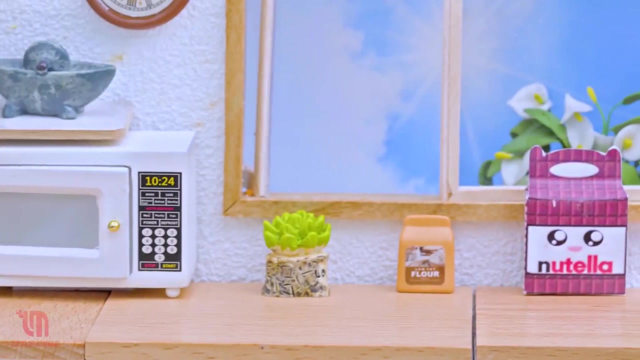 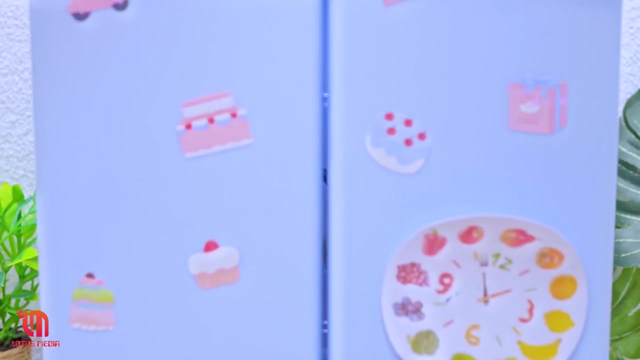 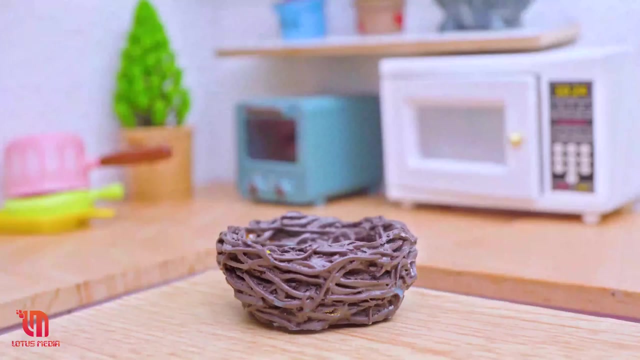 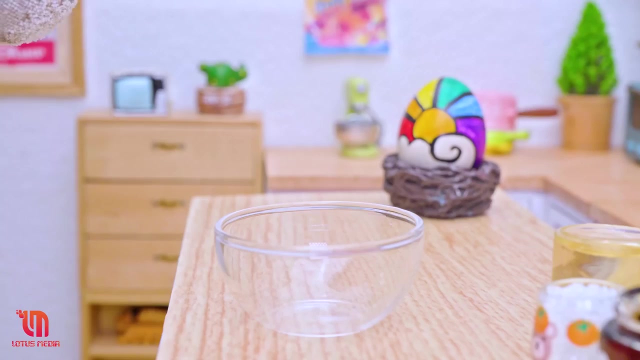 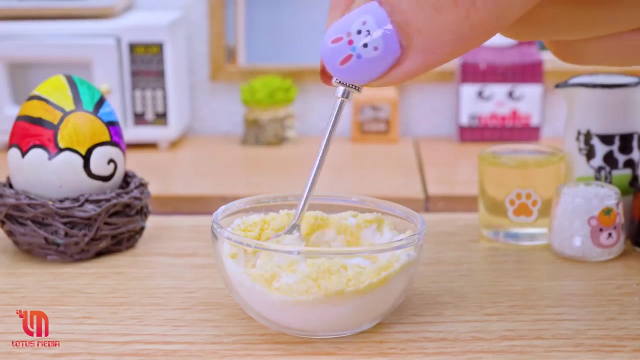 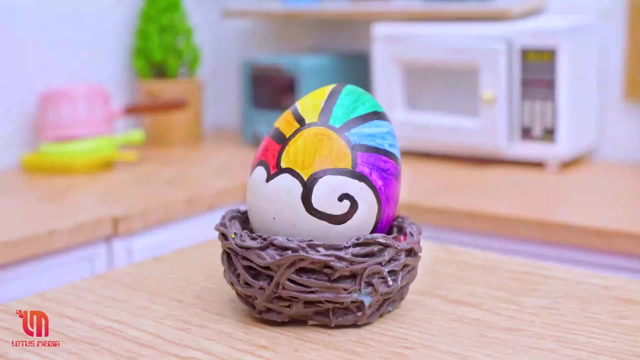 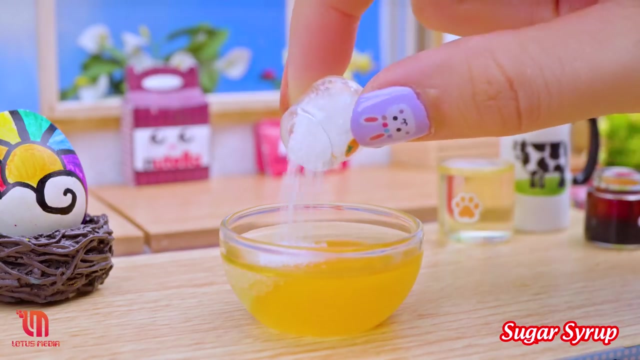 Wow, Sweet, It's for me, It's for me, It's for me, Tasty. I'm going to make a sweet and sour cake. Add 1 cup of water. 1 cup of water, 1 cup of water. 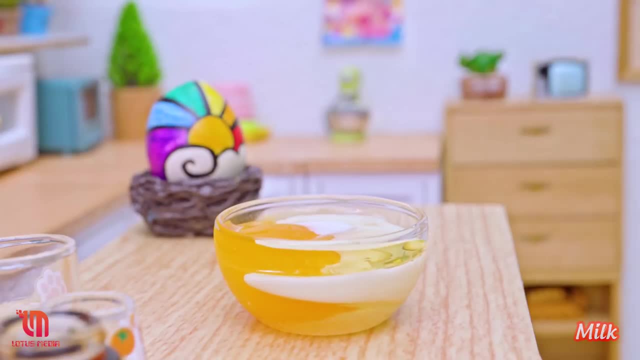 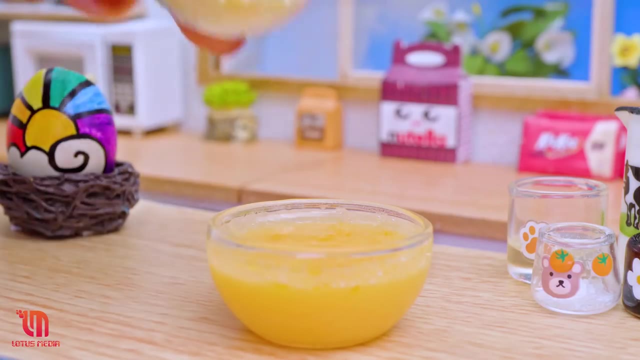 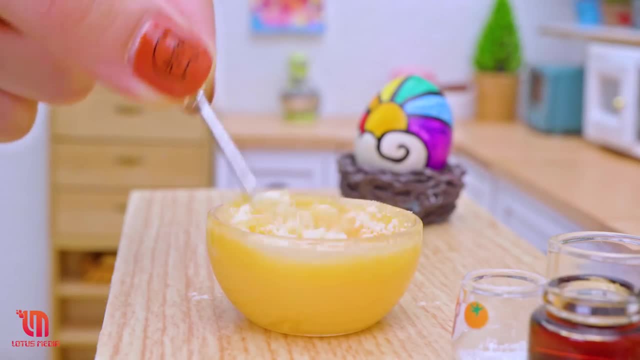 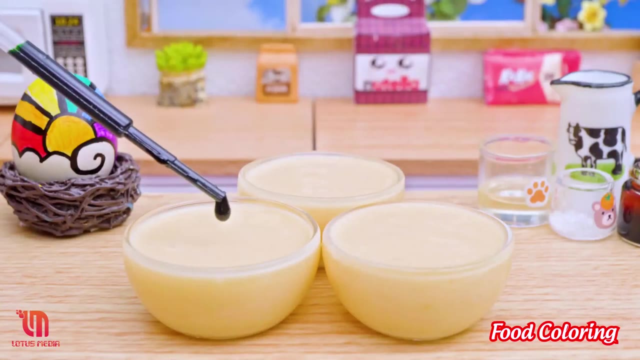 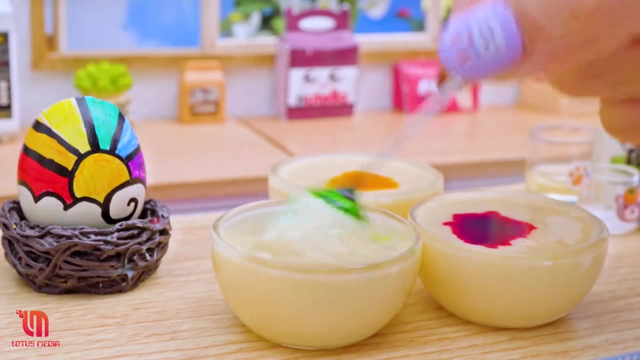 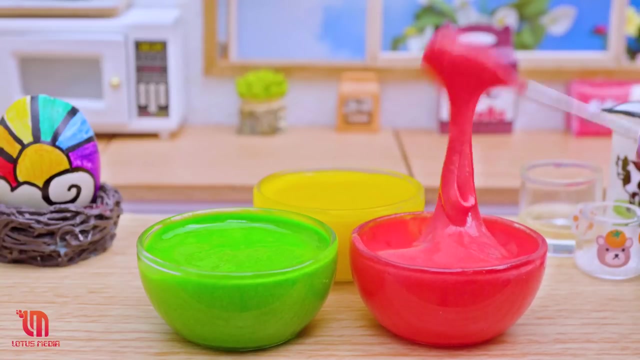 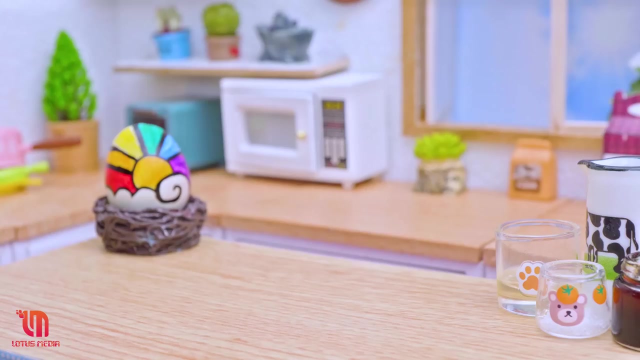 vinyl rolls, sticky plastic, glass, batter water, The Point05. Put the drawn mask and 啦, Make the pa. I'm going to make the sauce. I will put it in a bowl. I will put it in a bowl. I will put it in a bowl. 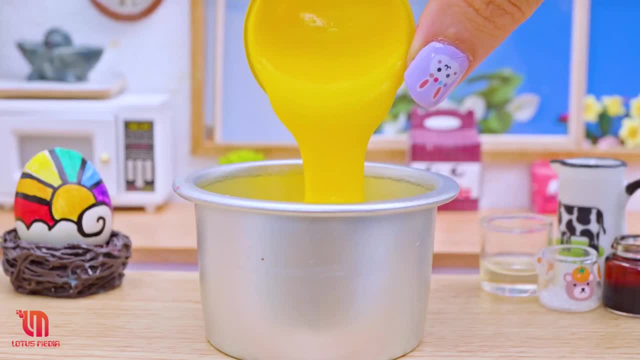 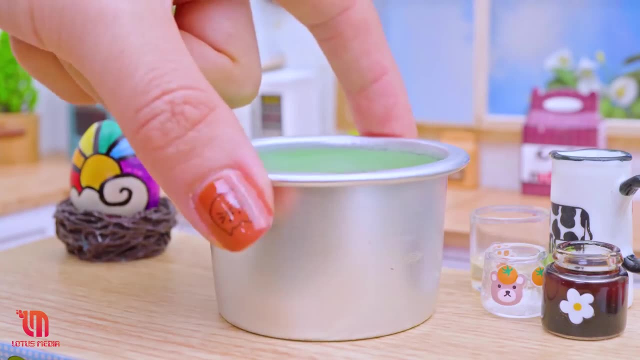 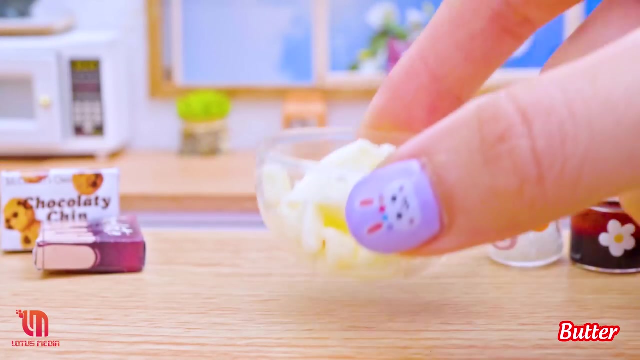 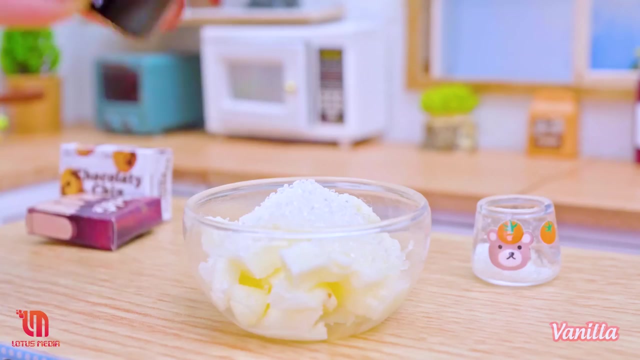 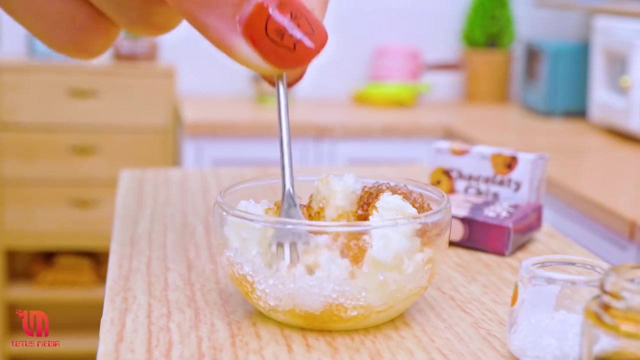 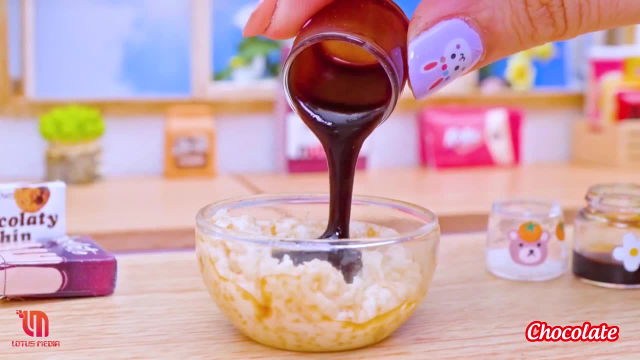 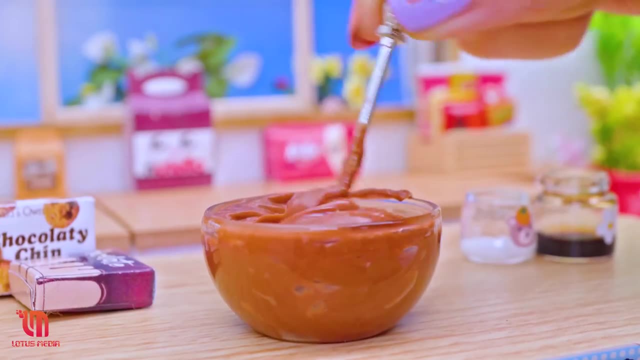 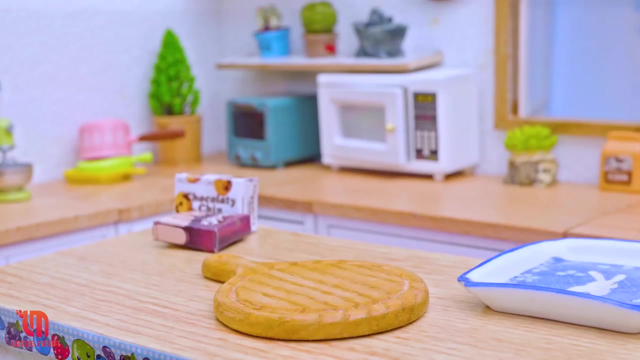 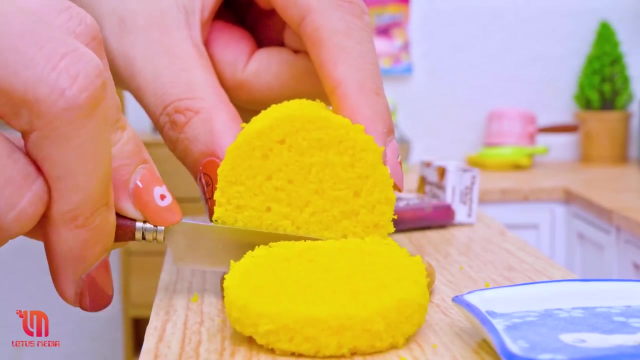 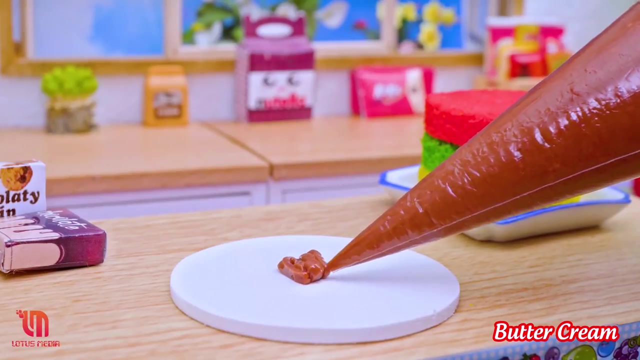 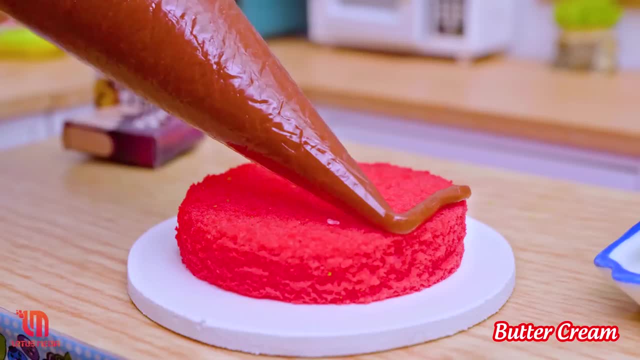 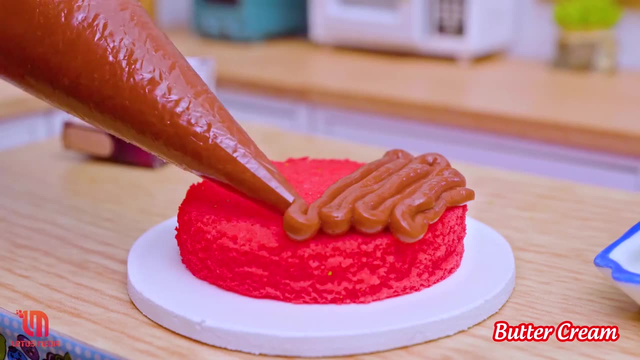 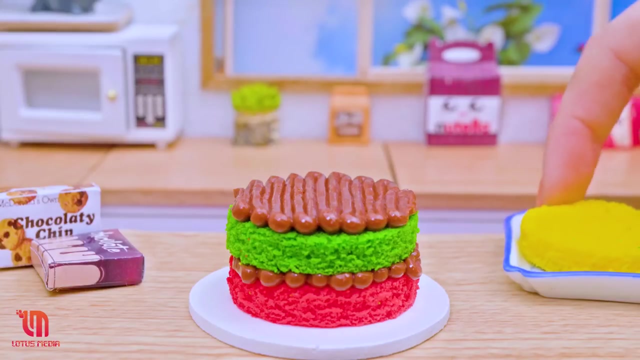 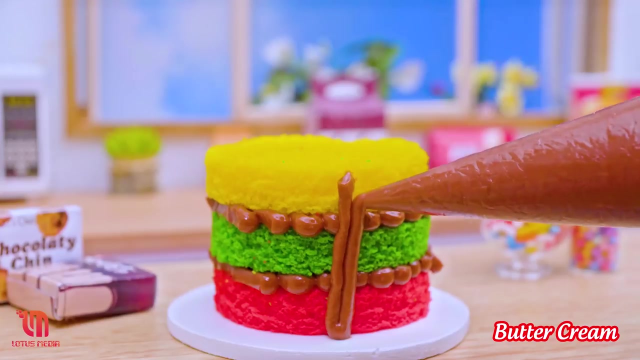 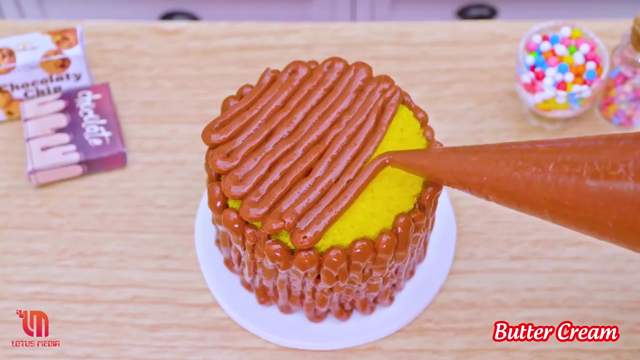 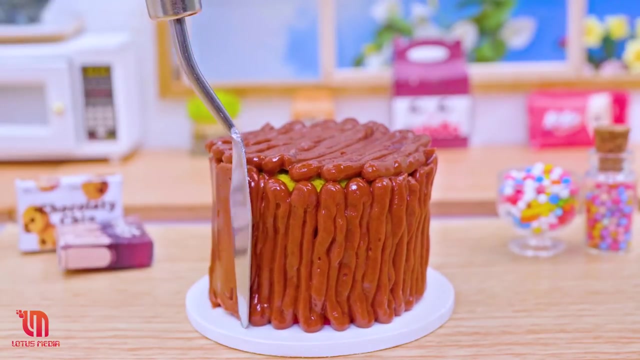 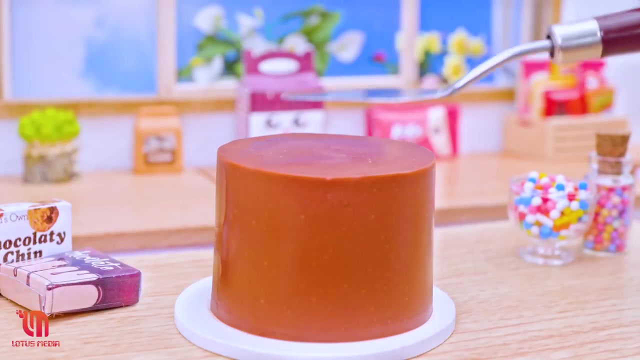 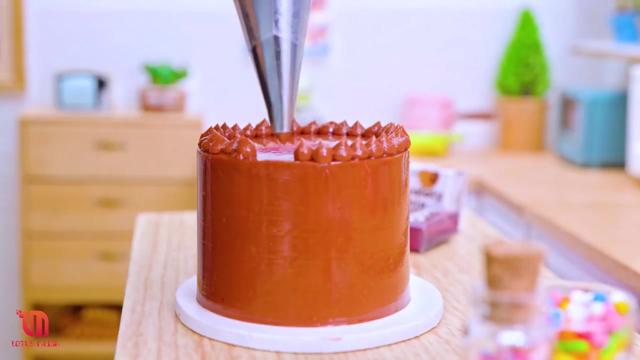 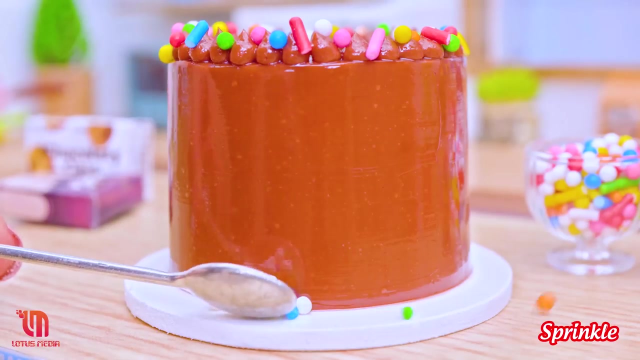 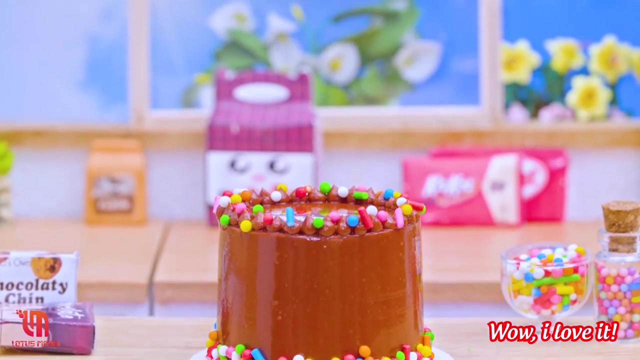 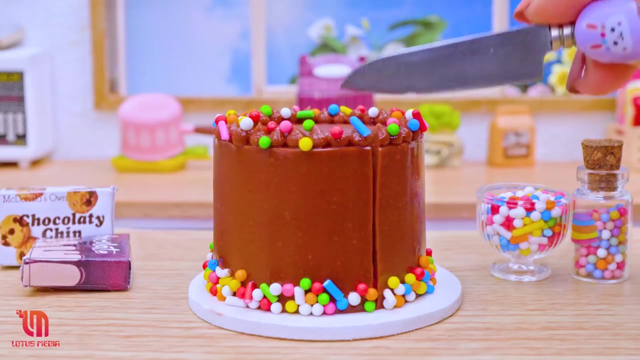 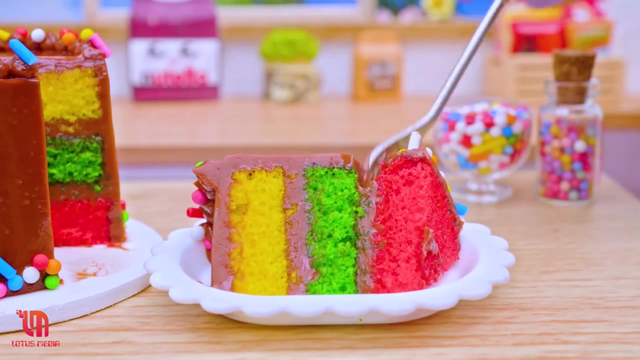 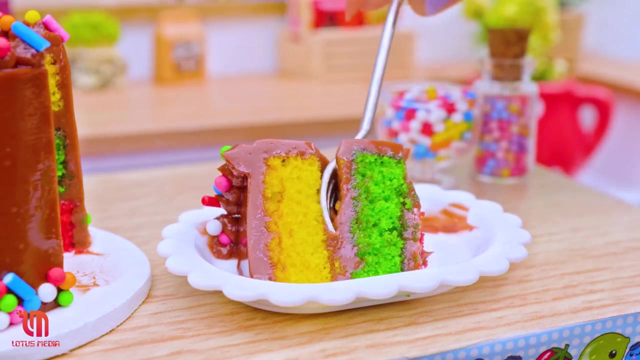 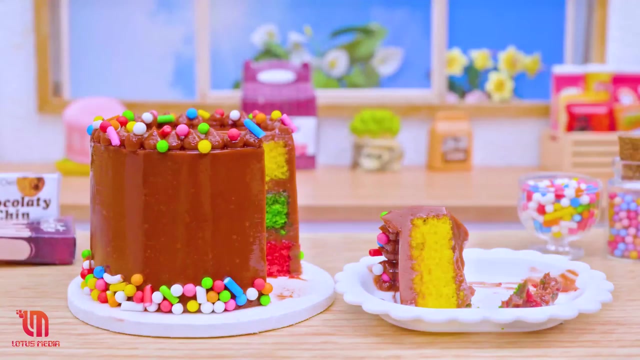 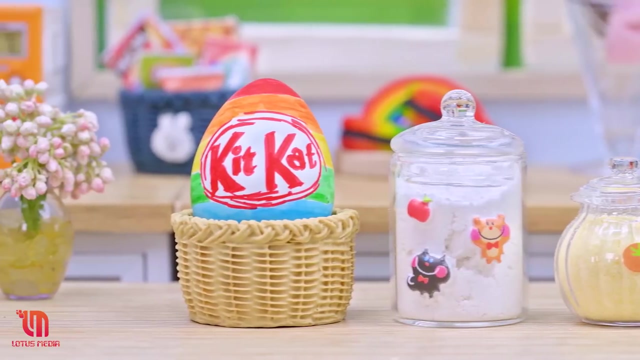 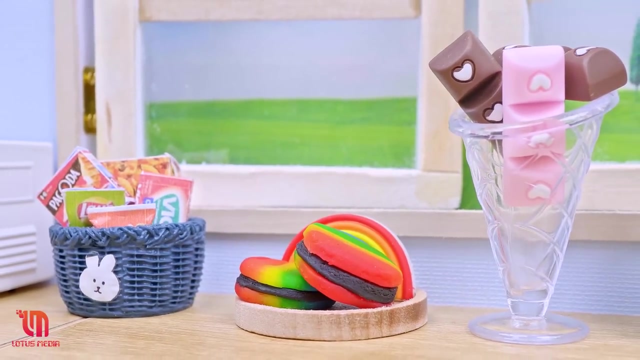 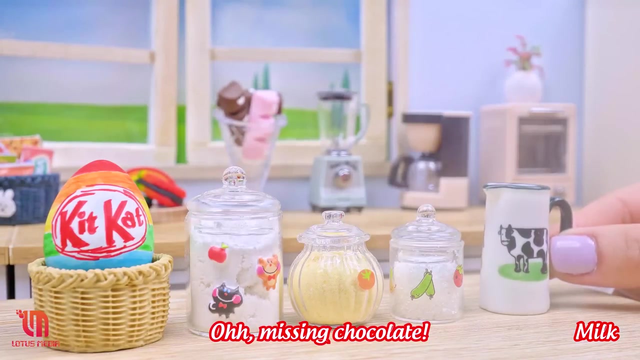 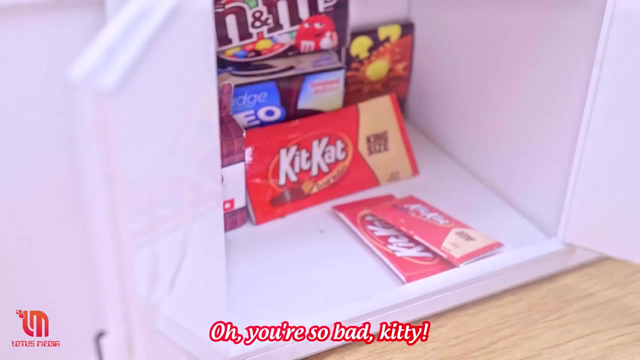 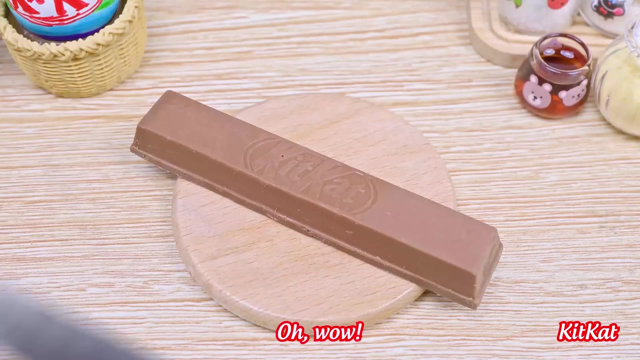 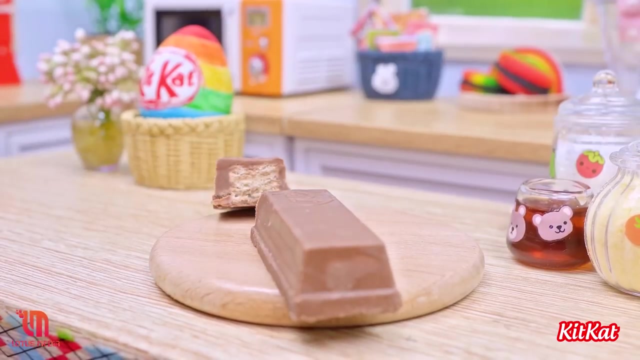 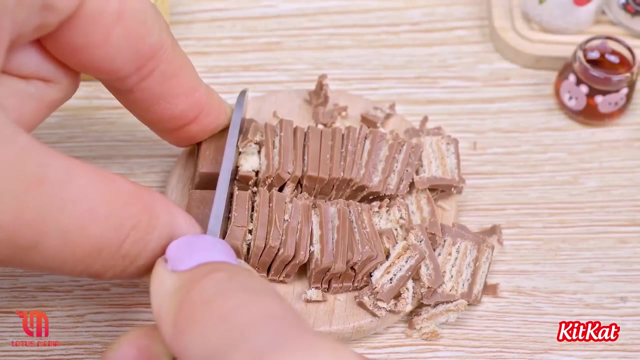 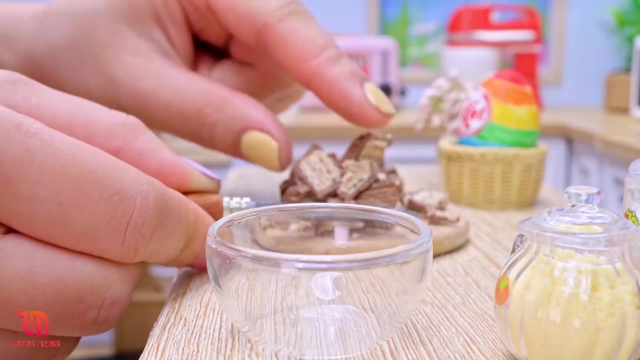 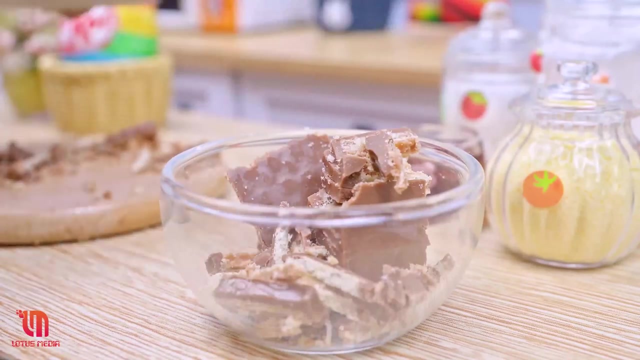 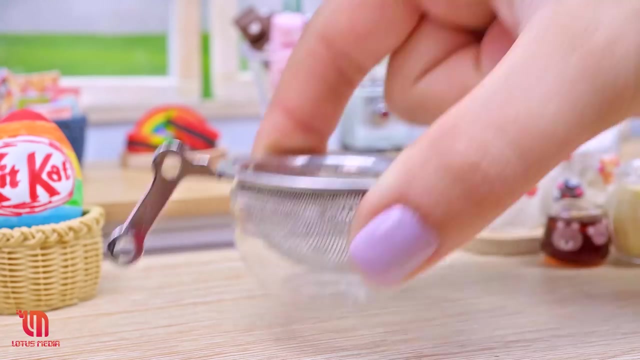 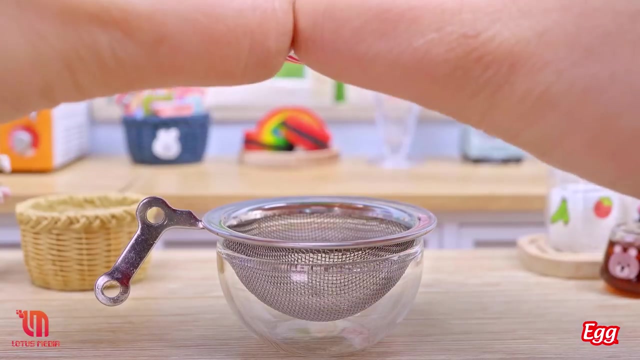 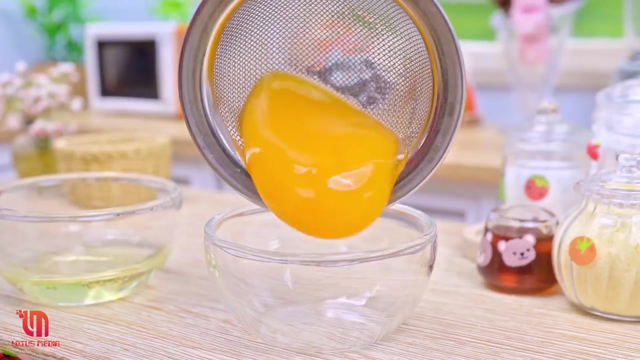 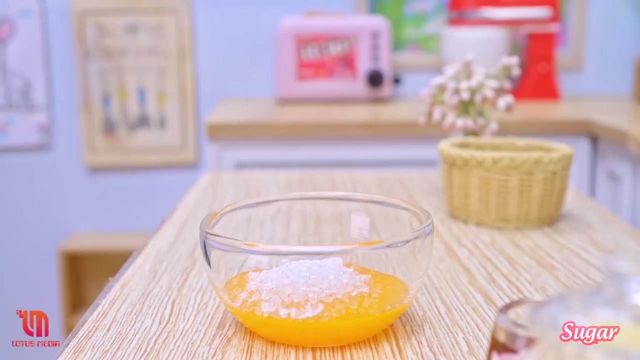 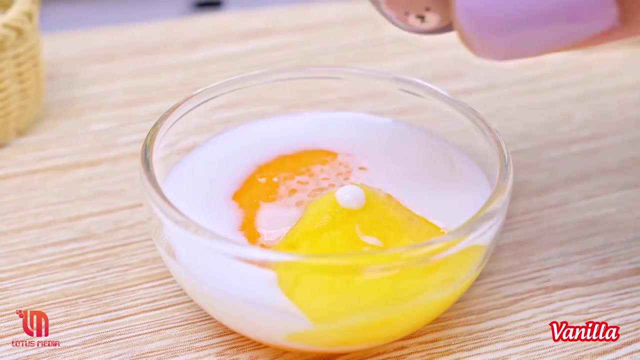 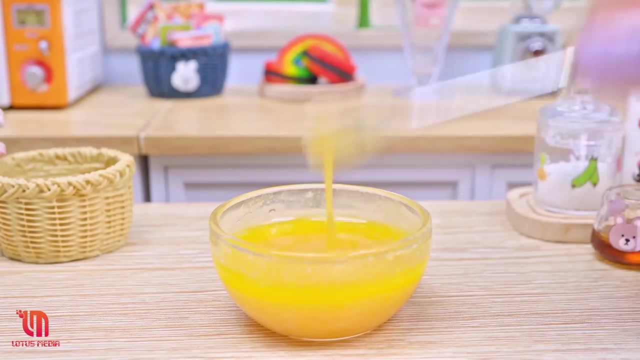 Let's do it. Let's do it. Wow, I love it. Delicious Yummy. Oh, missing chocolate, Oh you're so bad. kitty, Oh wow, Oh you're so bad, Oh you're so bad. 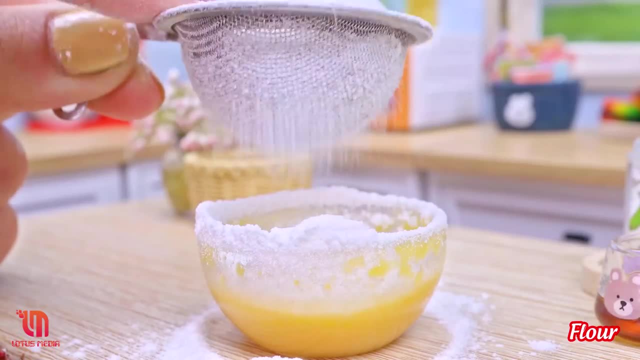 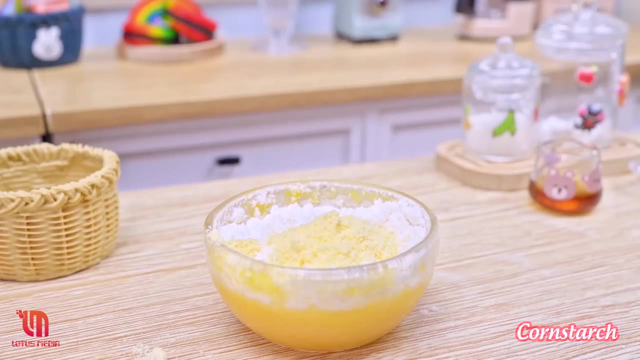 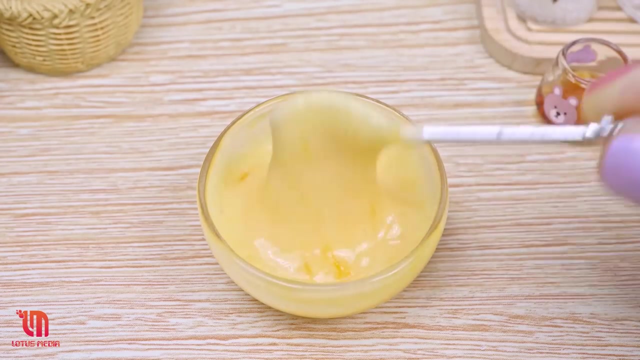 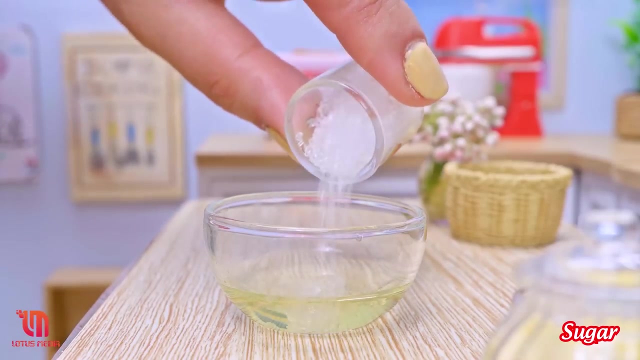 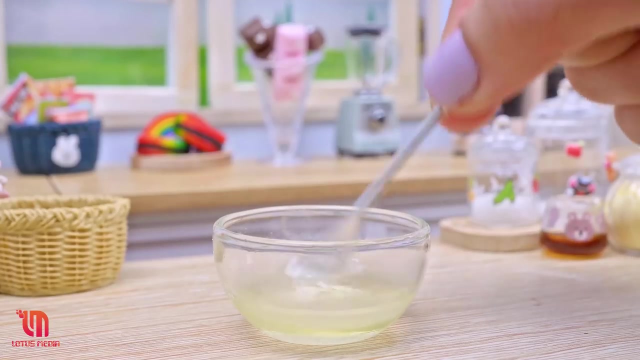 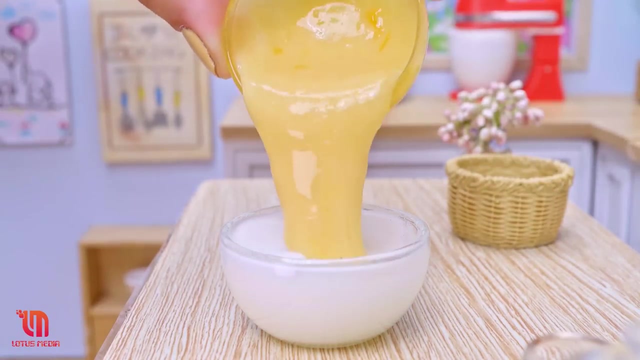 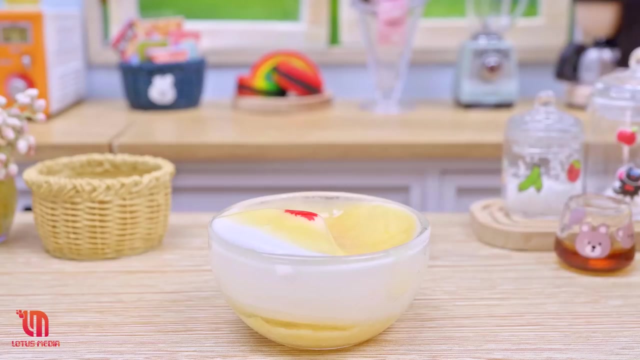 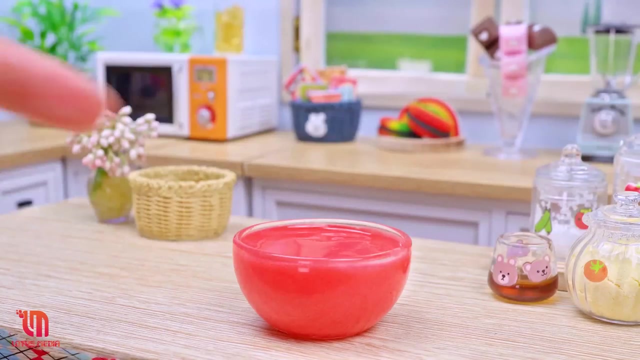 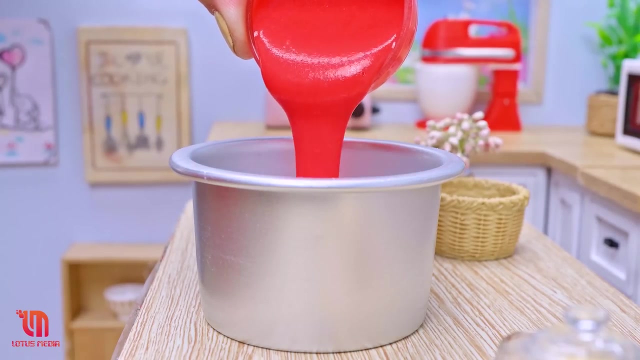 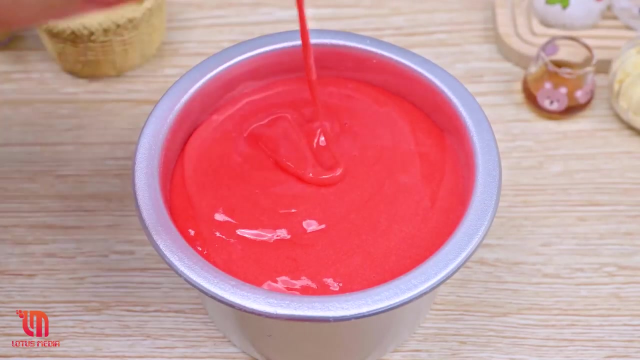 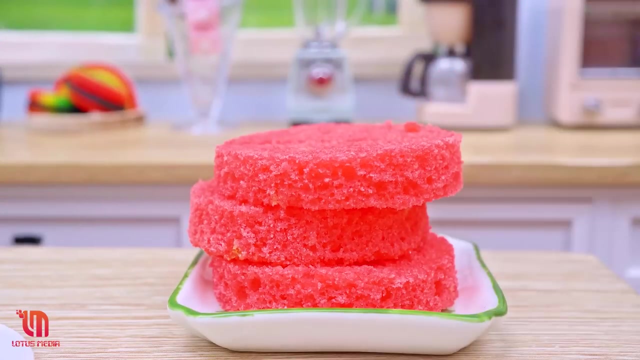 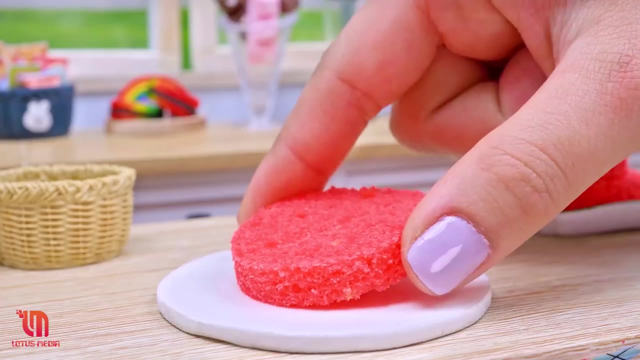 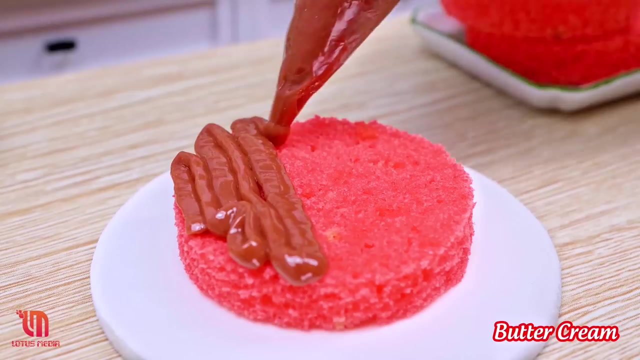 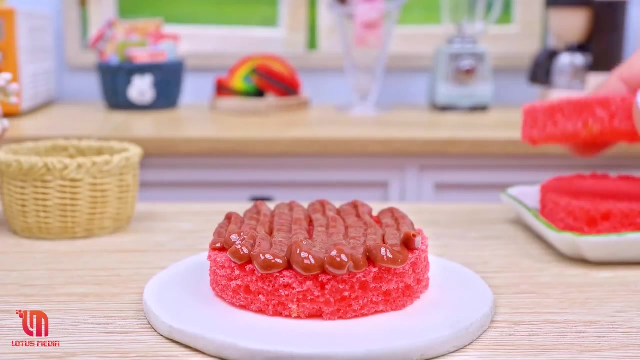 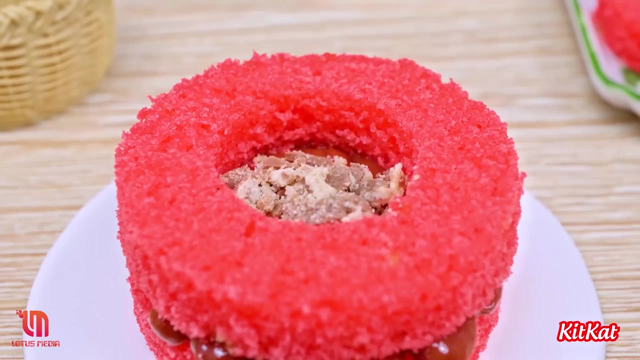 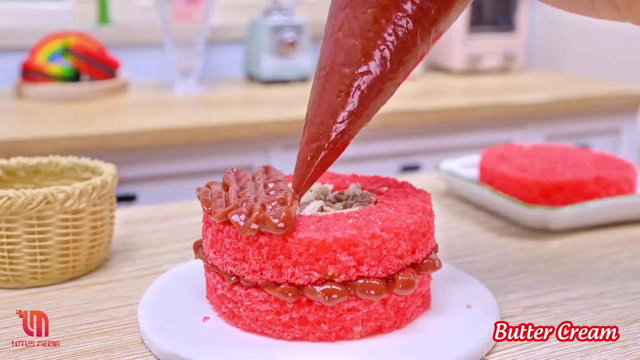 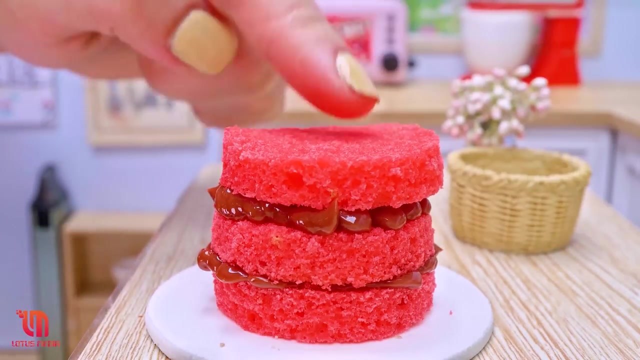 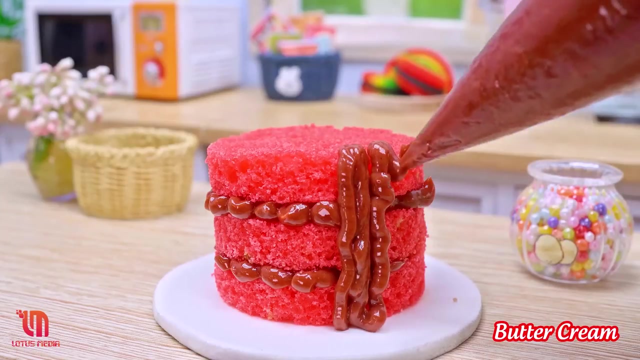 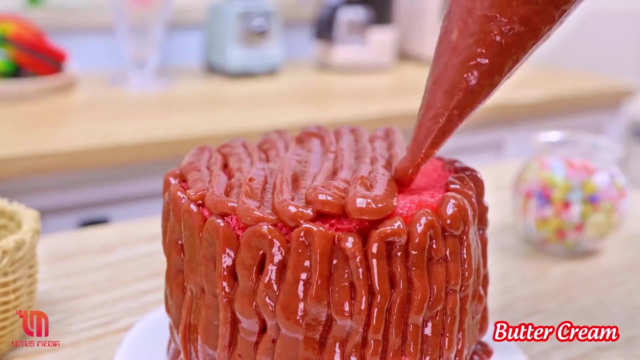 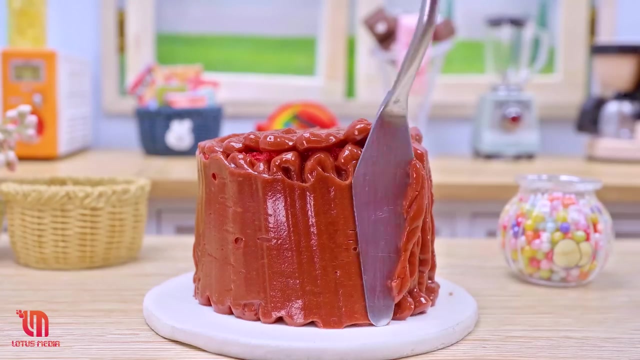 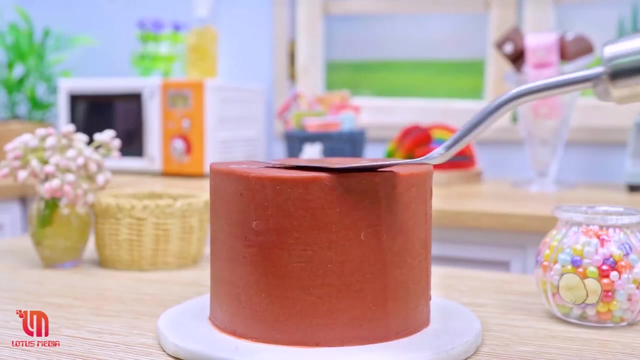 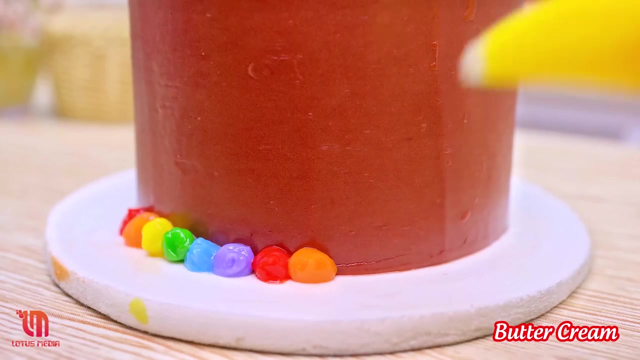 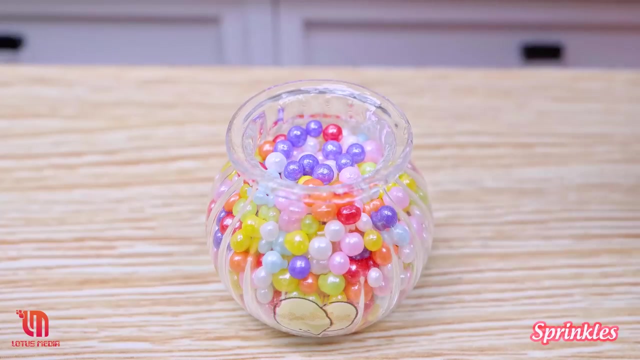 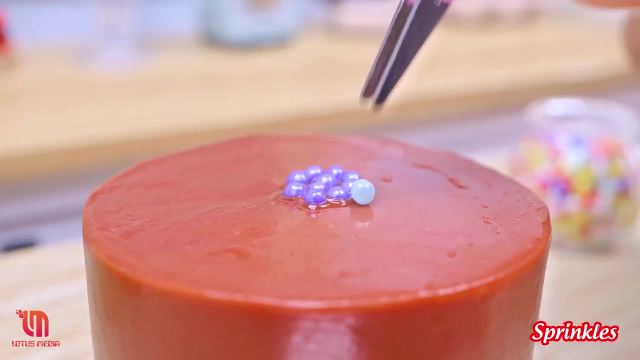 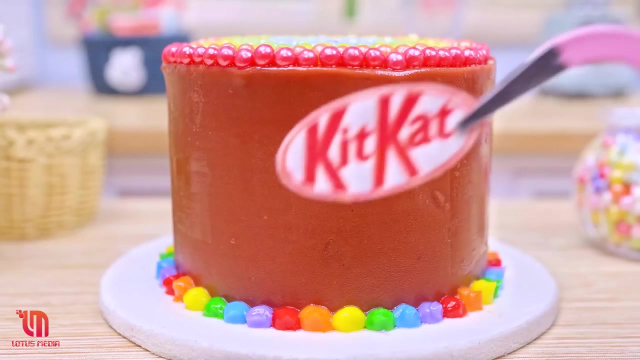 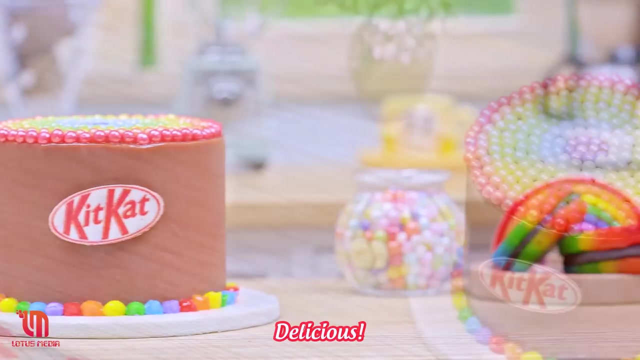 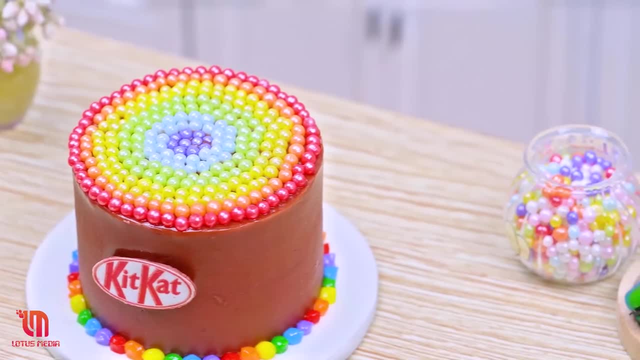 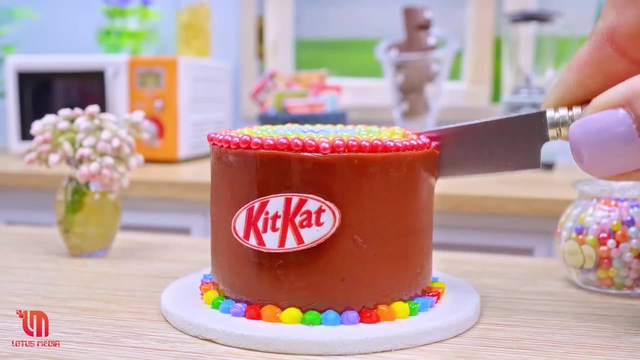 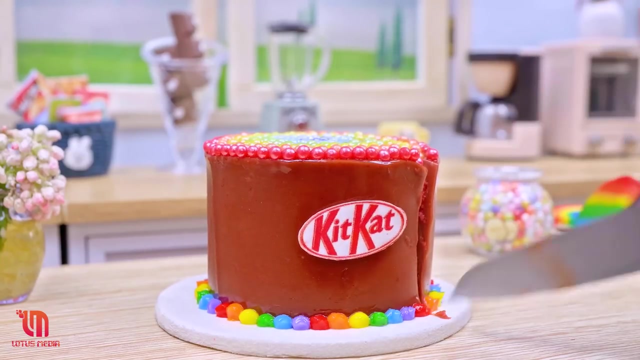 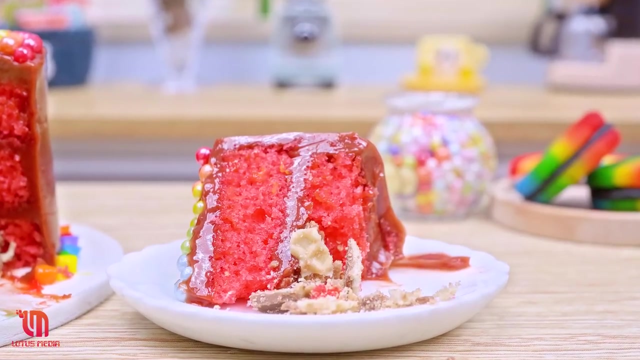 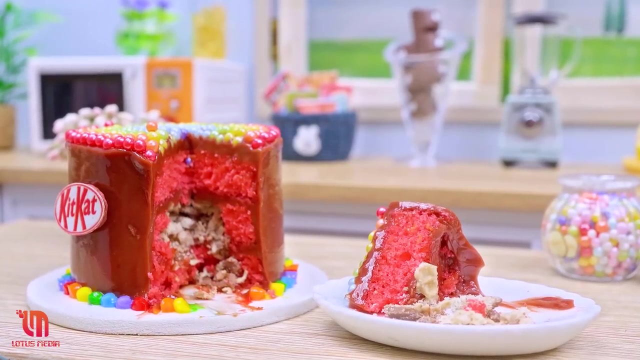 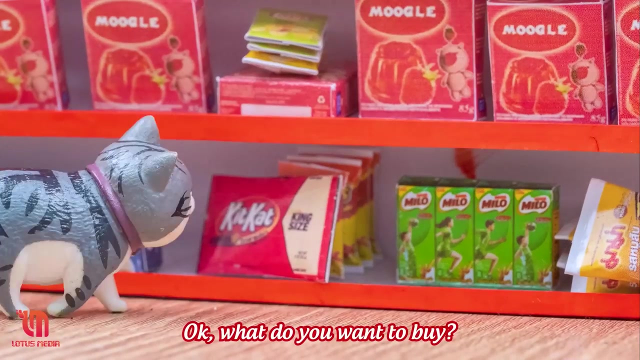 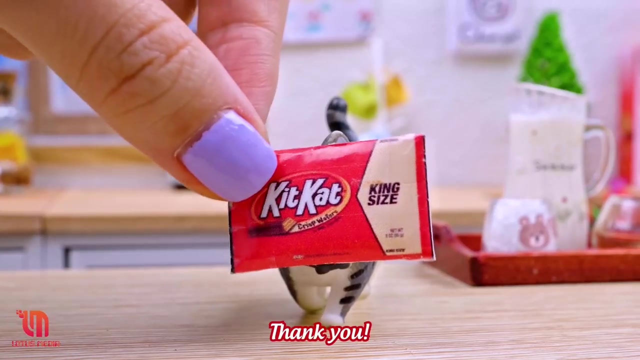 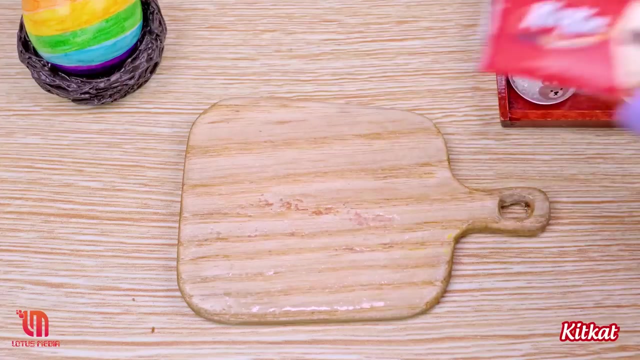 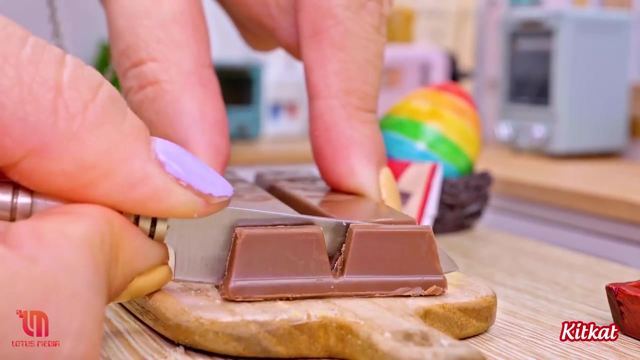 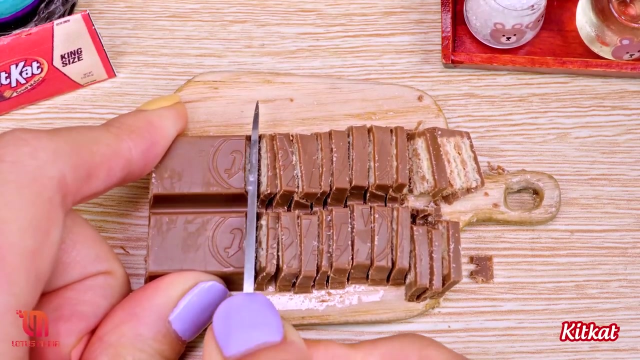 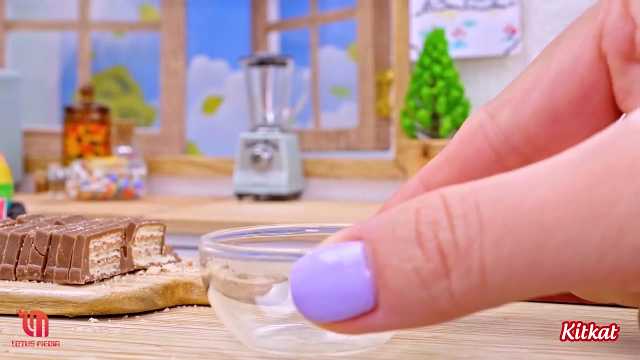 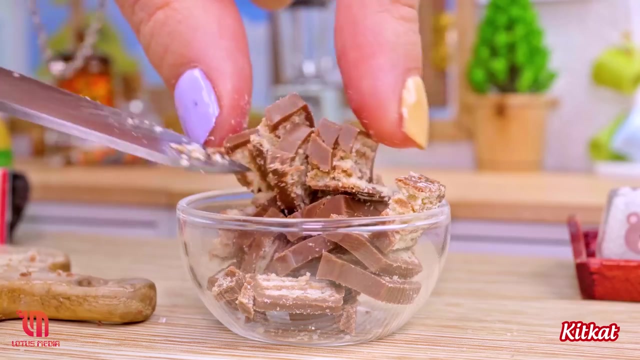 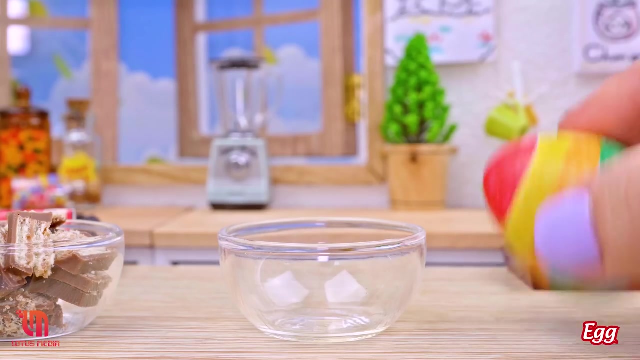 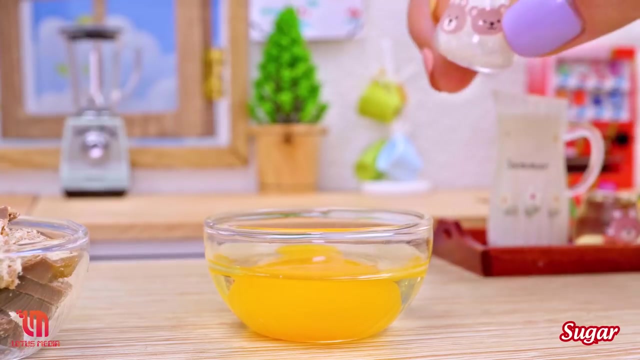 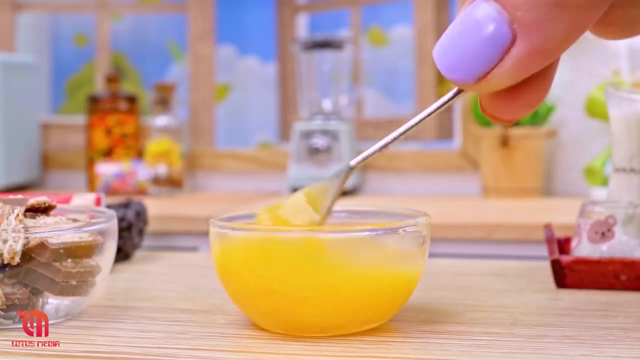 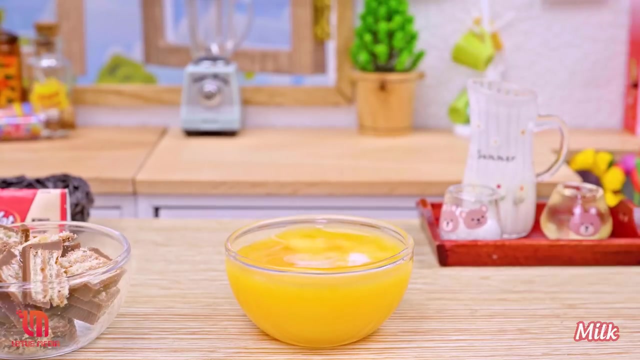 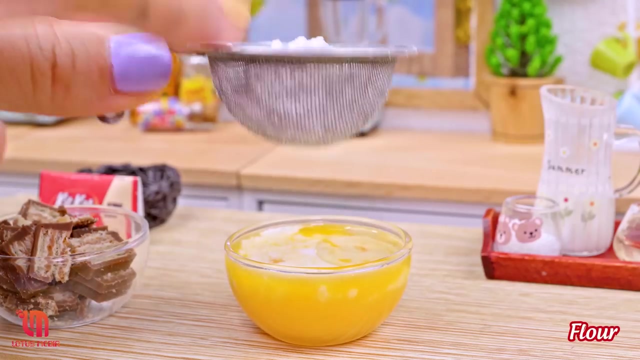 Oh, you're so bad Tasty, Wow, Wow, Wow, Yummy. Okay, what do you want to buy? Oh, good boy, Thank you, Good job. Oh wow, Oh wow, Oh wow. 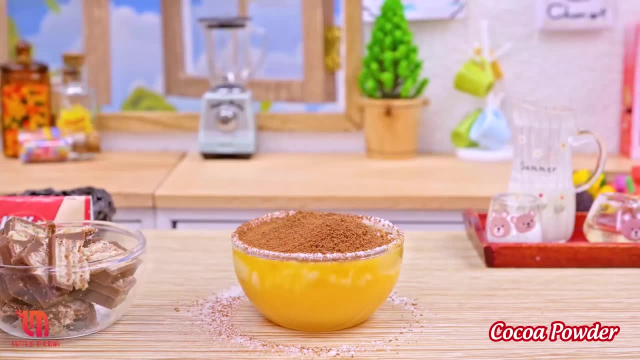 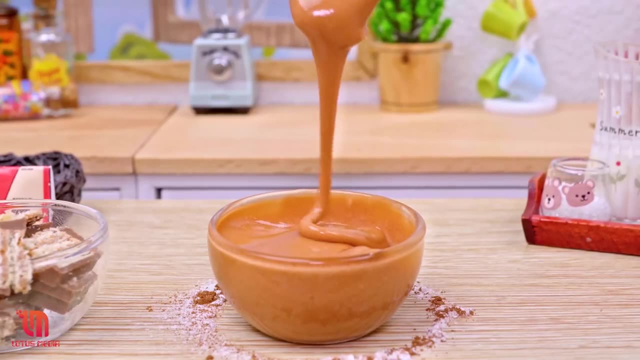 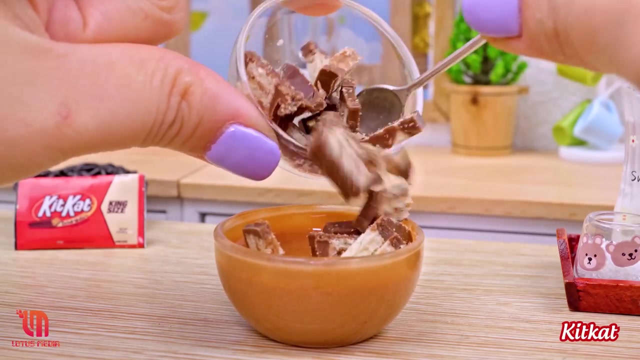 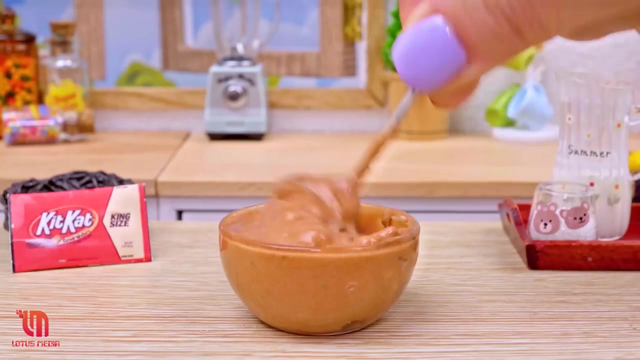 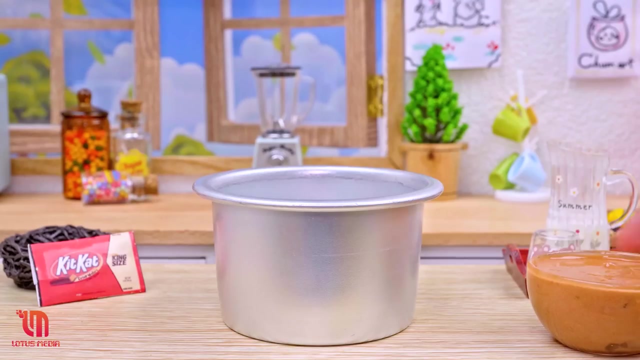 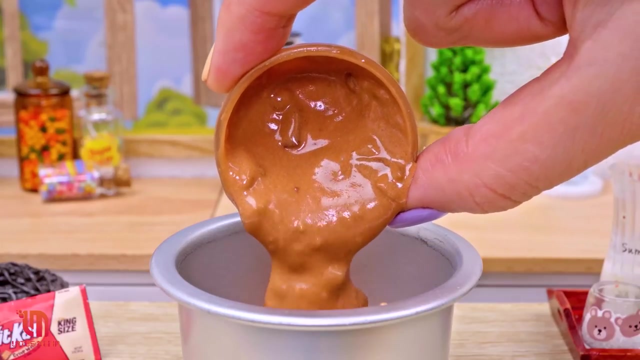 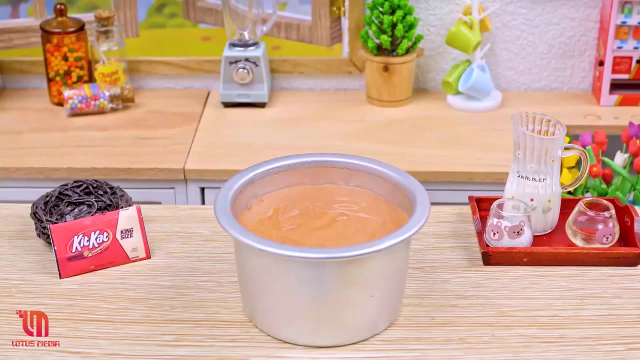 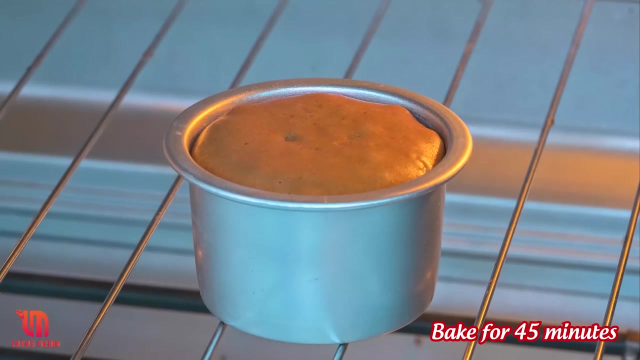 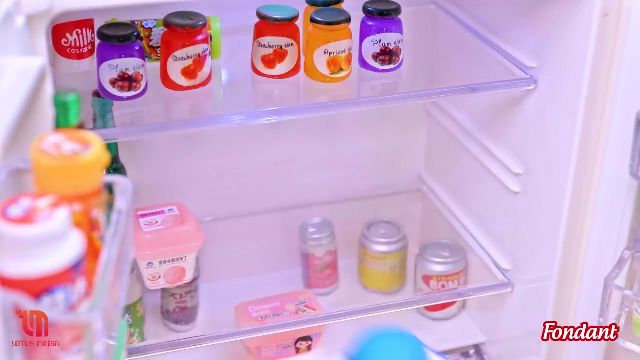 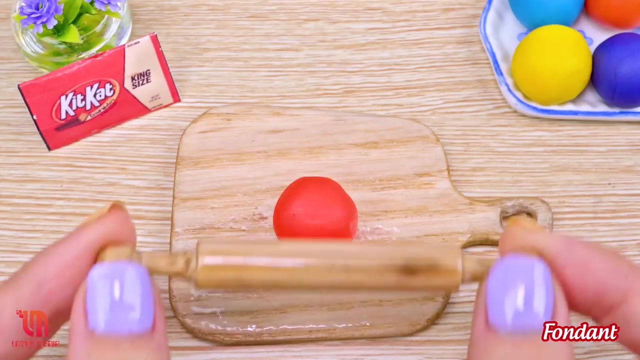 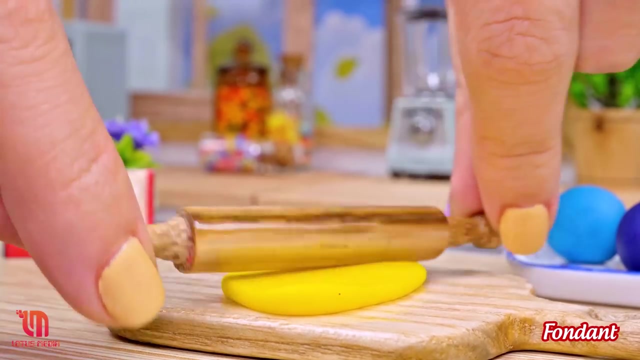 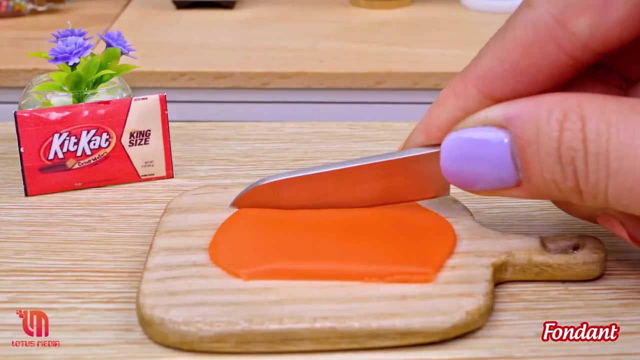 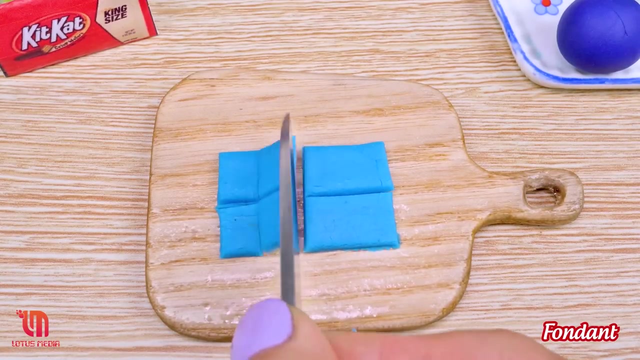 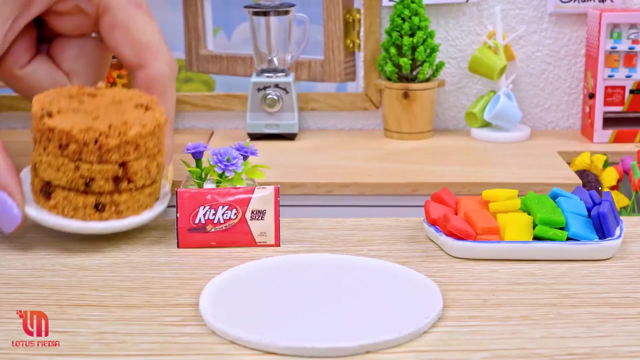 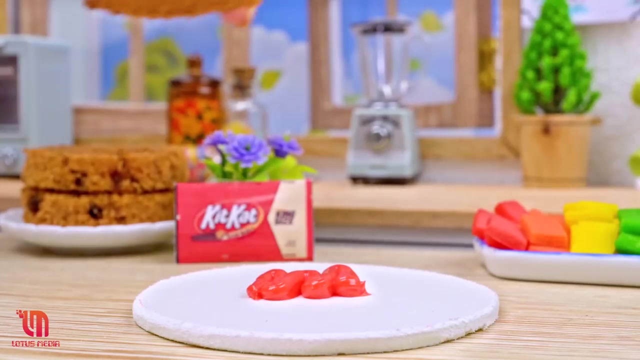 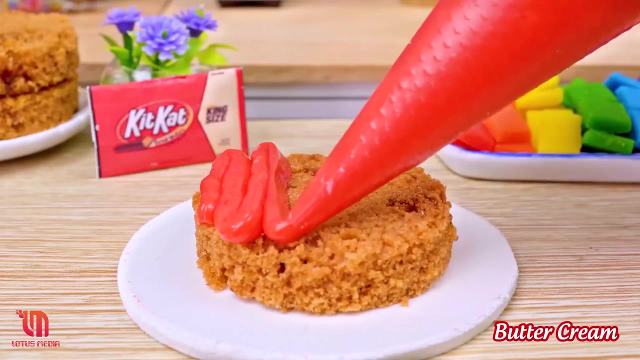 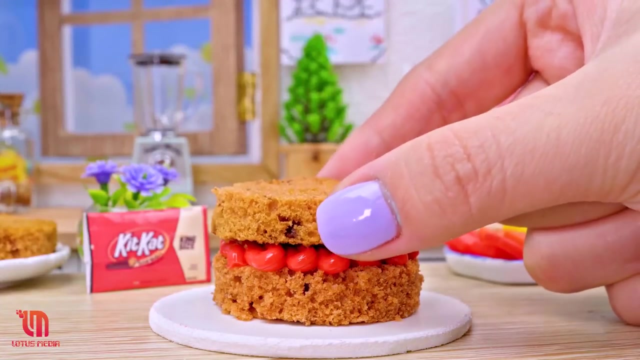 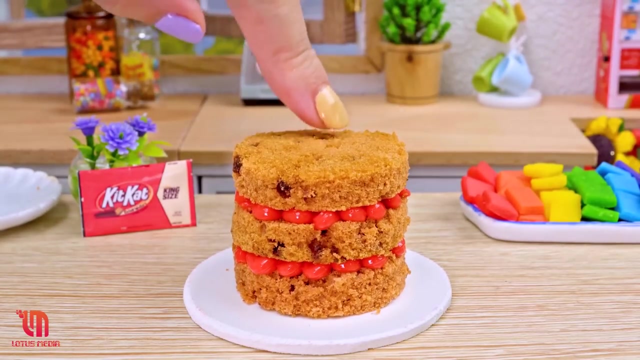 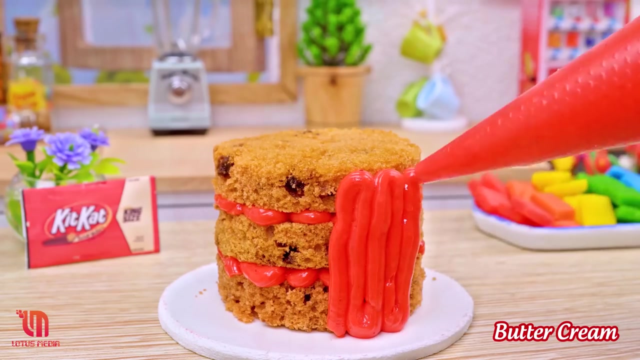 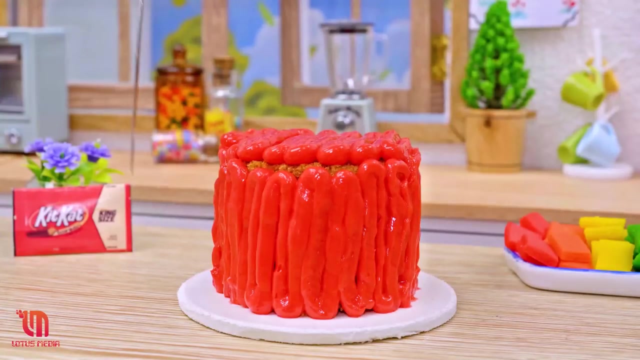 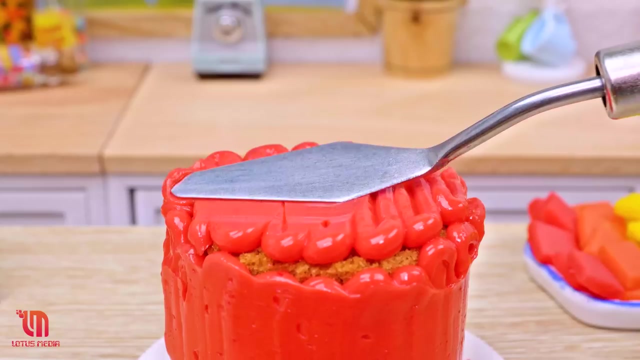 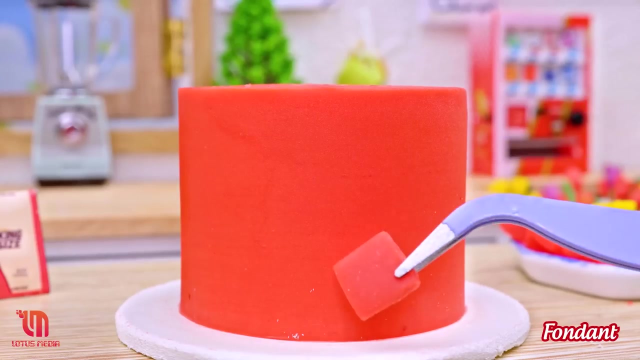 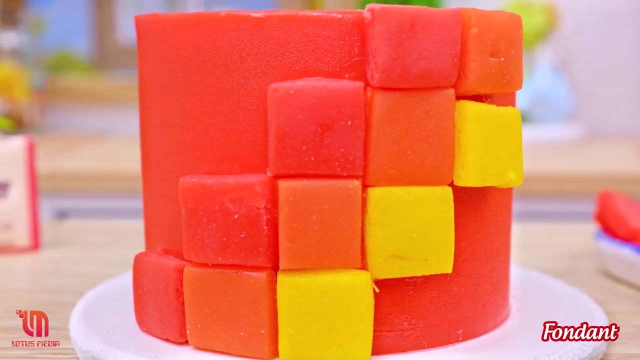 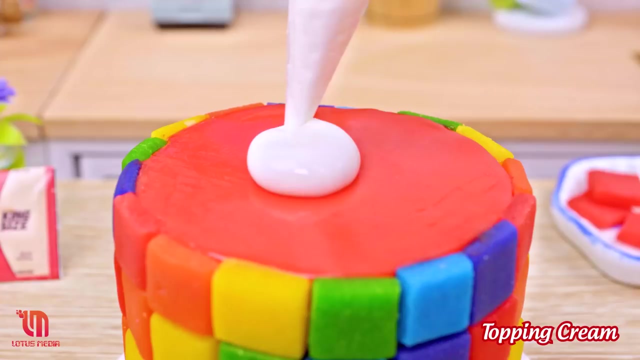 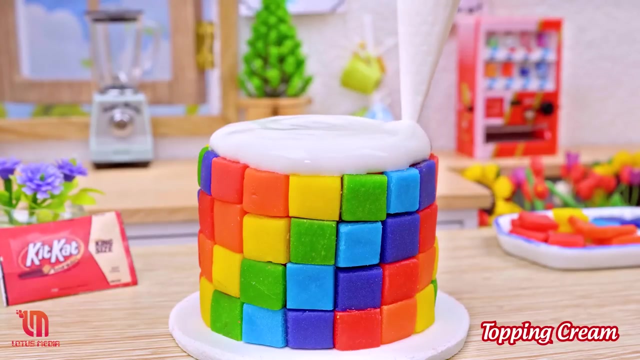 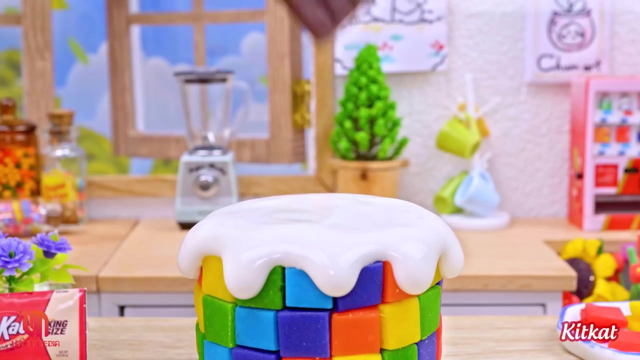 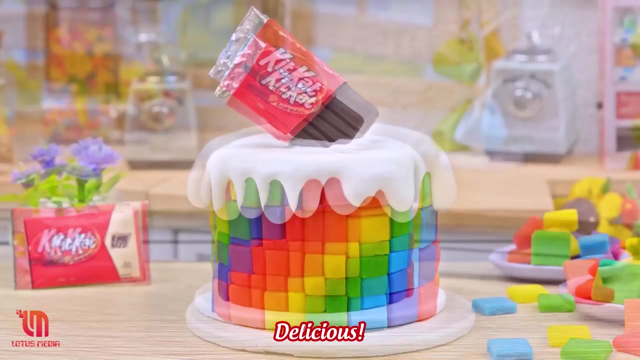 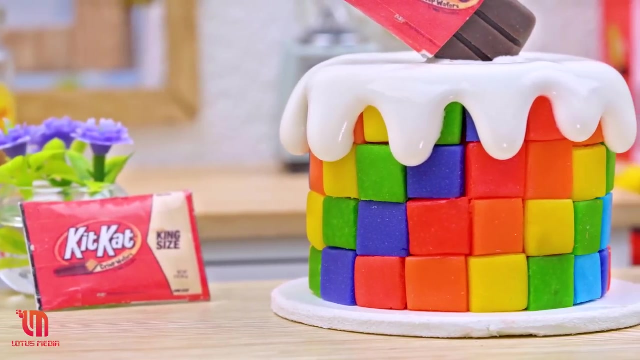 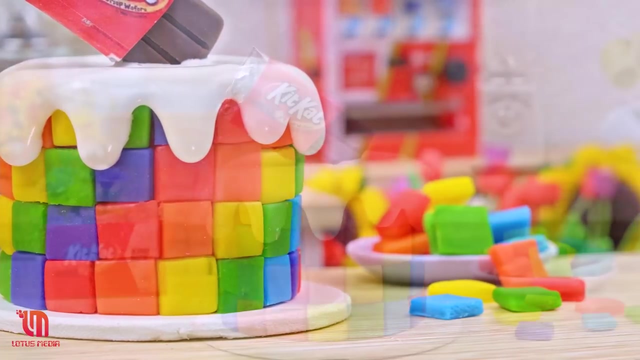 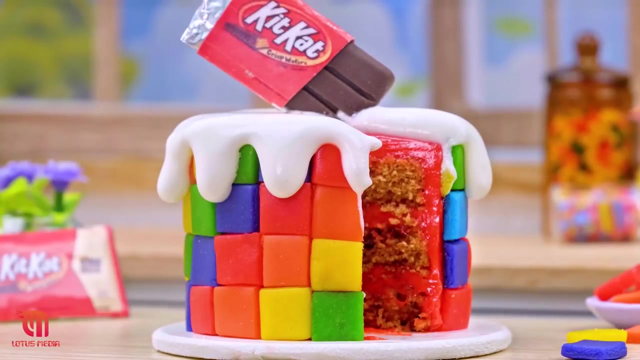 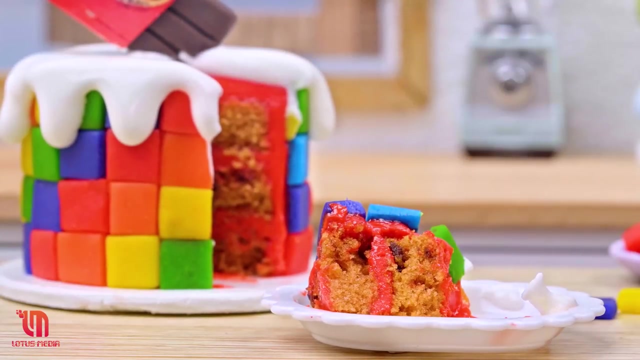 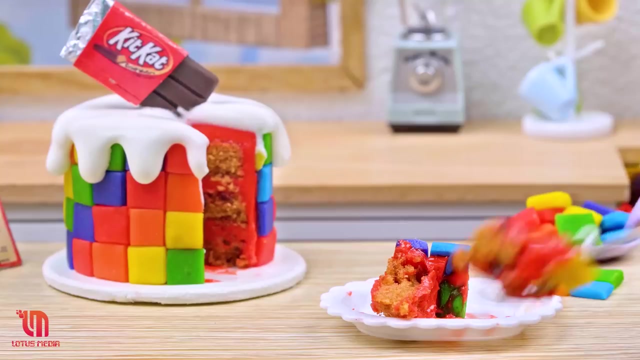 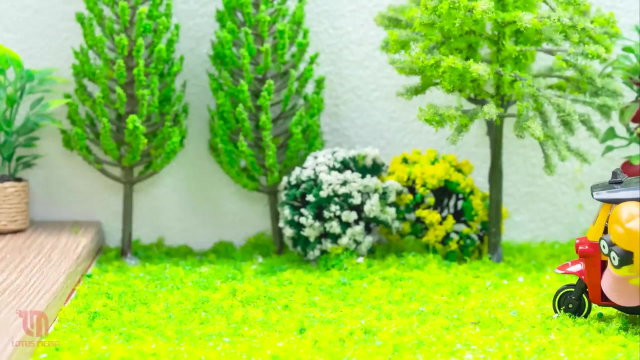 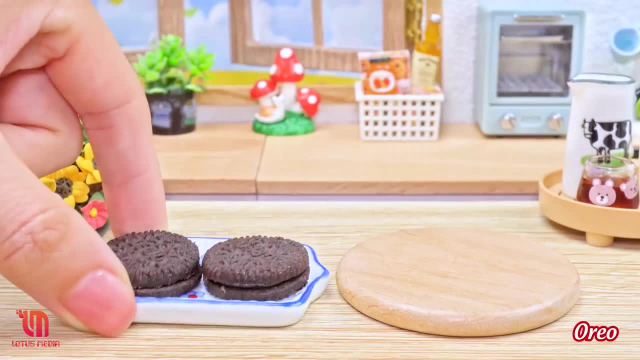 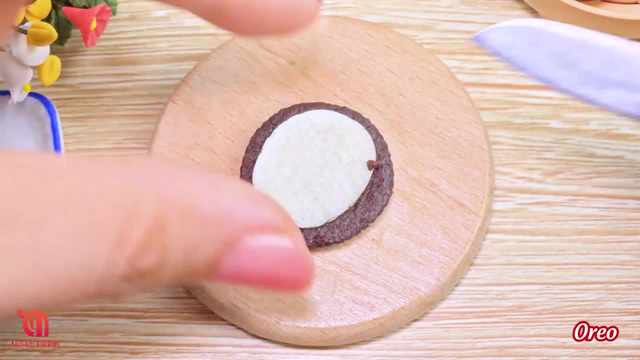 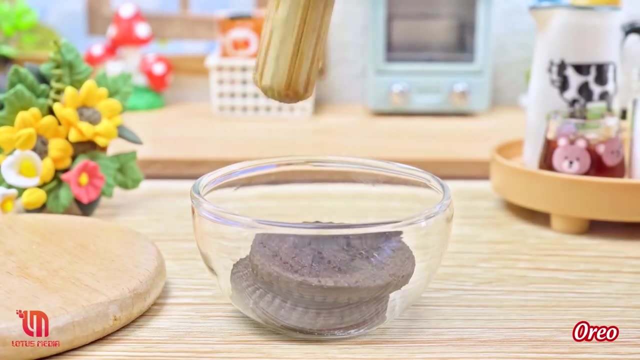 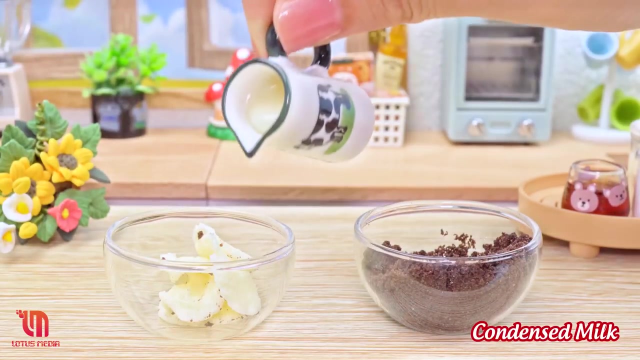 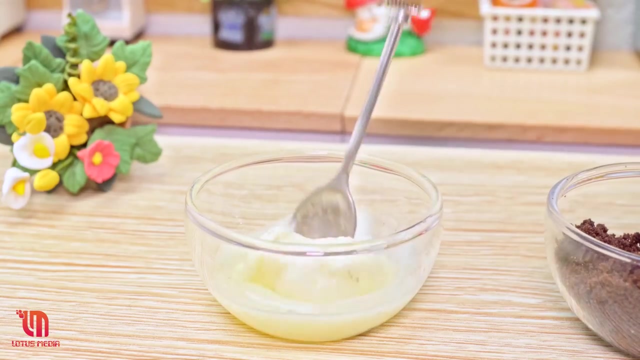 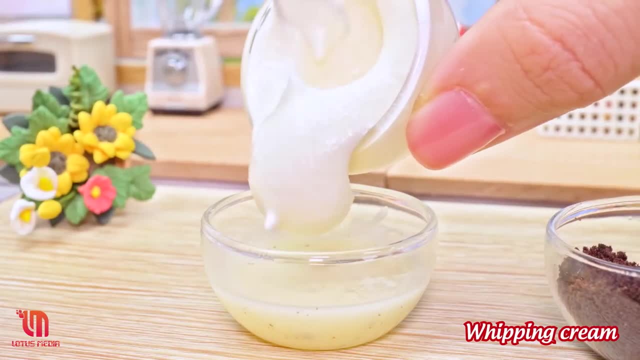 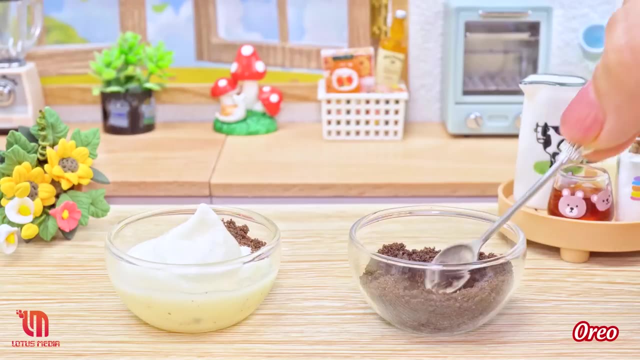 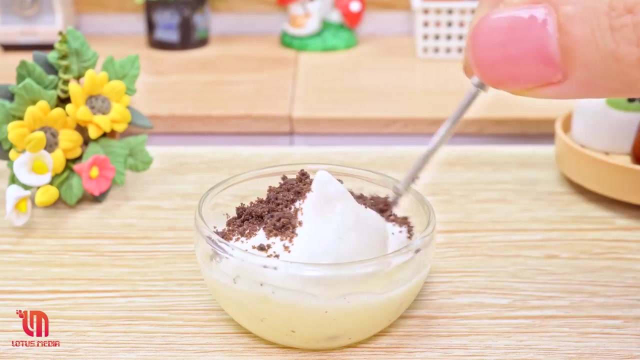 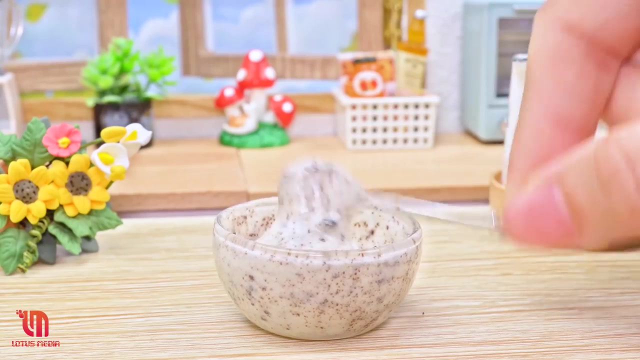 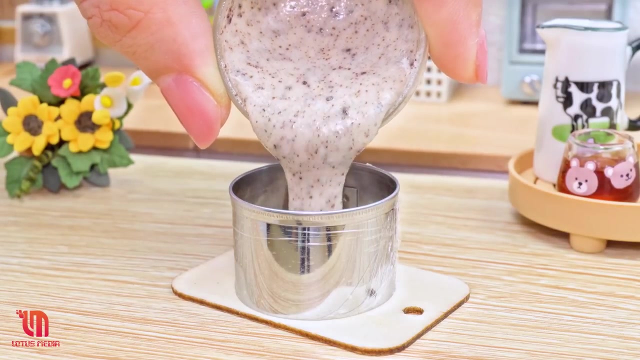 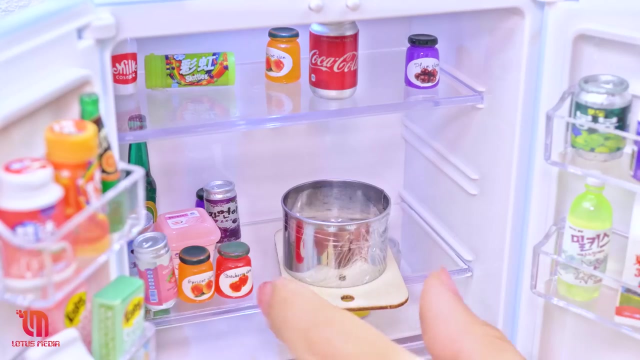 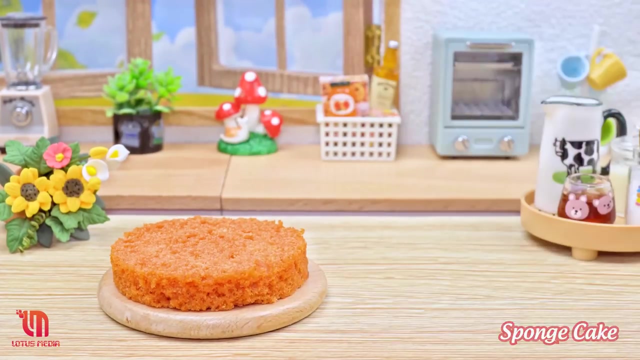 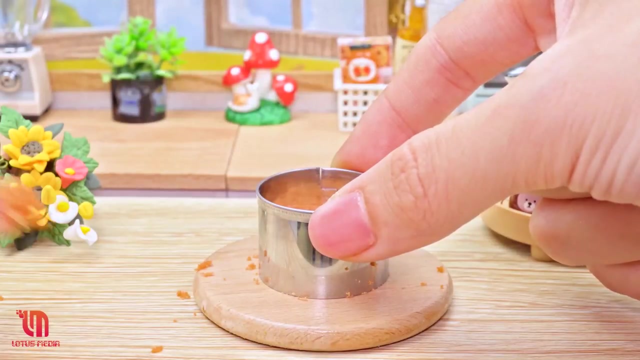 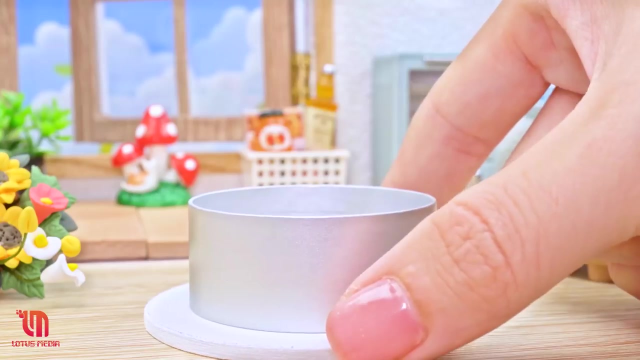 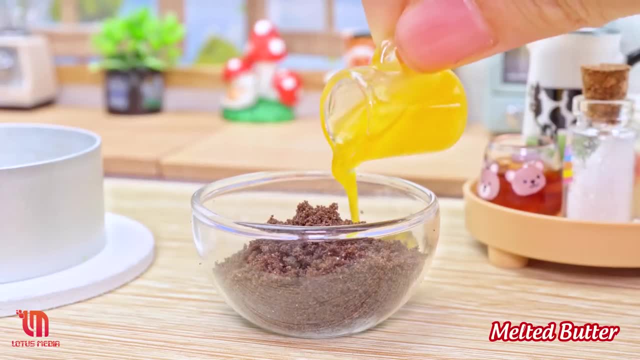 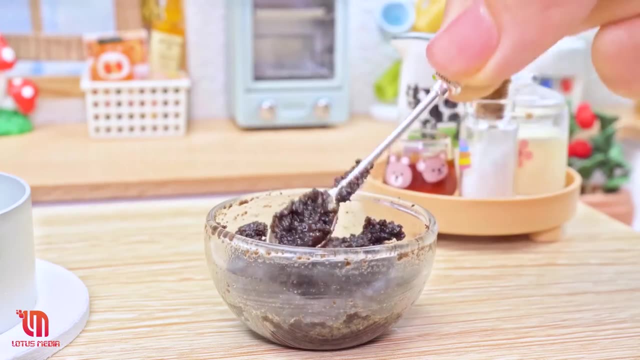 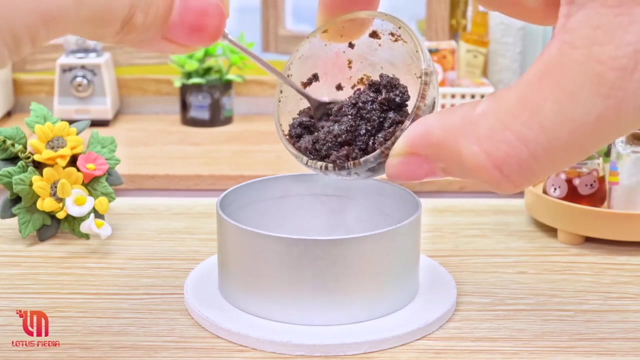 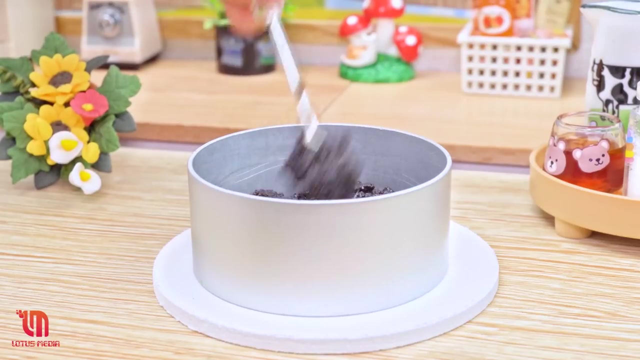 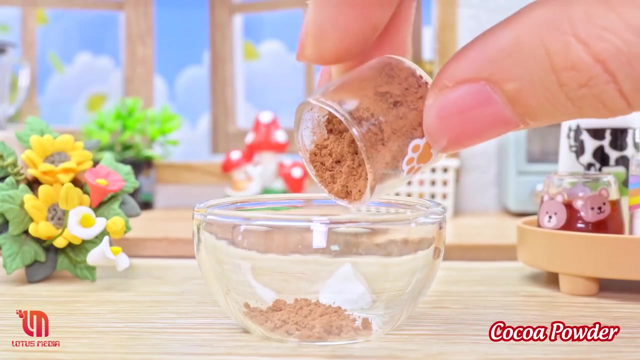 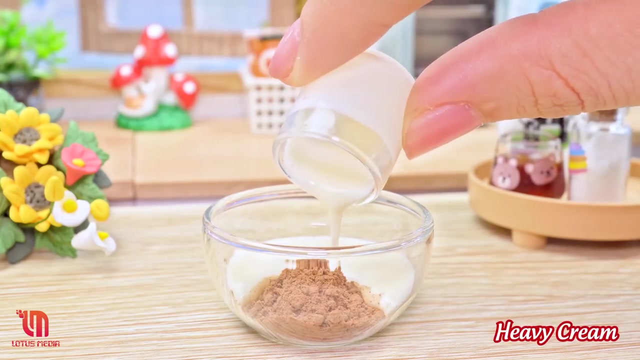 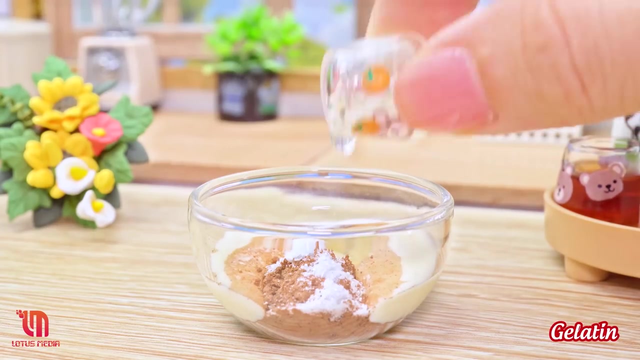 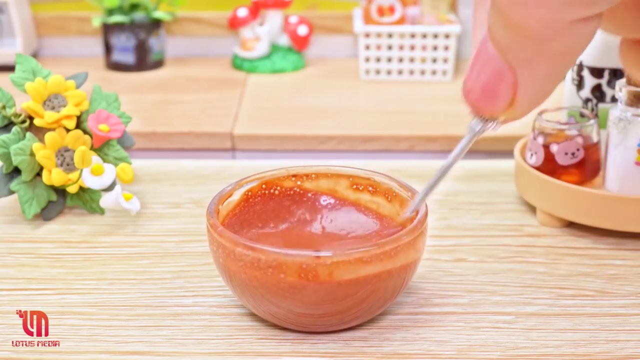 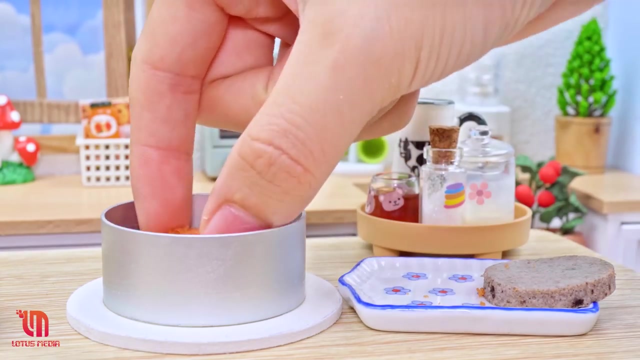 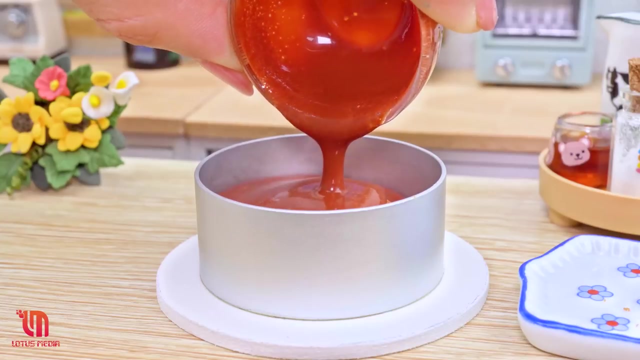 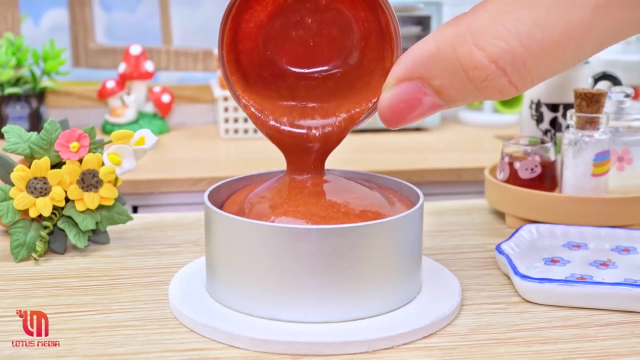 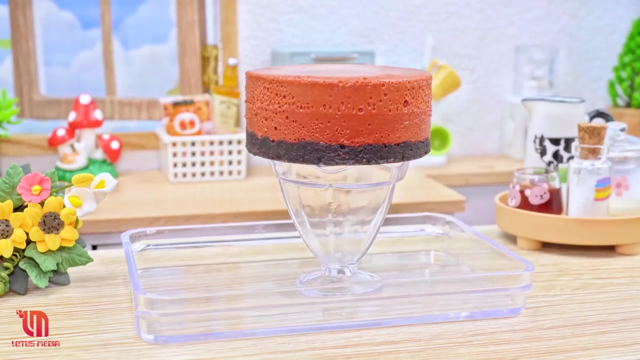 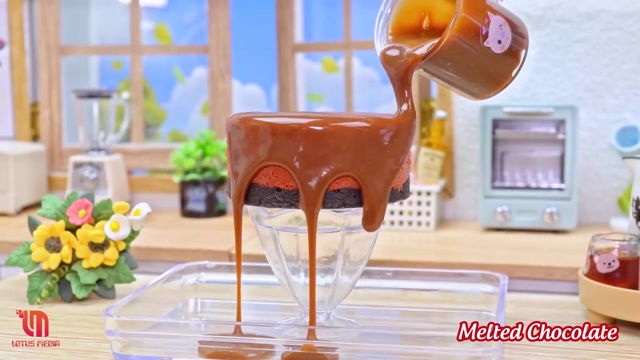 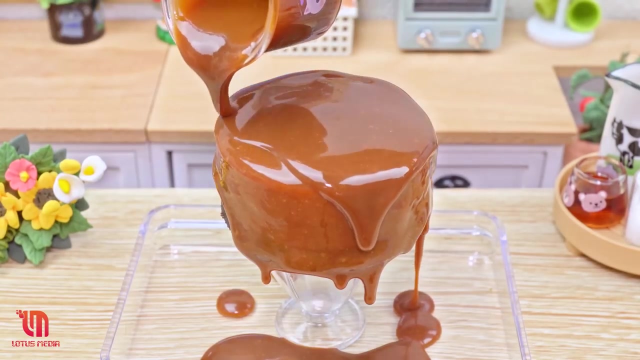 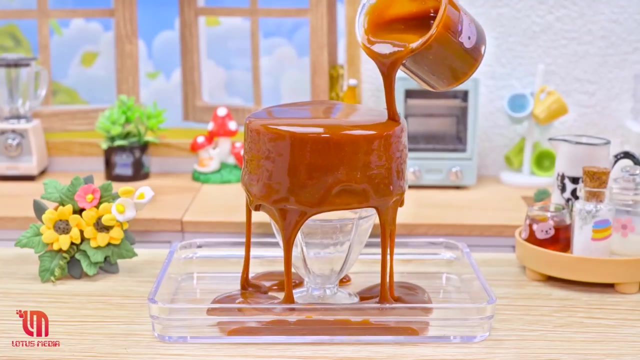 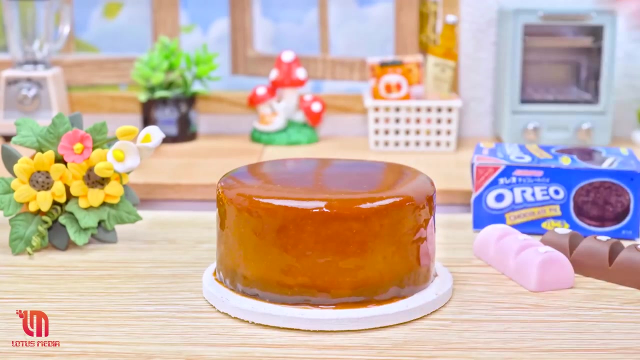 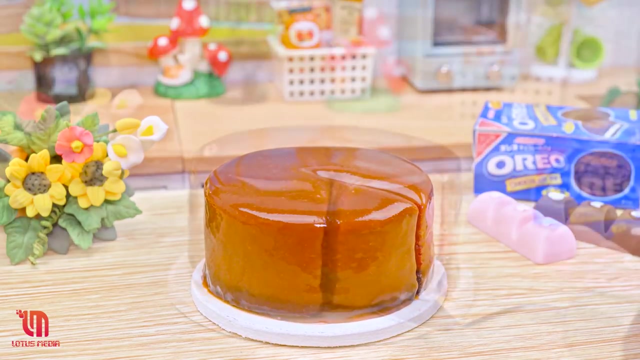 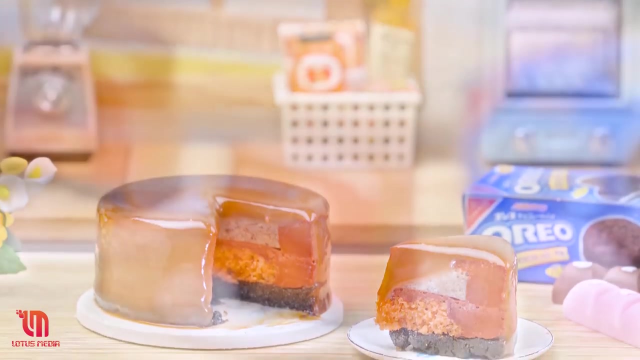 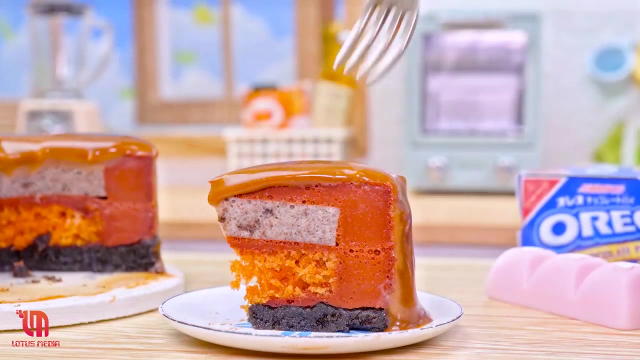 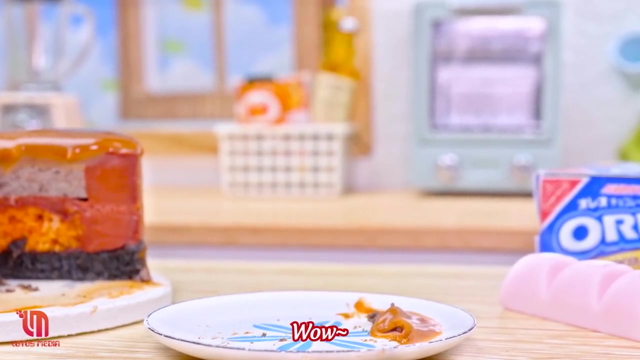 I will make a cake with this. I will make a cake with this. I'm going to make a fried egg roll. I'm going to make fried eggs. I'm going to make fried eggs. I'm going to make fried eggs Sweet. 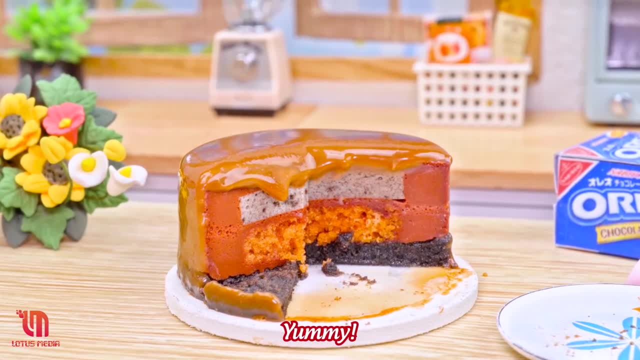 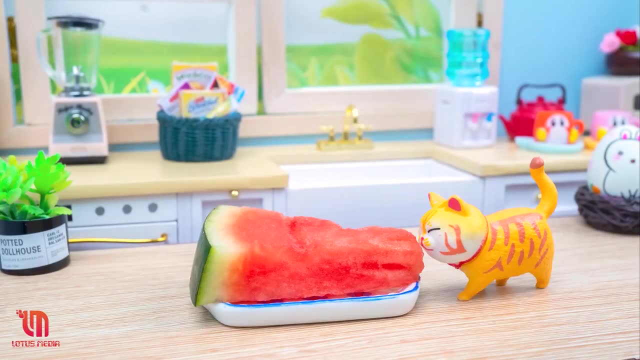 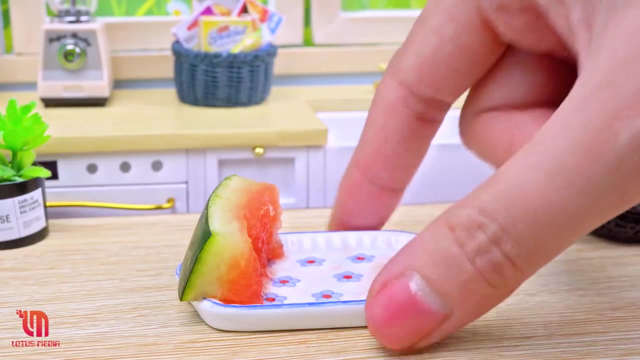 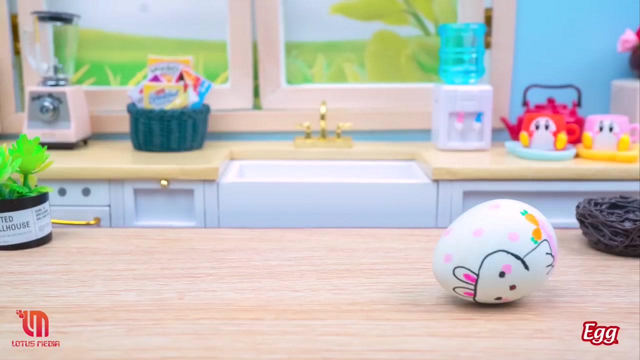 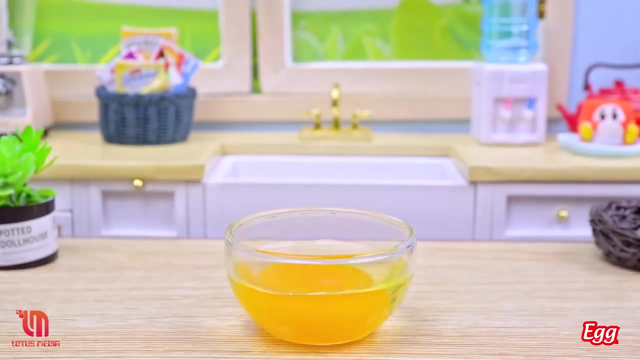 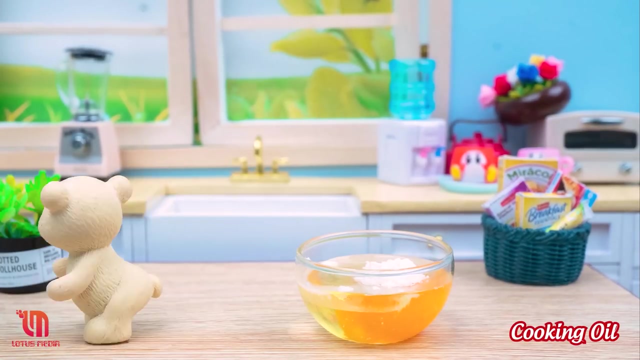 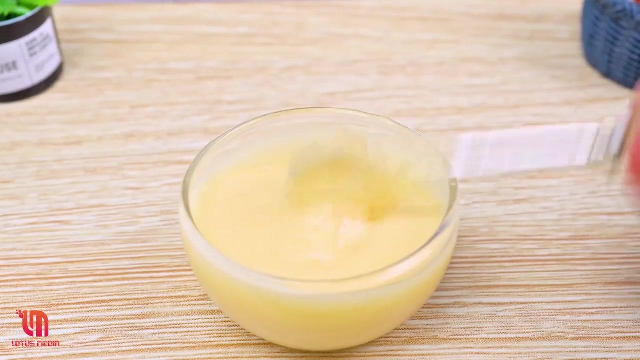 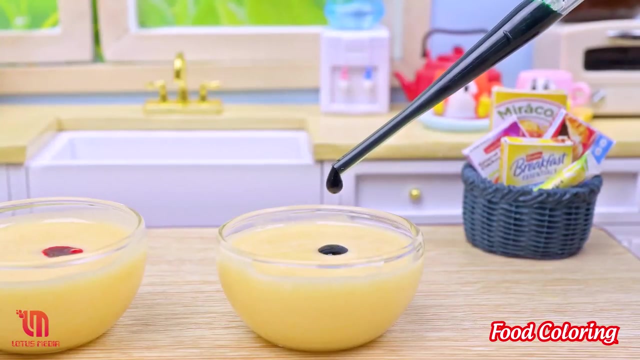 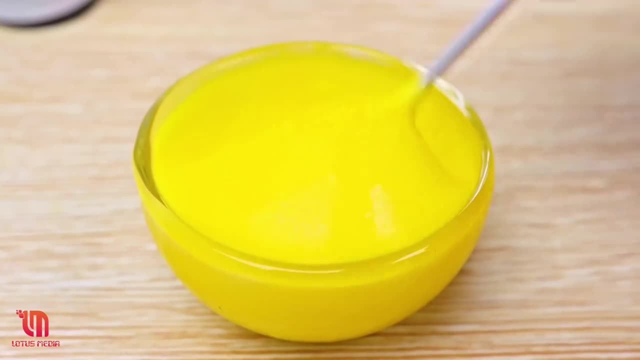 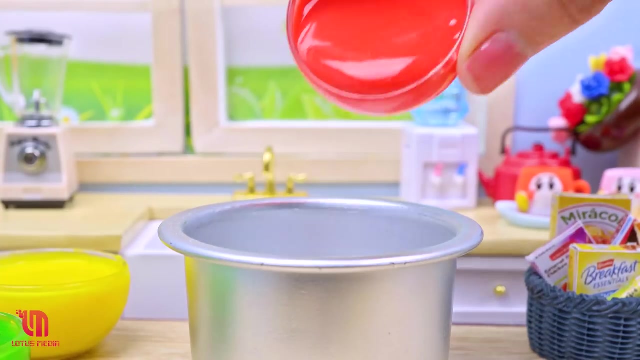 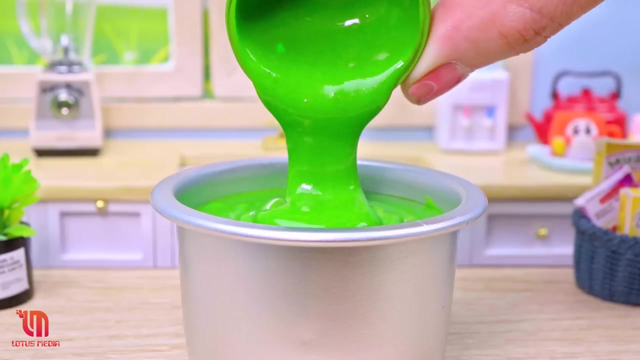 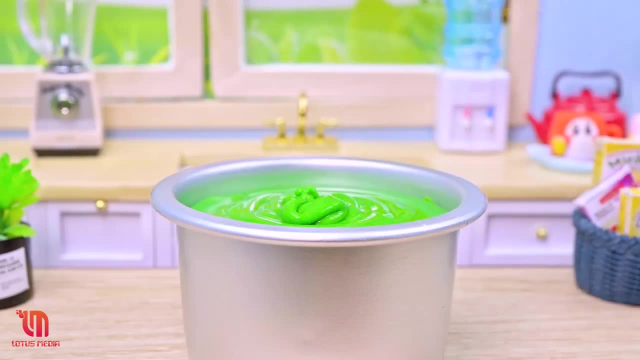 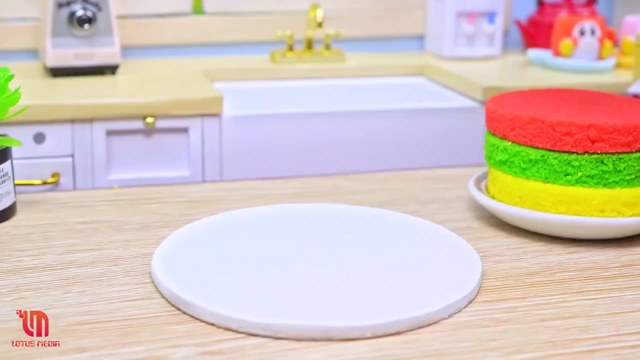 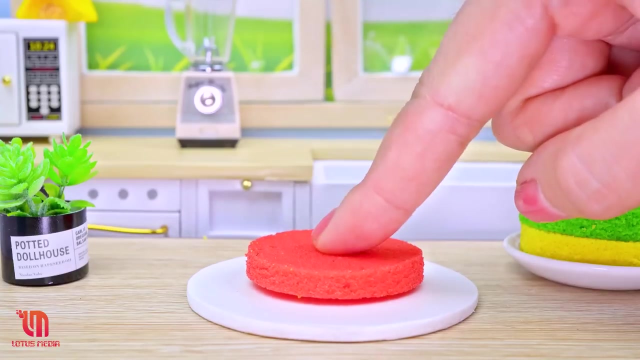 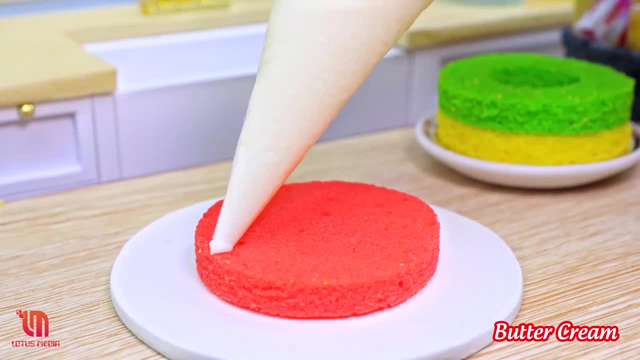 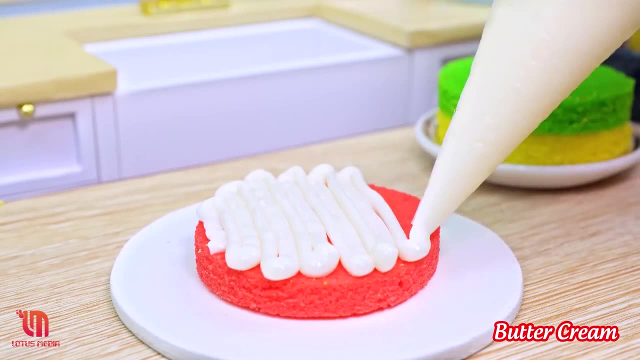 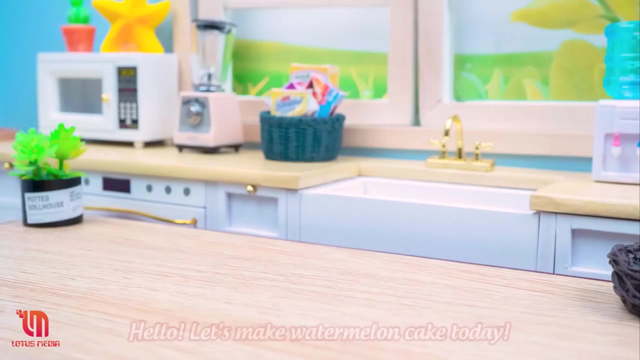 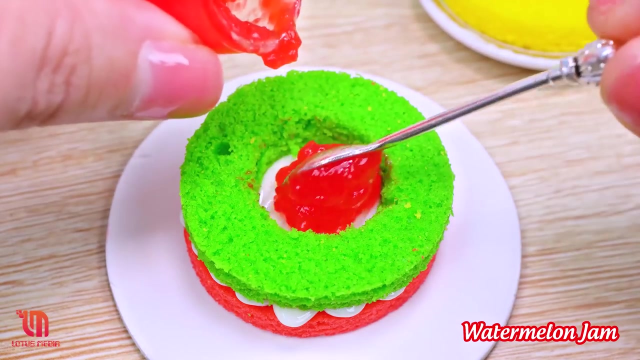 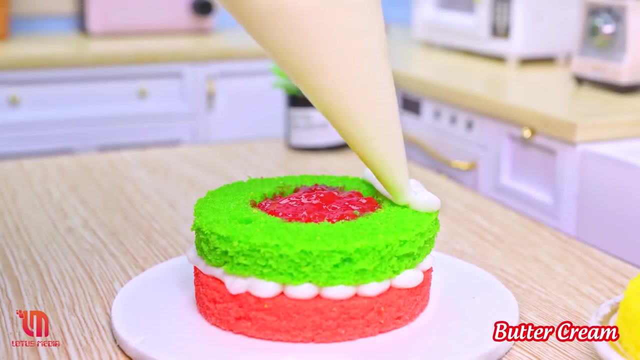 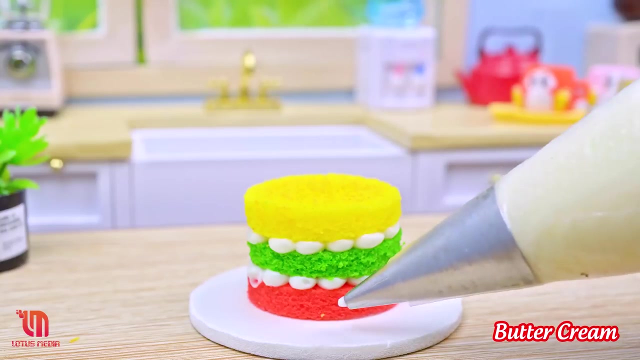 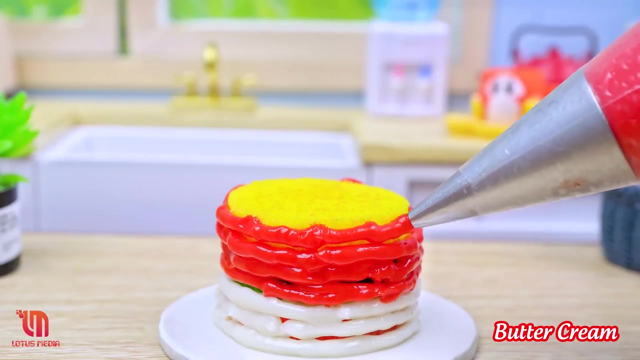 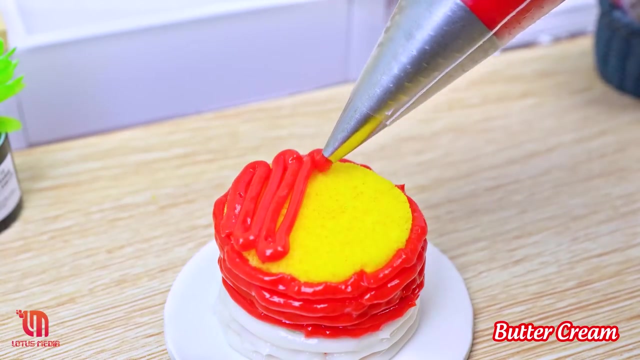 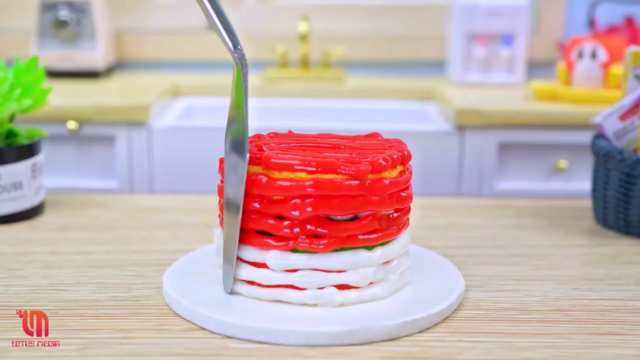 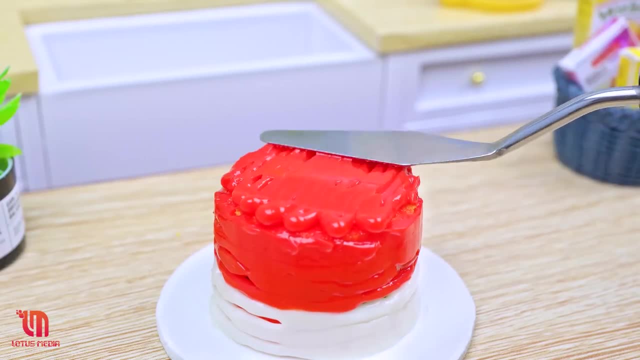 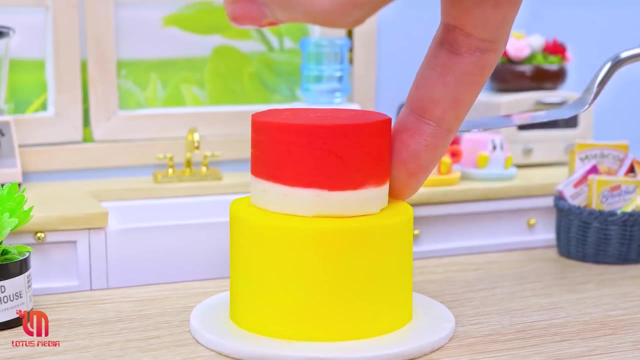 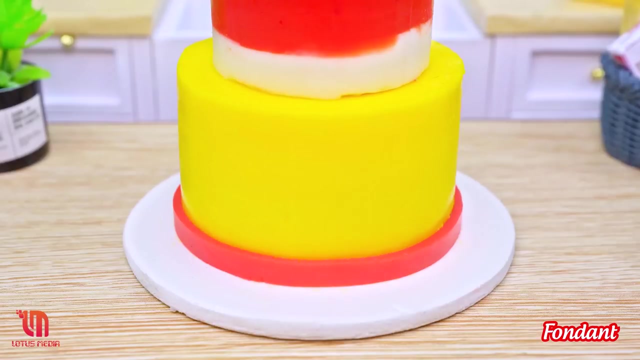 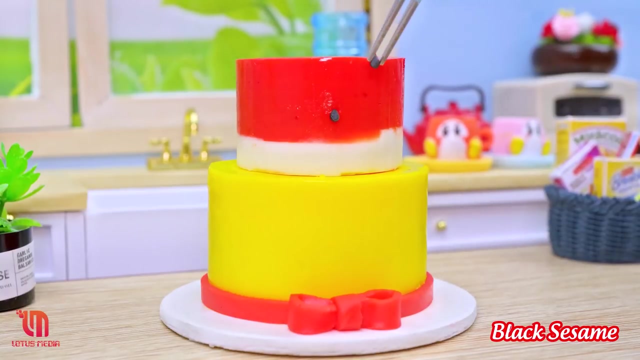 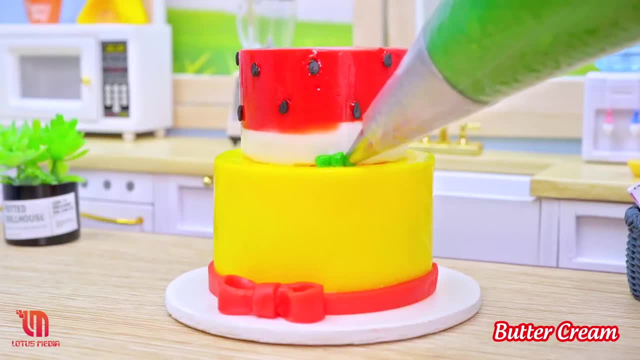 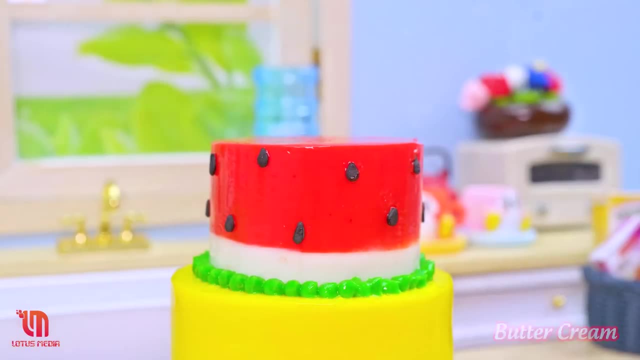 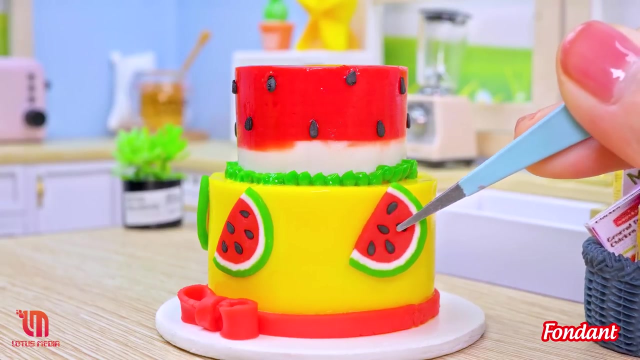 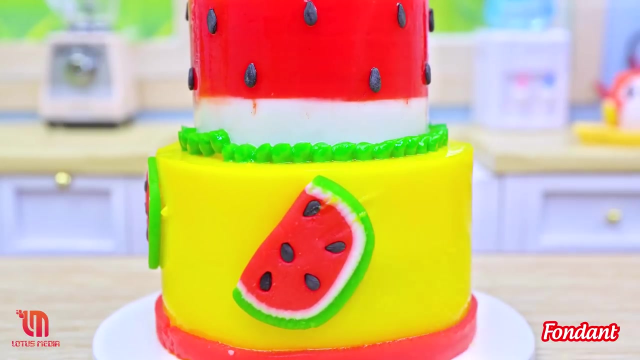 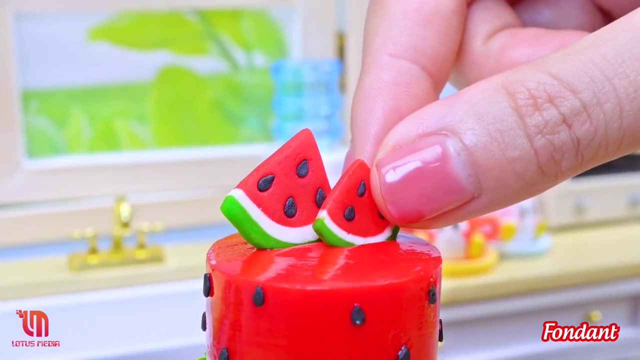 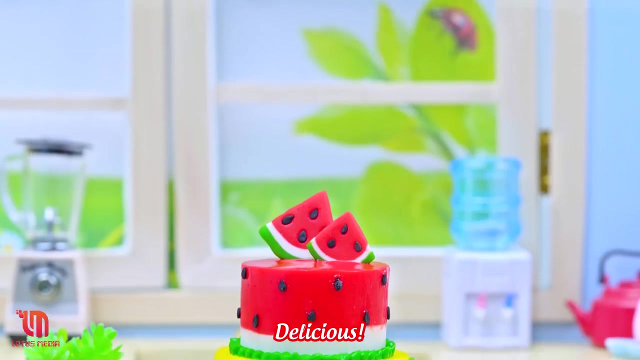 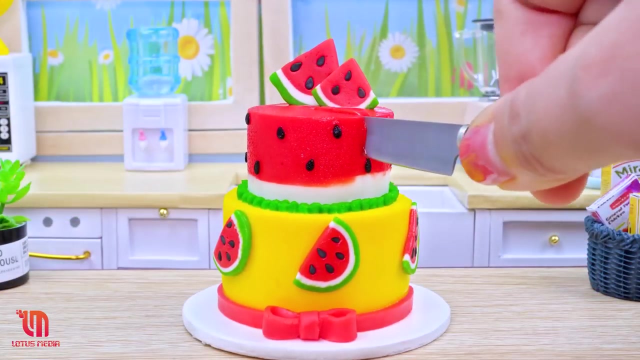 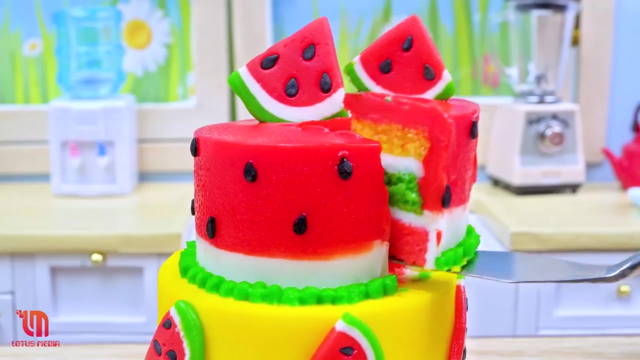 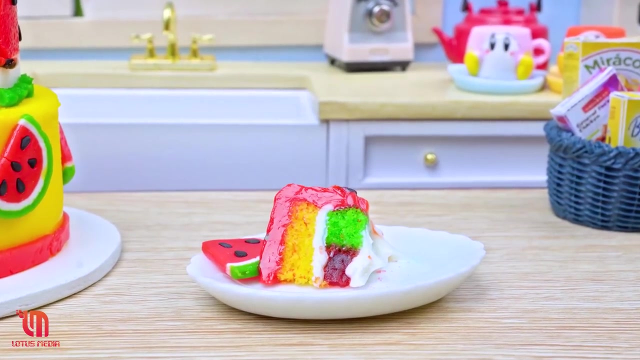 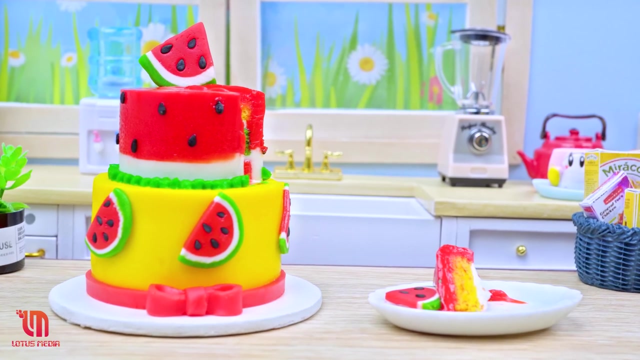 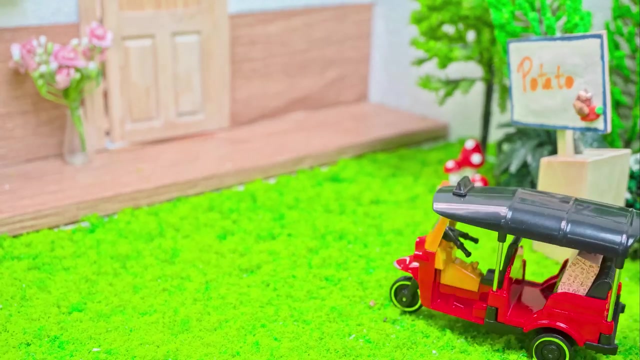 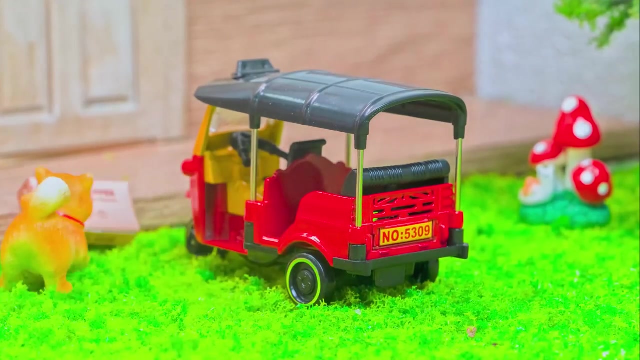 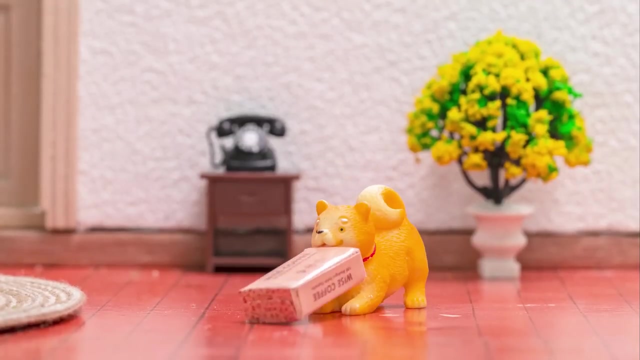 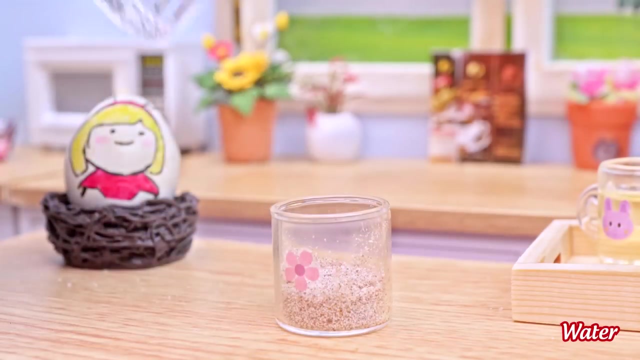 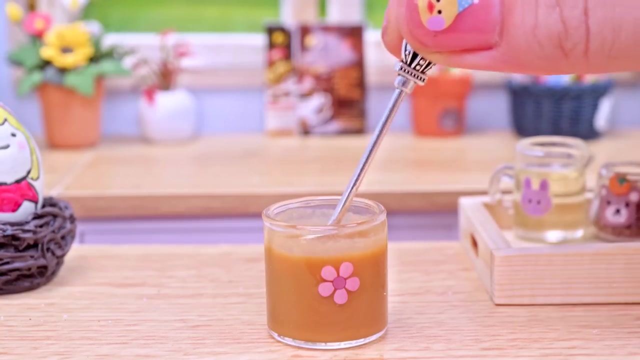 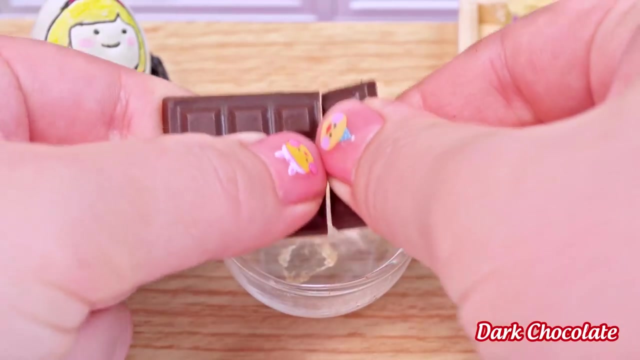 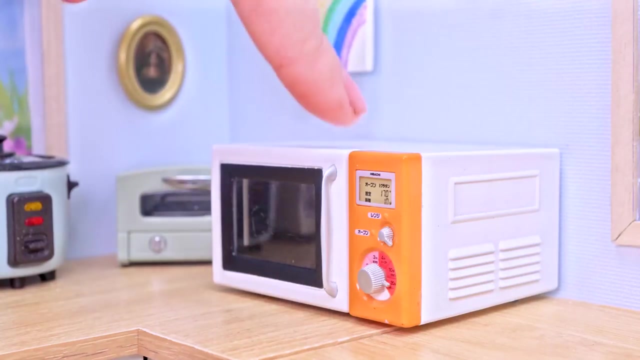 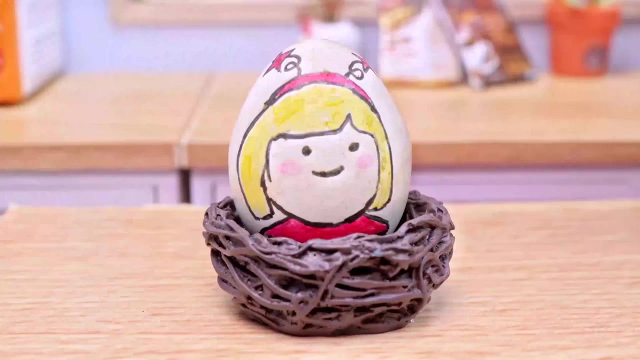 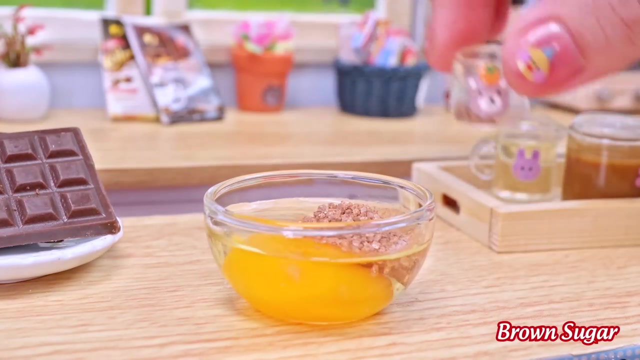 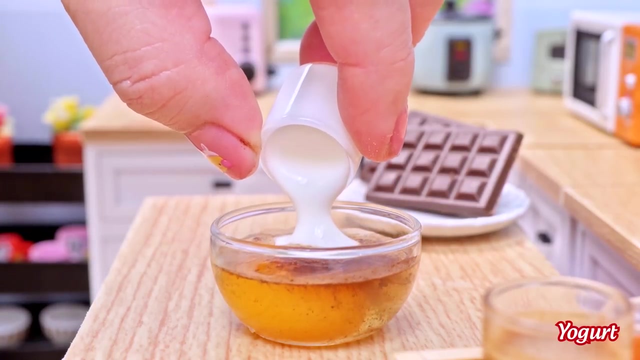 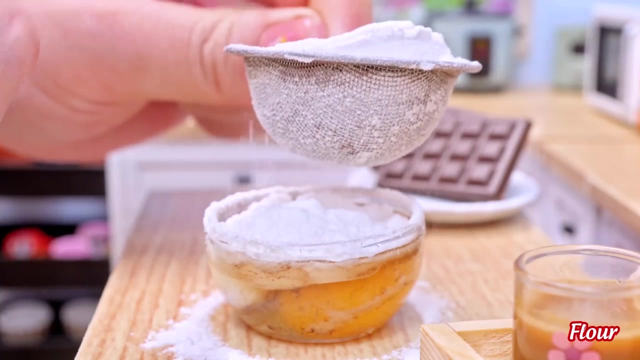 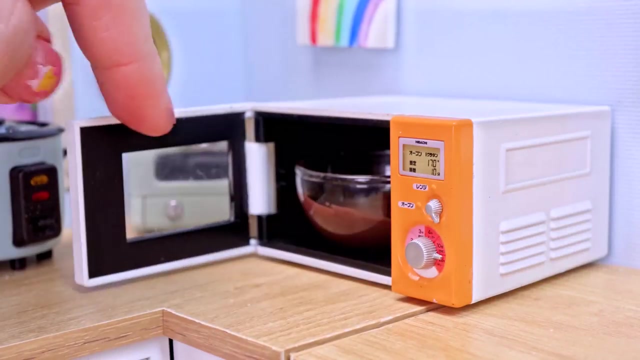 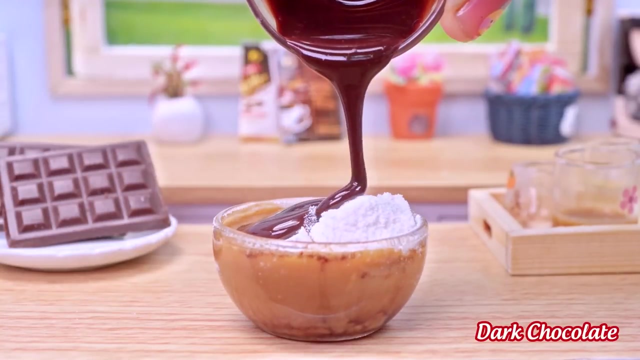 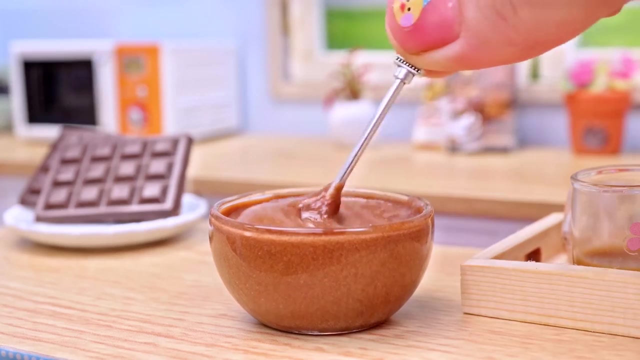 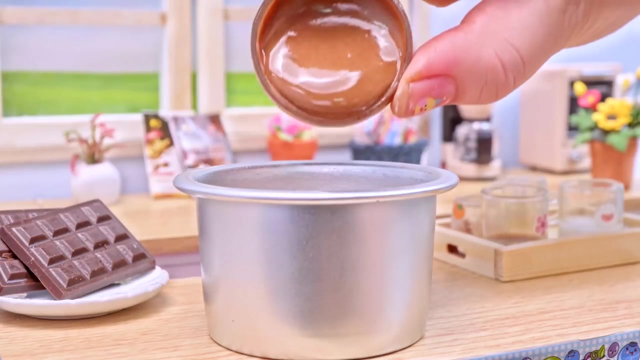 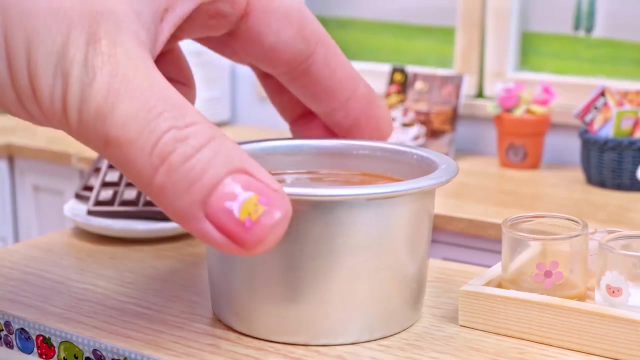 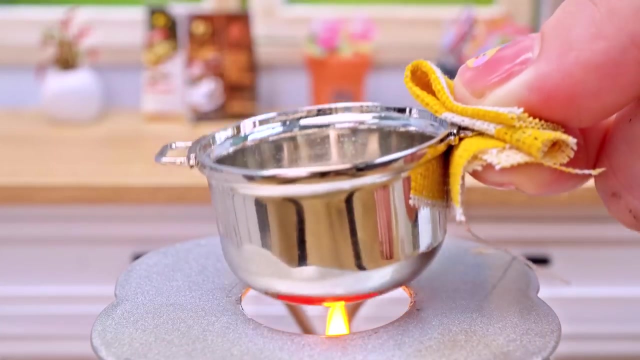 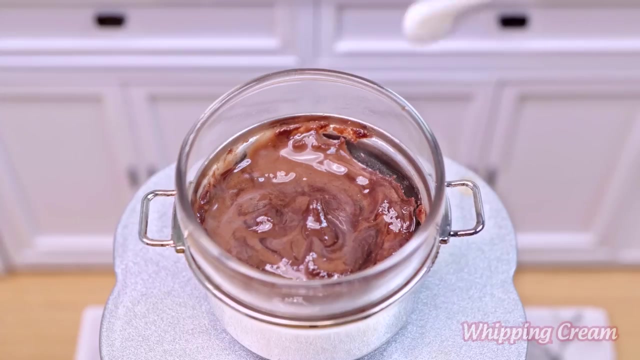 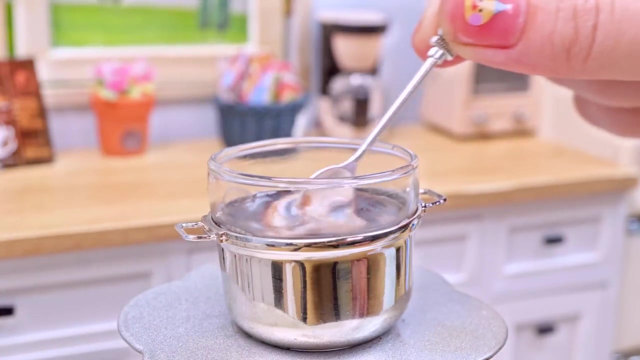 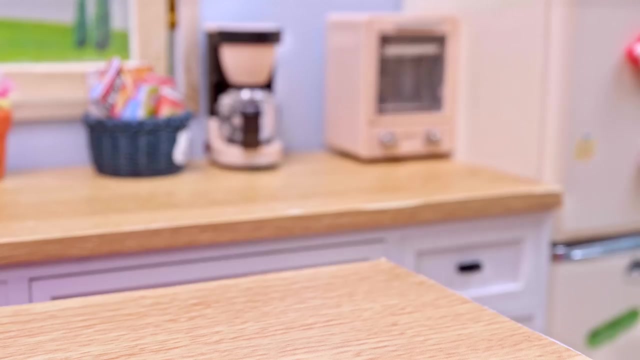 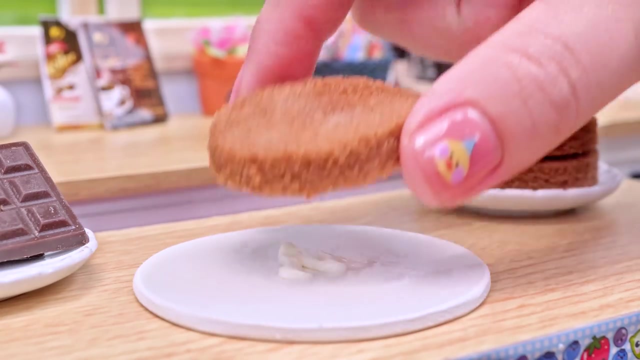 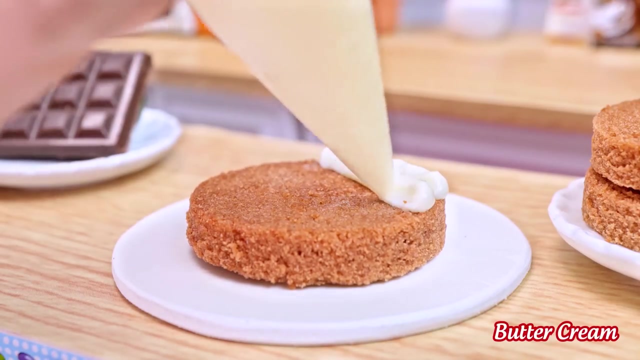 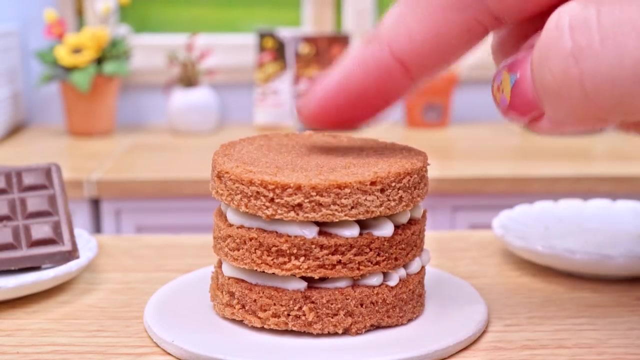 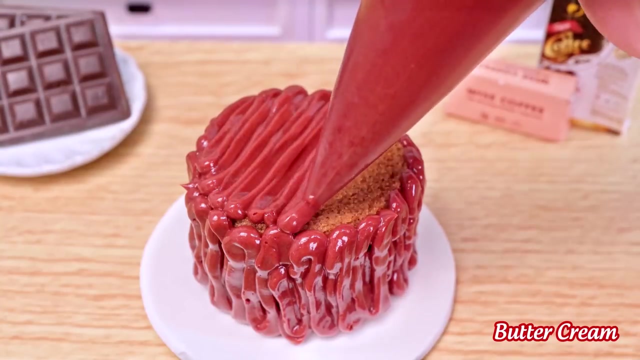 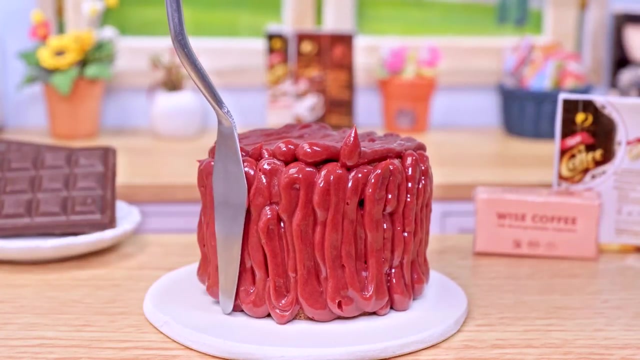 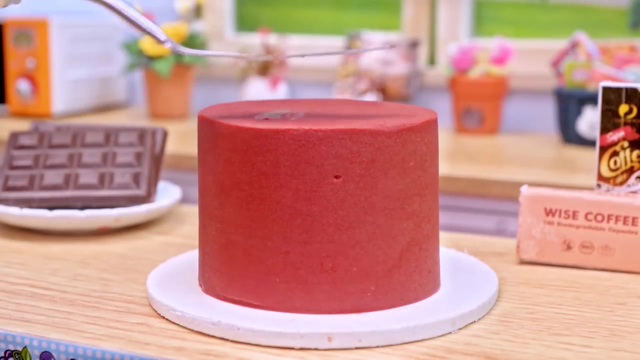 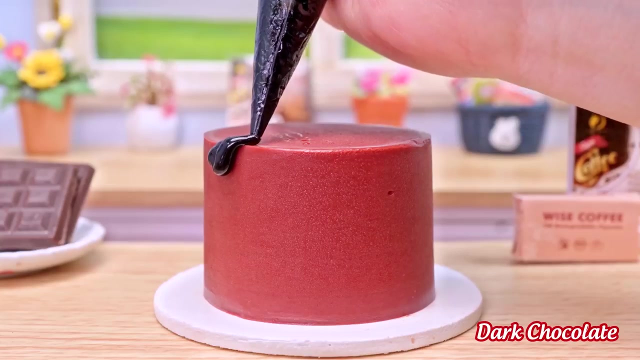 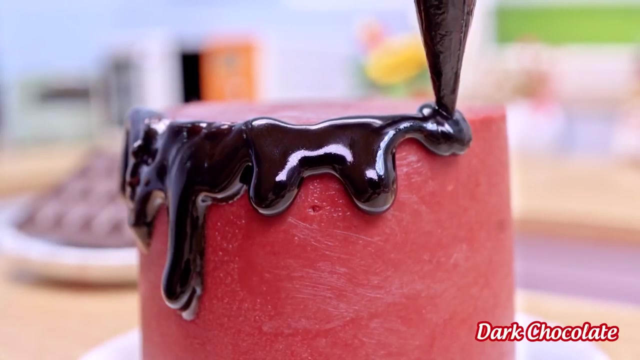 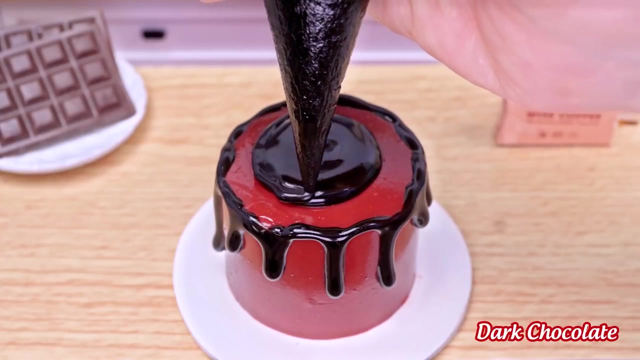 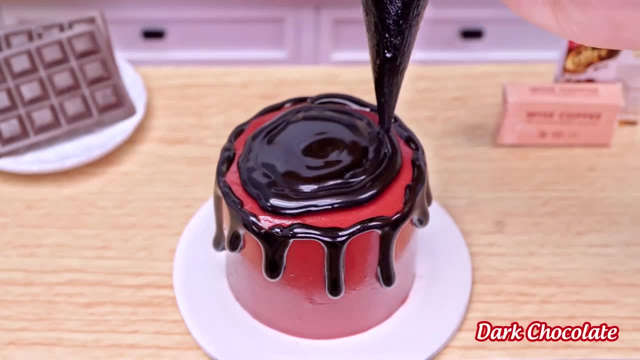 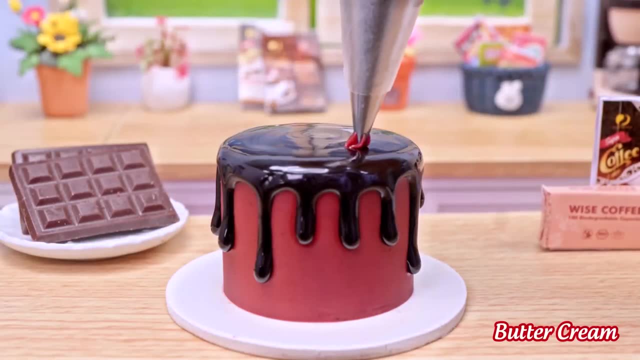 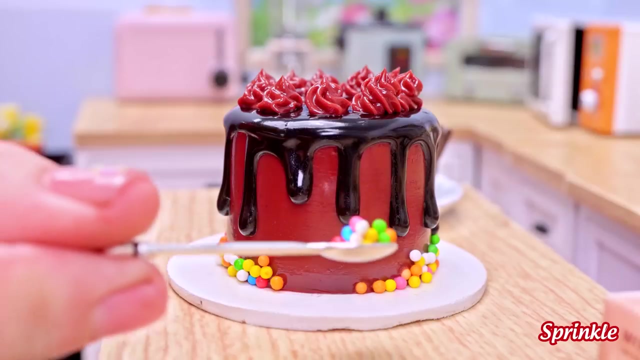 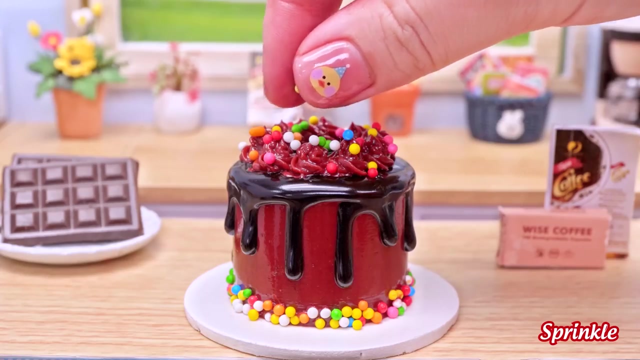 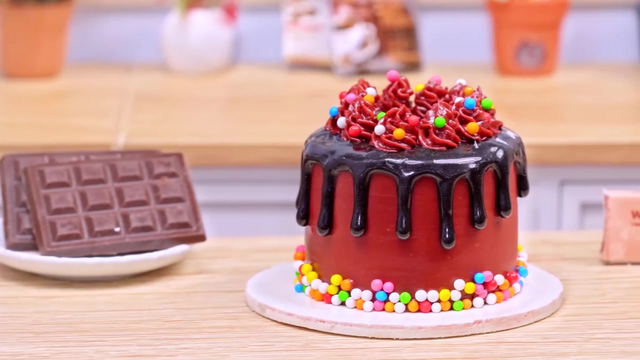 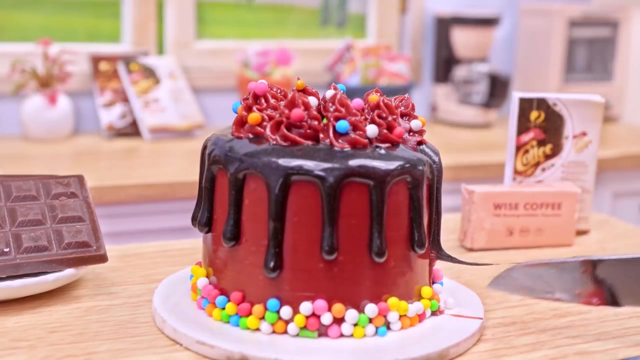 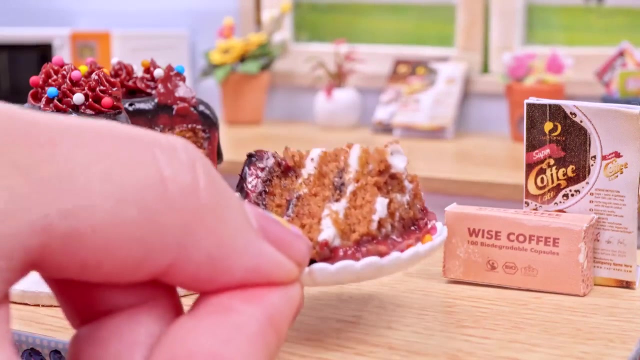 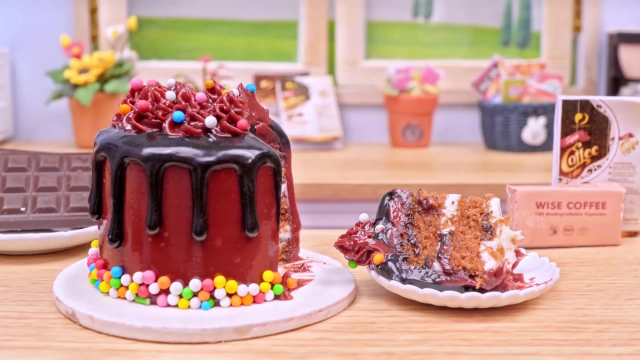 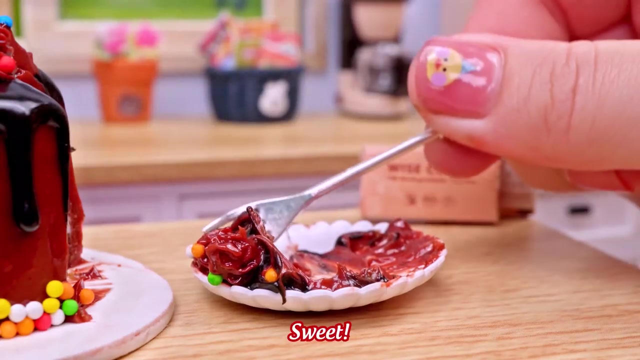 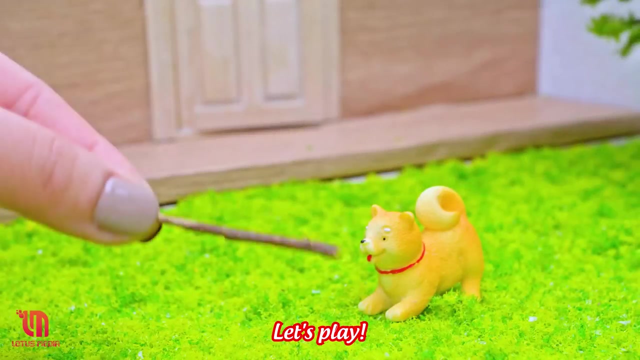 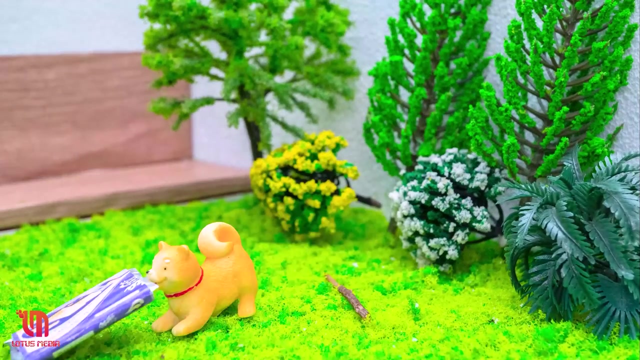 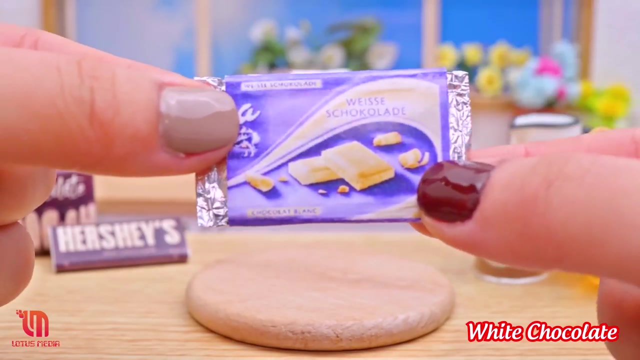 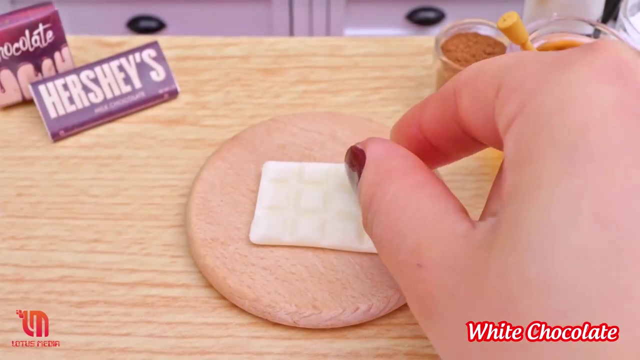 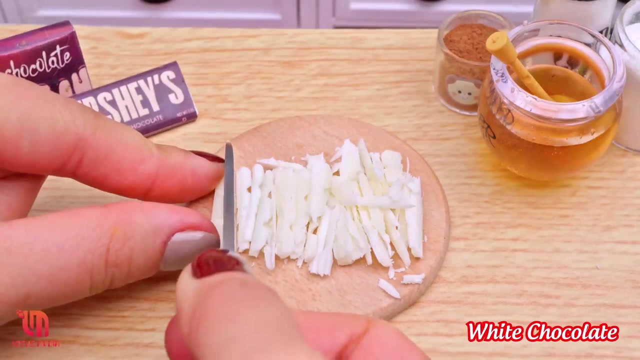 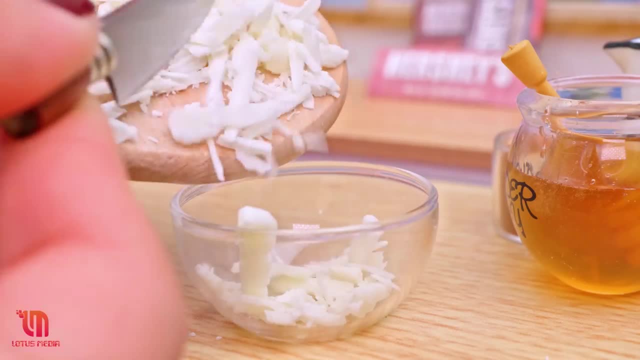 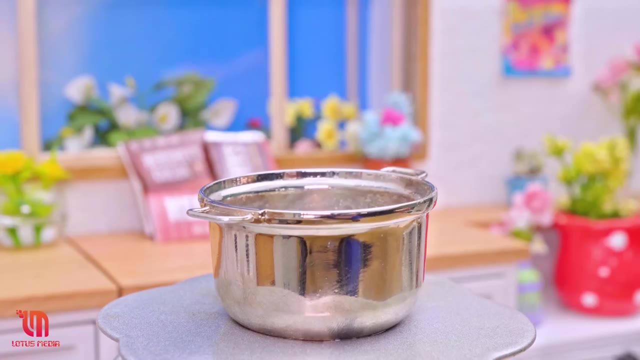 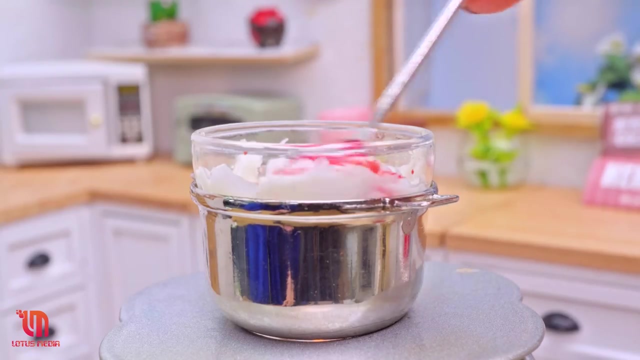 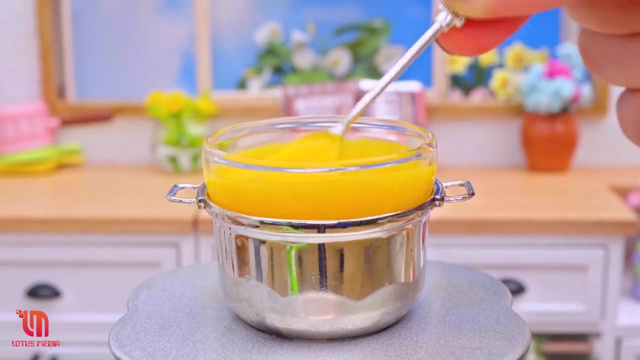 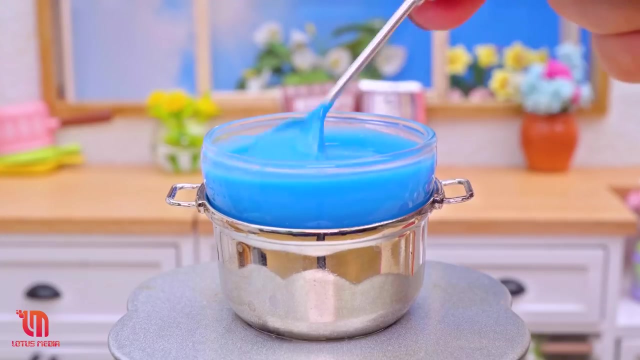 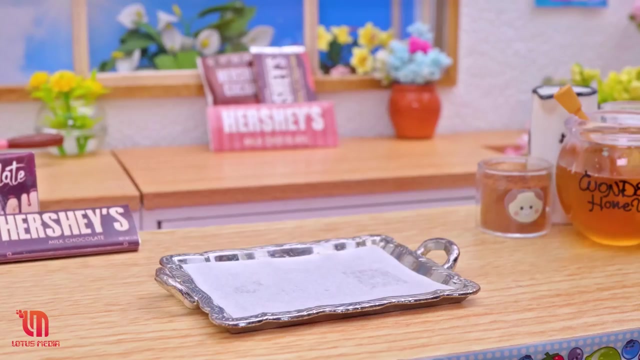 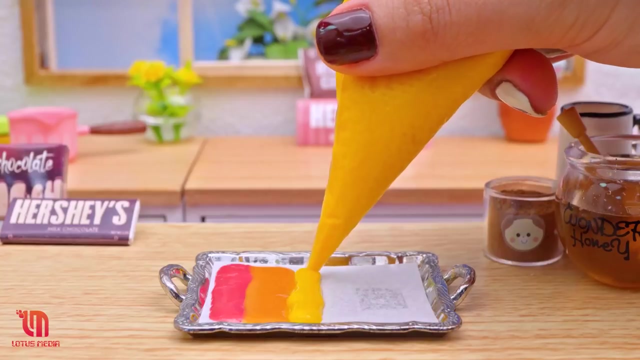 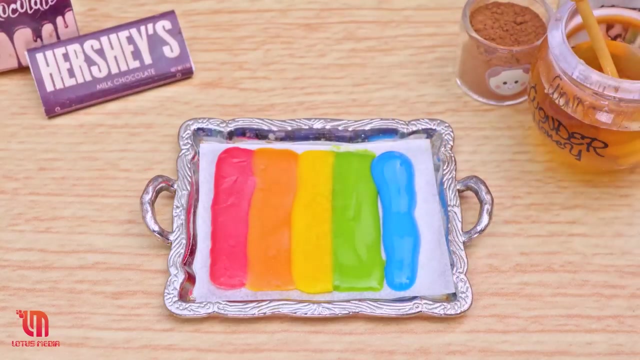 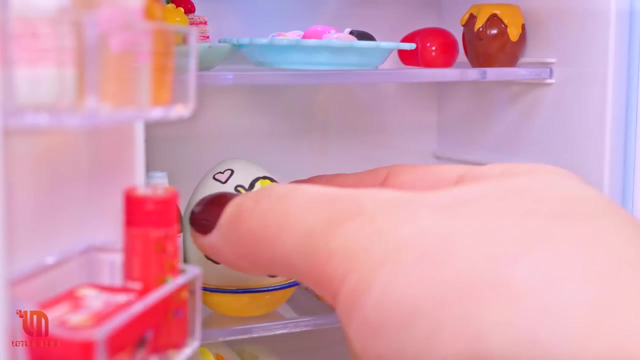 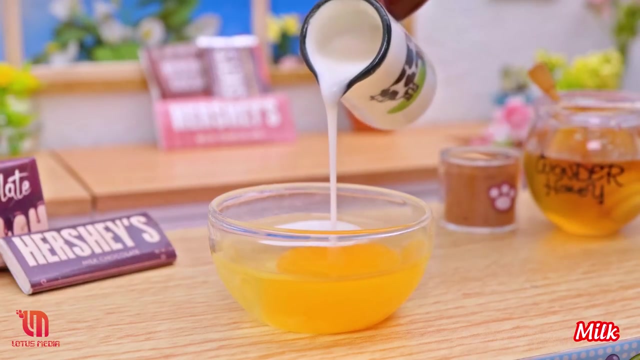 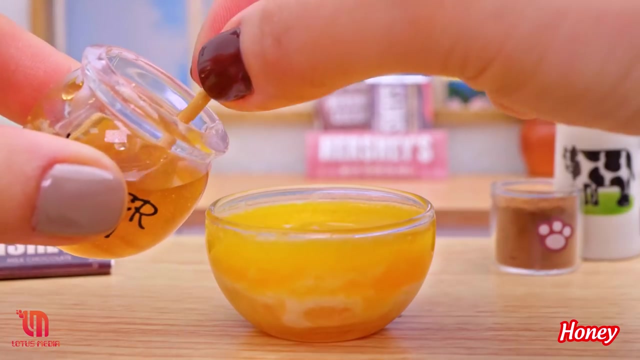 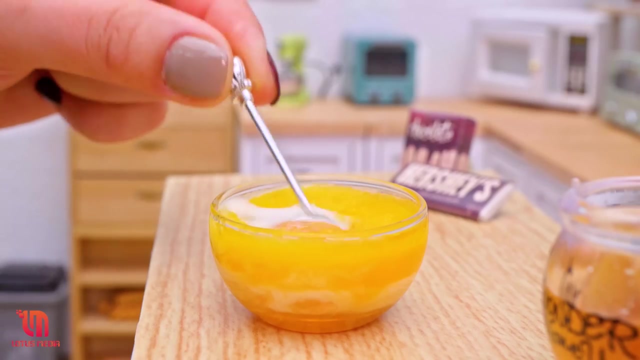 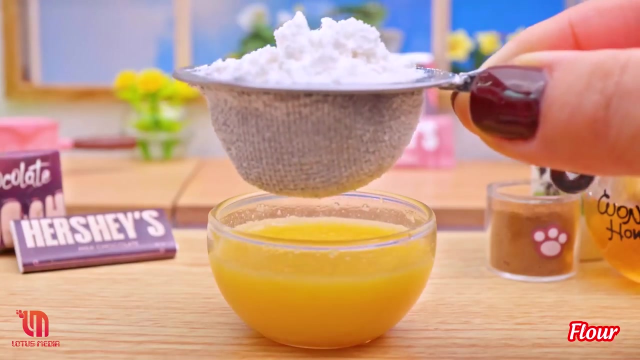 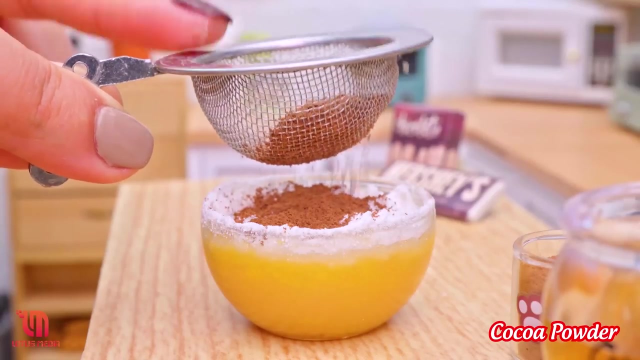 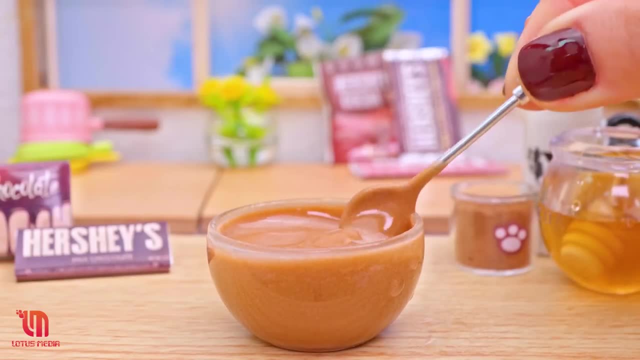 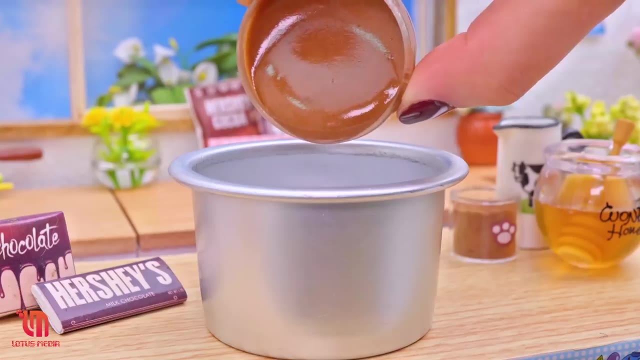 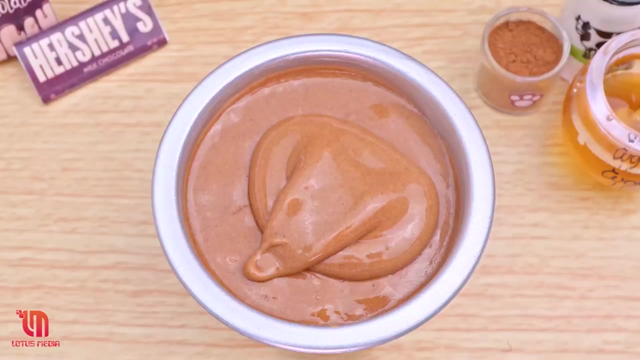 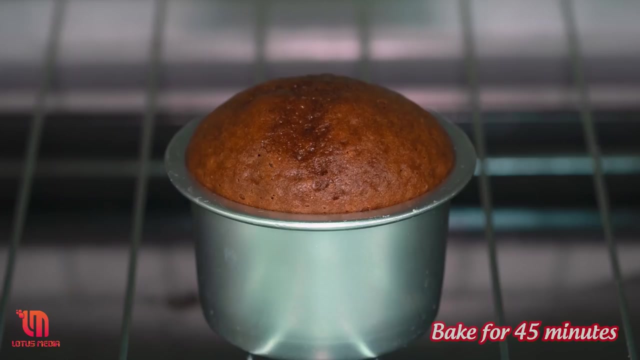 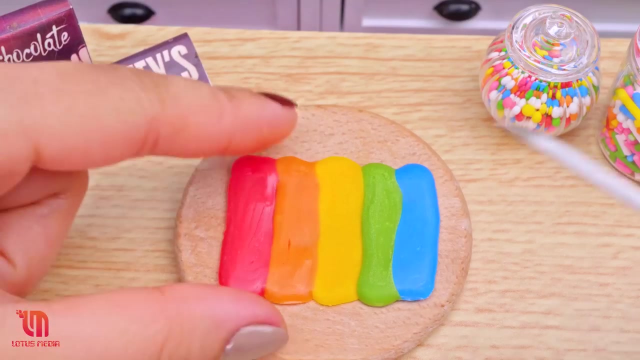 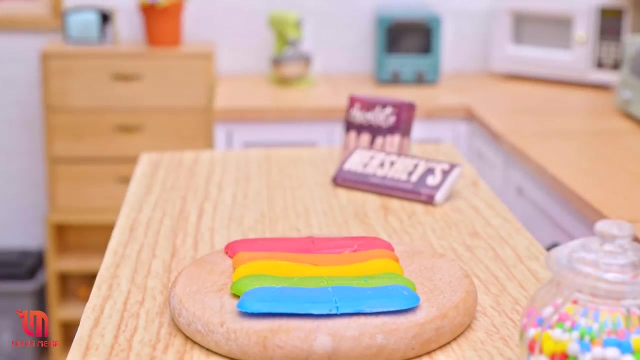 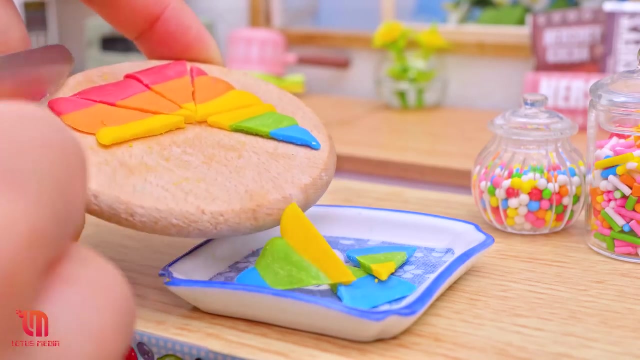 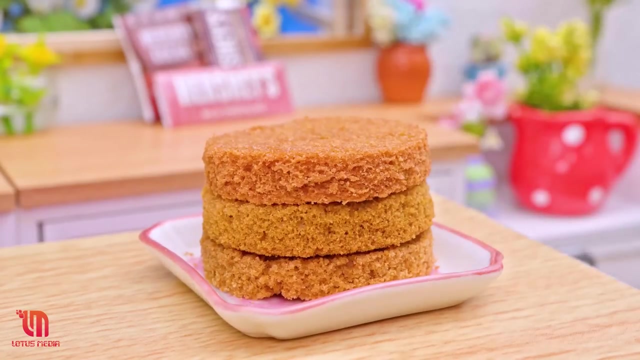 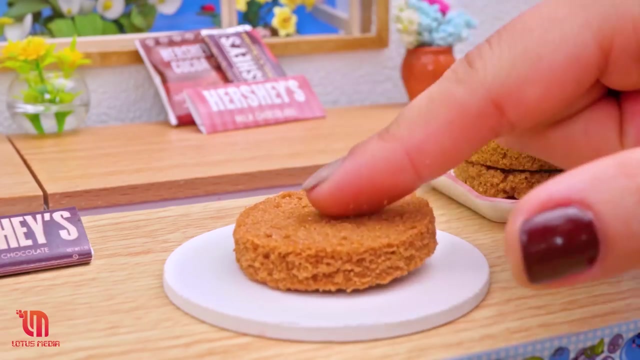 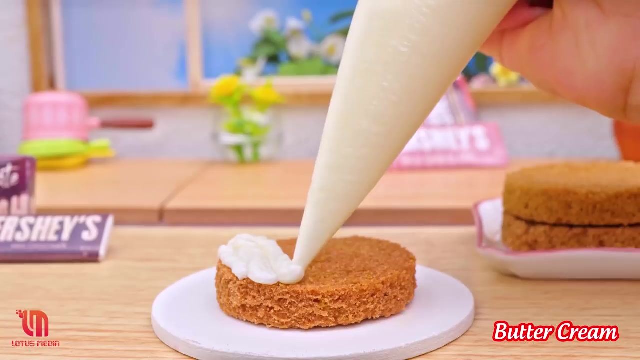 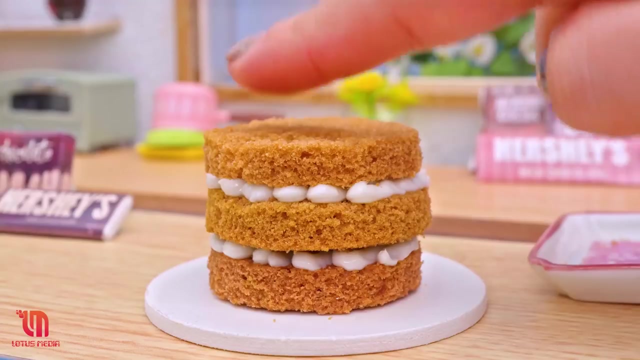 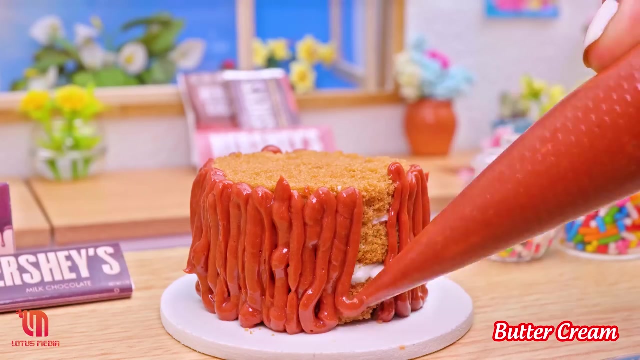 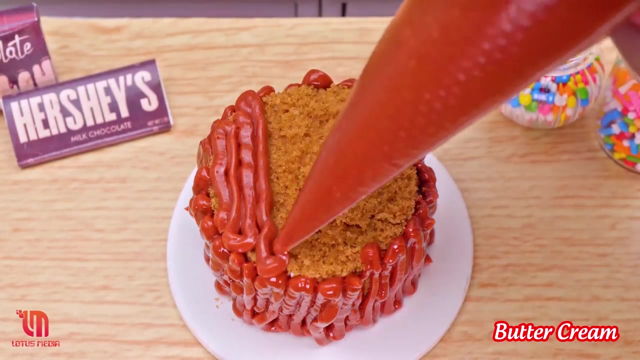 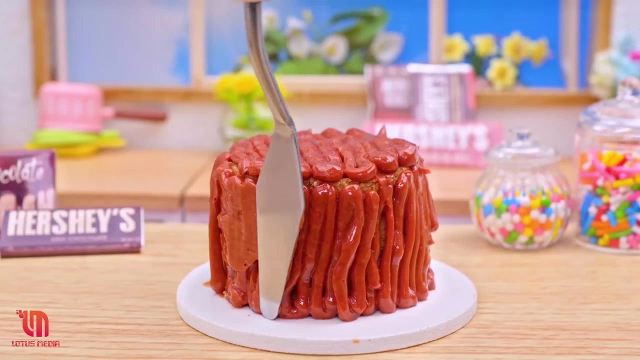 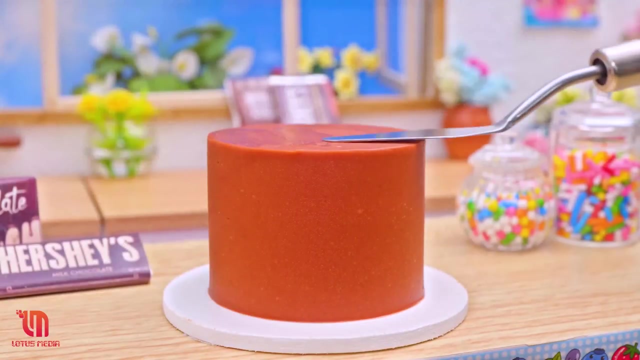 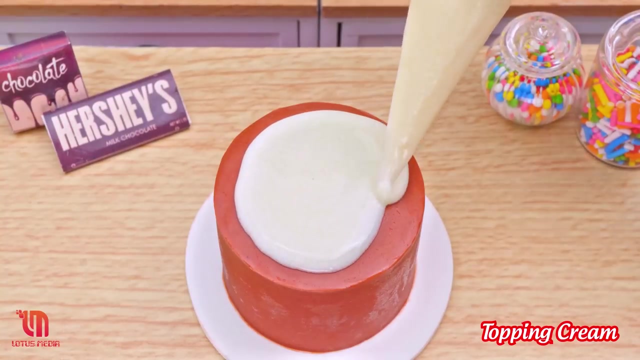 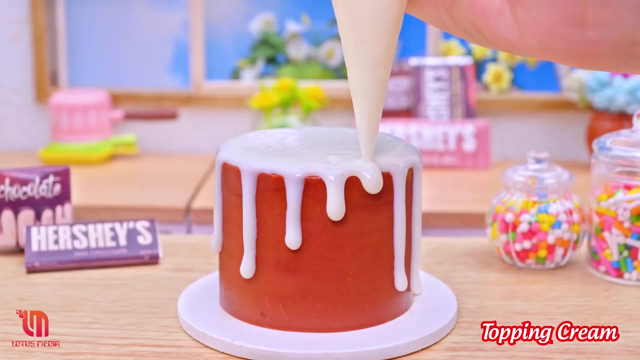 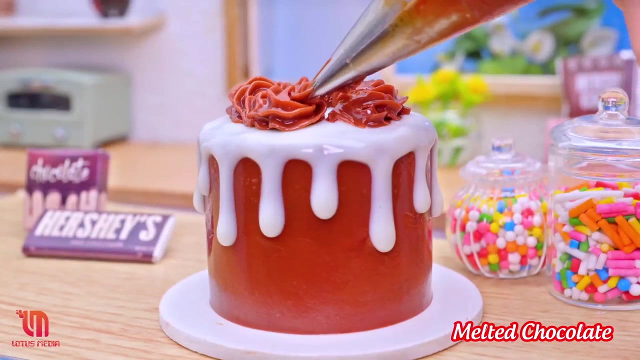 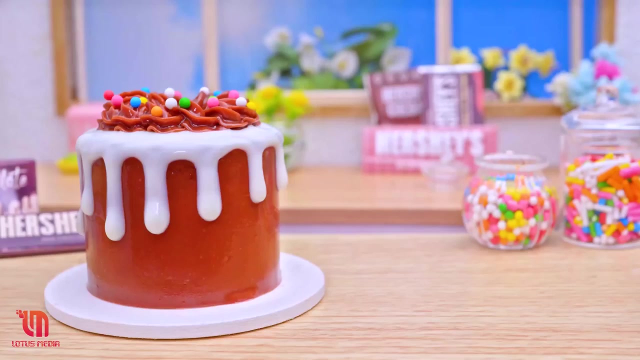 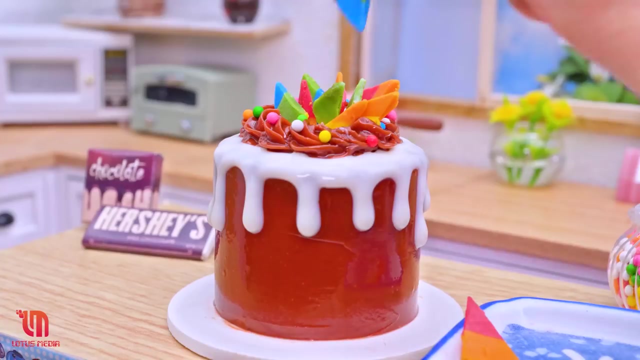 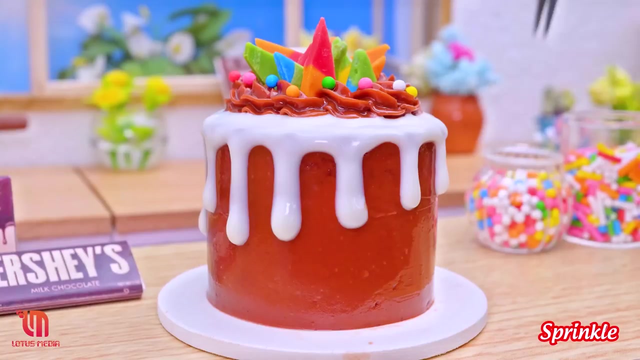 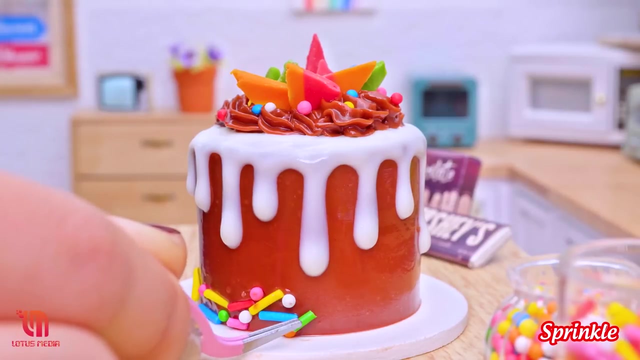 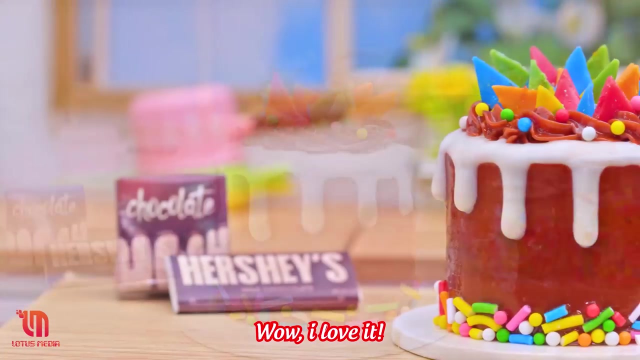 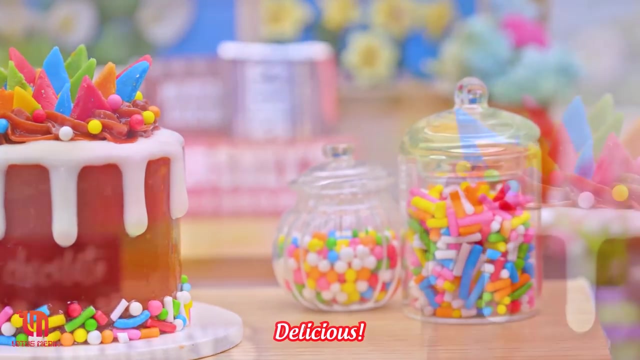 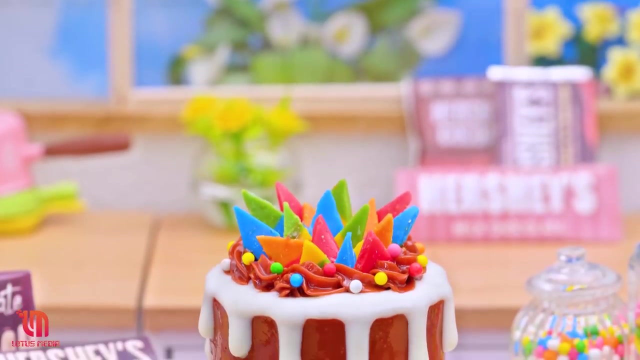 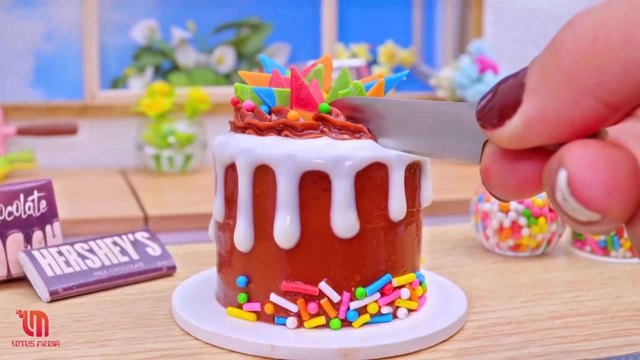 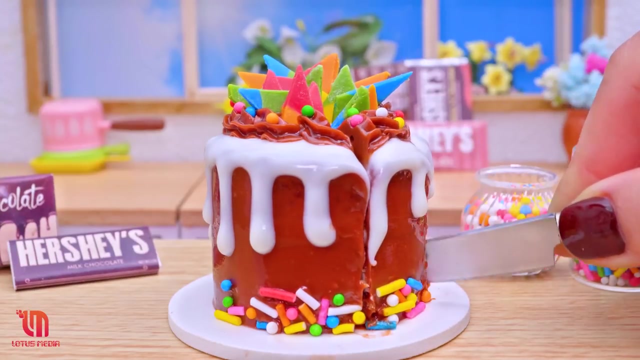 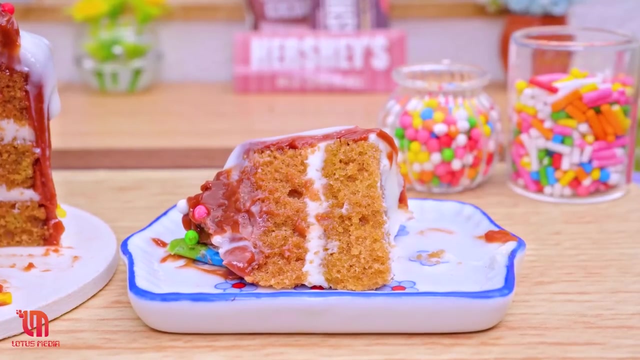 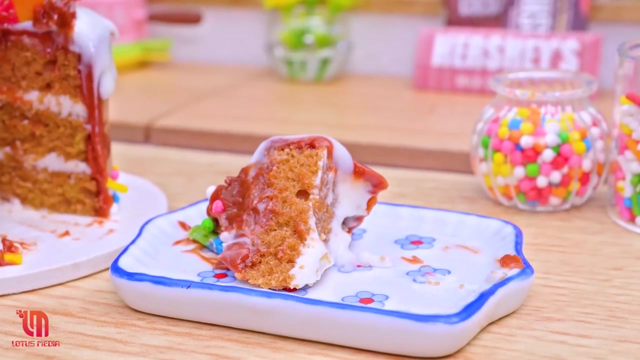 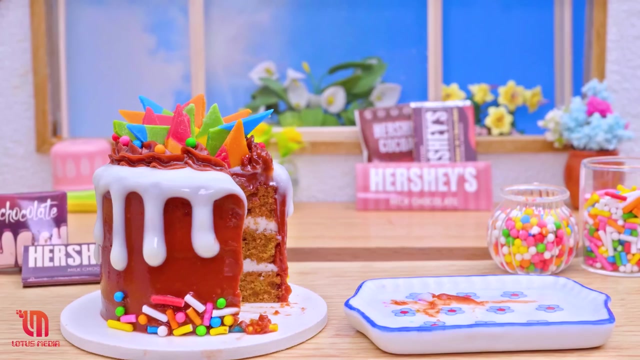 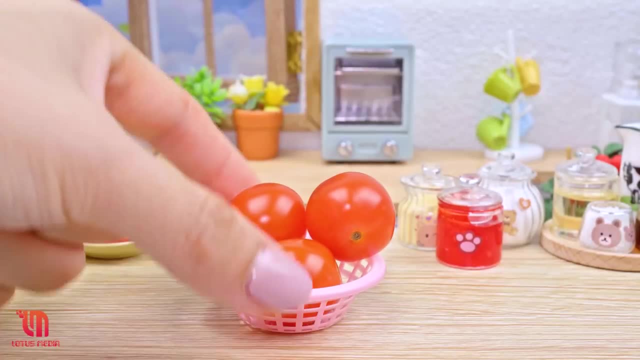 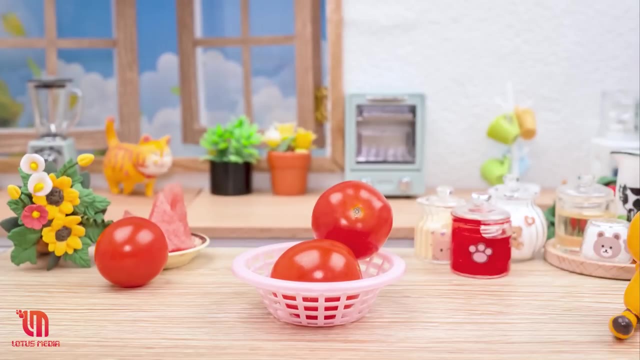 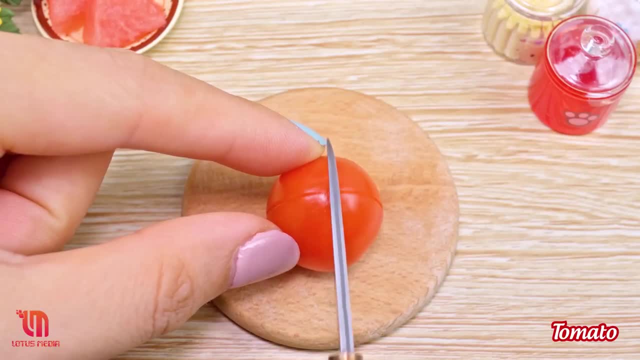 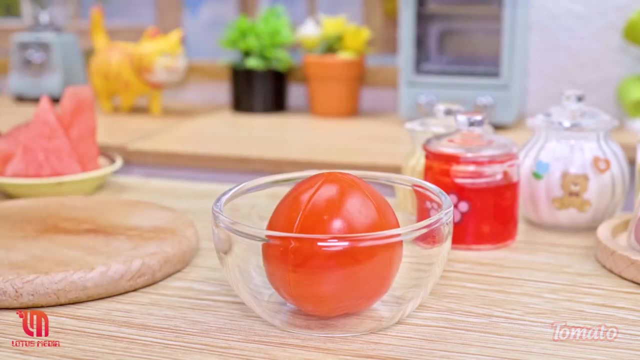 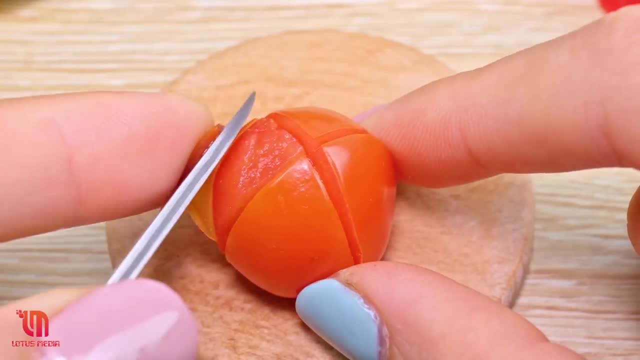 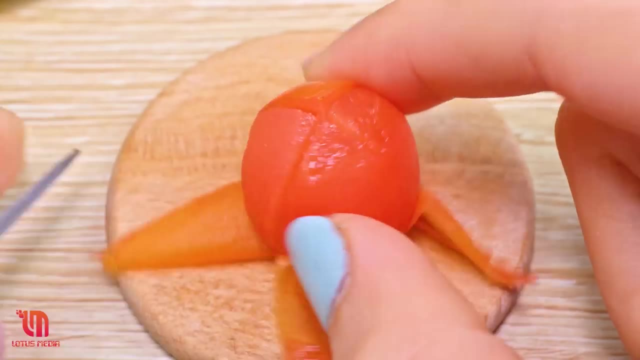 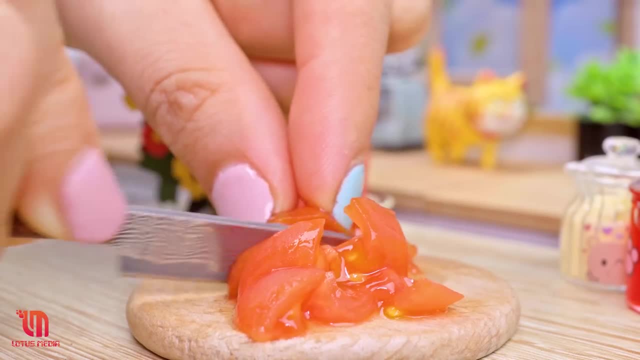 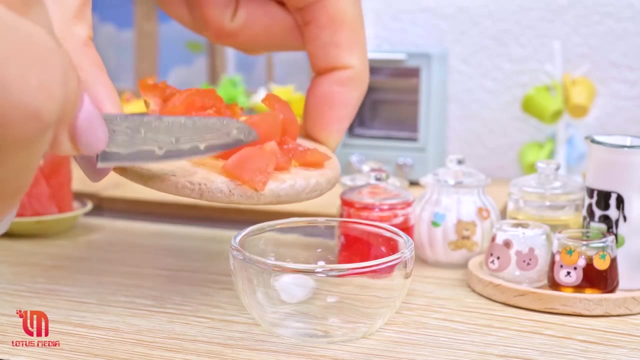 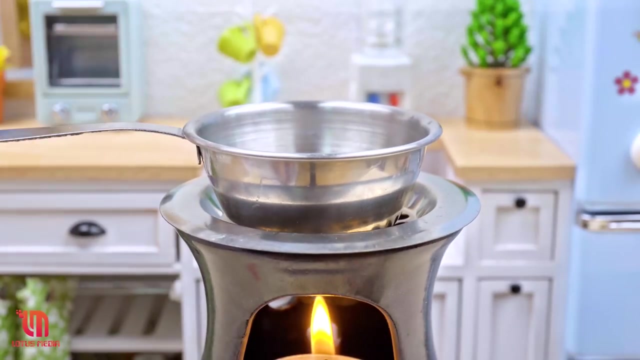 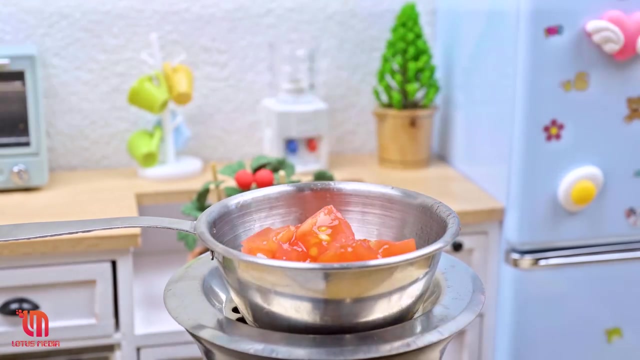 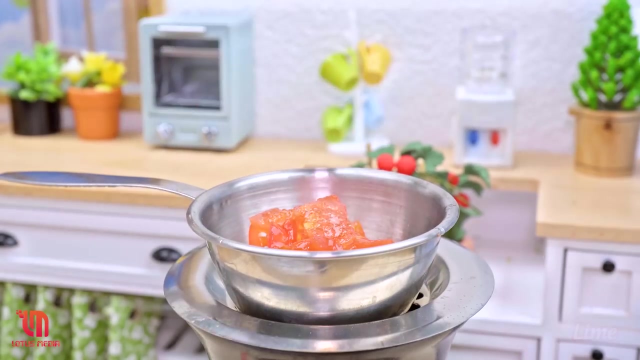 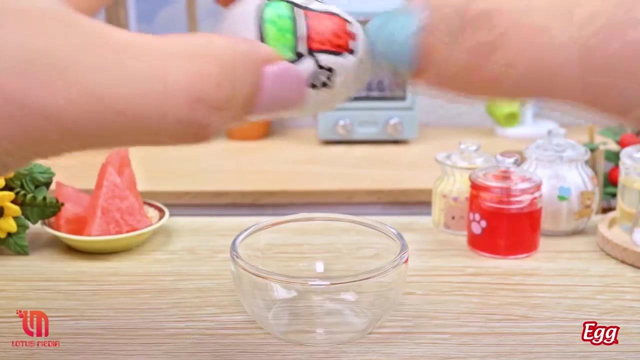 Yummy, Yummy, Yummy, Yummy, Yummy, Yummy, Yummy ateurs, Yummy, Yummy, Yummy, Yummy Shed Ан. Add the egg, Add the flour, Add the eggs, Mix. 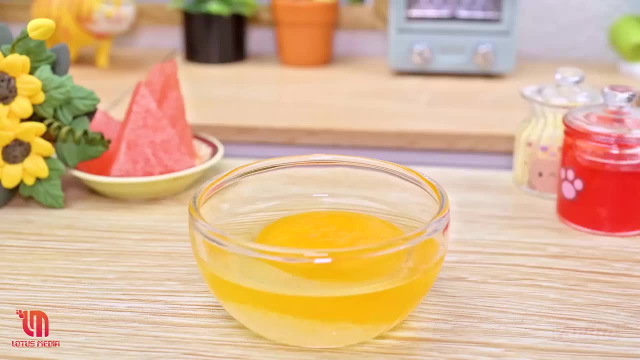 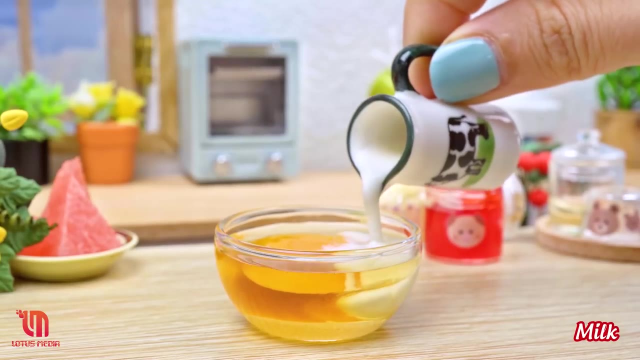 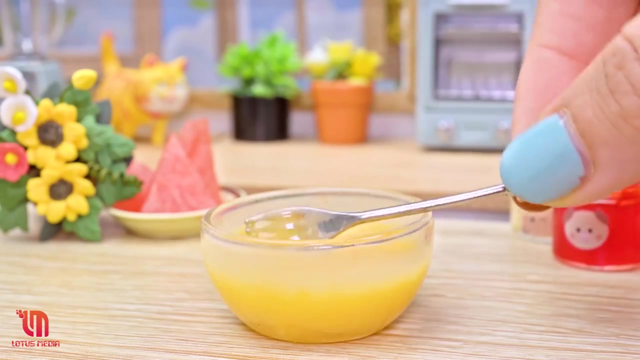 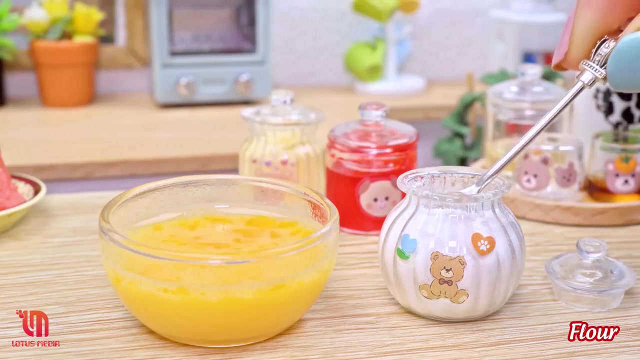 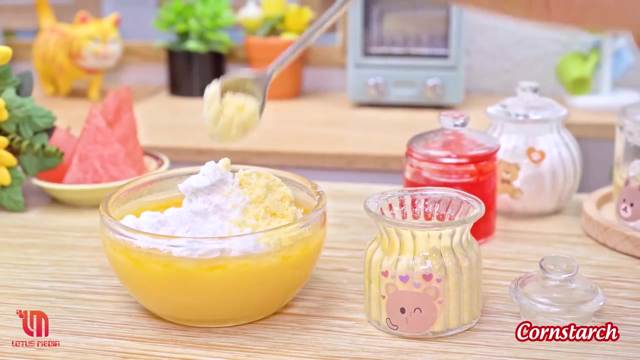 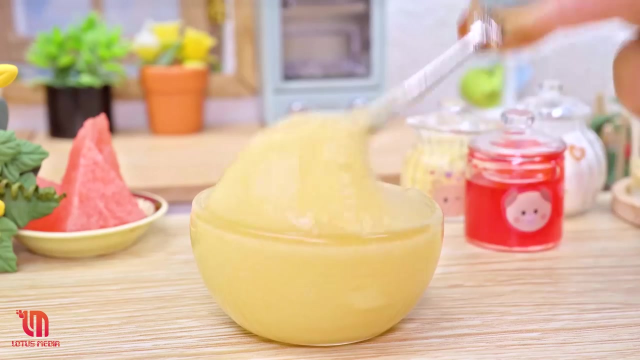 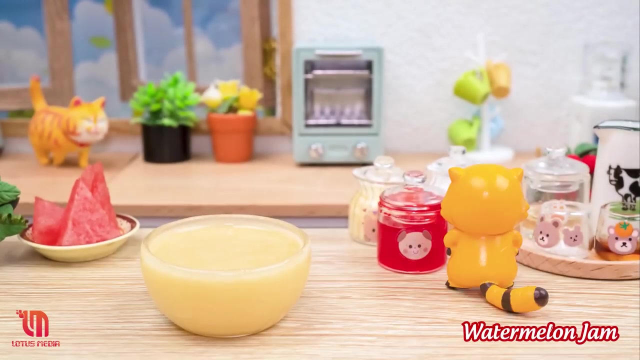 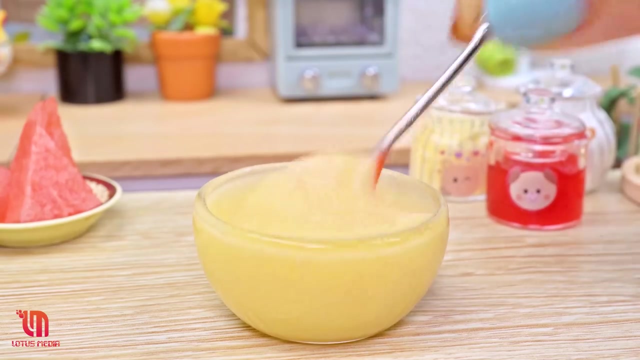 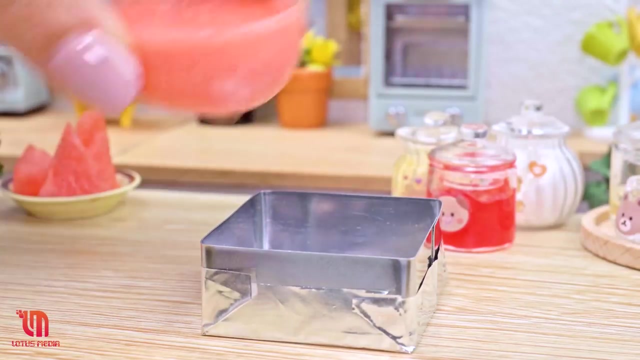 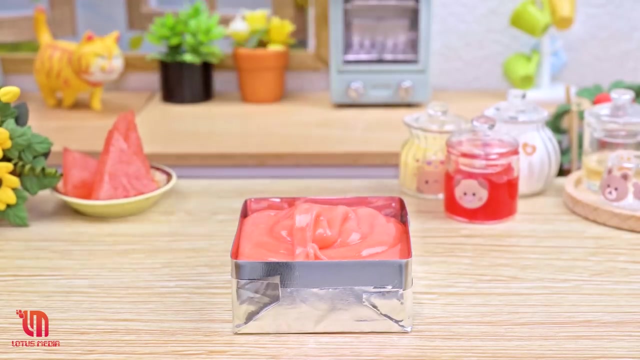 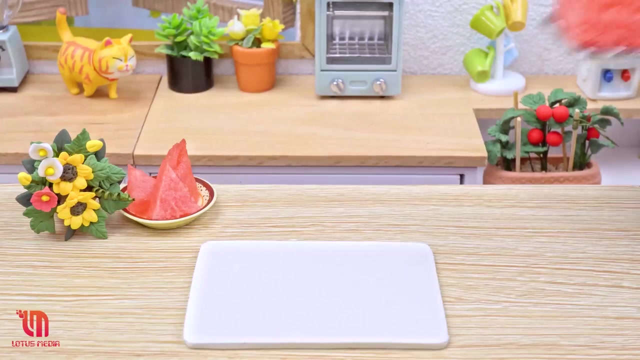 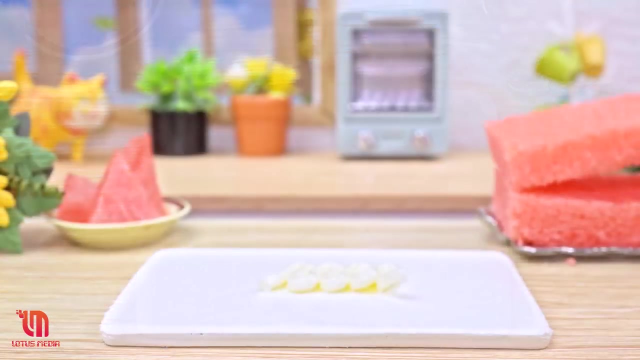 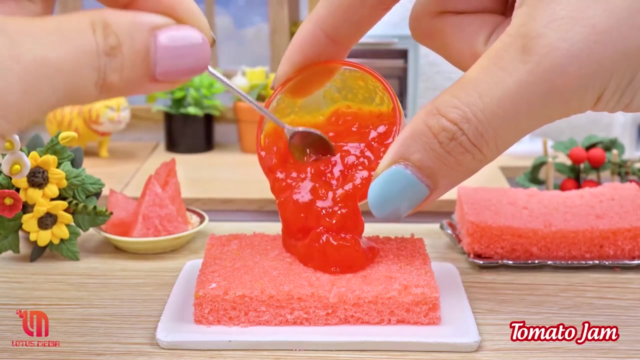 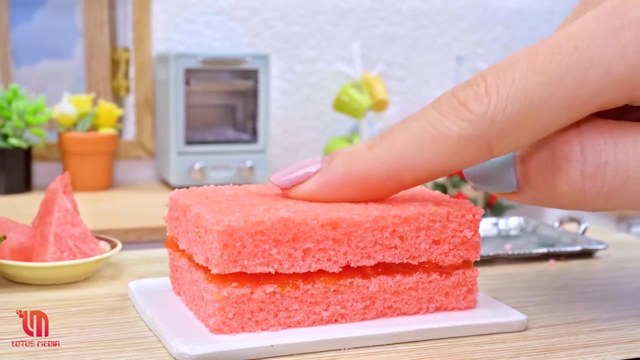 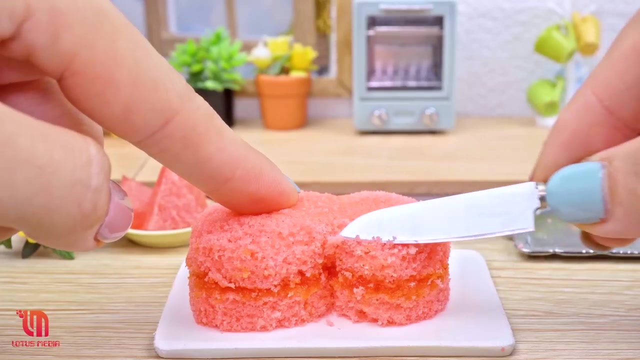 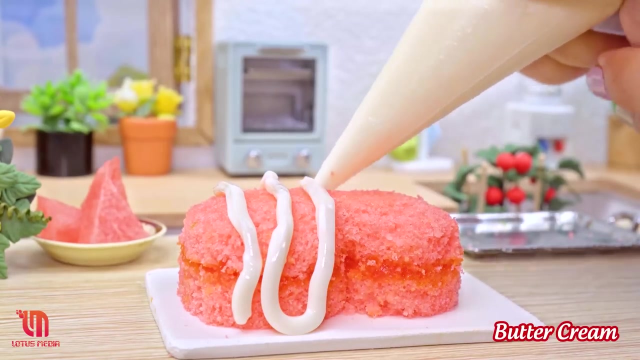 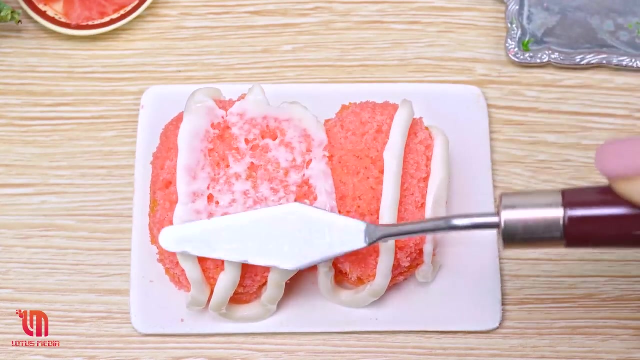 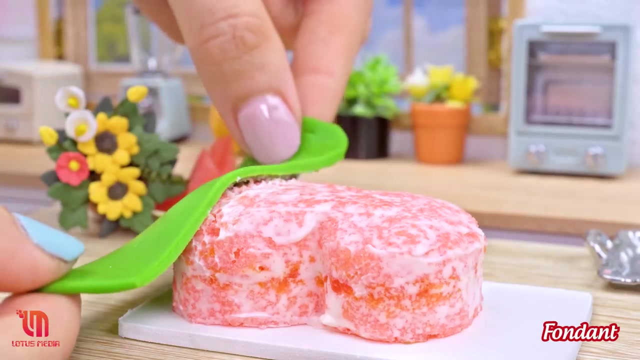 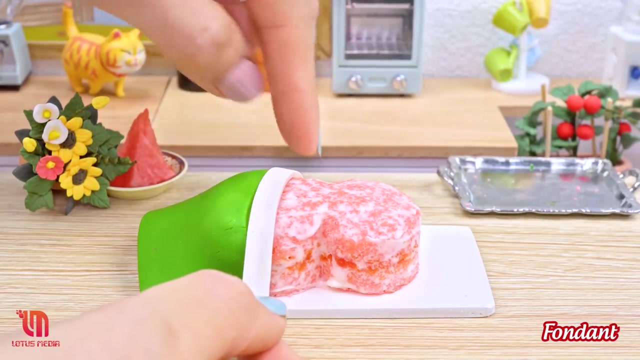 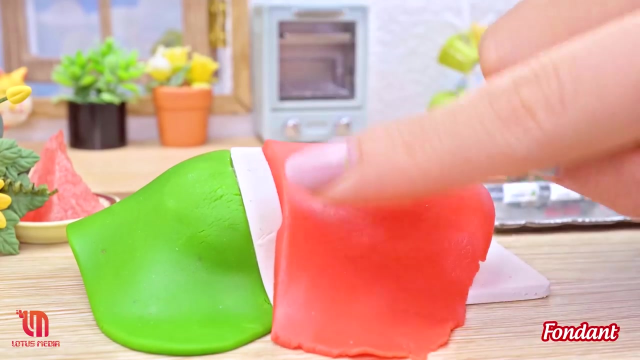 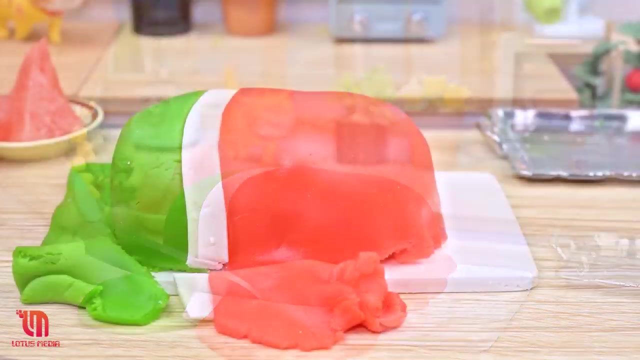 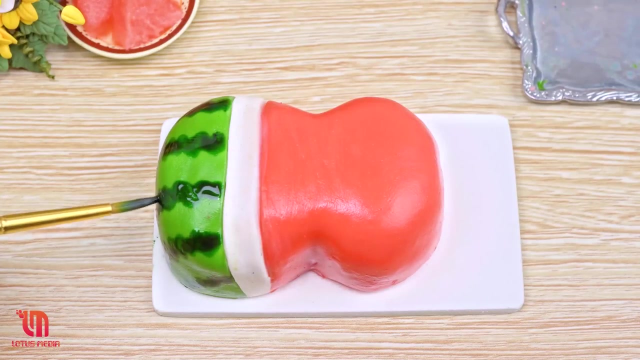 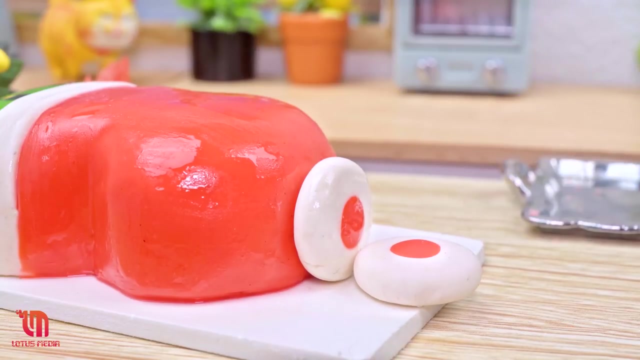 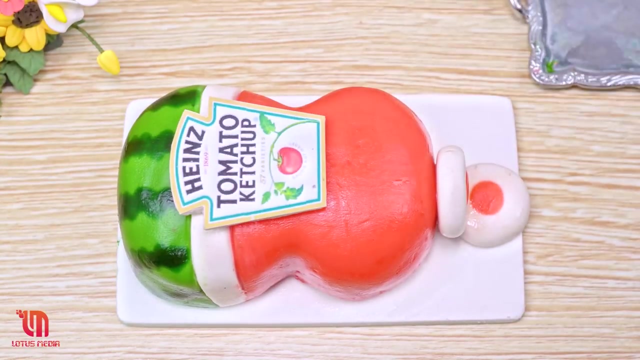 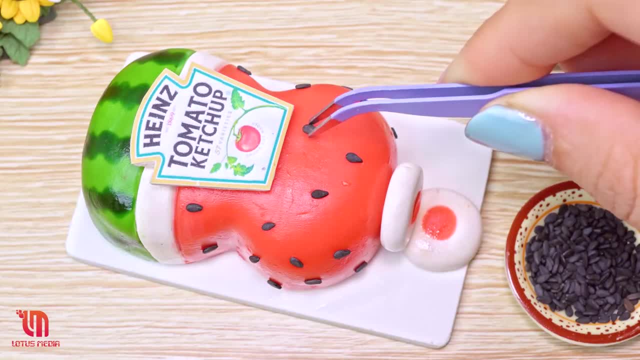 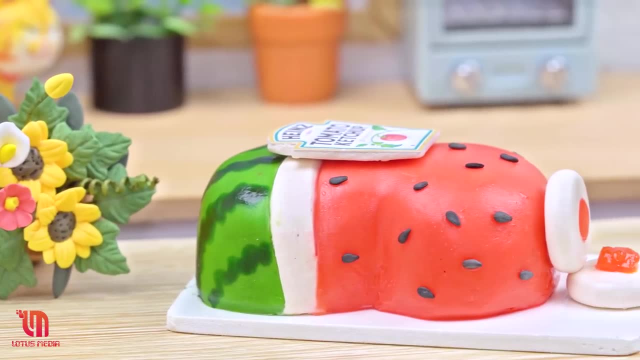 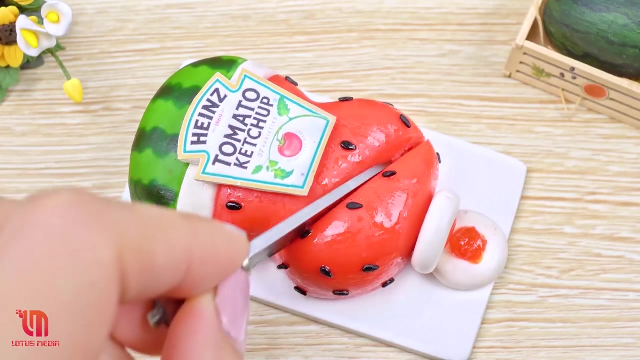 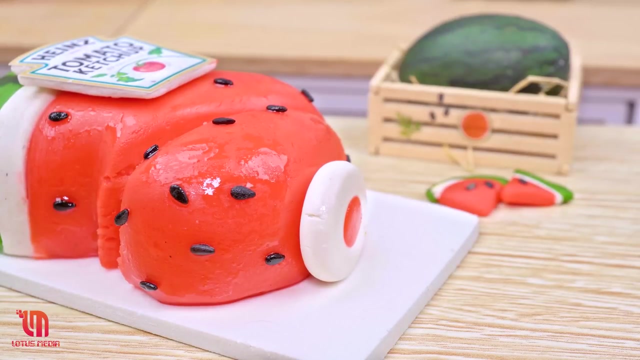 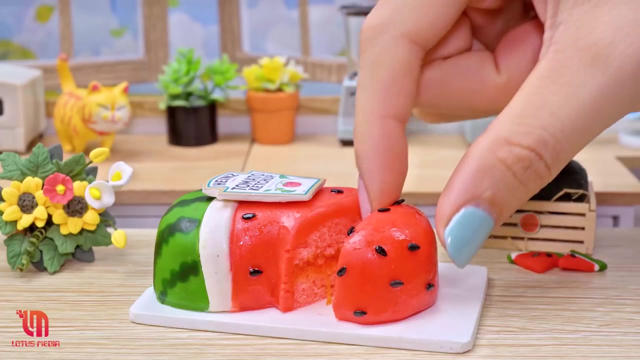 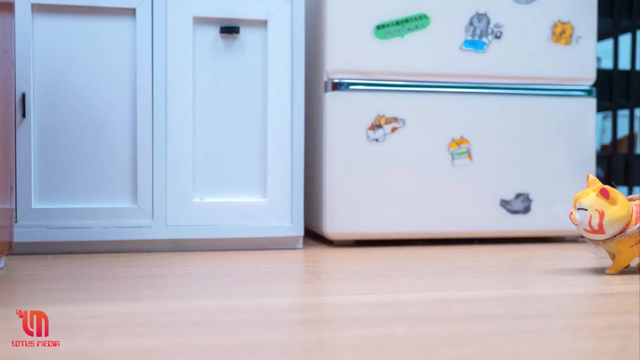 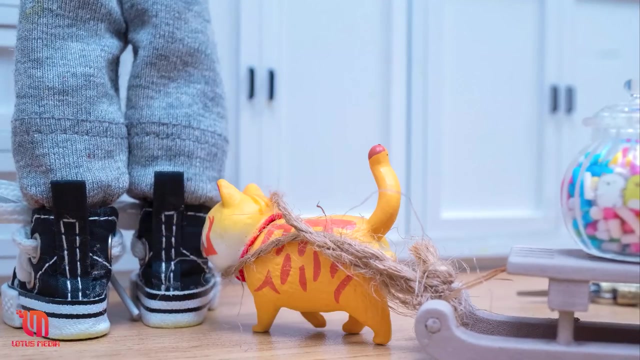 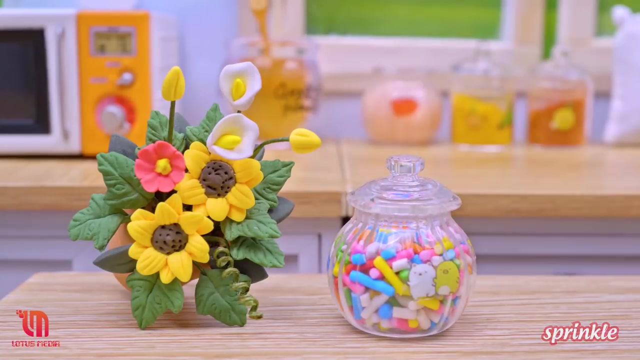 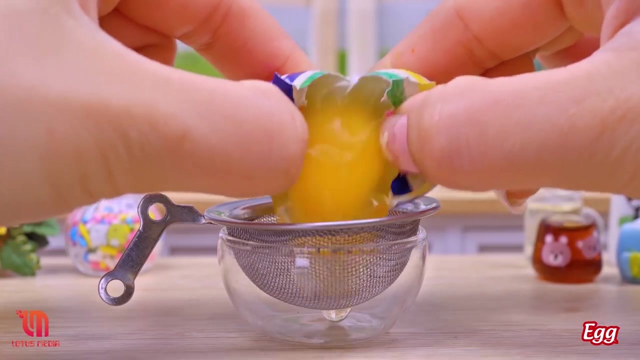 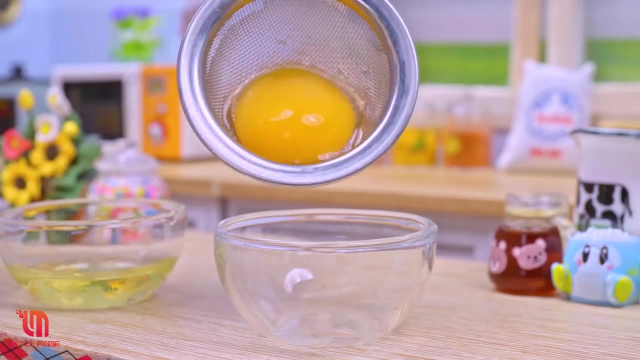 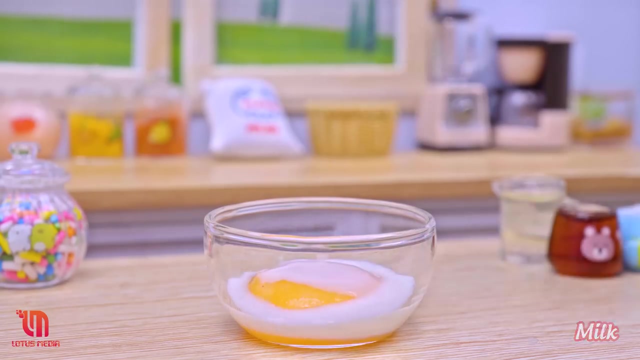 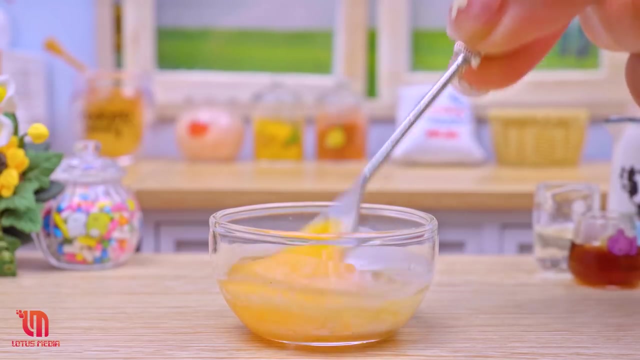 Wow, I love it. Delicious, Tasty, Wow, Wow, Wow, Tasty, Yummy, Wow. Thank you, I will make a cake with this. Ow Wow, Yeah, Wow, Yeah, Wow, Wow, Wow. 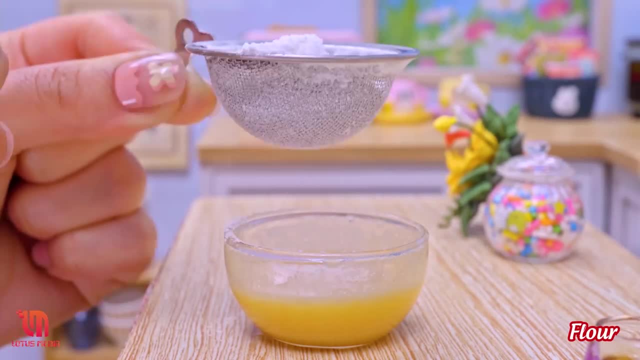 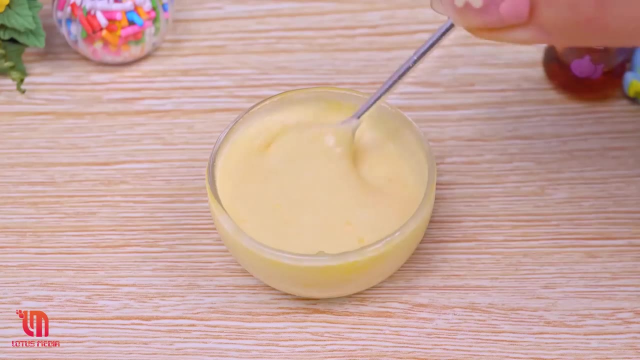 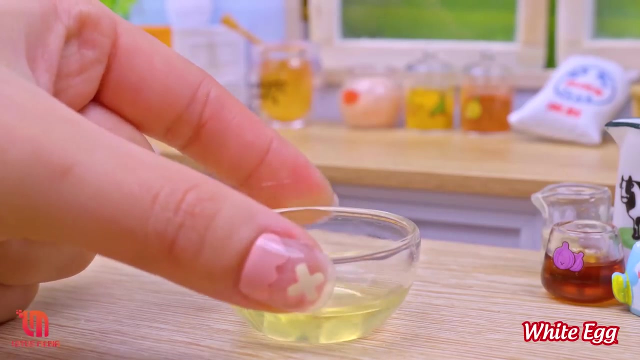 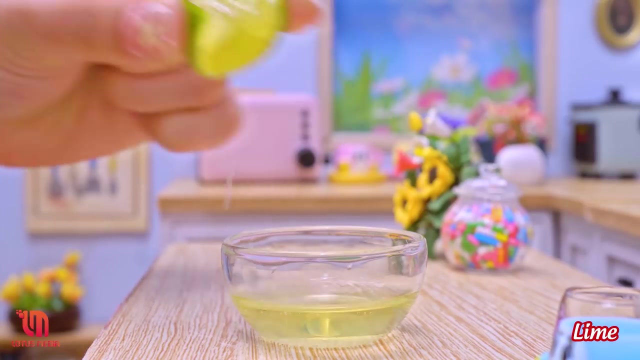 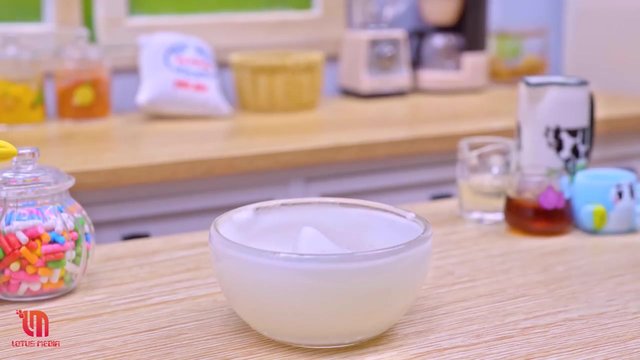 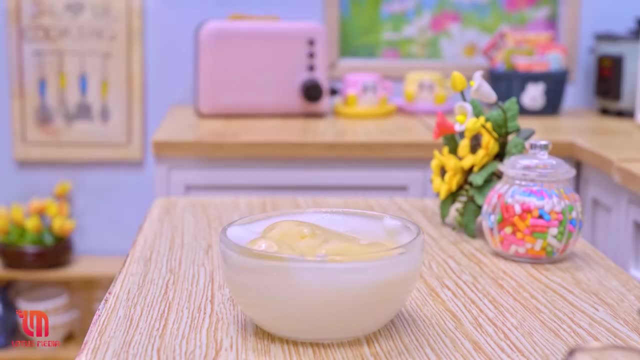 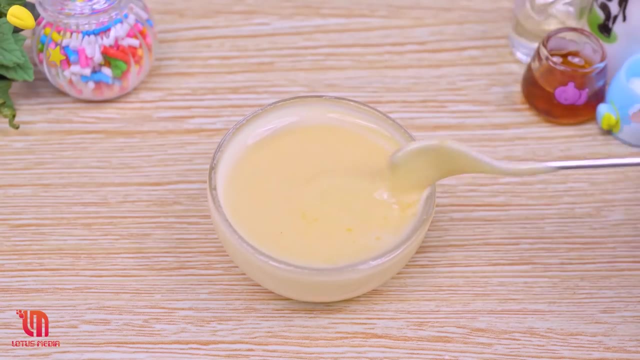 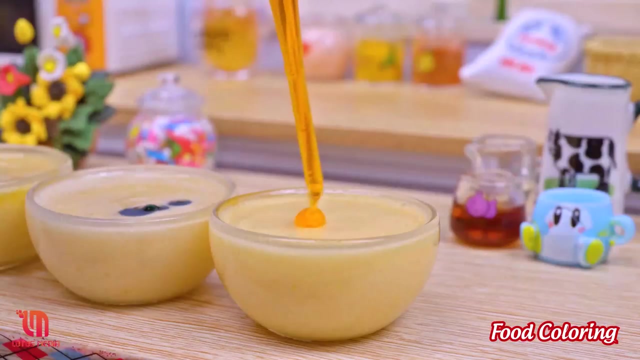 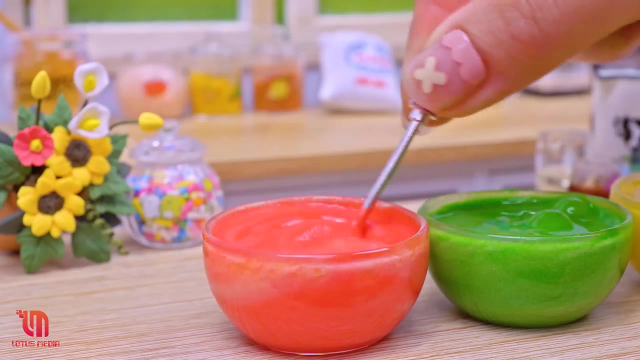 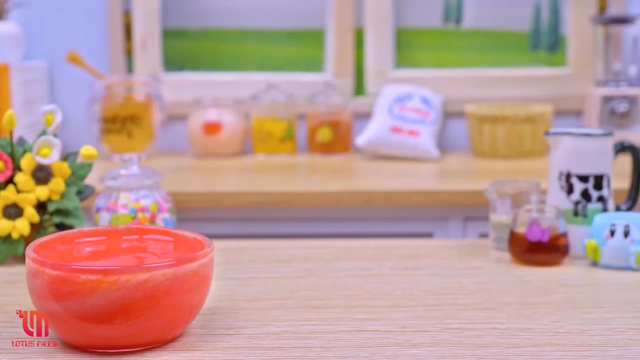 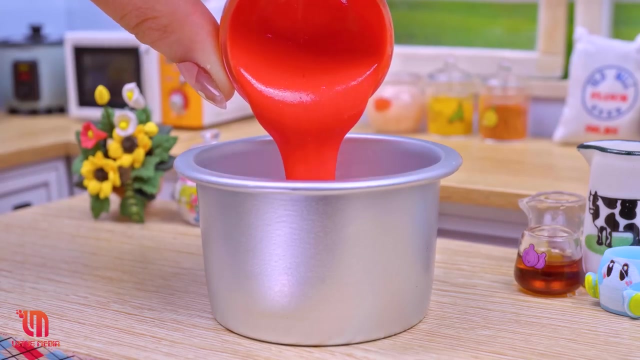 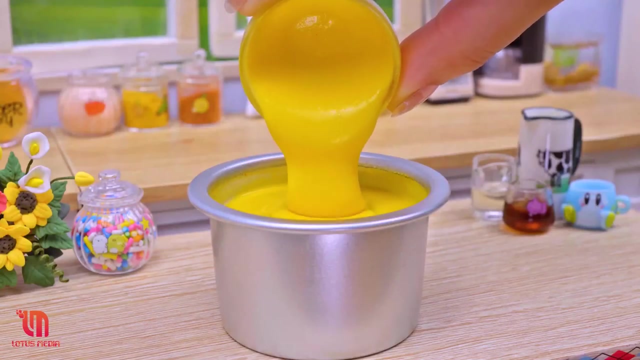 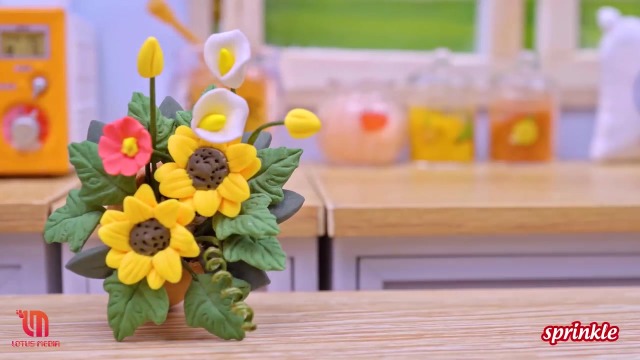 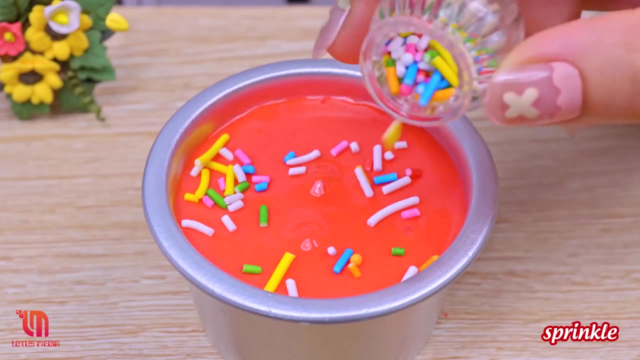 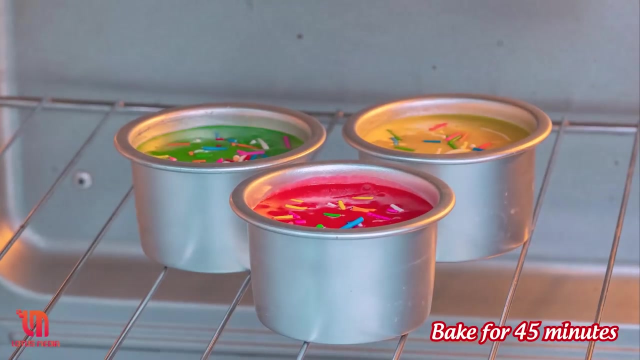 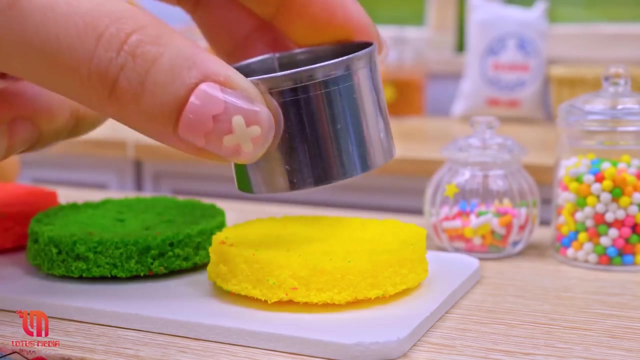 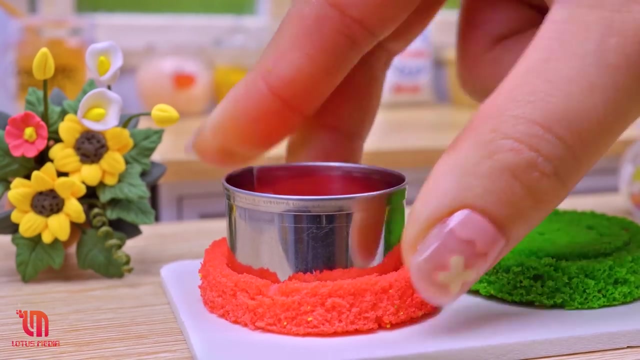 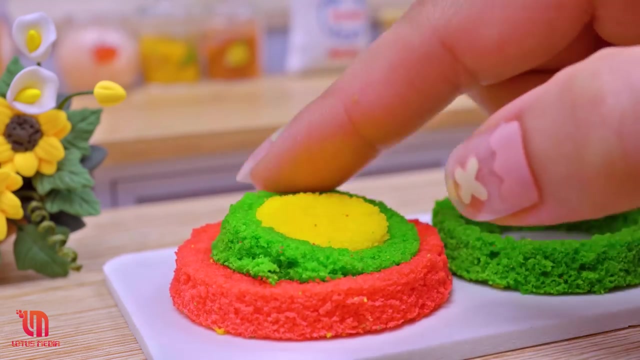